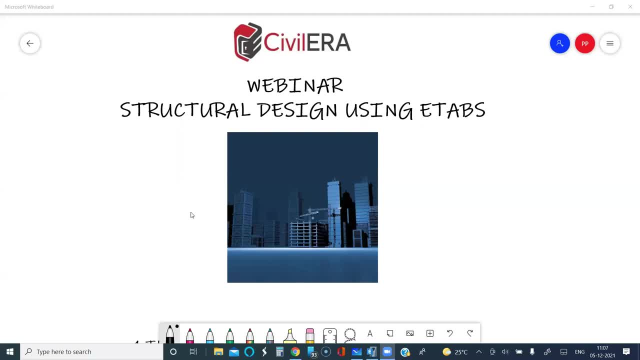 All right. Now, how many of you think that you also need structural concepts along with ETAPs To be a master Type? yes, again, Yes, Okay. so today, let's focus on certain points that will help you as well, which will: 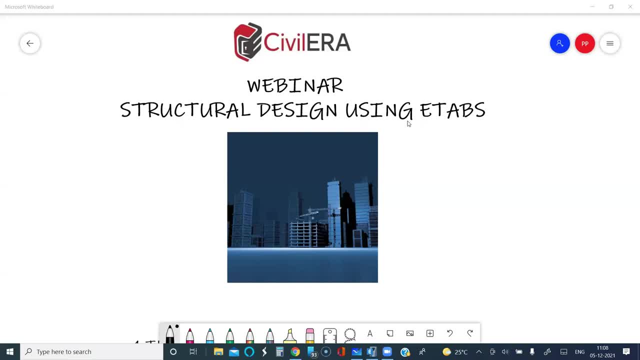 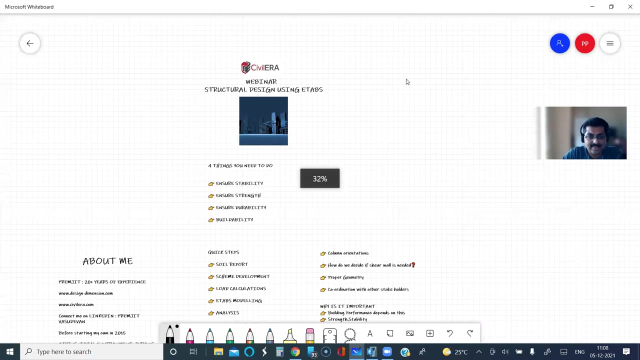 Lipun and Mudassir. I will give you an opportunity to speak later. at this point in time, Let us focus on ETAPs and other things. Okay, so before starting, let me quickly introduce myself. Some of you may be already knowing me. some of you may be completely new and may not be knowing. 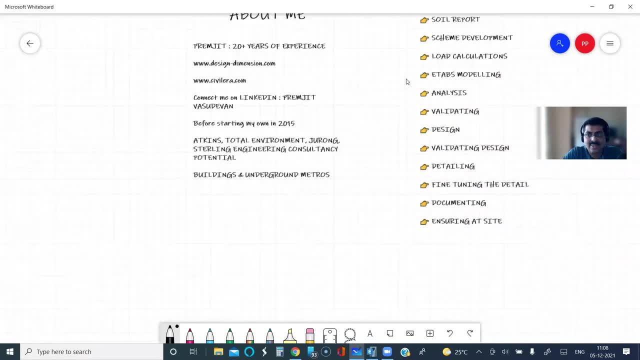 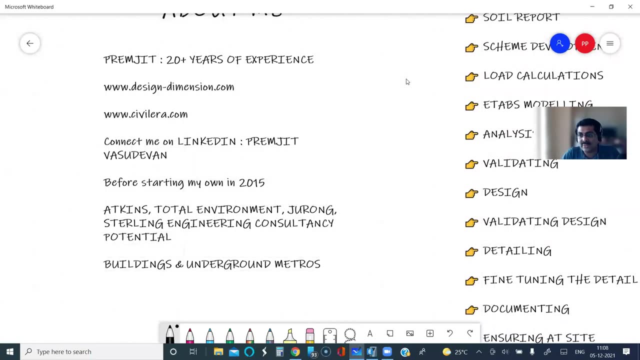 at all about me, So my name is Premjit. I'm a structural consultant, And I have given a brief about me here. I have about 20 years of experience working with various organizations, And I started my consulting practice in 2015.. And prior to that, I have been working with companies like Atkins. 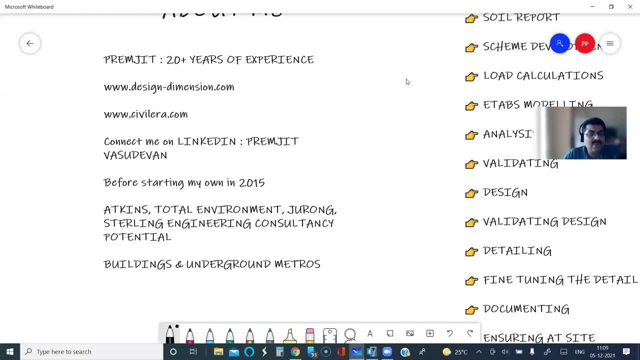 if you know them, and Total Environment, Durong, Sterling Engineering Consultancy and Potential Services Consultants. So most of my work has been with Atkins. I have been there for a long time And I have been working with Atkins for a long time, So I have worked with Atkins for 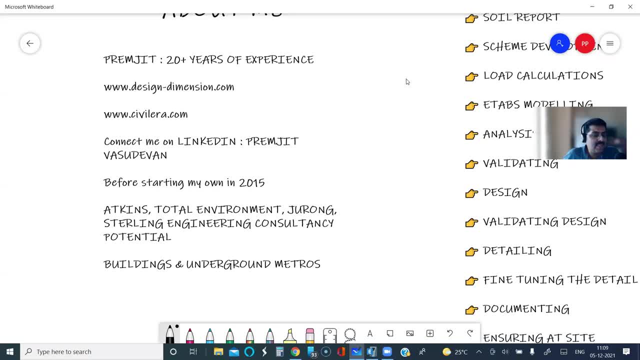 time and have been working in building projects based in Dubai and also in UK and a lot of underground metros stations, So this is my expertise. I'm an expert in building structures and metros And before starting my own in 2015,, I started off as a consultant in Bangalore and 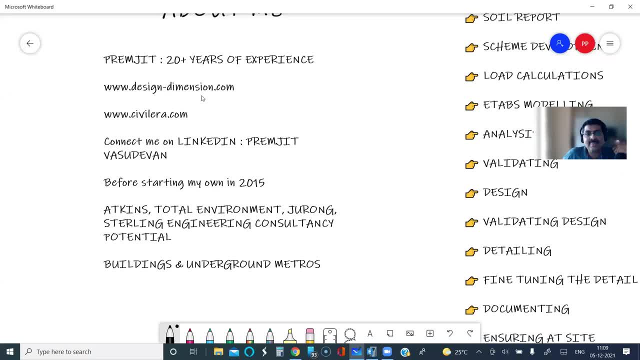 Kochi and Design Dimension. This is my website where we consult building projects Now off. late in 2015 itself, we diversified and started our training brand under Civil Era. So Civil Era is our training brand and Design Dimension is the consulting office. So that's a quick brief about. 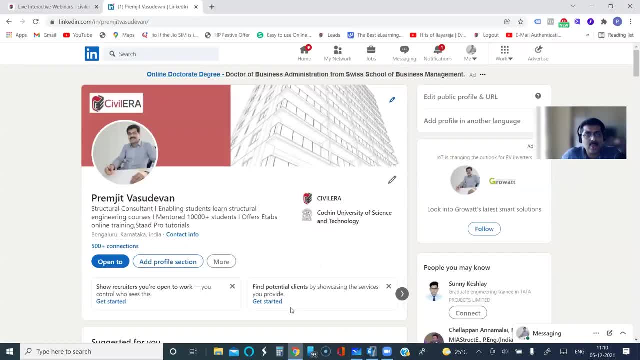 me. So in case, if you want to know more about me, what you can do is you can hop into LinkedIn and then LinkedIn Premjit Vasudevan. If you search, you will get me. you can connect me. I am an open network. I would like to connect to you And especially, I do post technical contents. 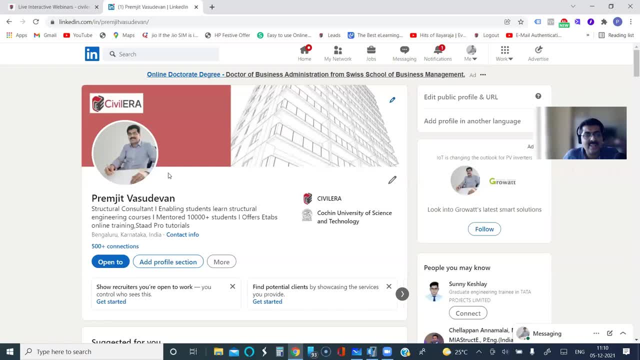 each and every day and try to educate students and learn from others as well. So you can connect me. you can feel free to connect me at Premjit Vasudevan in LinkedIn. So if you type, you will get me. some of you have already connected. 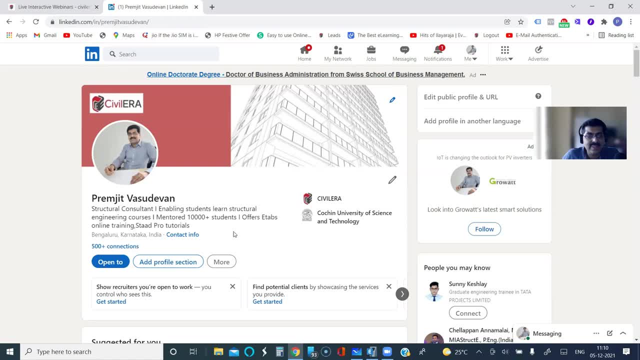 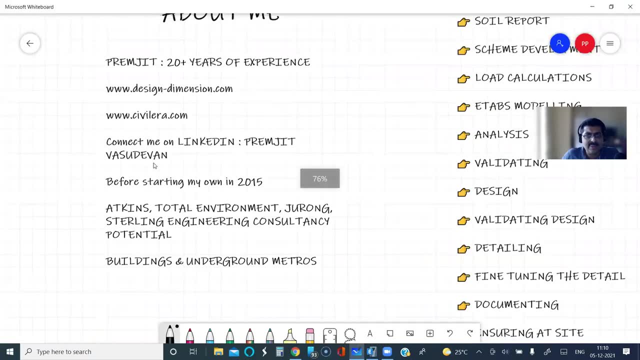 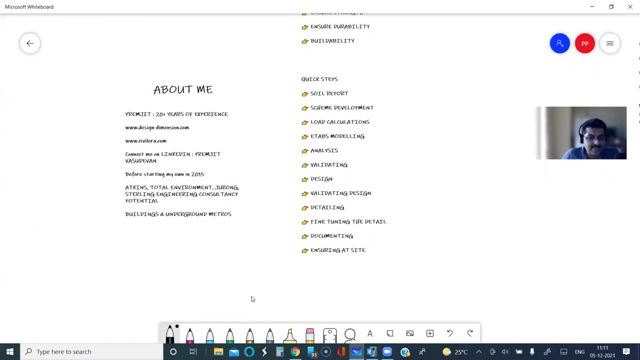 Happy to connect, you Happy to connect, and others who have not done that can also connect me here. So that's a quick brief about me. Now let us come to the topic we will discuss about ETABS Now. before getting into ETABS again, let me quickly tell you four things. that, as a structural 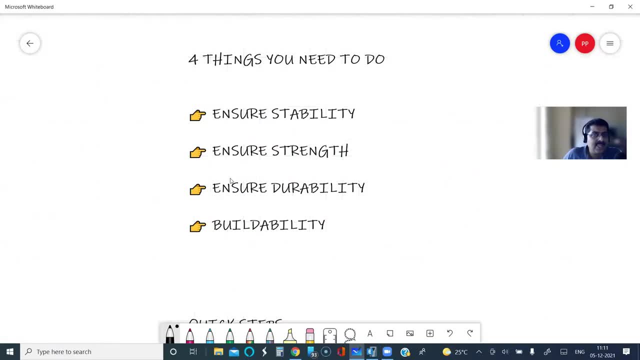 consultant or as an engineer. what is ETABS And what you have to do? Four things, minimal things that you need to do. one is that you need to ensure stability of the structure. So I had given you a free course, which would have given you a good idea on what 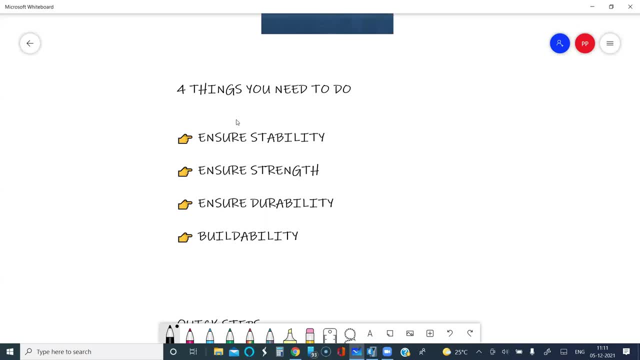 stability is now how to ensure that stability. You will have to go deep into it. some of the some of the things I had given you an idea on, what are the things that you need to look into? to instability. Then you need to ensure strength, the strength of your building. Now, how do you? 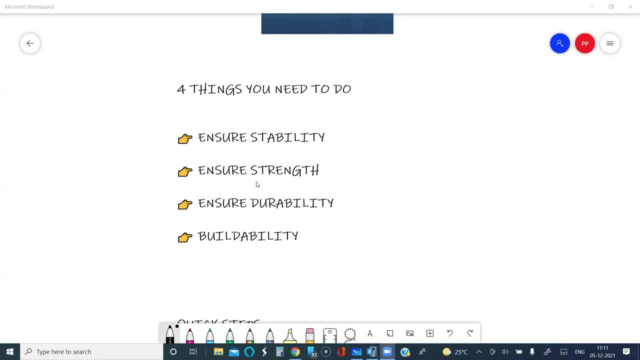 ensure strength of your building, That ETAPS helps a lot. Now will ETAPS help you in ensuring stability A little bit, not a lot. Yeah, there are a lot of things that you have to do manually if you have to ensure stability of your structure. It is not completely possible by ETAPS alone. 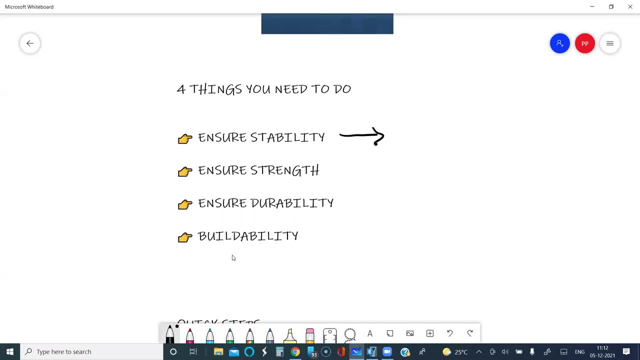 You need a combination of your own knowledge and ETAPS. I hope you can see my screen. Please type yes if you can Type no if you are not able to see the screen where I am sketching So you are able to see that right, All right, Okay, So ensuring. 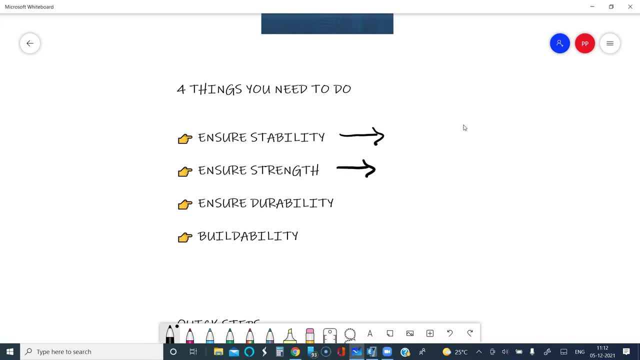 strength. This ETAPS helps a lot. You can design your structure, You can design your members. Everything can be done. Stability also: a lot of things like deflection, lateral deflection- everything ETAPS helps you Ensuring durability: No, you have to do it. All the code provisions. 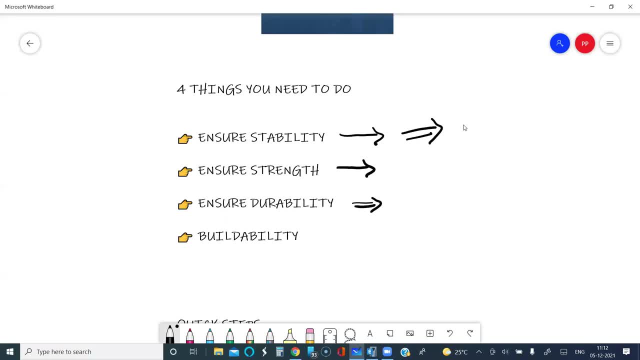 you need to know The maximum spacings. all that you need to know to decide the cover required. all that you need to know Buildability. No, ETAPS is not going to help you. You need to have experience to ensure that what you design is buildable. 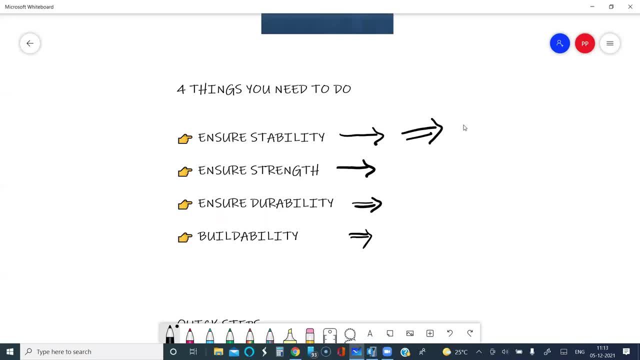 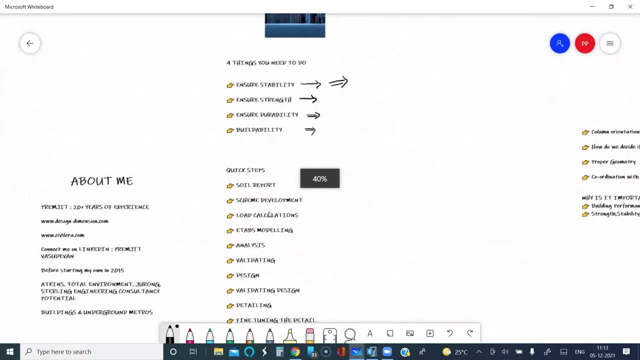 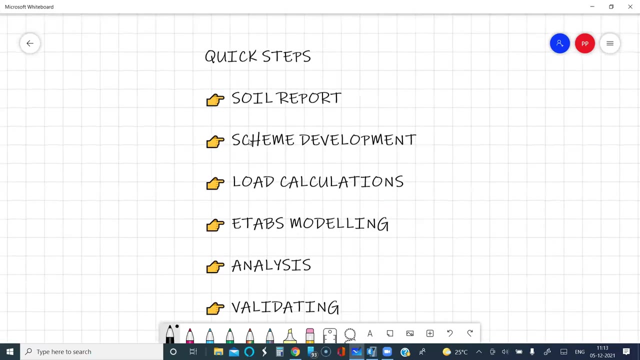 Yeah, So there are a few things that you need to know. There are a few things that ETAPS will help. You need to know a lot of things on your own before hopping into ETAPS. Okay, Now quick steps for successful project completion. Yeah, So you need to have a good understanding on soil report. 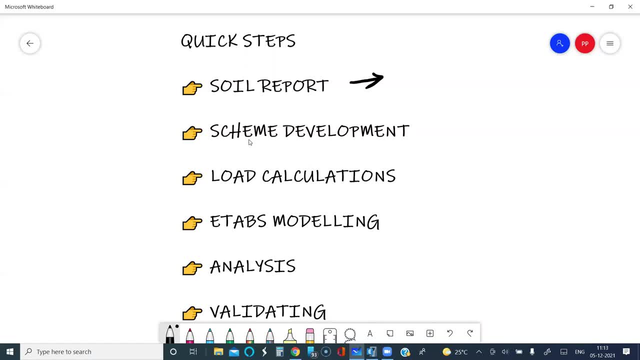 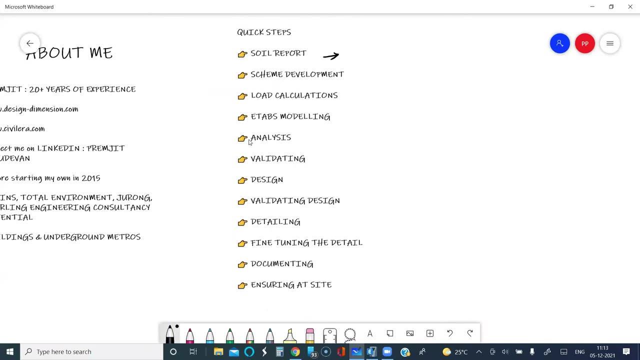 interpretations. Yeah, Without this you will not be able to be successful. I have given you a lot of videos and blogs in the Civil Era website. You can go and check that. If you want, you can post in the group and I will reply. if you don't find that, As a structural consultant, you need minimal. 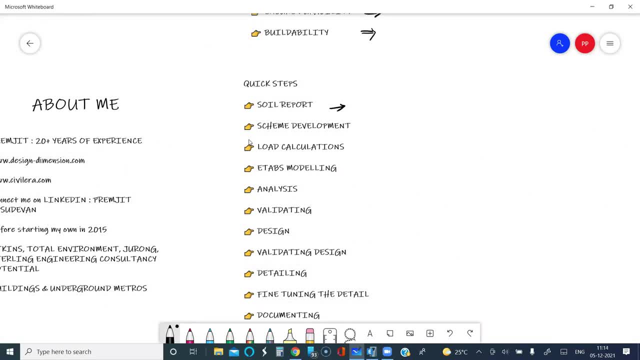 understanding of soil report investigation. And this needs to be done prior to start of project because sometimes your column positions and the numbers depends on the soil type. So ensure that you have a good understanding of the soil type. So ensure that you have a good 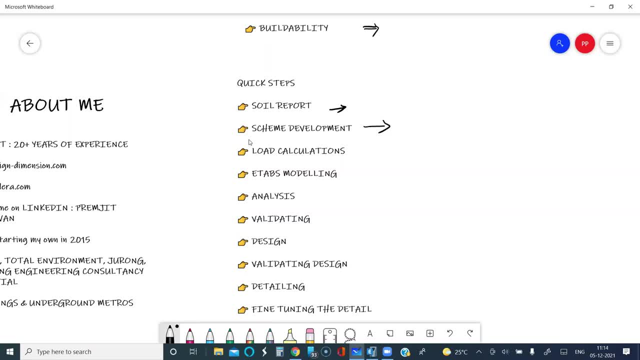 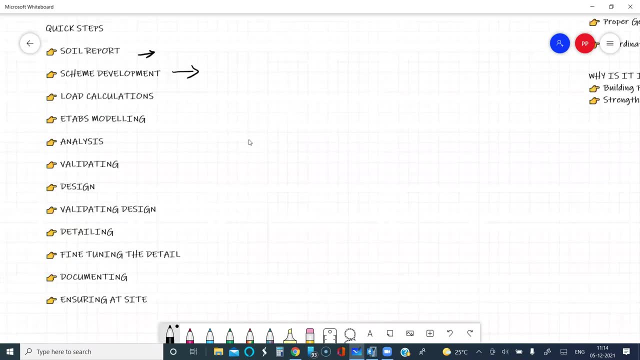 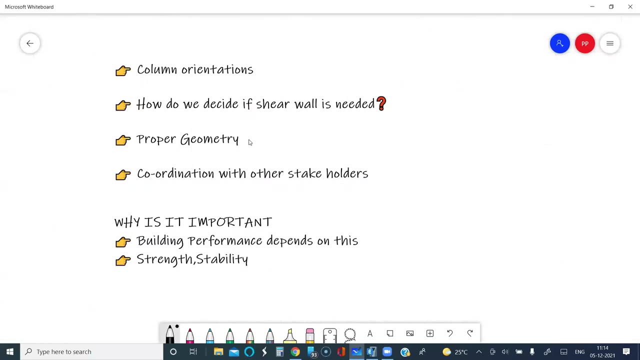 understanding of the soil type. So ensure you have that skill. Scheme development: This is one of the most important aspect. Yeah, Without a good scheme- when I say scheme, it means deciding your column orientation positions- How do we decide if shear walls are needed? ETAPS is not going to tell you. 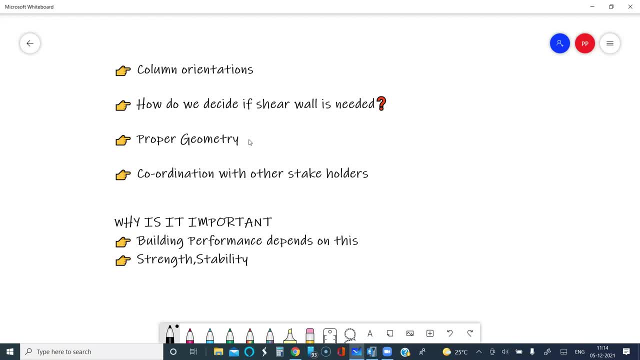 this: You can use ETAPS to check if your orientation is correct. You can use ETAPS to decide if shear wall is needed, but then it won't tell you that it's needed. So you need to know how to decide that, how to use ETAPS for that Proper geometry. Can you have an L-shaped building? Do you need to? 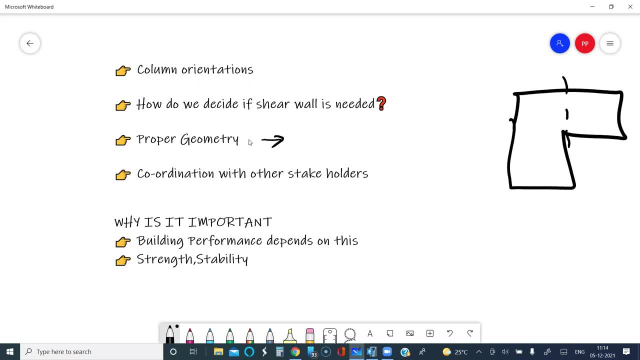 split this into two to make it regular, Or is it fine to have an L-shape? Things like that, Coordination with other stakeholders like architects, clients, electrical engineers, plumbing engineers and all that, Yeah, So all this comes with your understanding of the structure. 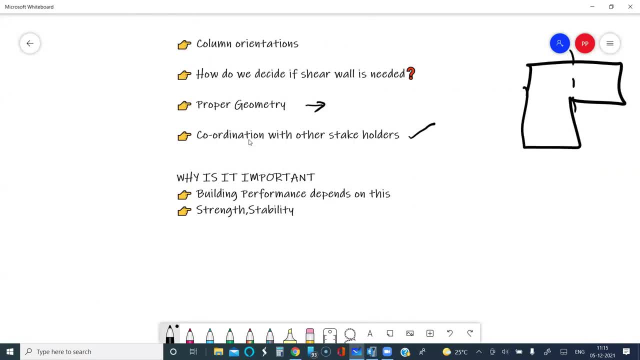 ETAPS will not tell you all this. Why is it important? Building performance depends on your scheme. Yeah, The greater the scheme, the easier you can design and make it work, And you will hit economy as well if your scheme is really robust. So the paramount thing is to 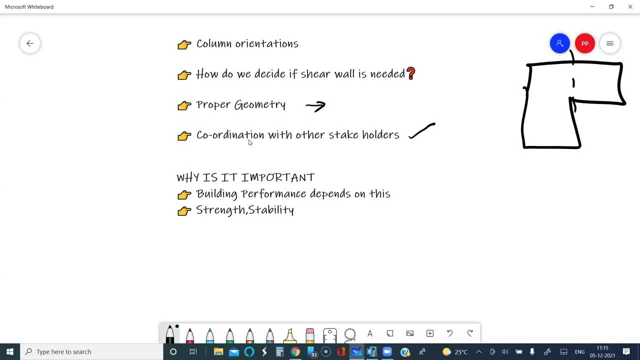 have a great scheme. If you don't know how to scheme a building, if you are doubtful, if you just don't think that you get a plan- architect gave you a plan- you can start straightaway modeling. No, you can't. You need to put in your structural principles. 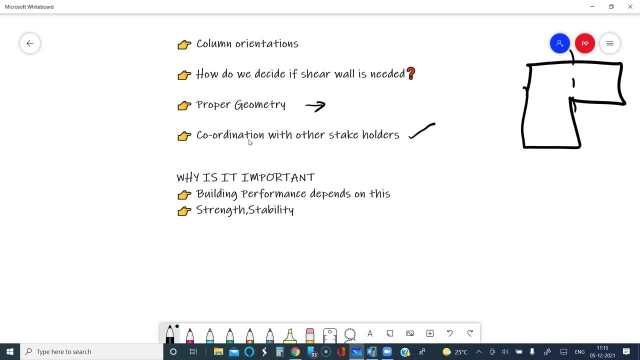 into play and then decide your scheme and then do a trial and error in ETAPS and arrive at the final scheme. Yeah, So that is your main skill needed, not modeling, And strength and stability completely depends on your scheme. The better your scheme, the easier you can. 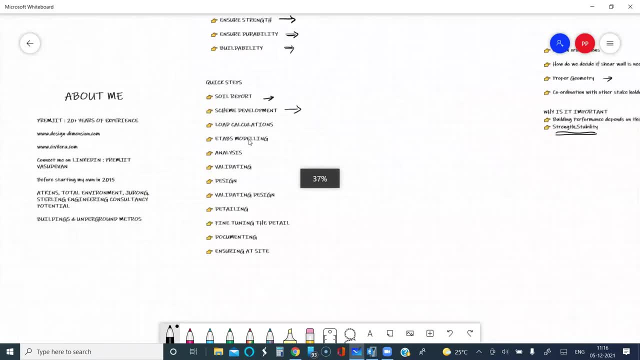 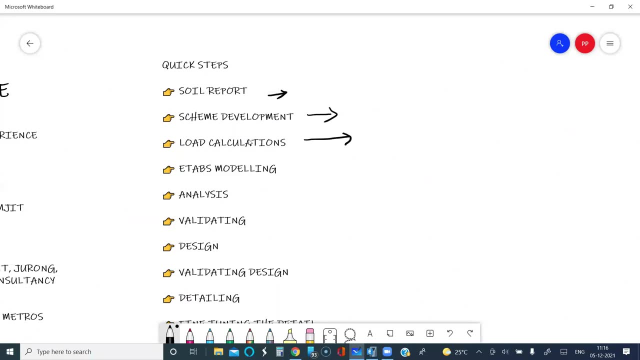 handle all these complications. Okay, So moving forward, you need to have a good structure. So you need to have a good structure. So you need to have a good structure. So you also need to know how to calculate loads: water tank loads, staircase loads- yeah, 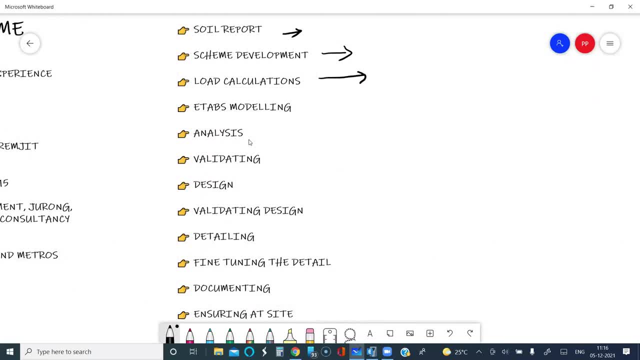 kilonewton or kilonewton per meter, per meter square, what I need to take. If there is a truss on top of your building, should I model it or should I take the load of that? wind load, seismic load? all this you need to know. Yeah, Now, some of you may be knowing about that Some. 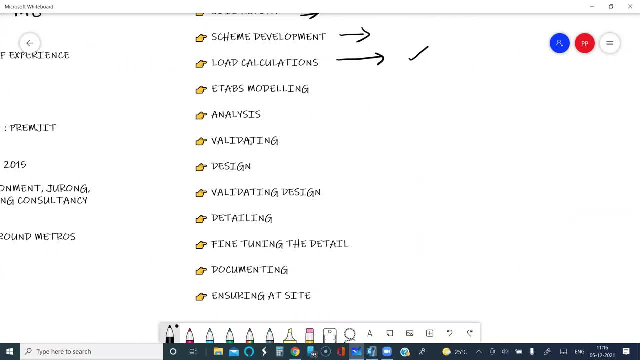 of you may be not knowing about that- How to take the retaining wall weight. I mean the soil retention weight. should that be included in the analysis? So you need to know how to calculate the soil retention weight. I mean the soil retention weight. should that be included in the analysis? So you need to know how to calculate. 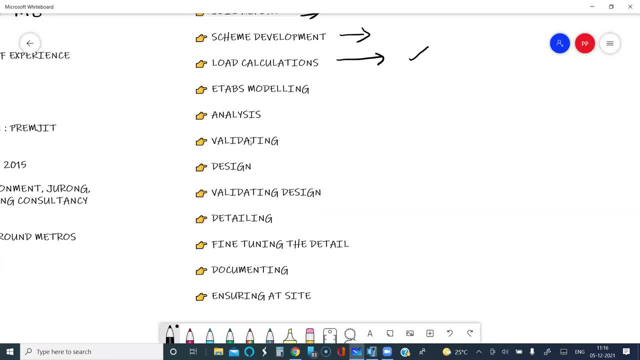 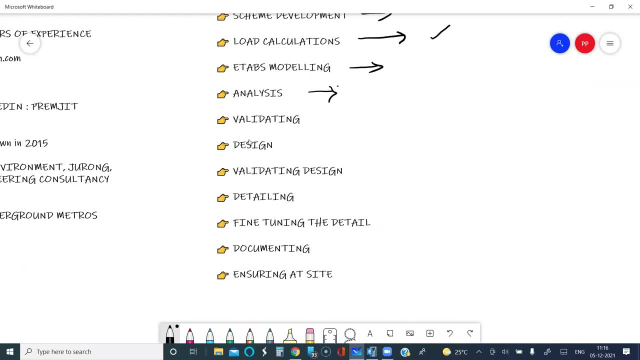 or can I ignore that things like that? ETABS: modeling: it is fairly simple. Analysis: it's fairly simple, but then you need to know how to validate your analysis. That comes with your structural understanding. Design: very simple in ETABS, but you need to know what parameters you 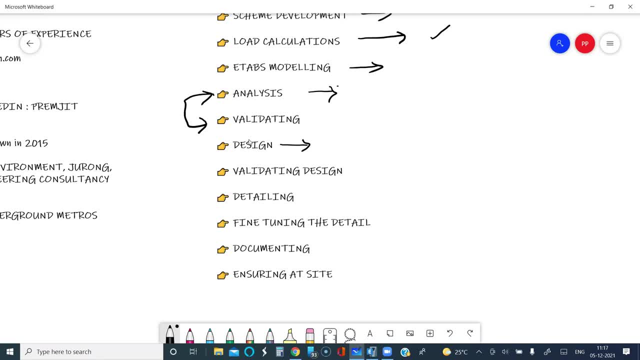 need to give what say, for example, effective length of column. How do you decide that? Can you leave it to ETABS? Should you give an input? Is it floor-to-floor height? Is it more than that? Many people take it from table 26,, 26 or 28,- I forgot in IS456- and take that both ends are. 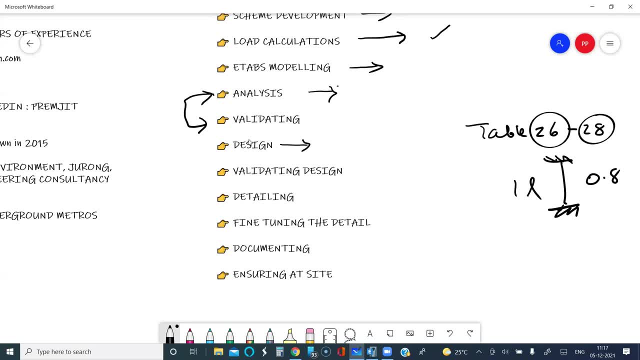 fixed and then take 0.8 or one time the height of the floor. That's wrong. That's not the way you have to design a column. There are much more than that. So if you know all that, it becomes simpler. 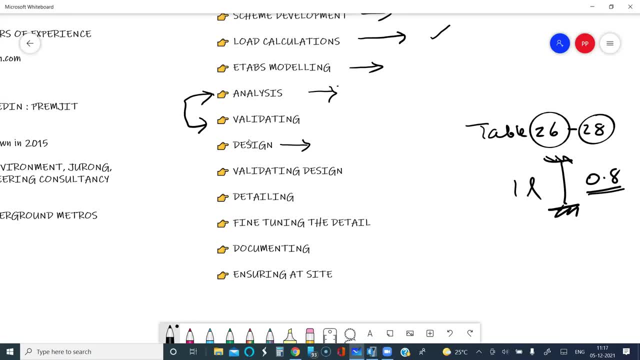 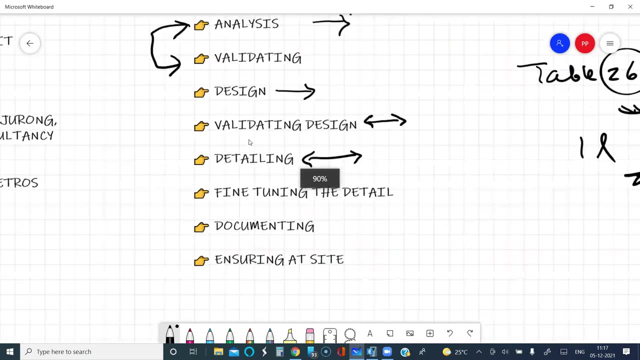 for you to Design, Then validating your design by hand calculations. Detailing. It's very important because detailing speaks about your design. Your client is not knowing how good you are in ETABS. Your client will not know how good you are in load calculations. Your client only sees your. 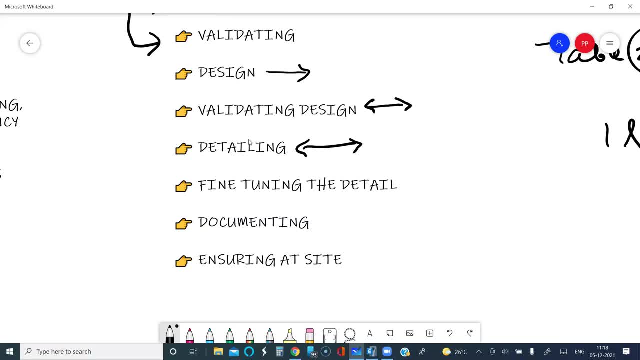 drawing, and your drawing needs to convey what you want to convey. If you don't do that, you will be always underrated. So, as a structural engineer, detailing is something which people generally ignore, but I would encourage you to focus on that as well, because detailing makes you perfect. 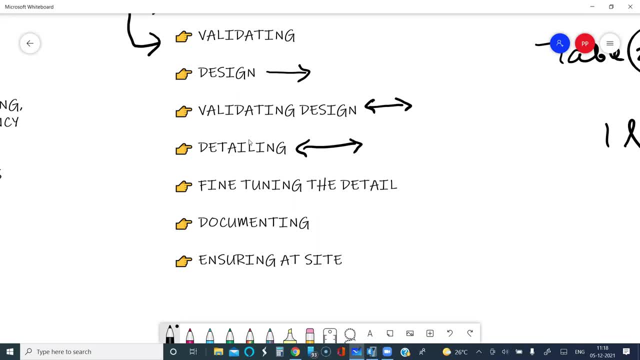 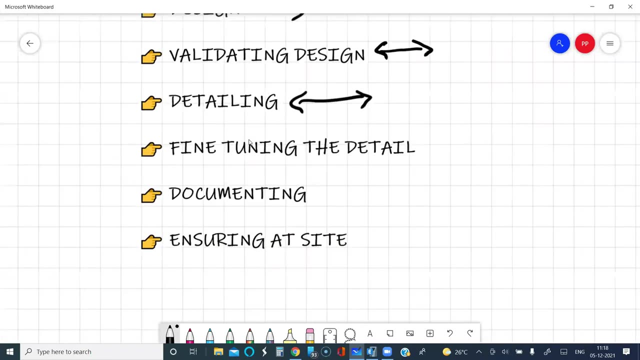 The design intent is conveyed to site only by detailing, So your drawing speaks for you. What good work you have done in ETABS can go 100% wrong if your detailing is wrong or if your detailing is not conveying in the right way. So focus on that: Fine-tuning the detailing. 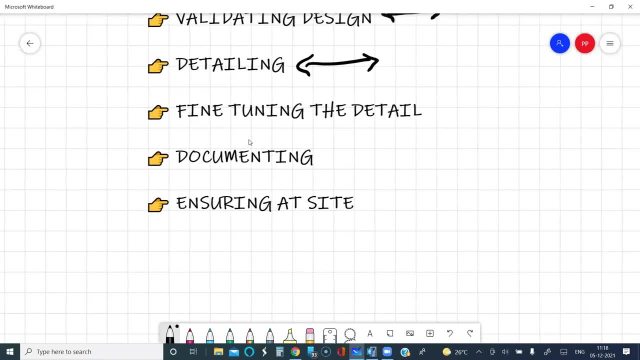 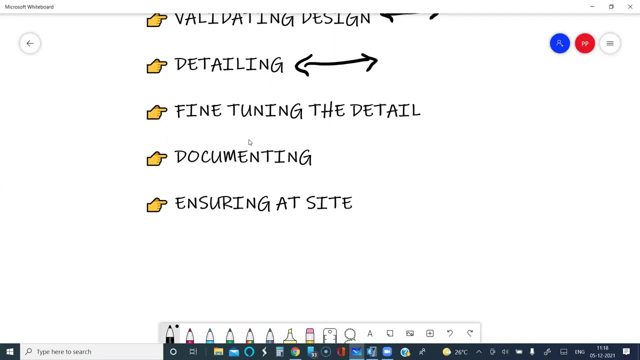 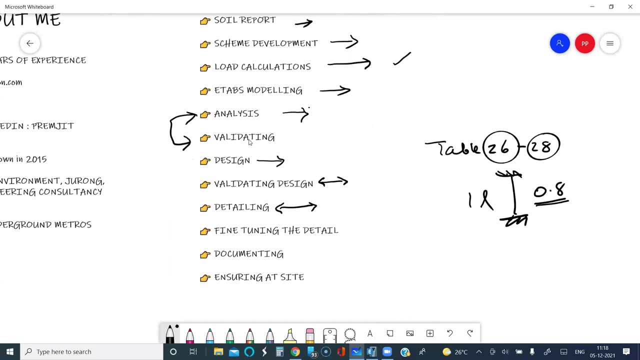 documenting what you did, your load calculations and your detailing. All that needs to be done And ensure that what you have designed is done at site. So this can be improved by a great level of detailing. If your detailing is great, then site engineers or site. 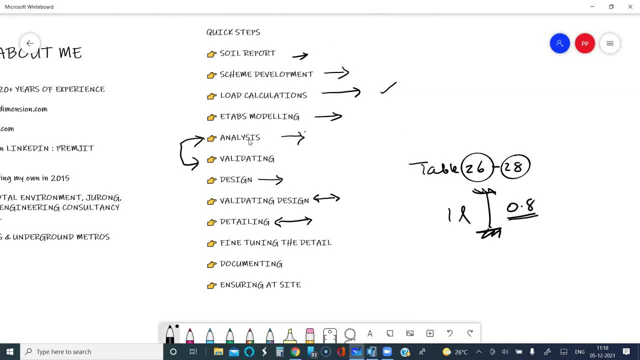 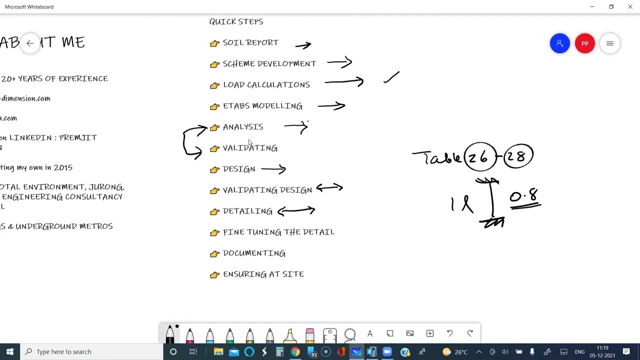 people will understand what you want and they will do it better. So your interventions at site, your site questions that you get by call, or the number of site visits that you have to make will drastically reduce if your drawing quality is great, If you convey things, 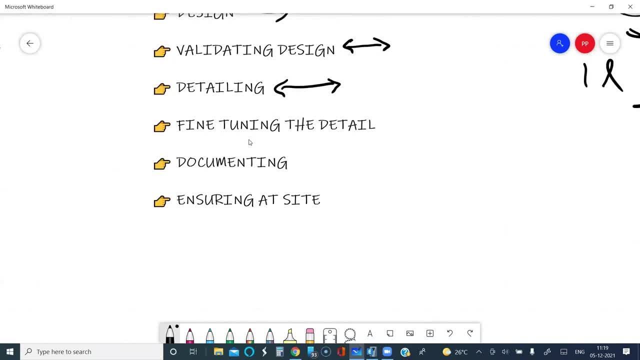 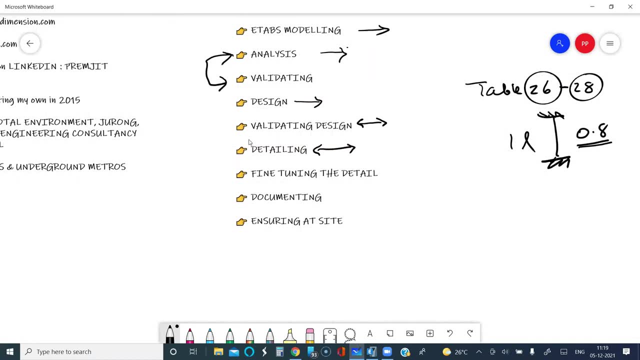 in the right manner. You can use tools like Revit for 3D detailing also and make your design workflow great. I use only two tools for my consulting- maybe three ETABS, Revit and AutoCAD. I don't need anything more And I have fully automated my design cycle with minimal intervention. 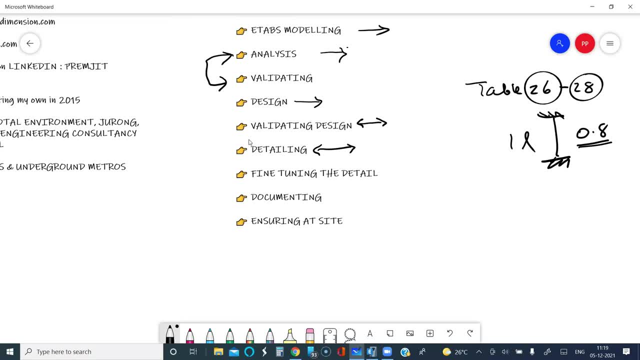 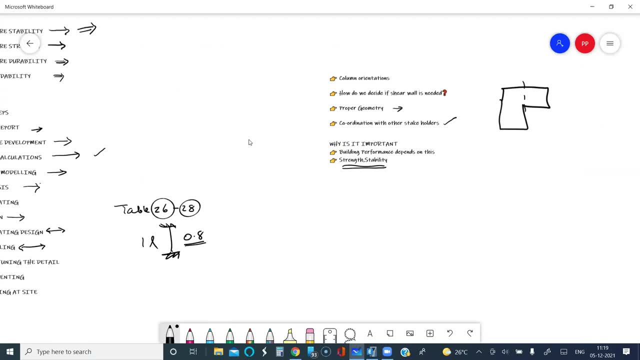 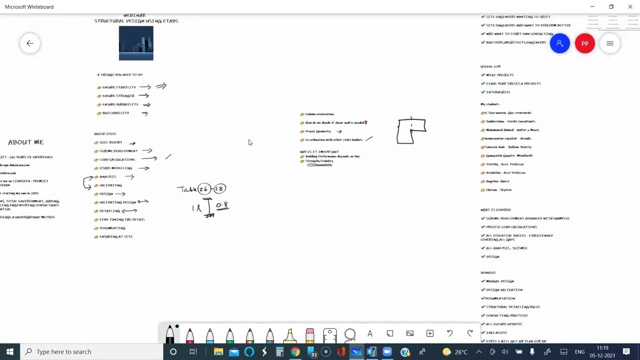 from me. So that's how you need to do as a young engineer: smart, technically right, no compromises. That should be your motto, And there is nothing wrong in using ETABS and other software in your workflow. Everything need not be manual, but you need. 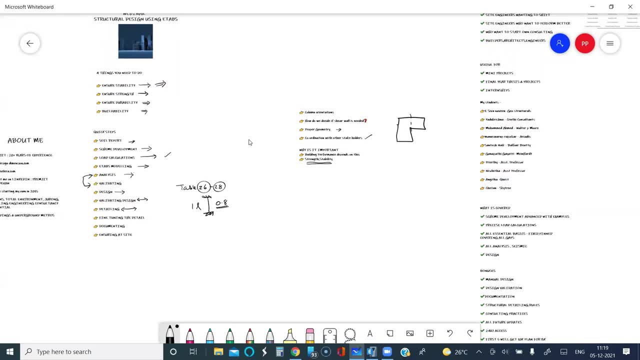 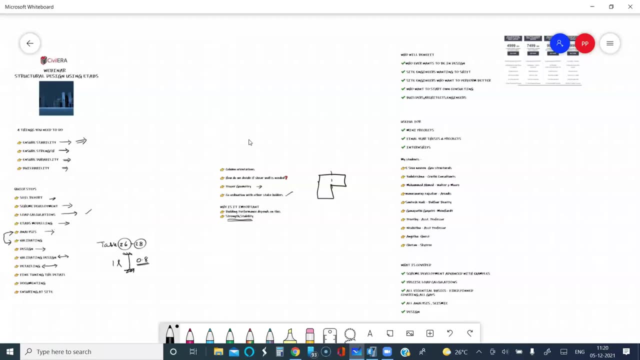 to be sure that what you're doing is 100% correct, ethical and with no compromise. If you are able to do it, you can use software or any automation in your workflow. Fine, So now let's come to ETABS. 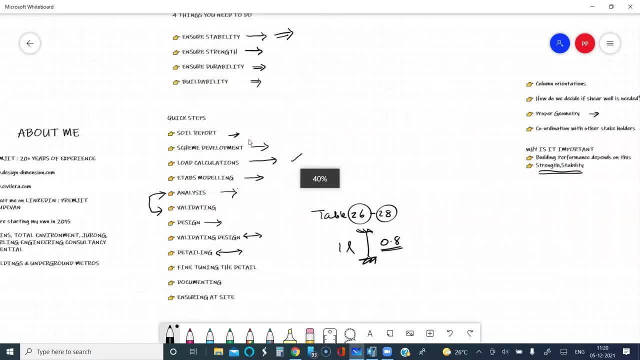 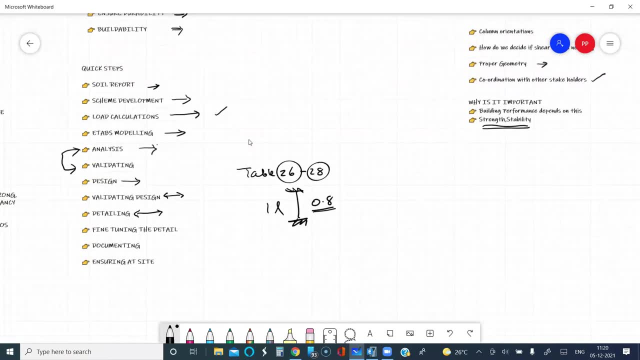 I'm not wasting your time more, but I have already told you only valid things. so, on what you need to focus. It may not be ETABS, but that's more important than ETABS. So quickly coming to ETABS, there are limitations with respect to time, So I have taken a small 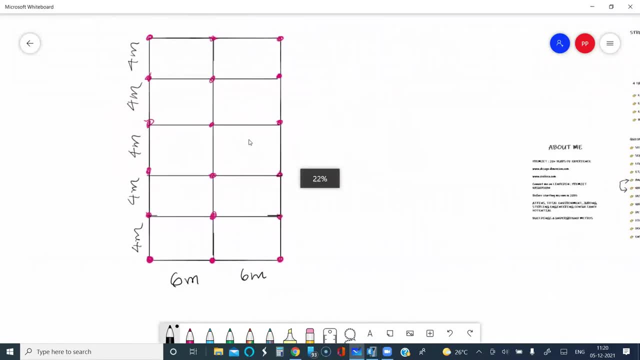 building or a plan I have given here. I'm going to show you how to model this. Yeah, So let's take something like G plus how many you want, G plus 5 or G plus 10, let it be G plus 10.. Okay, So this is what I'm going to do right now. 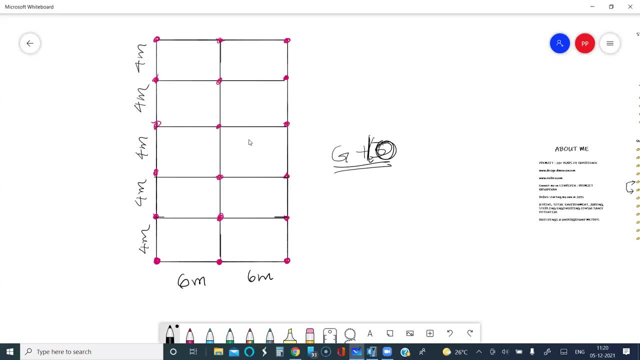 And I have given the plan here. In general, this plan you will have to make it depending upon your architectural plan and the client requirement. You have to coordinate and make it. Most of the times you are on board after the architectural drawings are made. but a very good. 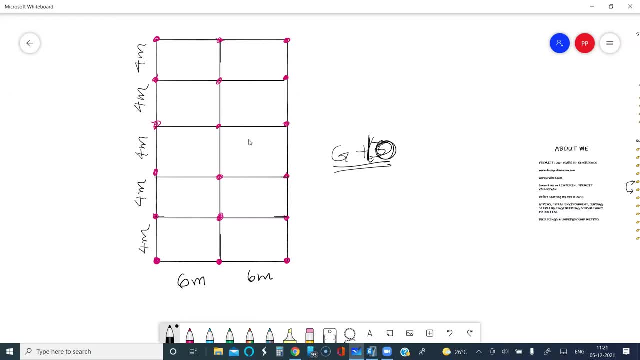 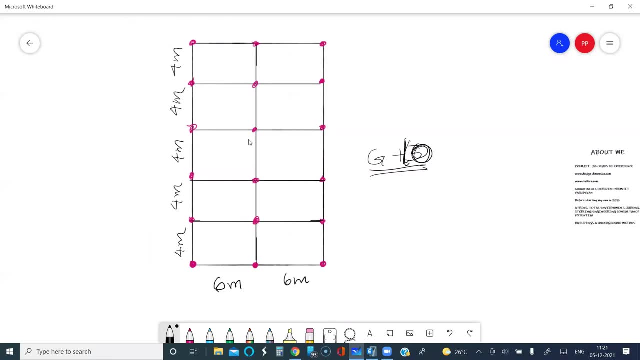 project and very good architect and very good client would employ you much before this architectural scheme is made, so that your inputs are taken and that's incorporated in the architectural plan and the structure behaves better. So the good clients will do that. Many may not do that. You will get an architectural drawing and that's when you are. 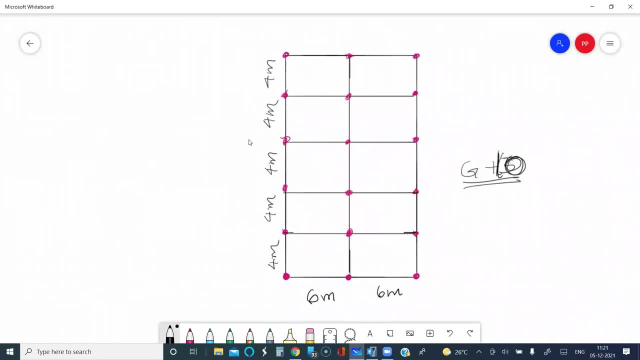 going to start working on it, So that becomes like rectifying mistakes rather than providing a great robust scheme. You will be working on a restricted plan. Anyways, I'm not going to get into it right now, So let's focus on what we have. We have a building. I have given a plan here. It's. 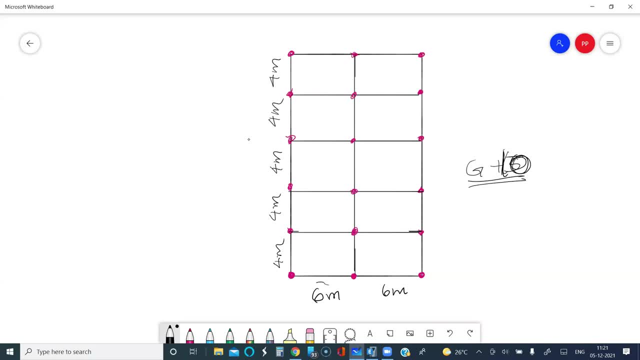 a simple plan. We are going to do G plus 10.. I have given the span here 6 meter. 6 meter, 4 meter in the other direction. So this is what we are going to do right now. Now with respect to numbers. 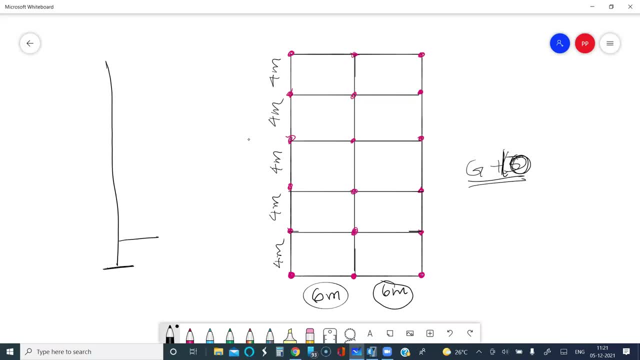 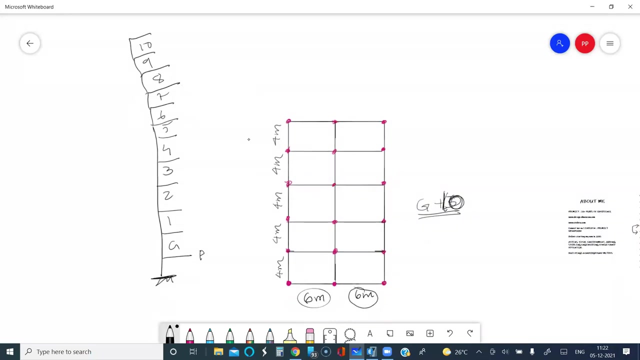 number of floors. you will have a foundation. You will have a plinth Ground: 1, 2,, 3,, 4,, 5,, 6,, 7,, 8,, 9,, 10.. So, as a young beginning engineer, always sketch a section like this so that you don't mess. 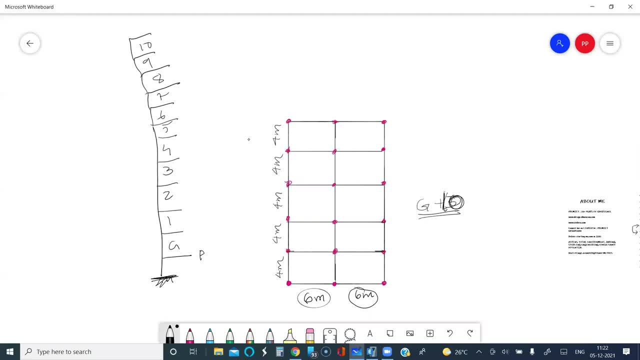 up with the number of floors. So foundation in ETABS is not considered as a level, It's a foundation. So you will have 1,, 2,, 3,, 4,, 5,, 6,, 7,, 8,, 9,, 10,, 11,, 12 levels for a 10-floor building. 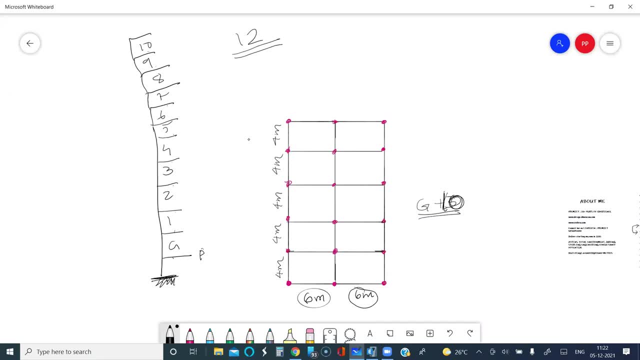 Now, as a beginner, you can either accidentally reduce one or increase one, So be sure that you sketch like this so that you know how many number of floors are needed. You need a plinth level. You will have beams at the plinth level. and you will also have a terrace, So you will have 12 levels needed. I think I have made a mistake. Yes or no? No, because this portion is under the ground. Yeah, So ground 2, this is not a floor. That will be say something like 1.5 to 2 meter, depending upon the soil. 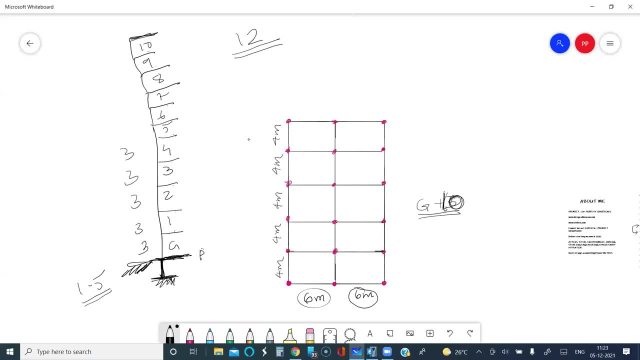 conditions. All other things are going to be 3.. Yeah, So you can count the floor ground: 1,, 2,, 3,, 4,, 5,, 6,, 7,, 8,, 9,, 10.. You need 12 slabs or 12 levels in ETABS. So let's do that. So. 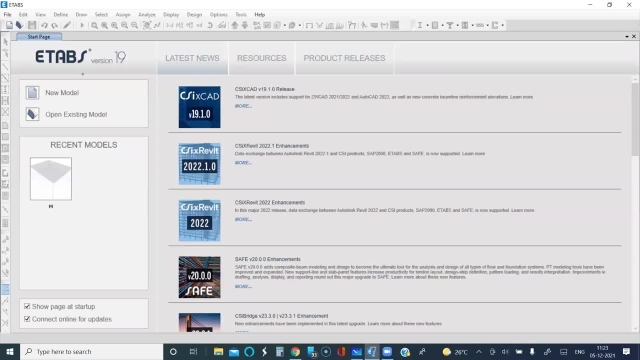 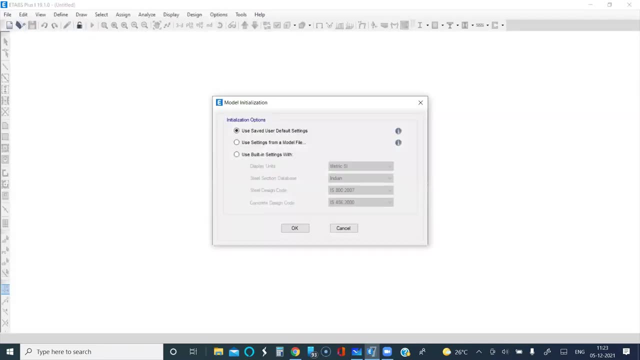 I'm going to get into ETABS and I'm using the latest version And I will go to file and then say: new model. Okay, Now here there are three options. I'm not going to detaily say this because it will take time. We have to complete. I had given you. 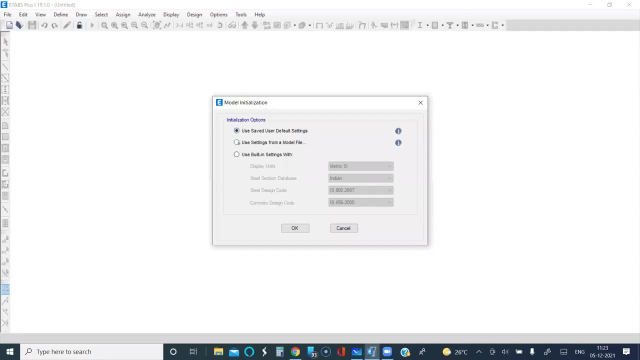 one link yesterday. in that it will be clear what to do with the other options. So here I'm going to use build settings with and then say metric SI. There may be many options. You are going to use system, international or international systems. Steel section database. Indian Steel design code. Indian Country design. 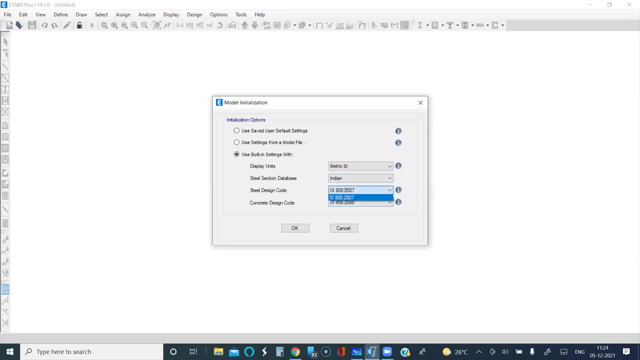 code Indian. In case, if you are wanting to use any other code, you will get different options here. If you are using a pirated, I encourage you to use an original, But then if you are using pirated or if you are using an ultimate version of ETABS with every design code supported, you. 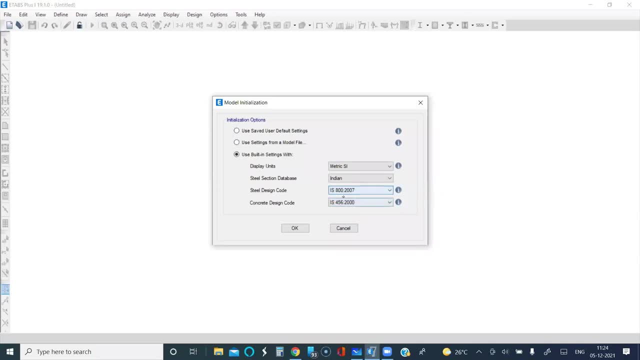 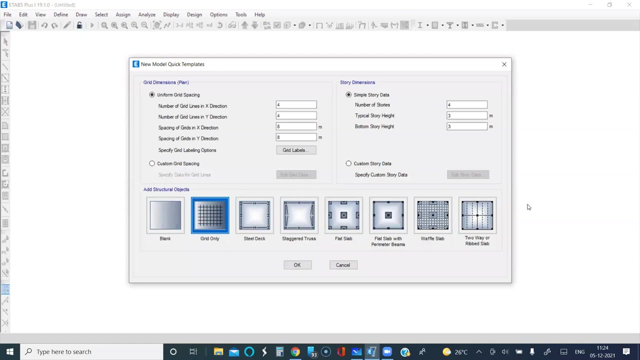 will get different options here and you can change here on different code. So you can use any other codes, But here I'm using an Indian version, So I have only the Indian codes. here I'm going to choose Indian codes and then say: all right, Now this tab. there are many options here. I would 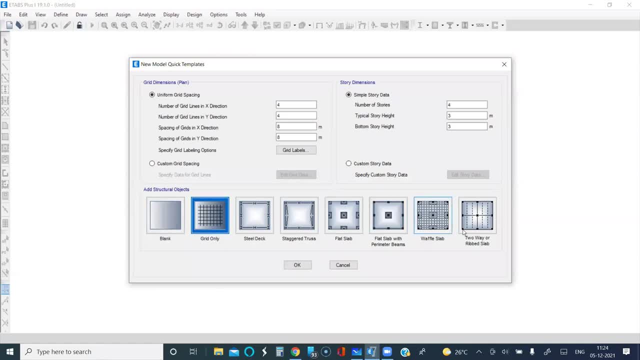 always ask you to go with grid only. I cannot explain you what are the uses of others. now, because there is time limitation, You can, for any general structure. you can go with grid only. You don't have to use any of it as a beginner or as an intermediate. Go with grid. 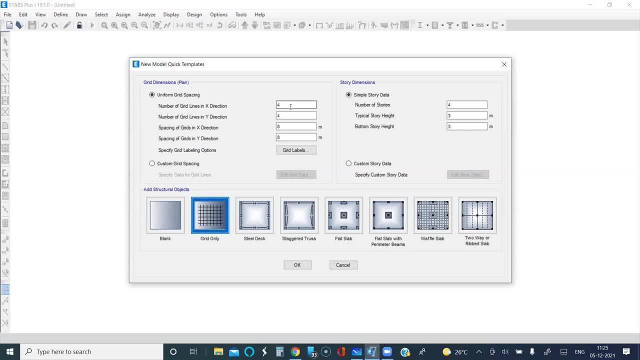 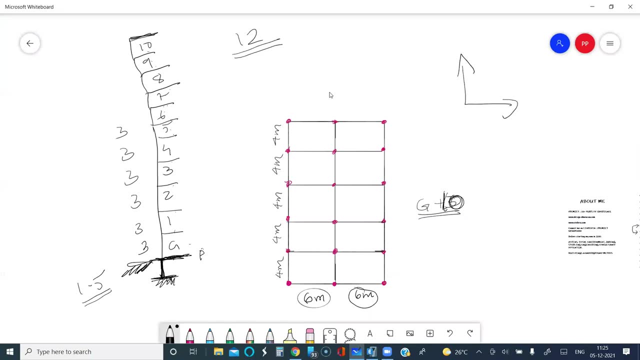 only Here it's asking you number of grid lines in X direction. So now your X direction in ETABS is: this is X, this is Y in plan And your height is Z, Just like your graph paper or just like your AutoCAD. So in X direction, you need three grids: One, two, three. This is your. 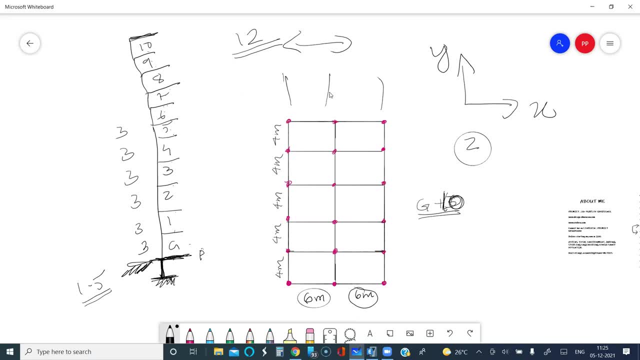 X direction. Grid is in Y direction, But along X you need three grids And along the other side you need three grids. So you need three grids. So you need three grids. So the other one, you need one, two, three, four, five, six grids: One, two, three, four, five. 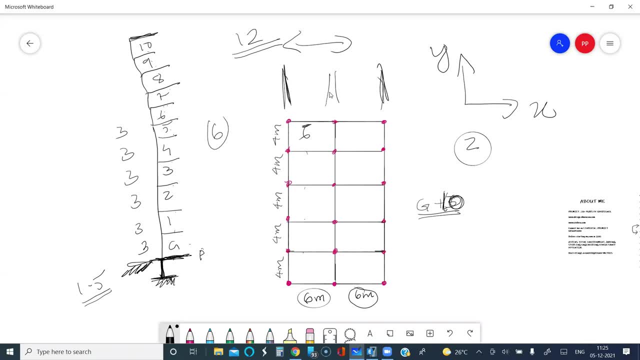 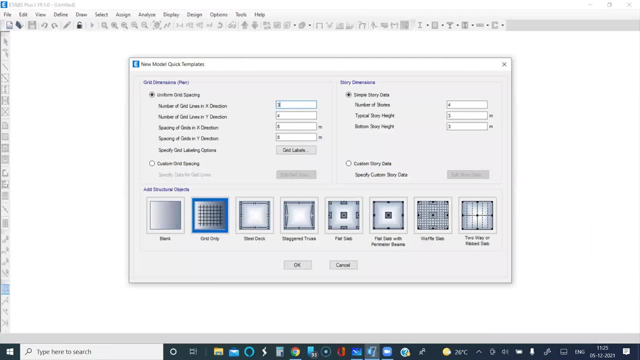 and six. Yeah, So three grids in X direction and six grids in Y direction. So I'm going to give three And here I'm going to give six. Spacing, let it be anything, But you know that it is. 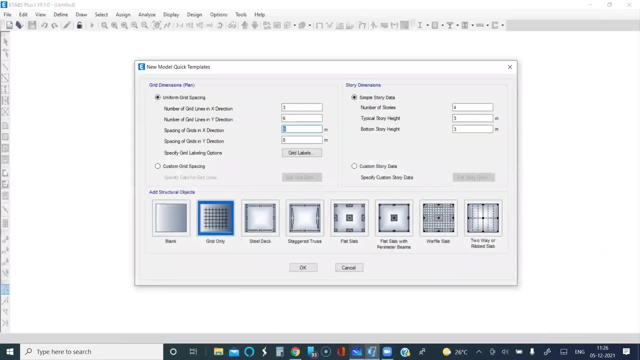 rounded off value. So I'm going to give it right here. You can also change it later, But then I'm going to give it right here. You can change it also if there is any problem. Number of stories: I have already told you 12.. Typical story: height: 3 meter. 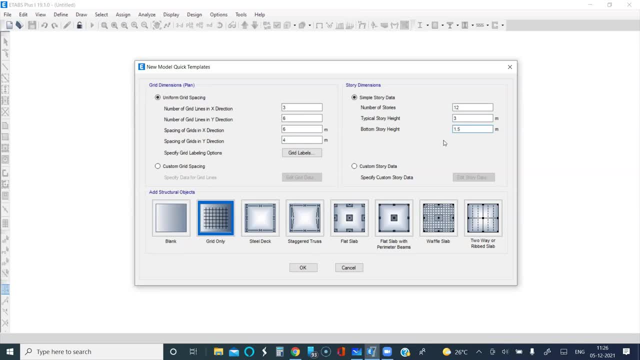 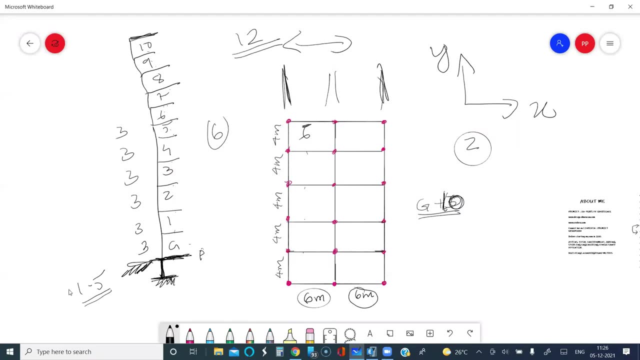 Bottom story: height 1.5.. Now, what is this 1.5?? From a foundation to plane. This need not be 1.5 always. It may change. It depends on the soil report. Okay, So it has. 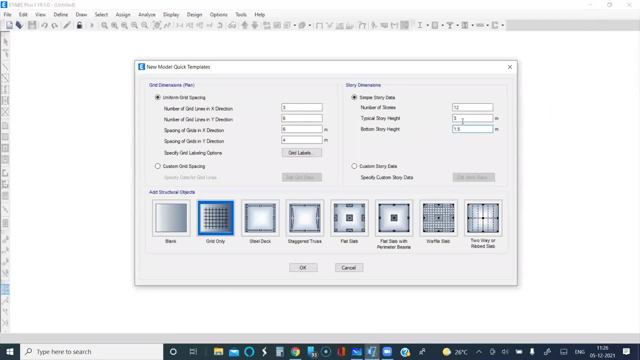 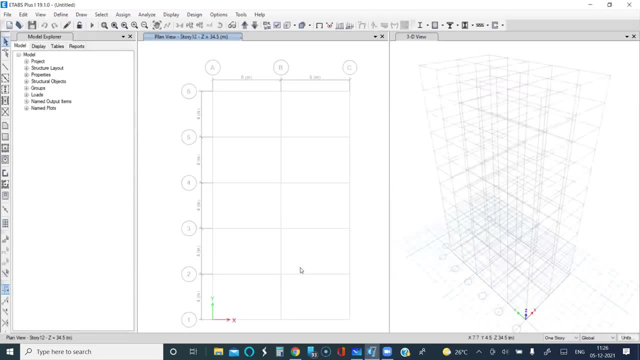 So it has a different level. It may be different, So they are giving you an option. All other floors, I'm giving three. Now I will say, okay, Yeah, So now your structural grid is done. You can see 6,, 6,, 4,, 4,, 4, 4.. Okay, Now you have three windows here: One, two and three. I would 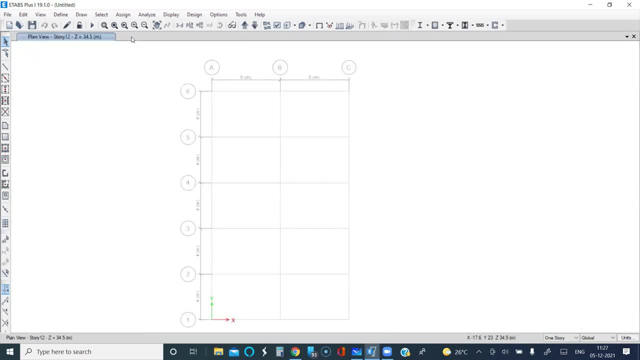 encourage you as a beginner, for lesser confusion, to close this. Now you have one window. As a beginner, I always encourage you to work in this, So you can see that you have three windows here In one window. Yeah, Now you have X, you have Y and Z. Also, you can see if you go to 3D view. 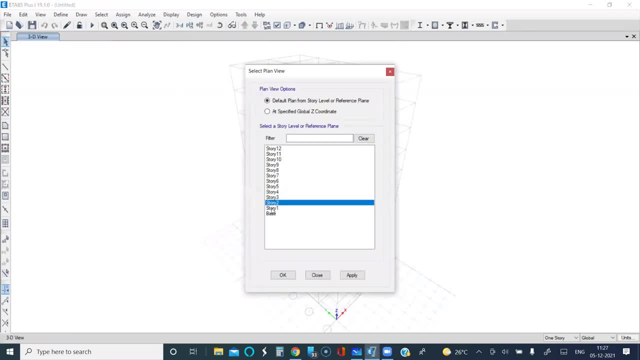 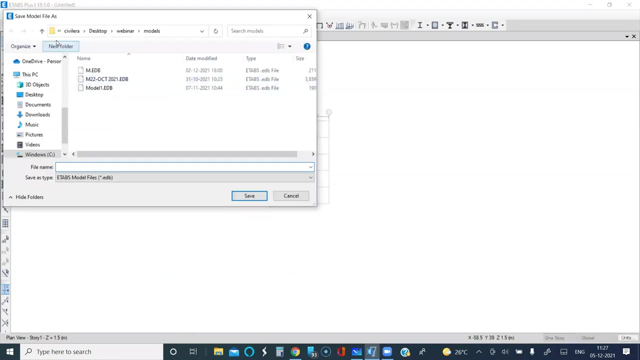 So you can see here I'm going to come back- Story 1. You can see 4 meter, 4 meter, 6 meter, 6 meter in one shot. I have got this. I'm going to save this. So I will save this as. 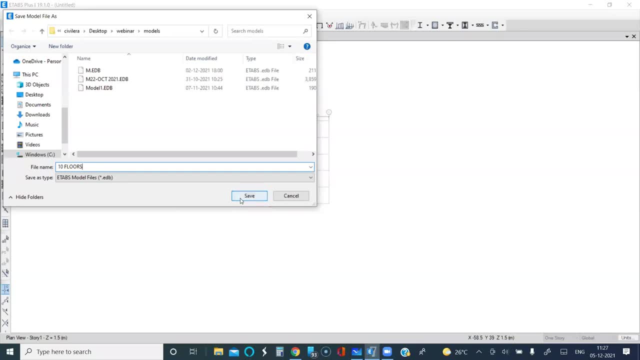 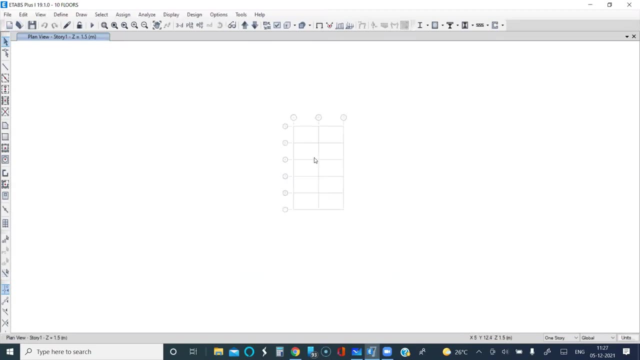 10 floors and save this All right. Now you have to do your modeling. Now, before getting into modeling, you have to decide your member sizes, your materials and all that. Okay, So, without wasting time, let's straight away head into define. So here, section properties: 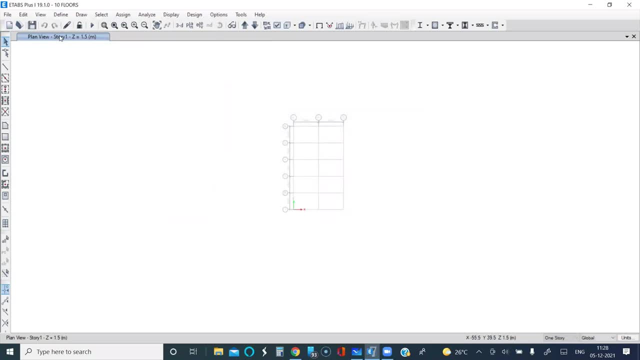 Name section or material properties. We can do material properties first. There are certain things here. Don't bother. I'm going to say add new material. Choose your location. material type: concrete Indian grade. Let's go with M20.. We can even go with M25.. You can go with M30. You. 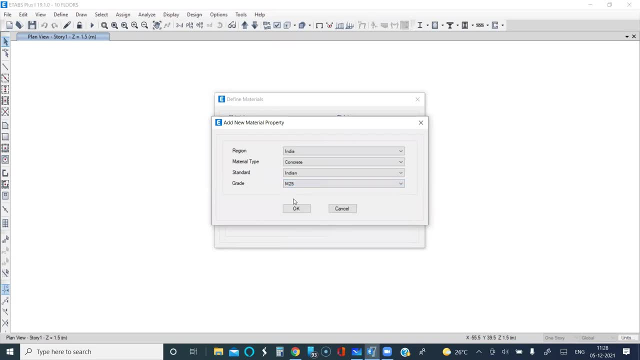 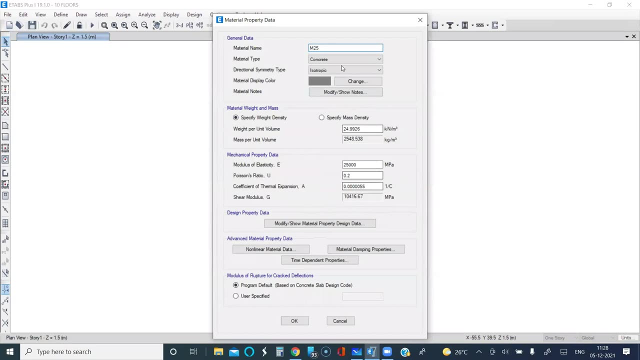 can go with M40. But then currently let us go with M25.. Okay, If it is not enough, we can change later. I'm going to say M25.. Every property of M25 will be automatically generated, So don't. 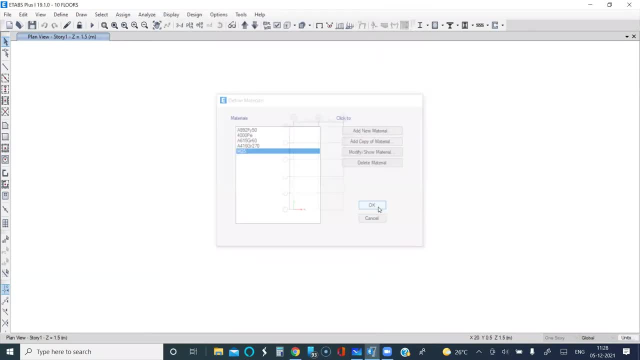 bother. Click on okay. Click on okay. Define material properties. Now you have to decide or define the material: steel or your reinforcement. Now in ATAPS there are rebar and steel. Always go with rebar. Steel is your structural steel. 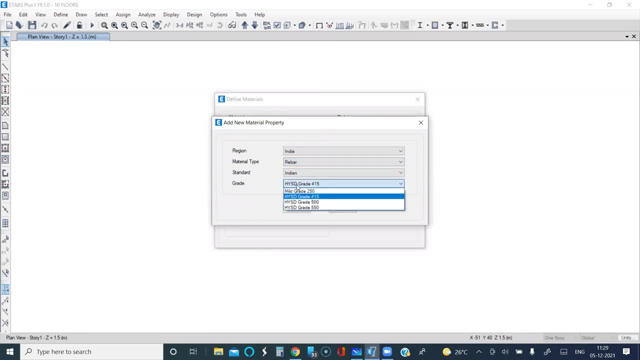 Rebar is your reinforcement, So go with rebar. I'm going to say 500 grade. I'm going to use So HYSD grade 500 define. Now define means it's like creating a library for later use. Yeah, I'm. 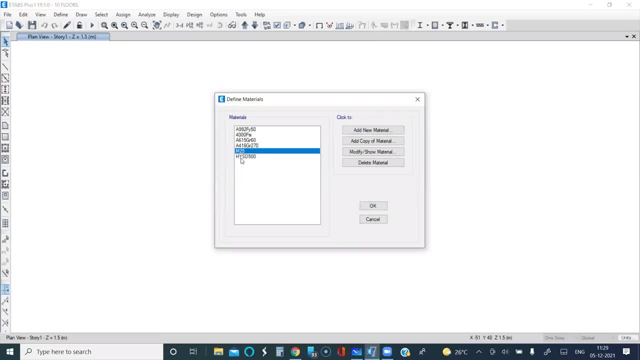 defining that I'm going to use these things in my project. It doesn't mean that I have modeled anything now. I'm just creating a library of materials. So if you want, you can create a 415 and M20 and M30,, M40 and keep it ready. You can create a library of materials. So if you. 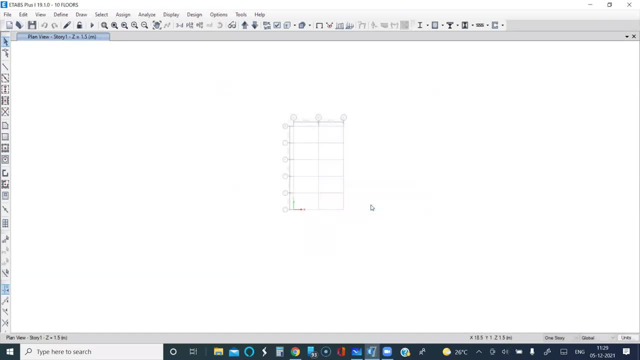 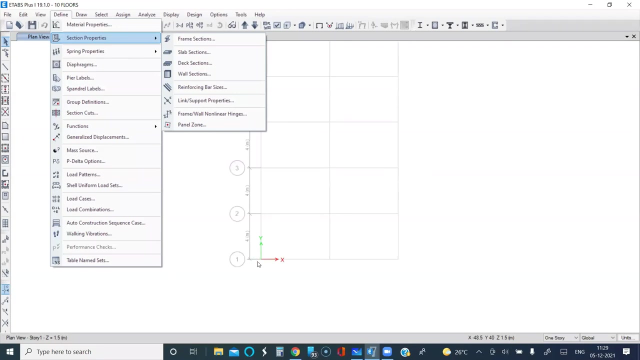 want, But I'm not doing it right now. Then define section properties. I'm going to decide some column sizes. I don't know what size will be needed right now. I can use my thumb rules and then decide the size, But then I don't have time to show you the thumb rules. So what I'm going? 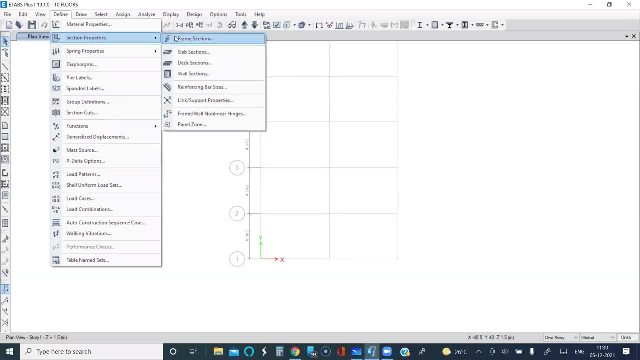 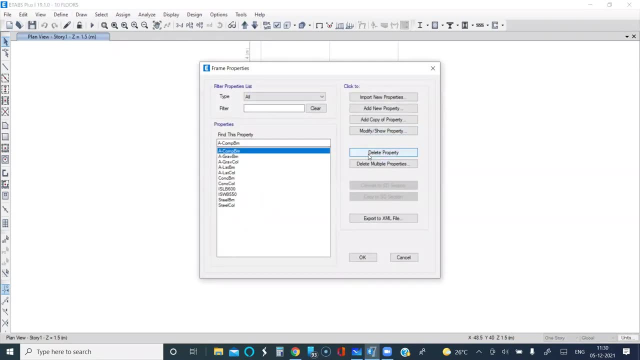 to do is a trial and error. Okay, So from section properties I'm going to create some column sizes, Frame section. Okay, There are certain things here. As a beginner, I encourage you to delete all these what are available here. Don't keep unnecessary things. 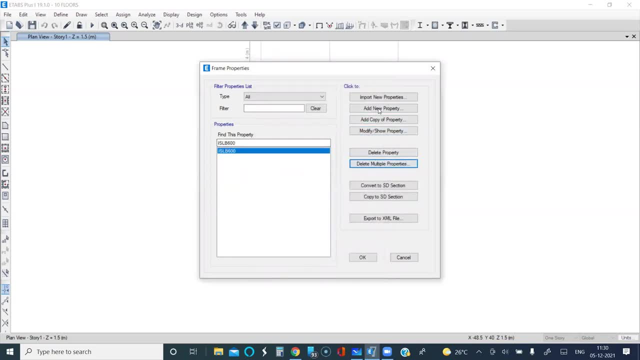 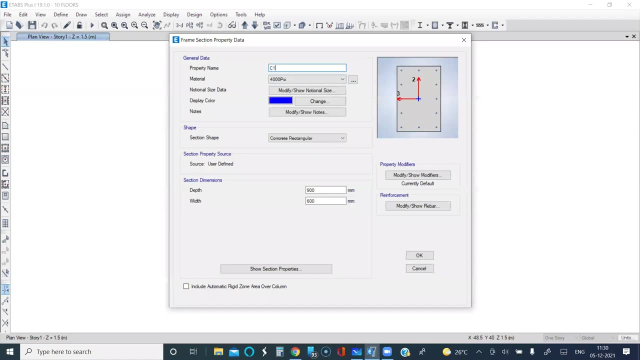 here. Delete everything. So add new property Rectangle. I will name it C1.. 300 by 600.. I don't know what will be needed. I'm going to do a trial and error right now. Here you have to change. 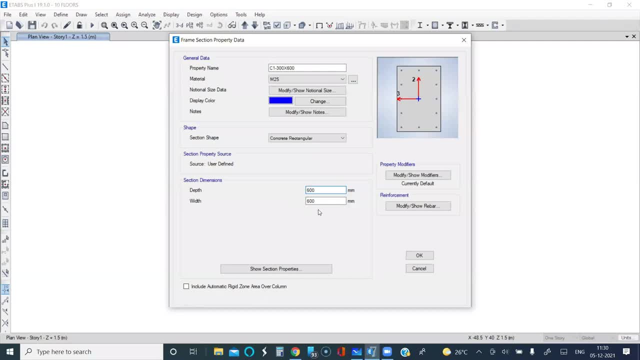 the size. Here you have to give your size 600 by 300.. Always give the first dimension as the larger and the second dimension as the smaller. There is a reason for that. Again, that's a very important reason. You should not give it as 300 by 600 by any reason. That will mess up. Never give. 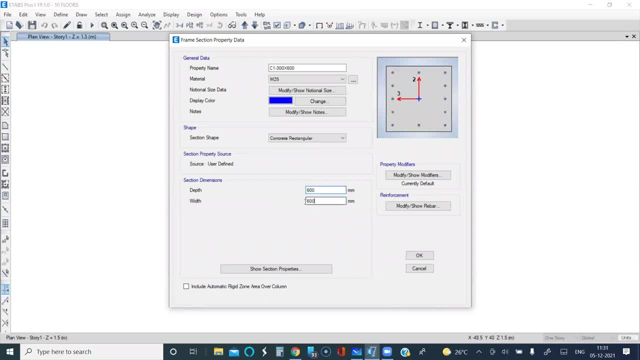 it like this Reason. I will tell you in some other time or I will create a blog for you, But right now, remember that The depth has to be the larger dimension, has to be the depth for columns and width as the smaller dimension. Always do this, Don't do anything else. Fine, Now leave this. This is: 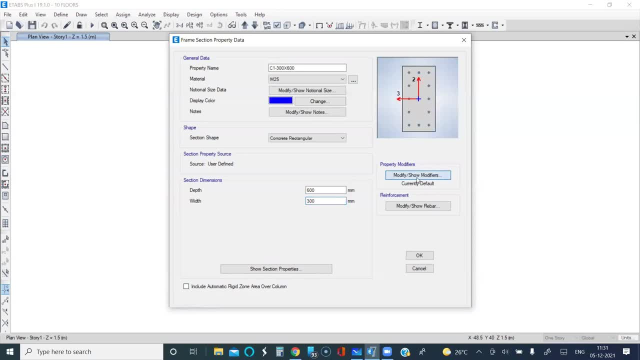 not needed: Leave this right now Not needed. Modify: Leave this right now, Not needed. There are uses of this. Distortional constant is very, very important. Then moment of inertia: this is very important. There is something called stiffness reduction, which is needed for tall. 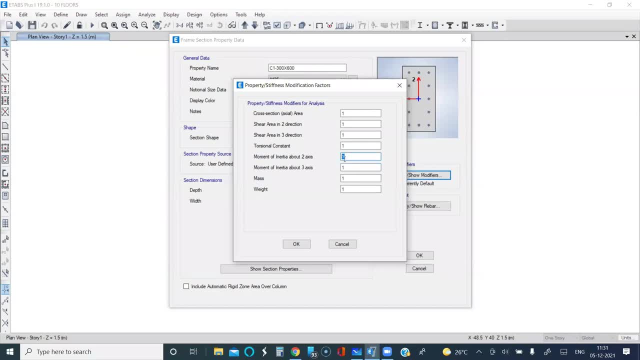 buildings. But for the time restriction I am unable to tell you this. Later we will see if we have time, I will come back in the end and talk about this. So for the time being, not everything is one Distortional constant. you need to modify Moment of inertia and a moment. 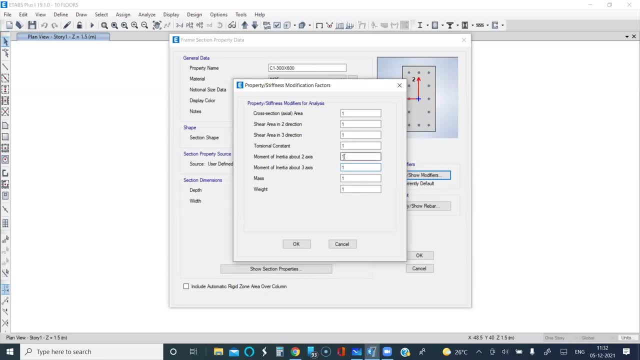 of inertia. you need to modify for larger buildings, Very larger buildings. it will help additional things, advanced things, But at this point in time one. So G plus 1, G plus 2, G plus 3, all this it's okay. to what do you call? It's okay to use one. So I am going with. 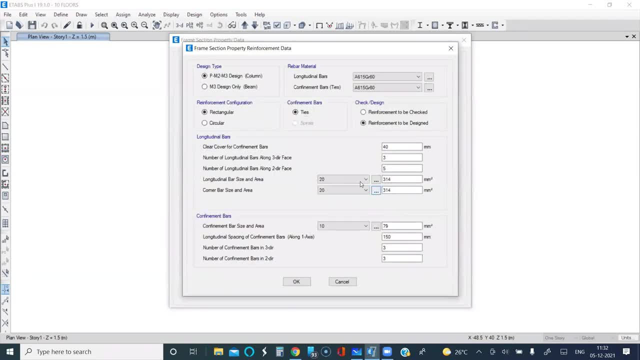 that Now here, modify, show rebar. Here you have to change your rebar grades. Yeah, You have to call it as a column. So it's a column, not beam. Yes, it's a column Now. reinforcement to be checked. reinforcement to be designed As a beginner: always go with. 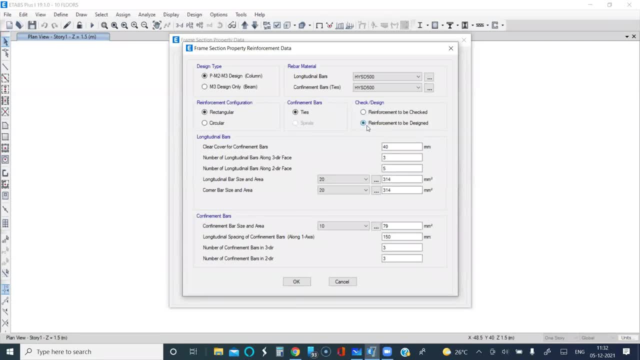 reinforcement to be designed, Leave other things. So when you are saying that reinforcement to be designed, you can ignore all this data. Don't bother. If you give this, you have to bother. You have to decide all this. Yeah, But you cannot check now because you have not even. 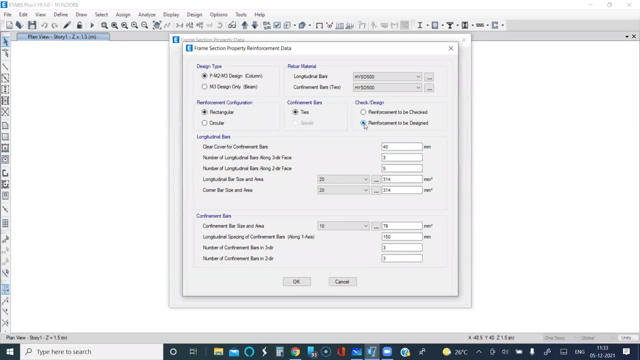 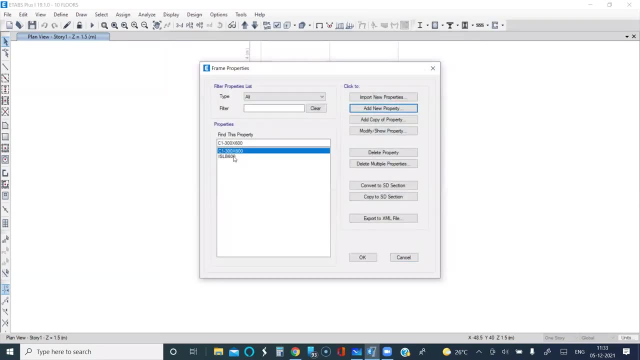 decided the size, So go with reinforcement to be designed here. Click on okay, Click on okay. So one column is done. Okay, Now beam you need to create. So I am going to say add copy of property. That will save a lot of time Instead of saying 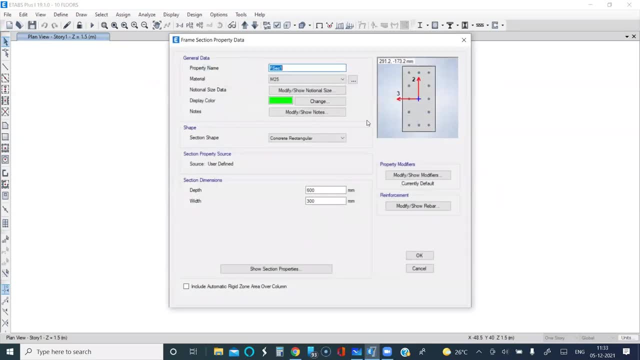 add new property. I am going to say add copy of property. So the copy of C1 is made. Now I am making it to B1. I will go with 230 by 500 size. So here this becomes 500 and this becomes. 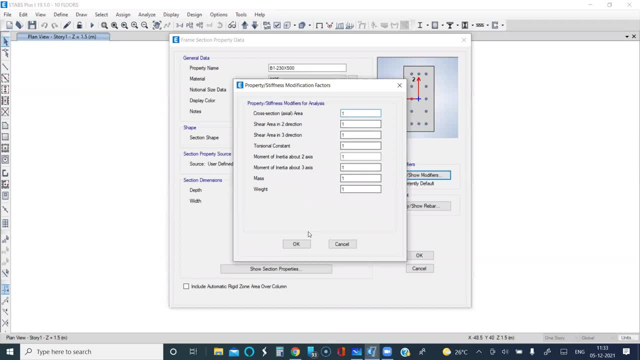 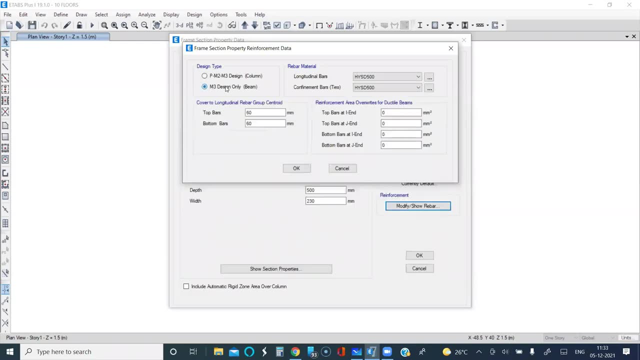 230.. Now, mind you, this is a column because I copied the property of a column, So you have to go here and then change this to beam. But my work reduced a lot I had, I need not change all this. 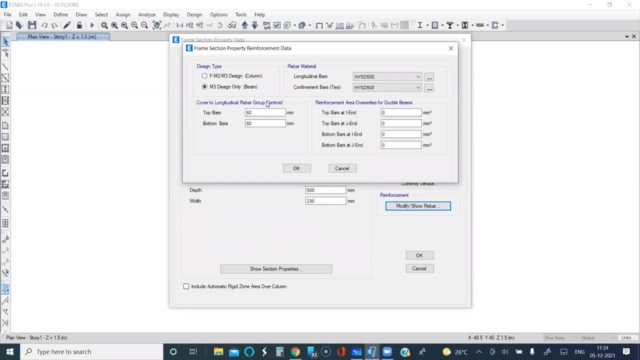 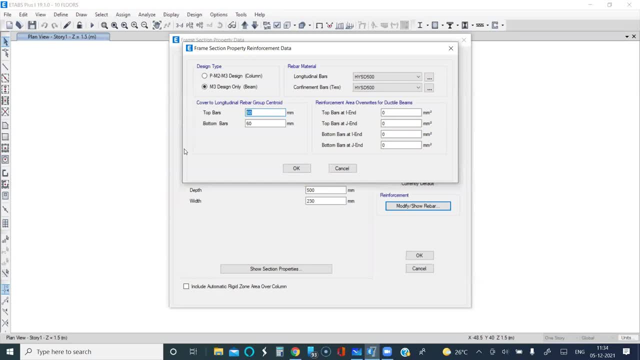 of the rebars. So the clear cover is 25.. If you work out it may come to 50 or more or sometimes less. It all depends on the diameter of the rebar that you are going to use. But at this point of 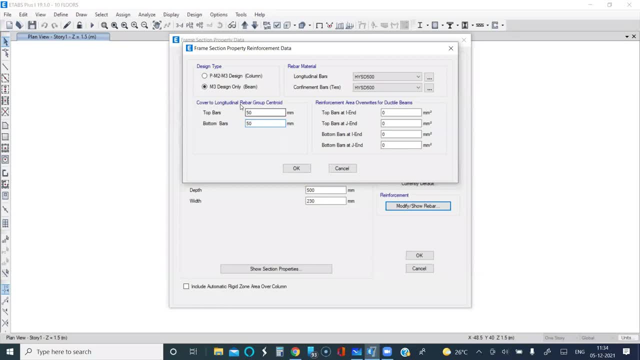 time you don't know what rebar you are using. So I am giving this approximately. Later you may have to fine tune this, But at this point in time I am just using 25 as the clear cover. Then you have stirrups, Then you 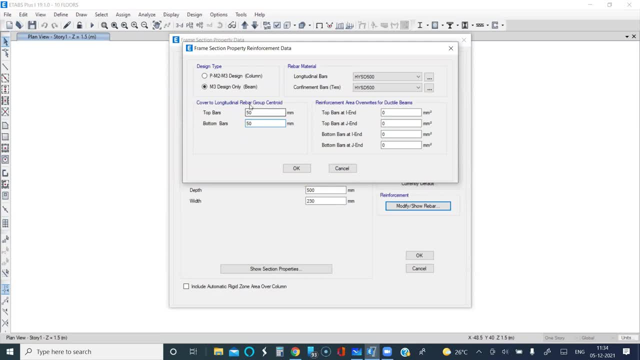 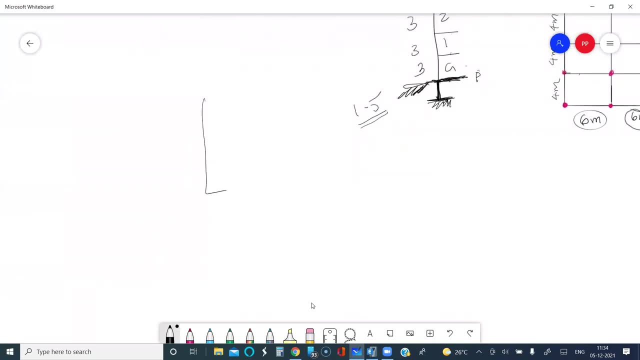 have one or two layers of rebar in your beam, So I am giving this, Yeah. What I mean is, if this is the beam cross section, this is your total depth. You will also have stirrups here, Yeah. So your effective depth at the midsection is something like this And your effective cover. 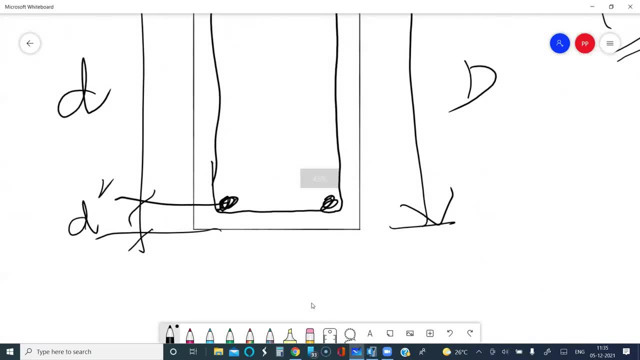 is this to the center of the rebar. Yeah, You may have one more layer, in which case you have to find the group centroid of this and it will be somewhere here. So that distance day dash is what I am giving as 50 here. I don't know how much it will be, It will be 25.. Clear cover will 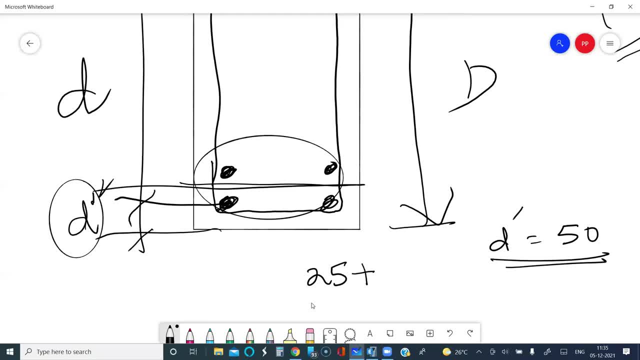 be 25 for beams Some distance. So without deciding the diameter of the rebar we will not be able to finalize it. But I am taking it as 20 plus something like that. Yeah, So 25 plus 20 plus 10 becomes 55.. 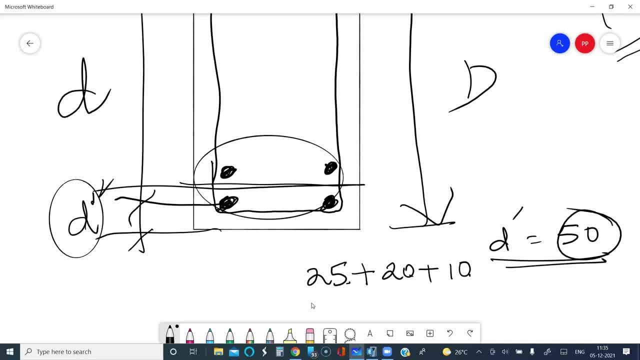 Yeah, Or maybe this may be second layer, maybe 16 diameter, So this may be 8.. Yeah, So that way I am deciding it to be something like 48 to 50, something like that. Yeah, So that's the reason. 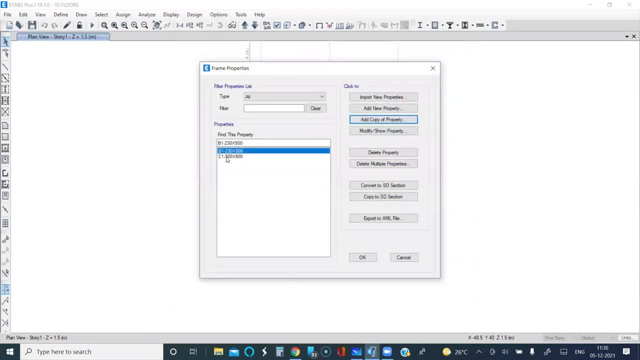 I am giving here. Now one beam and one column is defined. That's enough. We will see it later if we have time. Yeah, So now I have to model this. How do I model? Very simple, in ETAPS. I am going to come to. 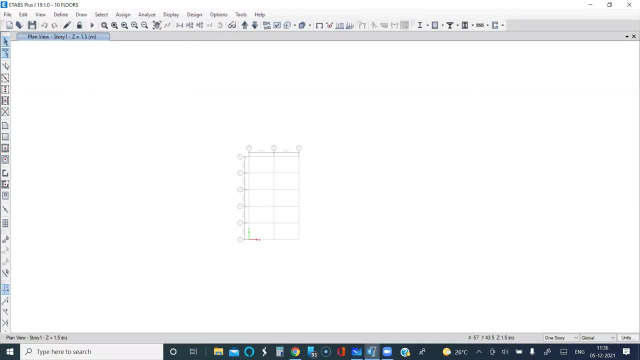 draw command. You have all the tools here also, But as a beginner you can always go along this line. Yeah, So you have defined. Now you are going to draw Now here, if you go, you will get commands for drawing. So here you can either pick one level and row column one by one. 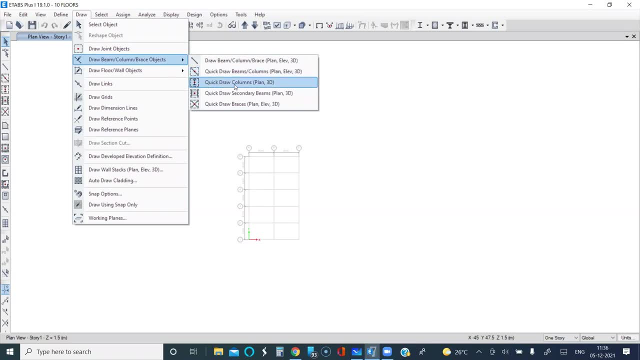 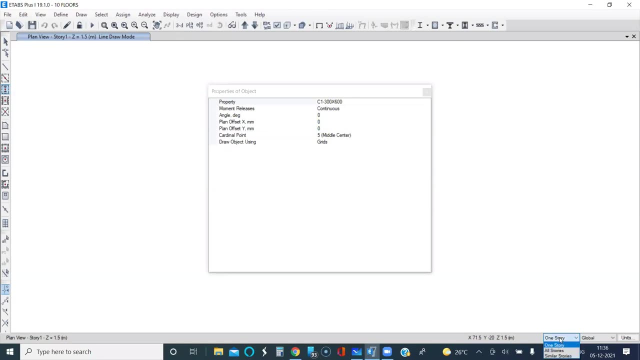 or I can use Qt draw column option. So I am going to pick that Qt draw columns Now here at the bottom. you can see here there are one story, all story, similar stories option. Yeah, But I am going. 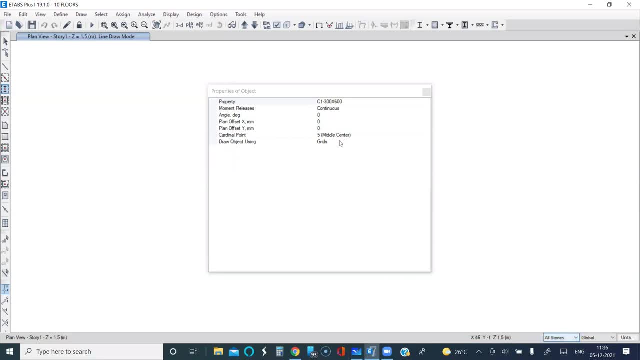 to take all stories here now, because it's all typical C1. If you want to change, you can change, But then C1 is what we want here And it's continuous. You can go with the default option: All stories. You can see the beauty In one shot you can place. 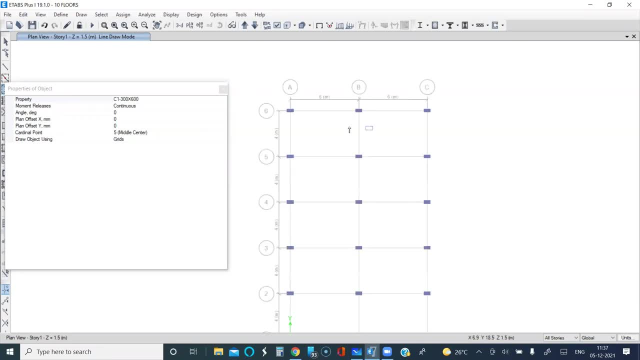 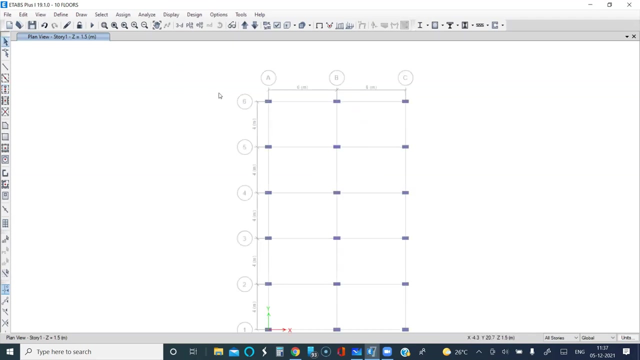 all your columns. This is when you have grids. When you have grids, all your columns are placed in one shot. Okay, Now orientation of the columns. How do you decide? There are two aspects to it. One is related to your gravity: loads So larger. 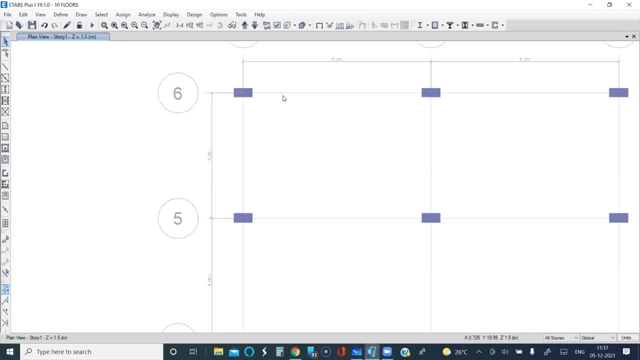 span Here. four is less, Six is more. Yeah, So you are orienting it towards the larger span, because your moments or the deflection of the longer beam will be larger. So you are orienting it towards that. Now, the seismic point of view, it may be different. 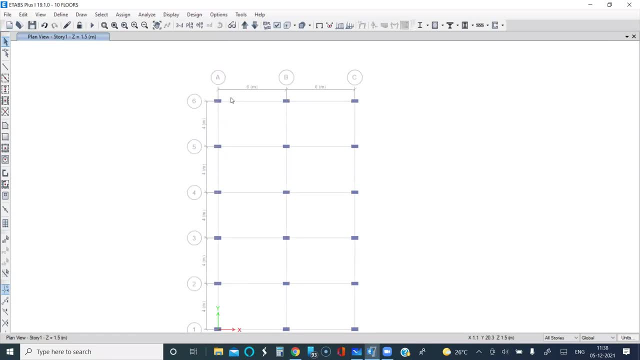 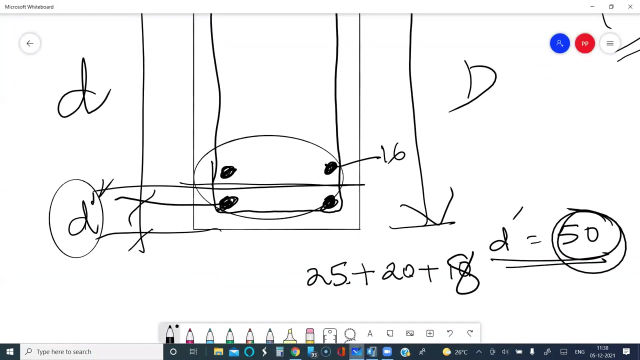 But then I cannot explain it. I will take one hour to explain that. Yeah, So we will do it on another webinar, But please note that our idea is to ensure major axis of your column. Major axis means this moment, That is, if I draw that. our idea should be that. 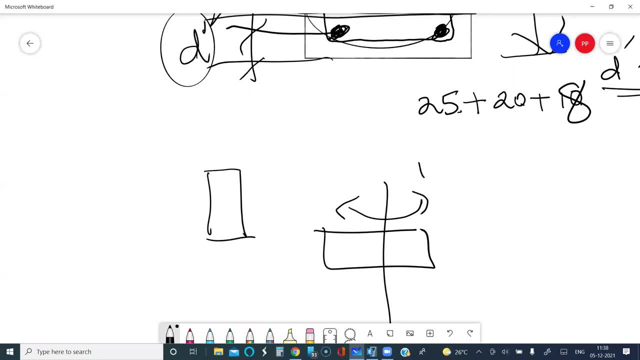 if this is the column, this moment, mx or m3 in etabs, this should be more than the minor moment. Major axis moment should be more in the critical design. Then your steel will be lesser. That is the basic principle. Yeah, How you do it, why you do it, I can't. 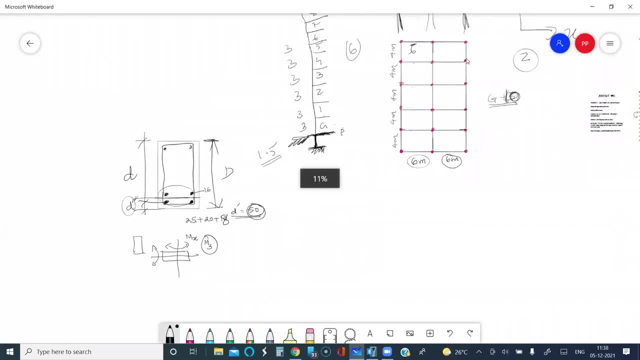 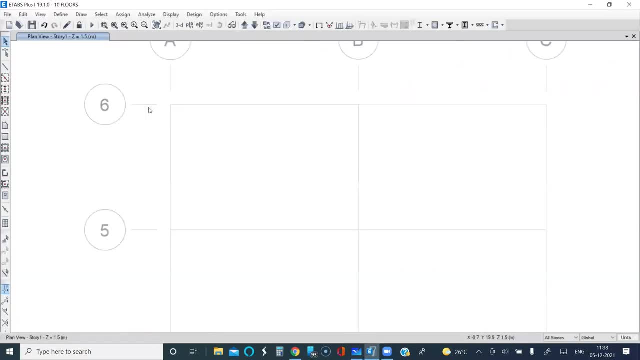 tell you completely now, because it takes time. Yeah, So please note that You have to orient your column And it can be a trial and error basis. It cannot be in one shot, especially when your buildings are in one shot. In this case, I can maybe close my eyes and say that this is the correct orientation. 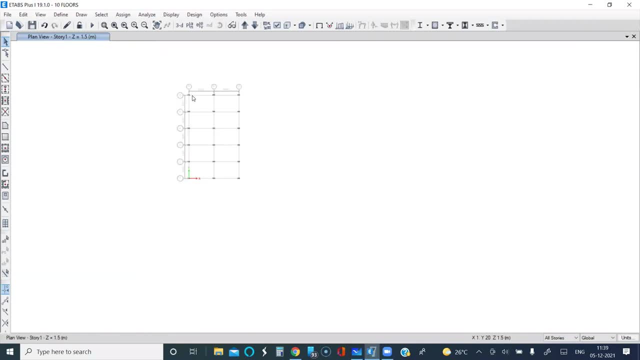 But when it becomes more and more complicated, when the shape are different, I may not be able to decide that just in one look. Yeah, It may have to go through some iterations to decide that. Okay, So here, the width of your building is less length of your building. 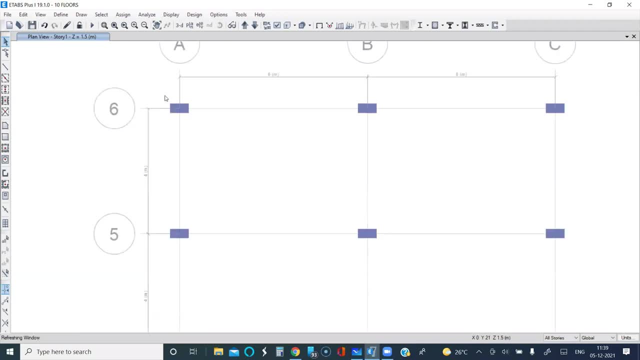 is more So. seismic point of view also, I find this orientation more suitable, So I can say that the width of my building is less length of my building is more suitable Because if you remember, or if you imagine a stool or a table, and if you imagine that, 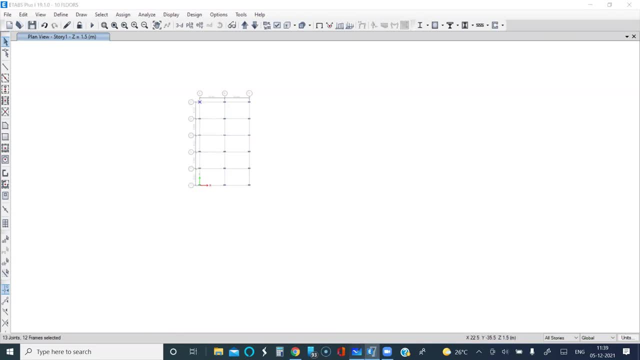 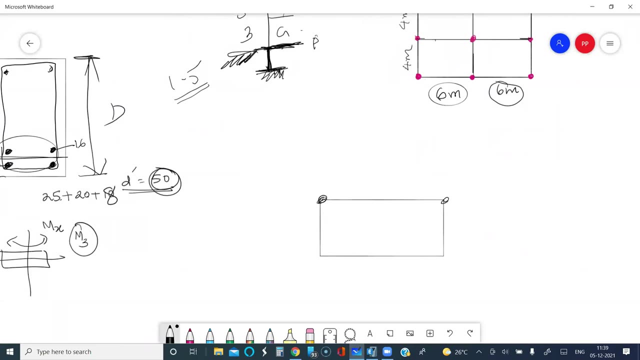 you are pushing it and trying to overturn that. you can very well think and understand that If you have a table like this with four legs- this is the plan And if I draw, it is easier for you to push in the width direction and overturn that Because it's less stable. 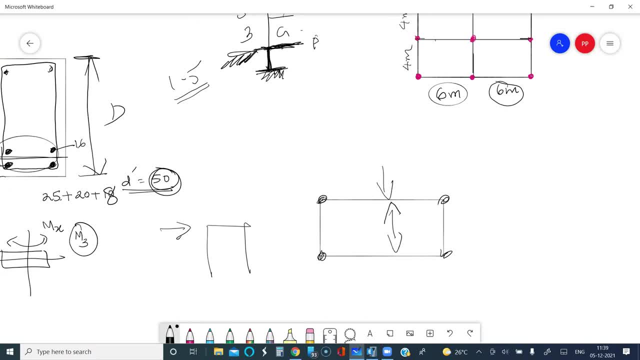 in this Because it's width is less, Which means that a building which is slender along the slender direction it will experience more instability. Yeah, So it is better to orient your columns in the slender direction, because that will give it more stability. Otherwise it might. 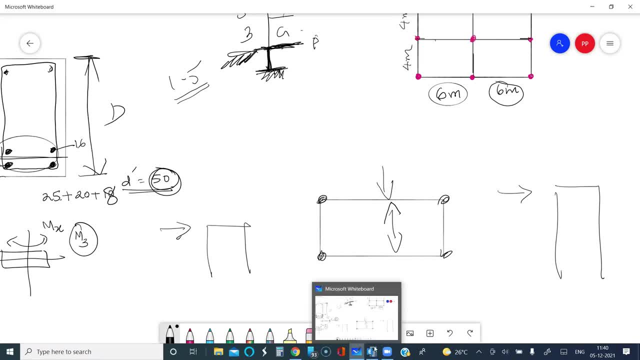 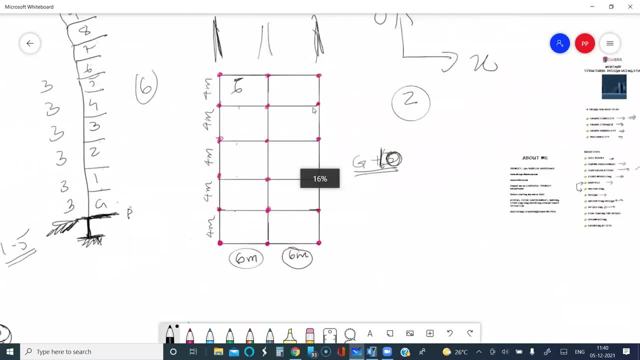 overturn. I had explained this in the free course. Those who might have done the free course would be knowing that If you have not done it, hop there and do it after the webinar or sometime when you are finding time. So that's the funda. There are more things there, but I cannot explain. 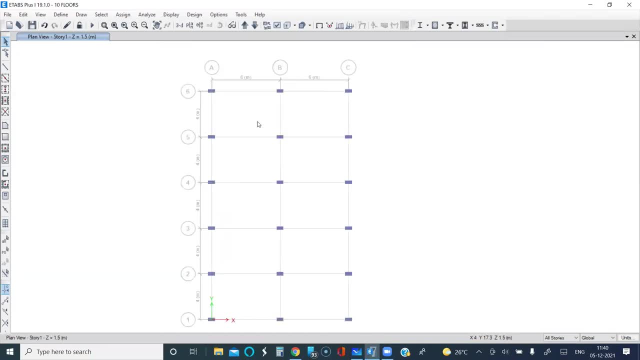 everything in a very short webinar. I will need hours to explain that. So now done. Fine, Now I need beams in all the levels. Now you can quickly see the 3D view. Columns are there in all the levels. I will come back to plan. I can go to any. 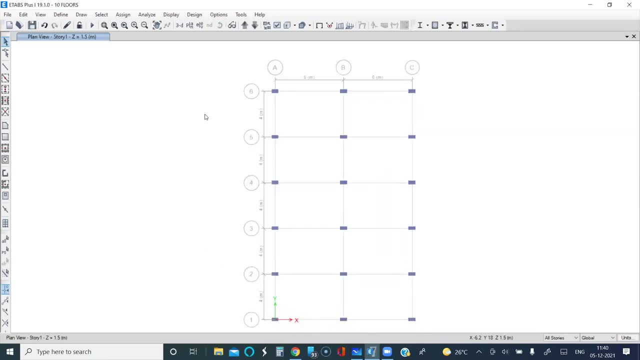 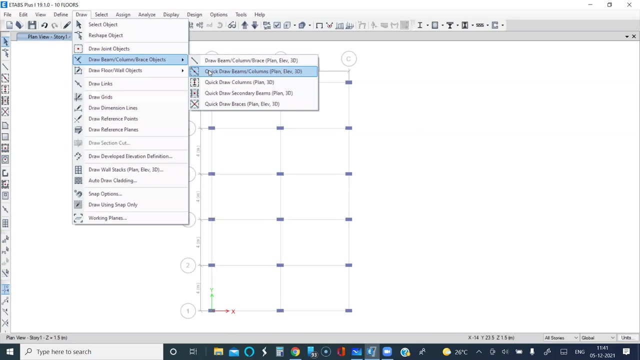 of the plan. So I am going to go to plinth level- Fine, And then I am going to model the beams. To model the beams, it's again easy. I can go to draw and then draw. Quick draw beams option I can take Now. this will work when you have grids, If you don't have. 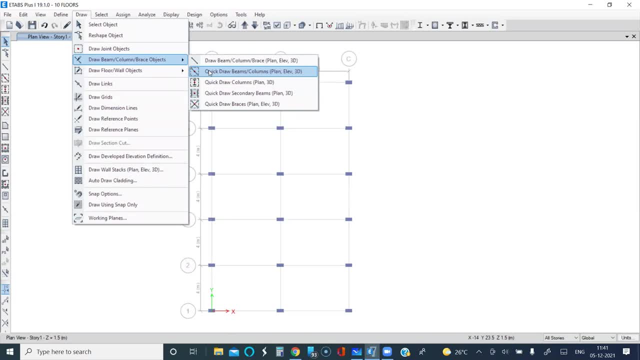 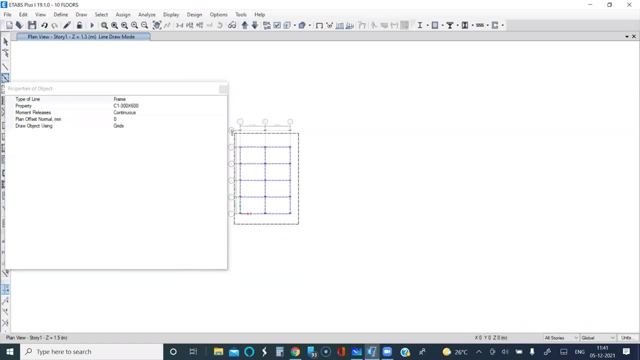 grids. quick draw beam will not work. You will have to draw one by one. But I am going to show you the easiest way now. So I am going to take quick draw beams Again. you can select like this: In one shot. your beams are done Now. your panels are 4 m x 6 m, So do you need a secondary? 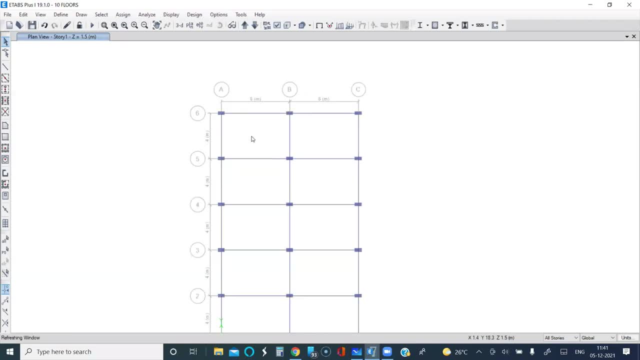 beam? Not really. How do you decide if it is needed or not? Do you need a beam like this, Like this in this direction? How do you decide that? Again, in the free course, I have explained it in the, I think in the. 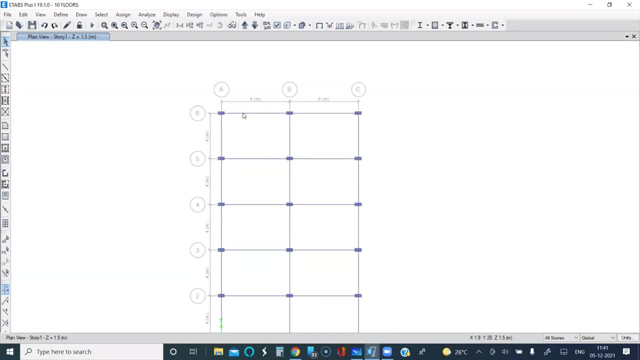 In the free course. In the free course, the slab thickness- i don't remember. if it's in the free course, it's based on the slab thickness. there are three things, three points that will decide if you need more beams. one main aspect is your slab thickness. second aspect is your wall positions. if your walls are coming on top of your 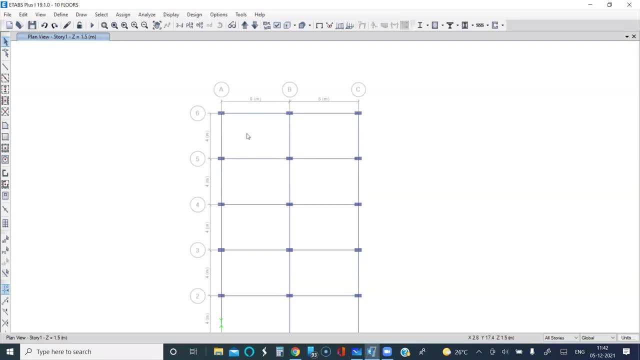 slab. it is ideal to give a beam, okay. and third reason is to tie the column. there are three reasons that you need beams. one is to split your slabs into manageable thickness. you cannot have 200 thickness for a residential building. yeah, so that is one of the main reason. 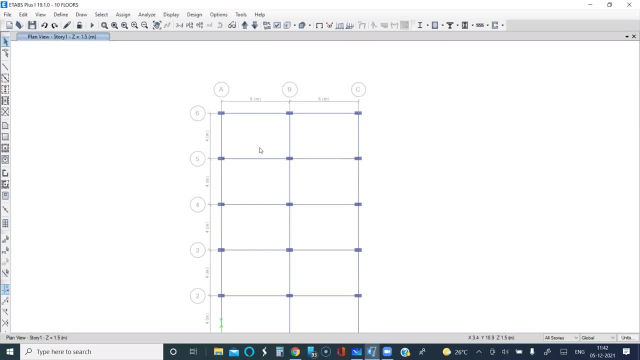 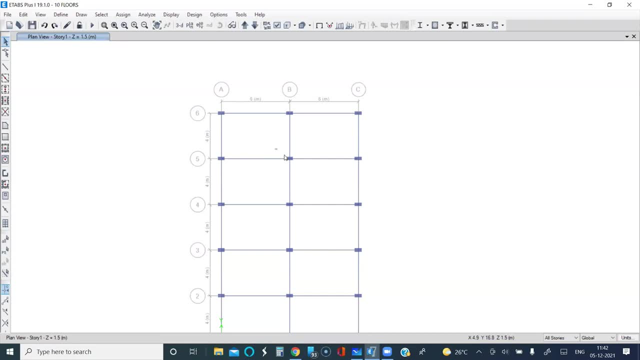 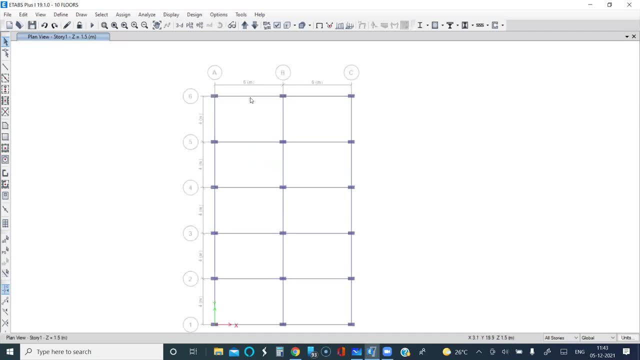 to explain you everything. so here i'm not giving any secondary beam, because four meter is not so huge. how to decide the thickness? l by d ratio. mostly slabs will be guided or decided by l by d ratio. so i don't foresee anything more than 125 millimeter for this continuous slab you will be. 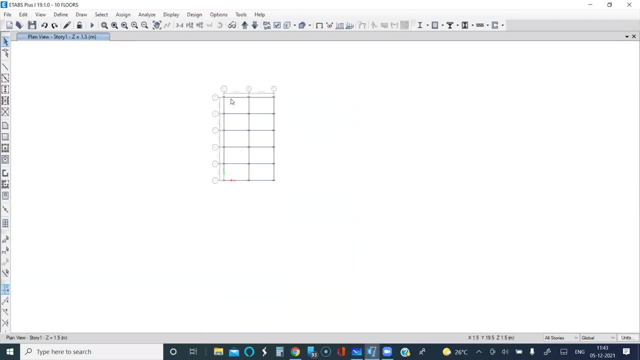 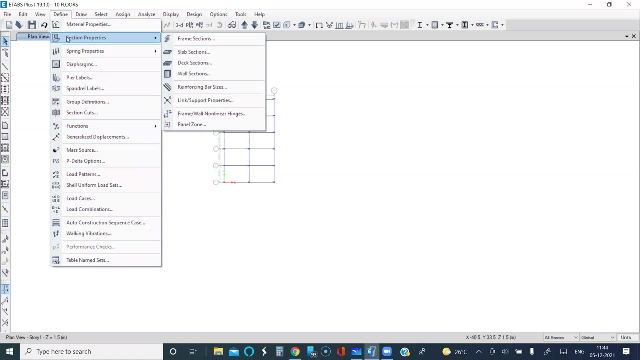 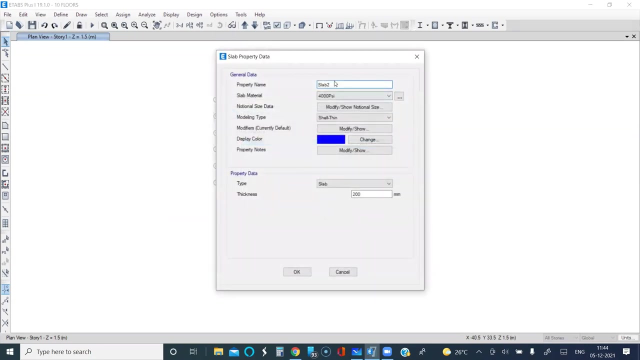 able to manage with 125 or maximum 150. 150 won't be needed, 120 to 125 you can manage, so i am not going to give a secondary beam in this case. okay, so i'm going to define. i have not defined a slab, so slab section. i'm deleting this. add new property. i will call it yes, one, i will need only 120. i'm. 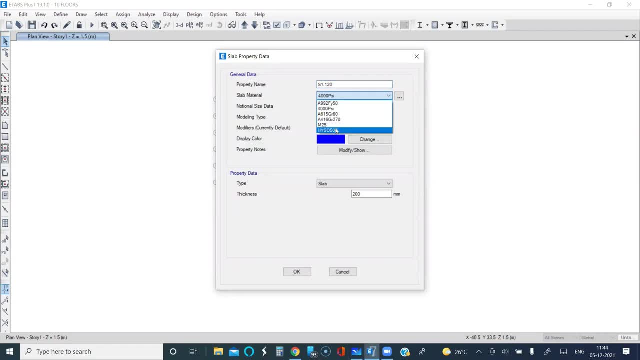 almost sure about that and grade i'm going to give m25. m20 should be sufficient. and here there are various options: membrane shell thin, shell thick. i think in one of the group i have uh explained what is the difference between membrane thin and shell thick. if you want to know about it, please post in. 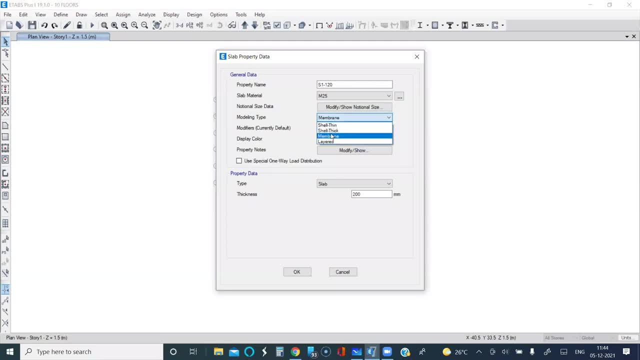 the group. i will repost that video. it will clarify why i am choosing membrane, why i'm choosing shell thin. when i have to choose that, yeah, shell thin would be ideal, but for simpler, smaller, regular buildings membrane is also fine. so i'm choosing membrane right now. membrane will 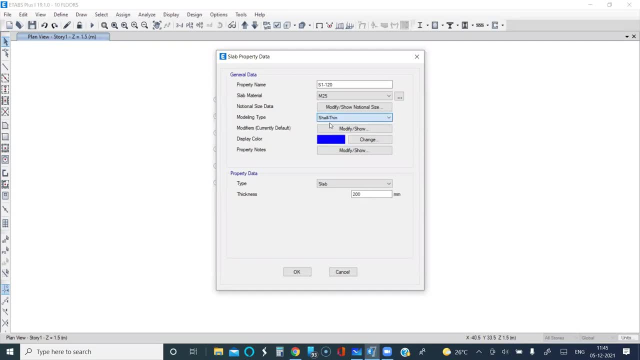 replicate e-line theory behavior. shell thin will be an fem where the slab stiffness is going to come into picture and it will account or it will act with its stiffness in the model. i am not going to say membrane, but this is a very important topic. you need to know, uh advanced things about this. 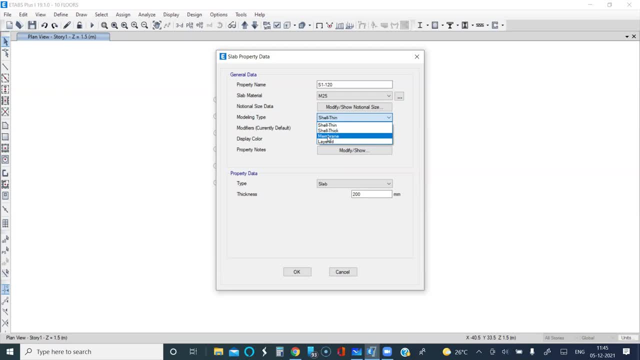 to be taking decisions on this. okay, so currently membrane, but please remember shell thin you may have to use at many occasions. shell thick: rarely for uh slabs, but for rafts you may have to use where shear deformations are critical. so here i'm going to say membrane thickness: 120, type slab. 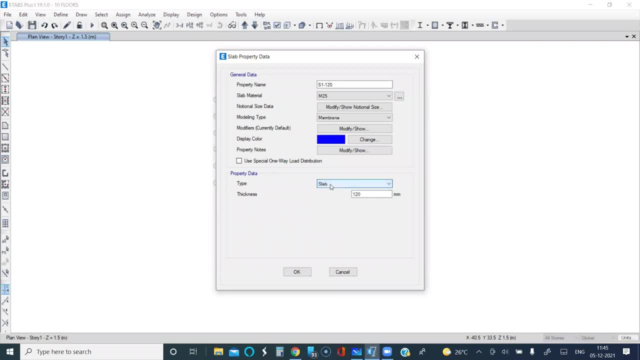 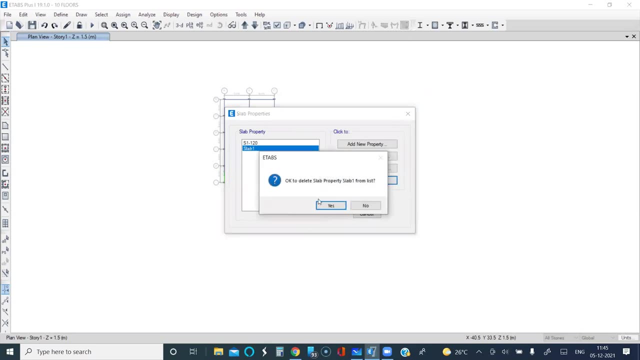 drop panel. there are so many options. but for a normal beam and slab system, choose this as slab. okay, yeah, so this slab i'm deleting. i don't want to keep anything which i don't use. so s1 120, fine, so that's done. now, again, this is all flows. i can go with three options: one, two and three. either i can. 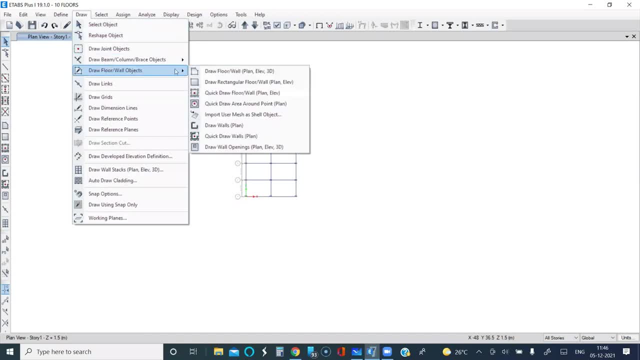 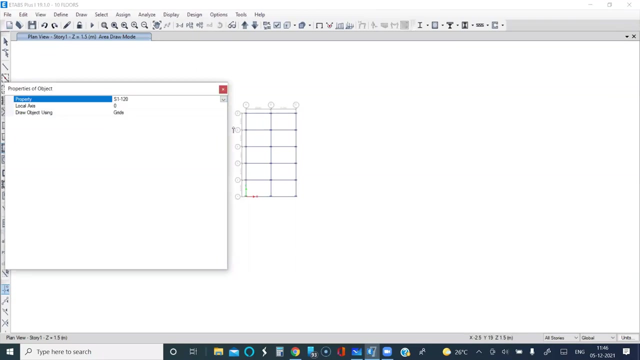 pick from here or go to draw and then say there are various options. i'm going to say quick draw option in this case. yeah, so that will i have to choose which one i want. so i'm going to choose s1. see, in one shot it will come. you also may have to draw it sometimes if you don't have grids. but 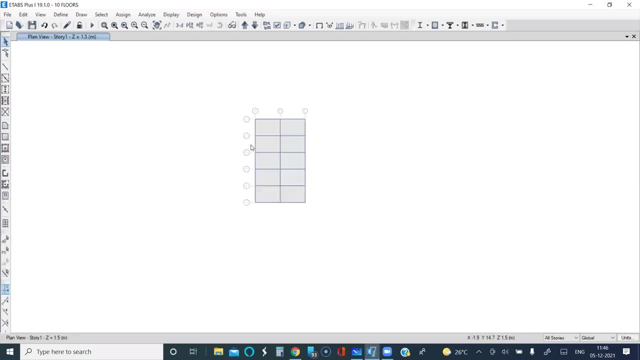 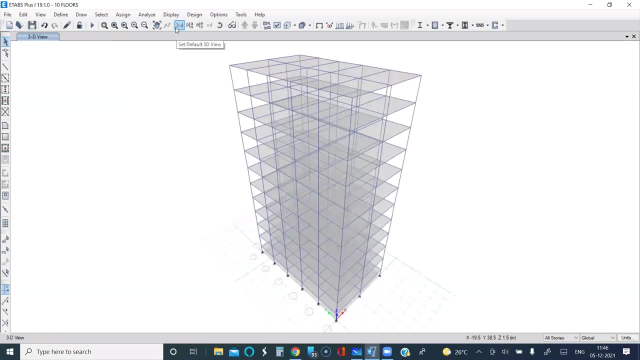 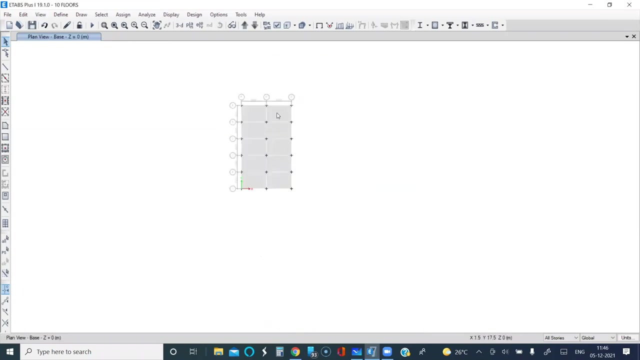 if you have grids, you can choose it like this. it's as simple as that. if you know stat, you can now see how easy it is. yeah, so now 3d. you have slabs, beams and columns everywhere. now let me show you one thing. at the base level, i have unnecessarily given slab which is not needed. 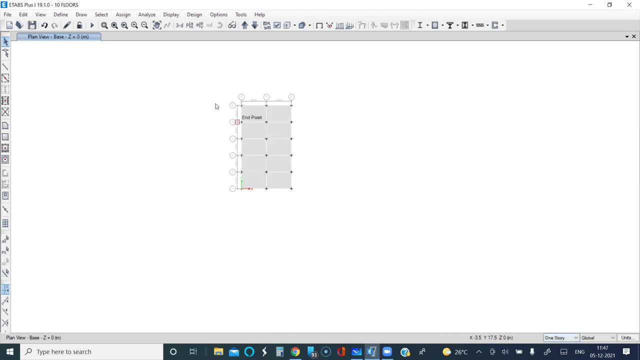 so i'm going to make it one story and select this and delete. if i keep all stories, it will go in all flows. now, in plinth level, do you need, uh, do you need slab at the plinth level? so actually you have put column instead of beams. do check out. okay, i can check it out. 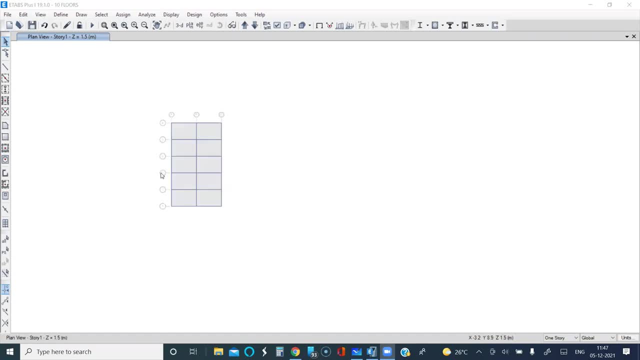 uh, yeah. so do you need, uh, slabs at plinth level, yes or no? you can type yes if you think slab is needed at the plinth level. you can type no if you think slab is not needed. no, okay, so it's a not a blanket. no, sometimes you may need. it depends on if you need a grade slab or not. 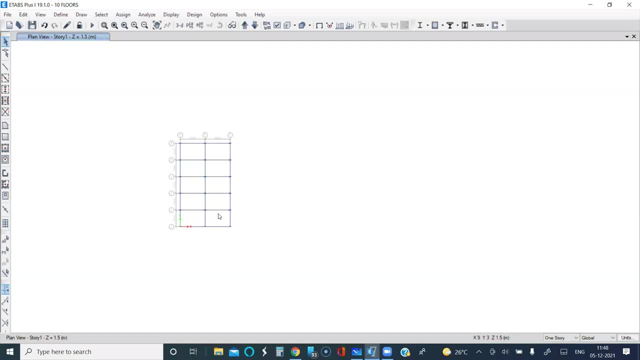 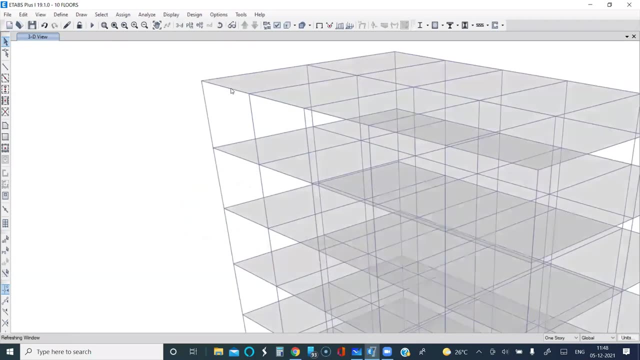 and it also depends on if you have water table in your project. so anyway, in this case, i am deleting that because i don't need it now. somebody had commented that, instead of being, i had modeled a column. yes, he is right. so you can see that instead of beam, i have taken column here now. 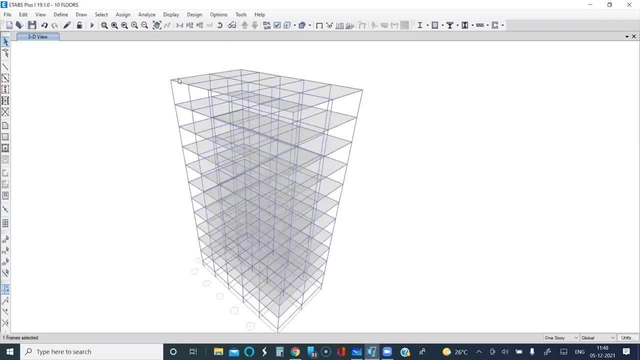 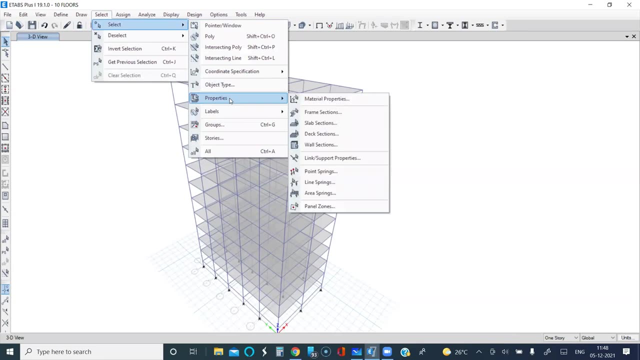 this is another beauty of e-tabs: it doesn't take column. ah, yes, Sasan, pleaseama can do that also. it doesn't take much time for changing this. you can change in one shot. so select, select properties or object type. yeah, you can choose in one shot. you can see that all the beams are. 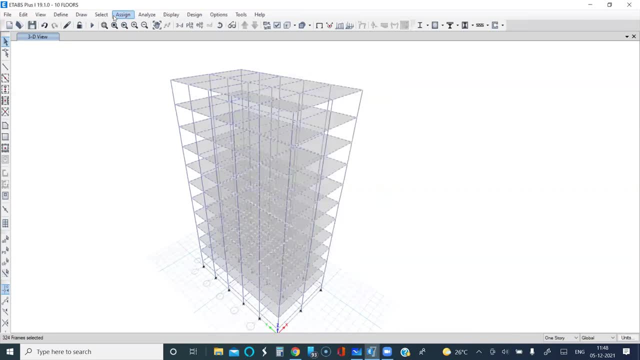 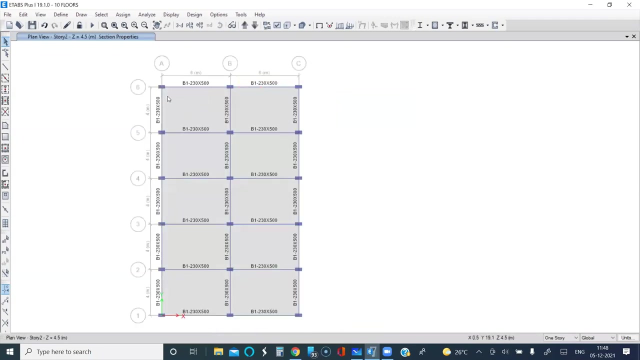 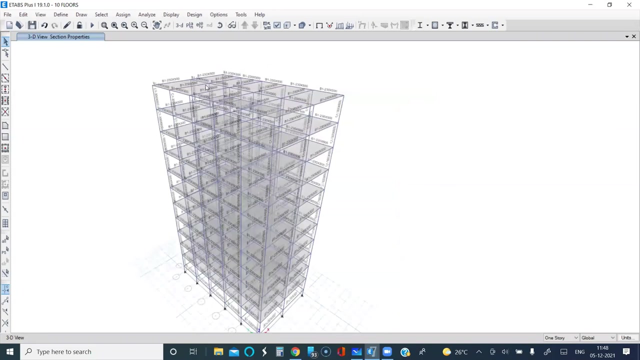 selected and i can change the assignment from what i have done, from c1 to b1- in one shot. yeah, so now you can see all are b1 and all are b1 and you can see the columns are c1. yeah, so in one shot you can change if you have made any. 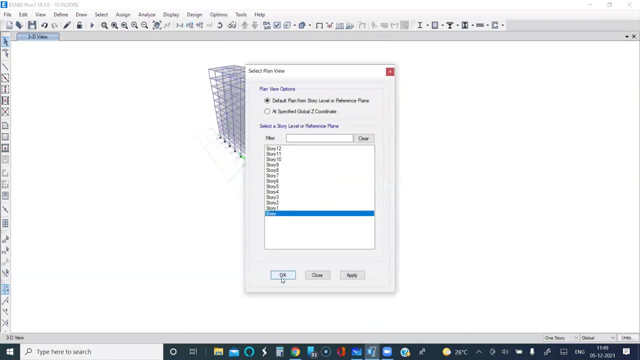 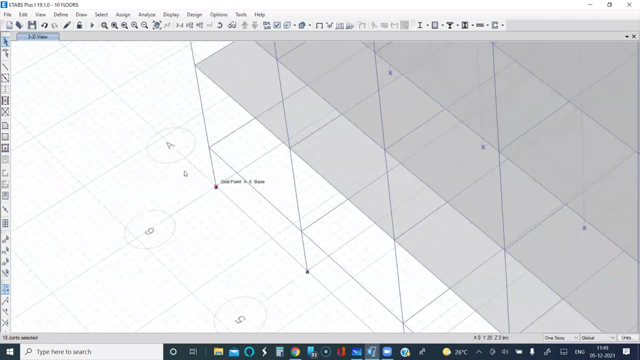 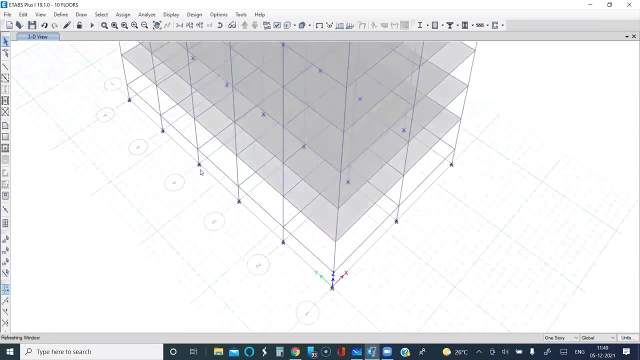 mistake, or if you want to change something after your first trial. now, if you go to your base, i have automatically pinned the base. yeah, so now there are school two schools of thoughts. some believe it is fixed, some believes it is pinned, some believes it's neither fixed or pinned. now who believes this is fixed? 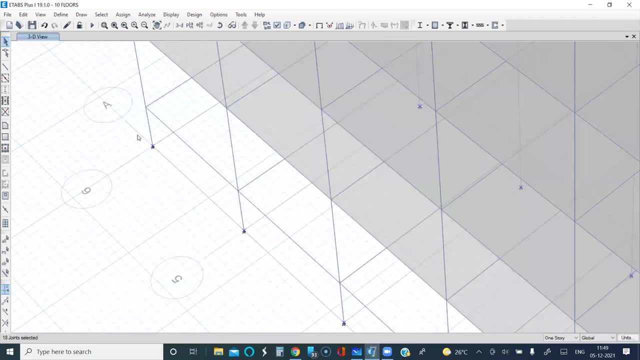 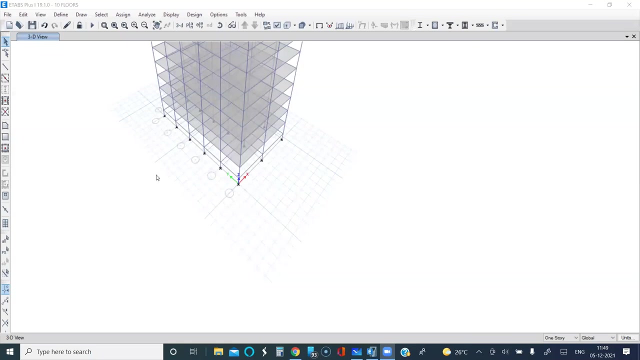 please type f. those who believes it is pinned please type p. and who believes neither of this type n. okay, most of the people are thinking it is fixed. some are thinking pinned now. in reality, it is neither fixed nor pinned. now. i have a simple question to ask you here, that is, you might have learned about fixed beam, yeah, but have you fixed? 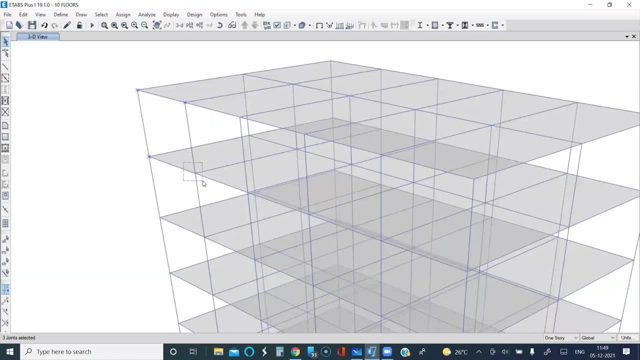 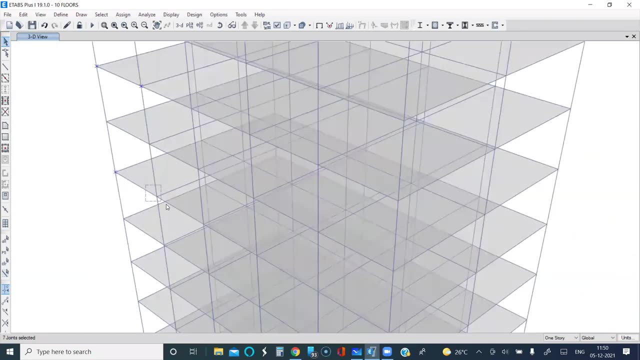 here. you have not fixed here. have you fixed here? have you fixed here? have you fixed here? why are you not fixing here? i had asked you in the group. i think in one of the group there are 10, 20 groups for me, so i don't know in which groups i have discussed this. but then just think. 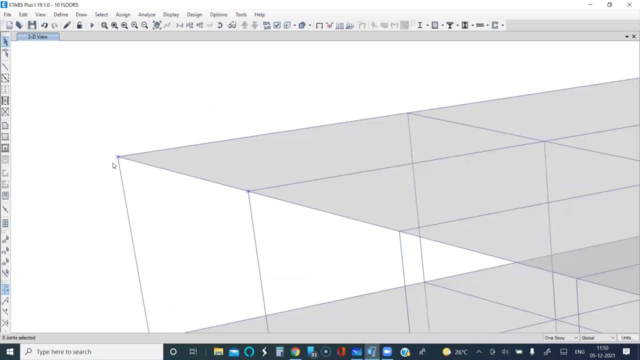 why are we not fixing or pinning here? because we want the beam and the column to interact. if you have done canny's method, moment distribution method, etc. you know that stiffness plays a role and, based on the size of the column and based on the size of the beam, this joint stiffness will. 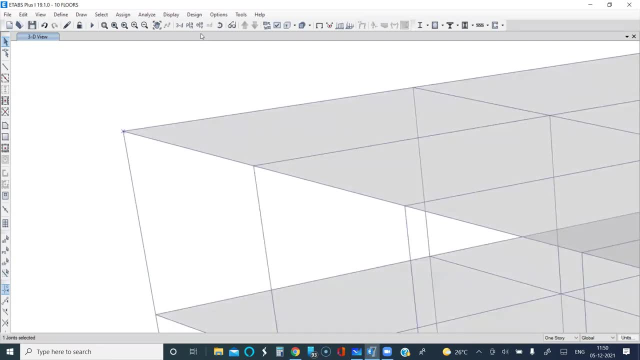 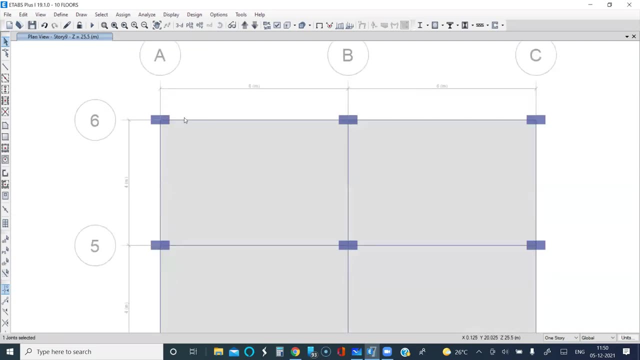 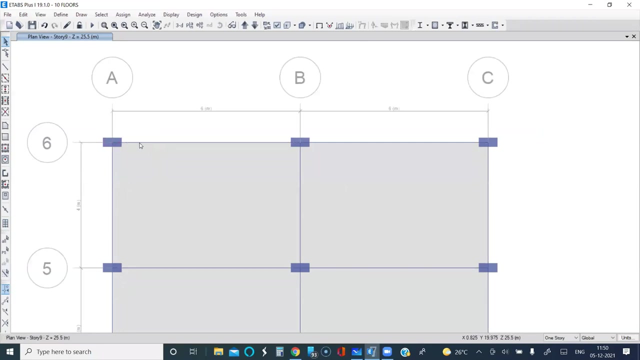 vary and the fixity also will vary. now, if you want to understand this, if you don't know about this, i don't have time to explain. but if you don't know about this, what you do is model a simple frame, only this much, or maybe. okay, if i show you that i will take time, so i'll come back. 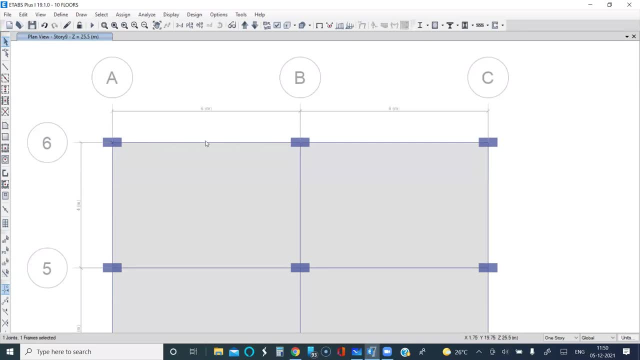 and show you if i have time. okay, so wait till the end. i'm going to show this if we have time. those who have time can wait. so here you do this simple exercise. in one building, you keep the column like this. in another building, you rotate this column in 90 degree and then check. 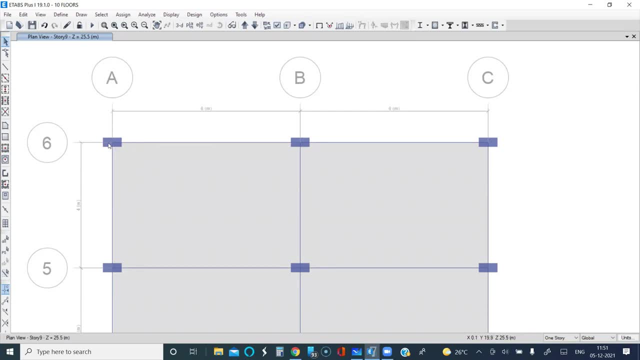 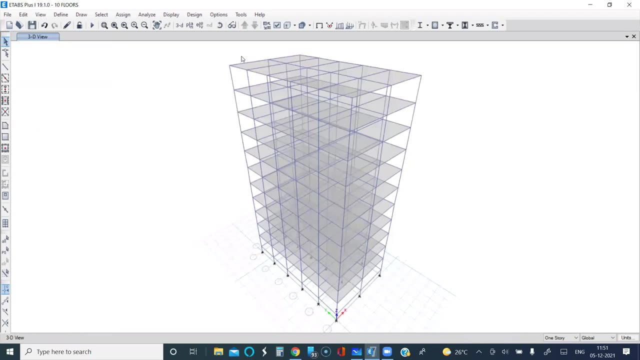 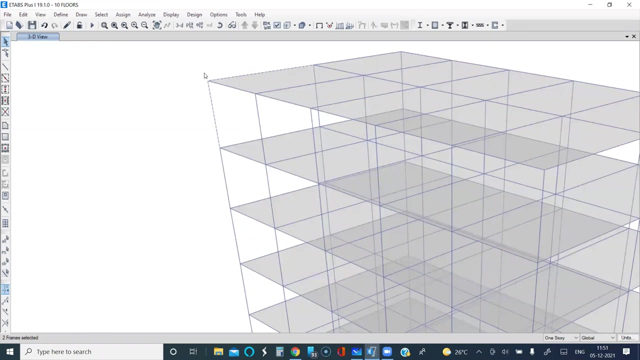 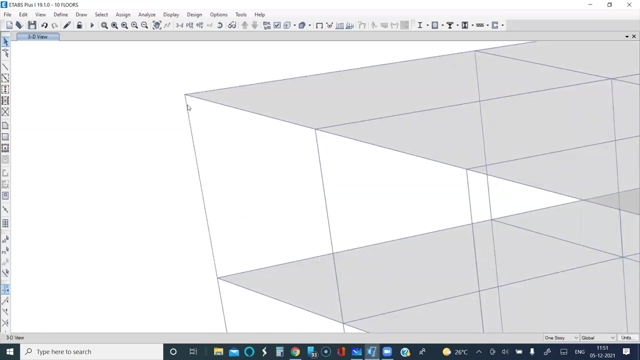 your moments, your beam moments, will be different. yeah, that's because of the fixity difference or because of the stiffness difference here. okay, so your column and beam. even though you learn about fixed beams, there is no fixed beam in reality. everything is relatively fixed, means one beam connected to 200 by 200 column is fixed, but another beam- same beam- connected. 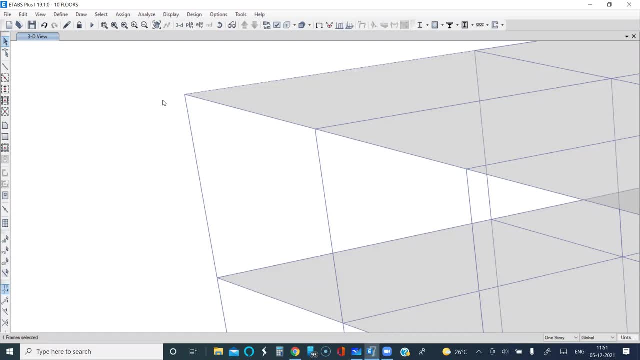 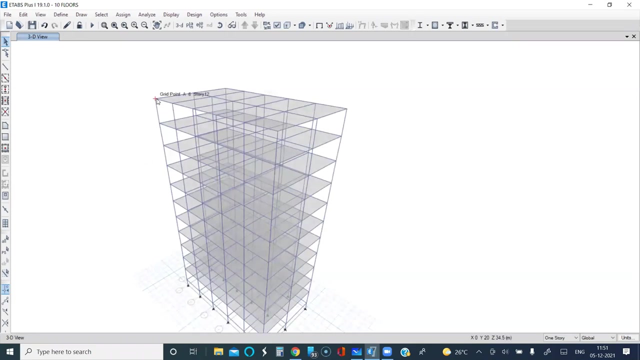 to 200 by 900. column is more fixed, so it's not fixed, it is partially fixed or stiffness decides the fixity. okay, and that's the reason, or that is what is all important in your structure and that's the reason we are doing a finite element or a software analysis. if 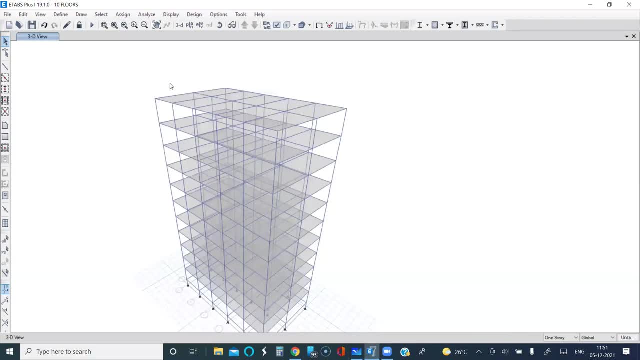 we were fixing or pinning all the column beam junctions. then we don't have to use a software. you can do everything by hand. it's as simple as that. but then your economy will go for a toss, your reality will go for a toss. there are various other disadvantages. yeah, so you have to employ a finite element: analysis. 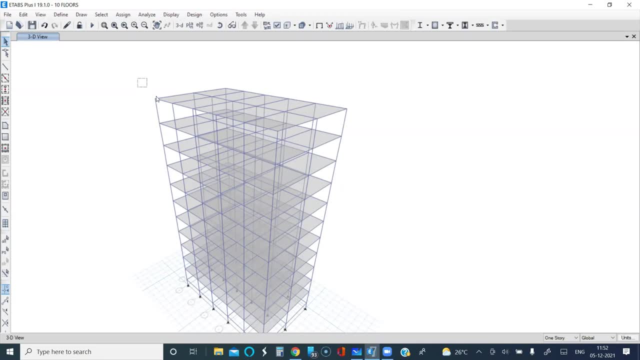 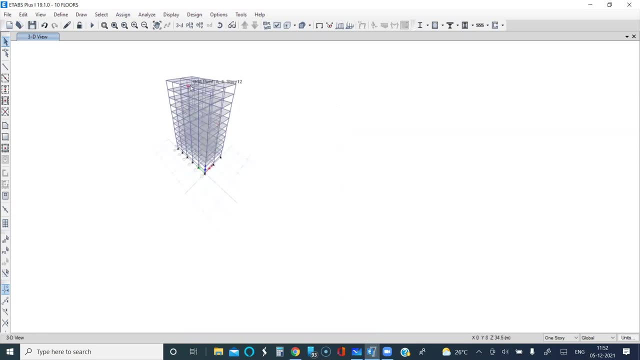 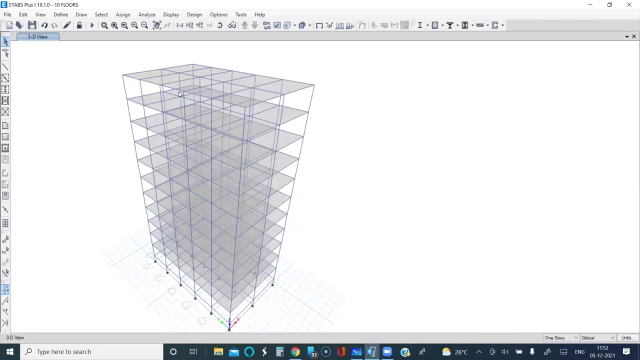 yeah, you have to use your seismic analysis. won't be right if you pin or fix all of your column beam joints. yeah, it has to be like a vertical cantilever. your building is a vertical cantilever for seismic. uh, when the seismic or when the ground moves, yeah, so you have to have that effect. 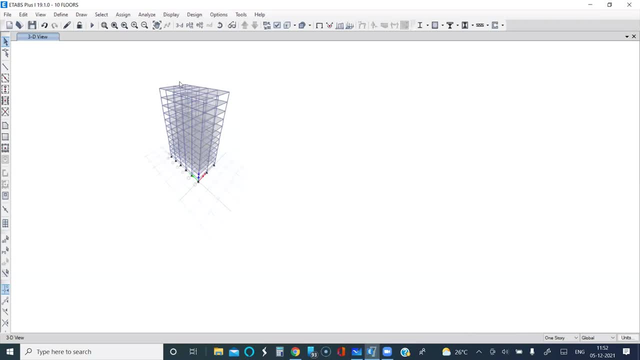 that's possible only if it is modeled correctly, as it is not by pinning or fixing. same way, i'm asking you, column: foundation joint is also a concrete to concrete joint. so why do we pin or why do we fix? why don't we model a foundation at the base? if it's a raft, model a raft if it's an 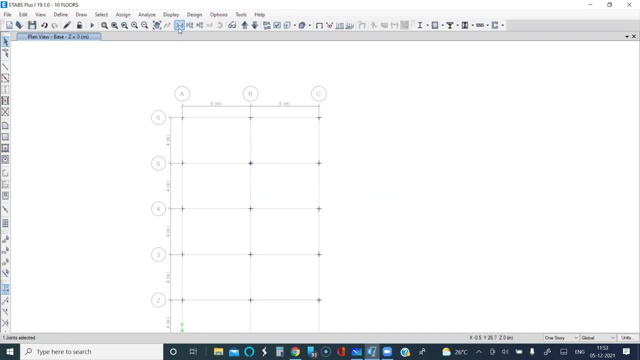 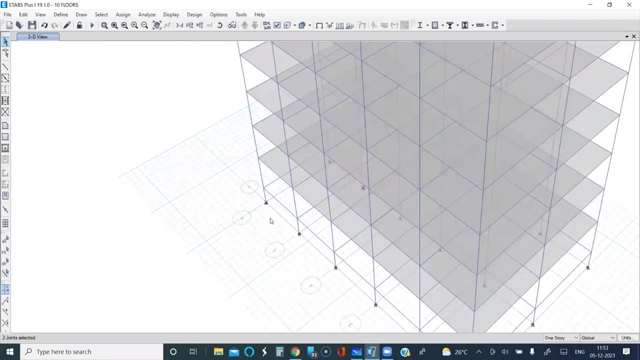 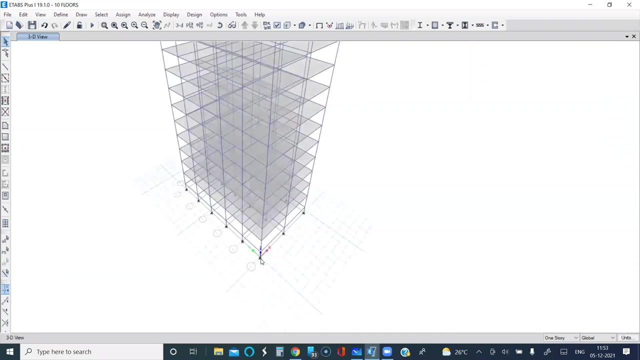 isolated footing, model it. why are we fixing? why are we pinning? is this right? why don't we use something else? or we model a foundation there. we can do it, but the problem is that you need to bring in the effects of soil also there. yeah, so if you really want, you have the option in a times. also, you have the option to. 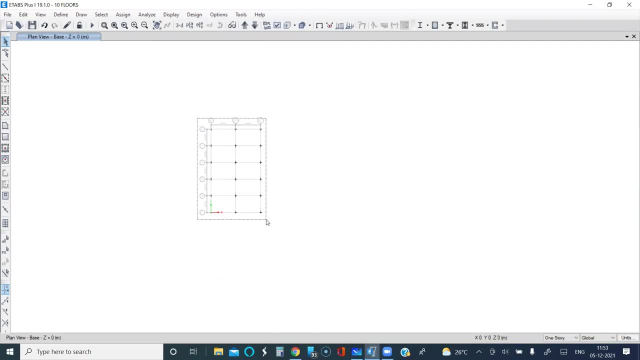 model a raft or an isolated footing and then bring in the effects of soil and make it behave as it is actual. but then that takes a lot of time. so from conventional uh time, from long time, conventionally we either fix or pin again. this is a topic that needs to be discussed in length. 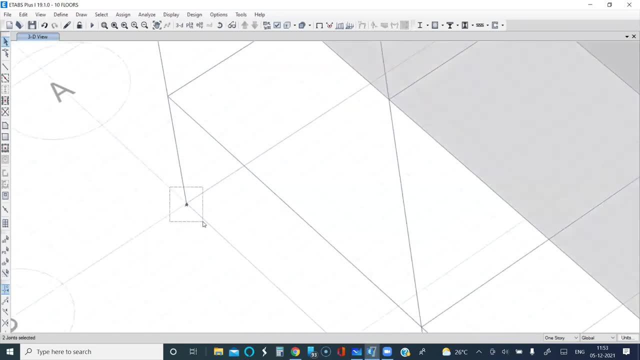 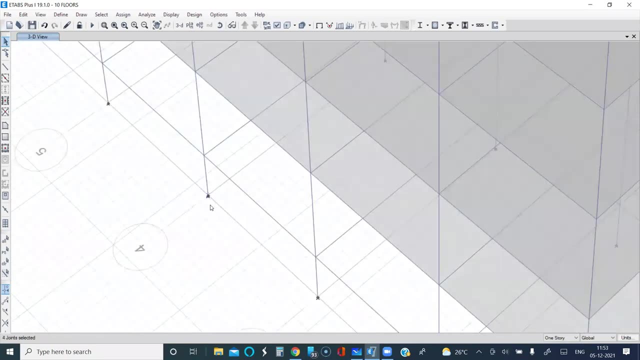 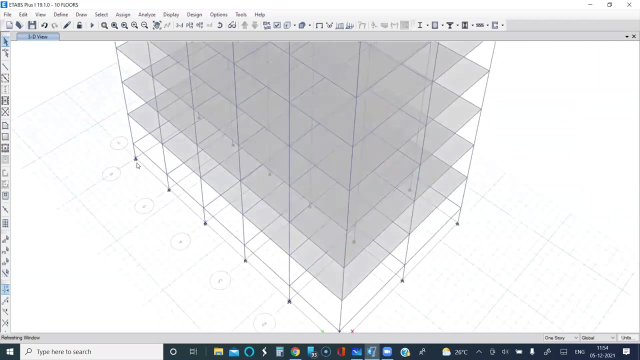 all i can tell you now is: if you pin your base, your forces will be slightly different. if you fix your base, your forces will be slightly different, in the columns and in the first joint at least. yeah, you can take a call on either of this, but then 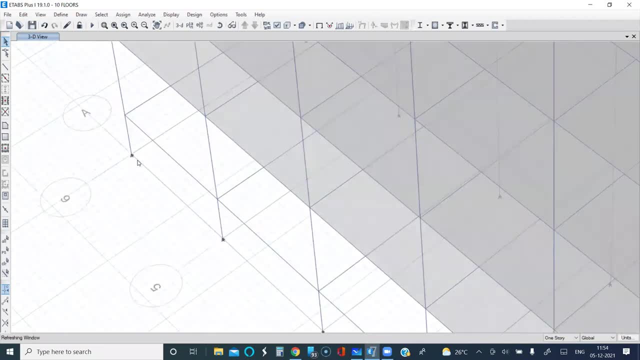 you need to have a consistent consideration throughout the project after issuing your foundation drawings. you cannot change your fixity. yeah, keep it constant throughout your project. as long as you do that, both should be fine, which is correct. both are not 100 correct. it's in between that. yeah, so i i need more time for. 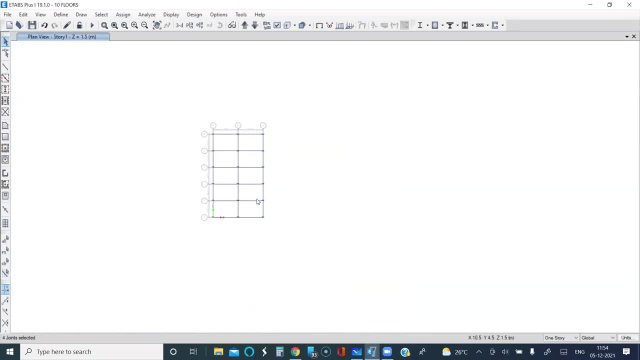 explaining this, but all i can tell you now is it's neither fix nor pin, it's something in between. so both of it is fine. as long as you are having a consistent consideration throughout the project. don't change your consideration after issuing some drawings. if you started with pinning, keep. 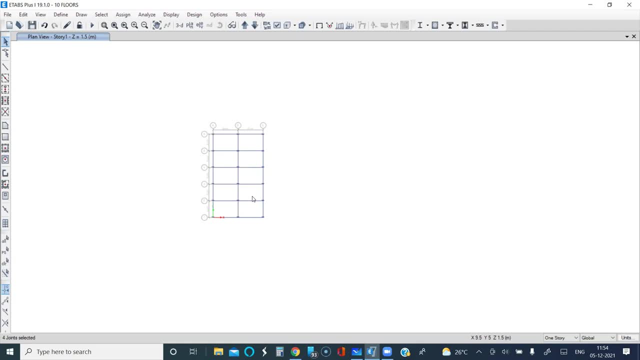 it pinned throughout. if you started fixed, do it throughout, otherwise you will have problems. why, how, what, i can't tell you right now, because it needs at least one hour again. yeah, we can have a dedicated webinar for that later now, so let us leave it pinned. okay, now let me get into the next. so all this you can not as points. 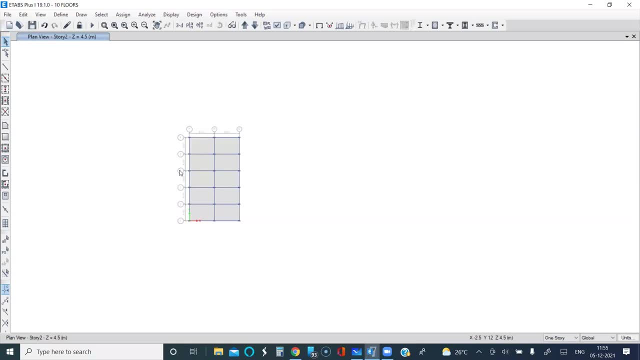 for your further learning if you don't know about it. pinning, fixing membrane, all that, all that, all that, yeah, whatever i'm saying, you can not down if you don't know for your further learning. okay, now we have to put the load, go to define load pattern. you can see dead and live, or already here. 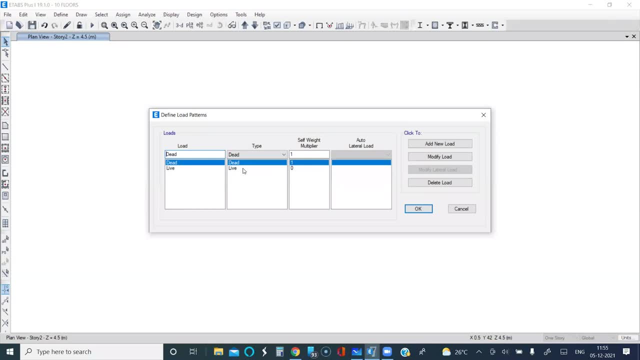 but that's only a pattern, like load case, but then your loads are not applied. yeah, only self-aid is applied, see self-aid multiplier. one means automatically that dead load would get applied. if you put the zero, then you have to calculate your dead load of the slab and input in now here. 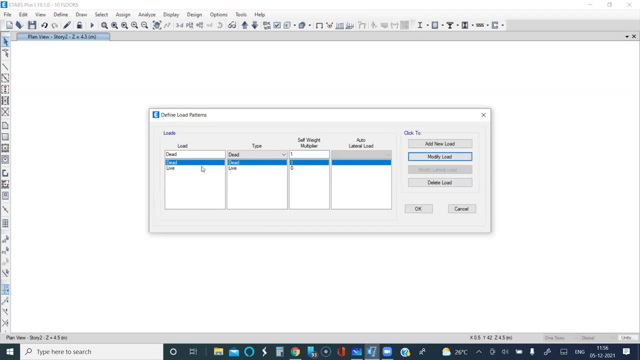 if you give one, it will automatically calculate and add your dead load. now many engineers put one here, also in live load. don't do that. that's wrong. only in dead load. one time you have to input your self-aid, which means every weight of the modeled entities. beam, columns, slabs are automatically. 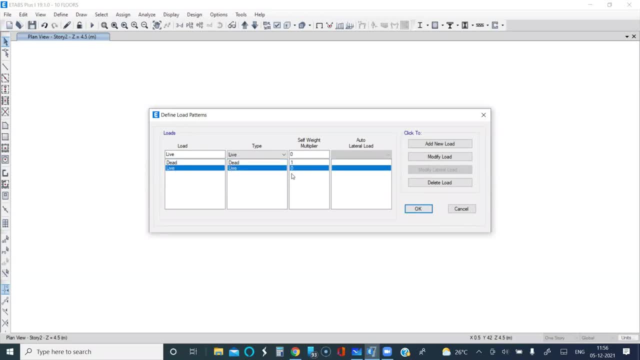 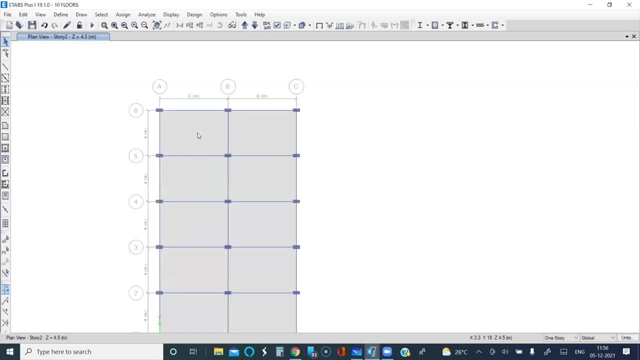 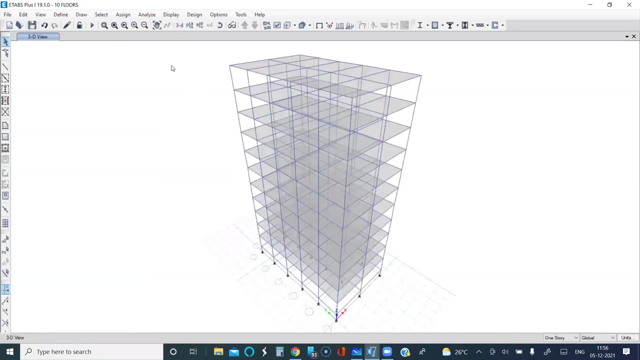 captured. okay, live load is not applied. dead load also is not applied for items which are not modded. modeled items which are modeled are loaded, but wall load is not applied. so you have to apply the wall load if you have a wall. yeah, so if you have a wall, and in most cases you will have a wall- 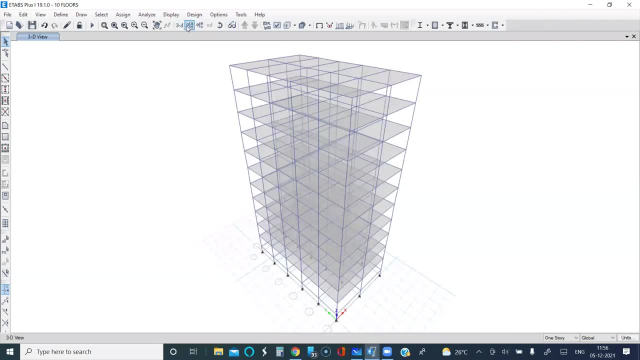 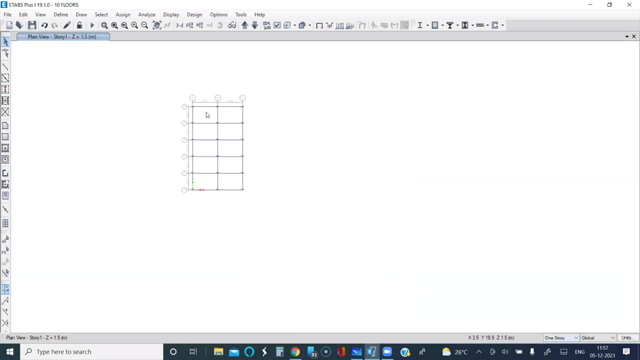 so that wall load you need to apply. how do you apply that? so i will do one thing for simplicity. i will apply show application in one level. yeah, so select all the wherever you have. so in the plinth level generally, you will have your walls at the periphery. let us assume that the lower level is. 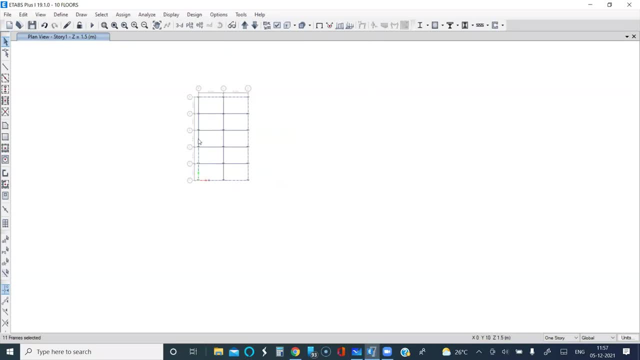 something like a parking, and only at the periphery you have your walls. you need to calculate this now. since this is a line load, this needs to be colonialized, so i will apply show application in one level. yeah, so select all the wherever you. Newton per meter. yeah, i am not going to tell you how i decided that it is kilonewton per meter. 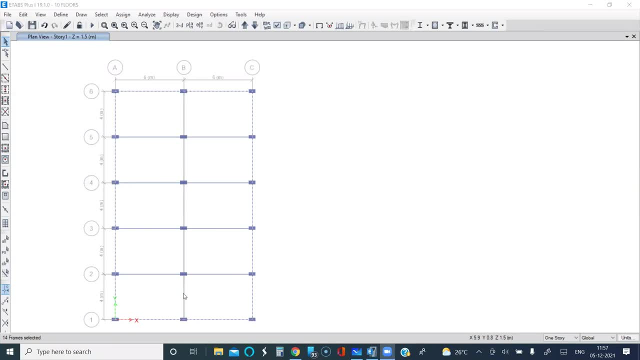 some of you may be knowing it, some of you may be not knowing it and, as he is saying, based on hard strata, it is fixed for normal soil pint. yeah, that is fine, but then there are much more rules for this that we will see later. yeah, what you said is roughly. 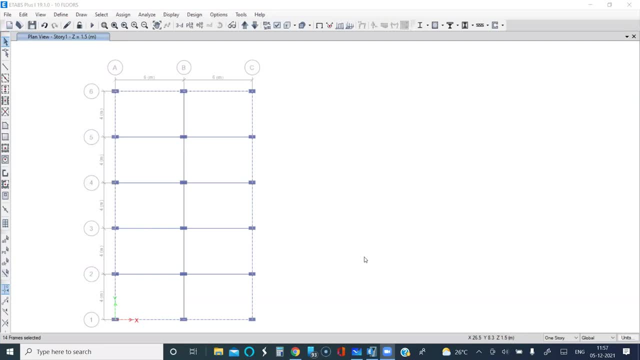 okay, but then there are many other things to be looked into. yeah, it is a udl, so it will come to around 10 to 12, based on your floor height. density multiplied by three dimensions will give you kilonewton. yeah, divided by whatever dimension you are applying that will give you kilonewton per 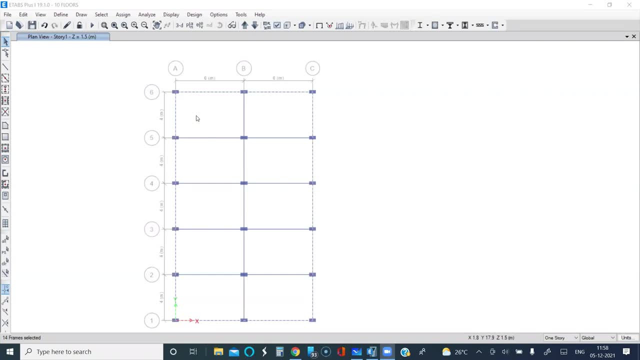 meter. so in this case, height of the wall multiplied by density, multiplied by the thickness, will give you the kilonewton per meter density: 20 multiplied by height, 3 meter minus beam depth, around 2.55. yeah, so 3 minus beam depth, 2.5 multiplied by 20, multiplied by, say, 0.23, so 11.5 will be your wall. 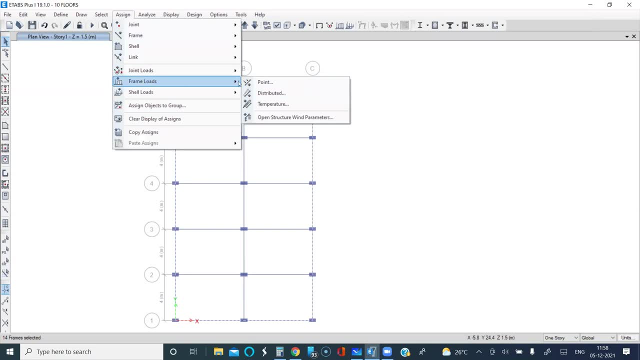 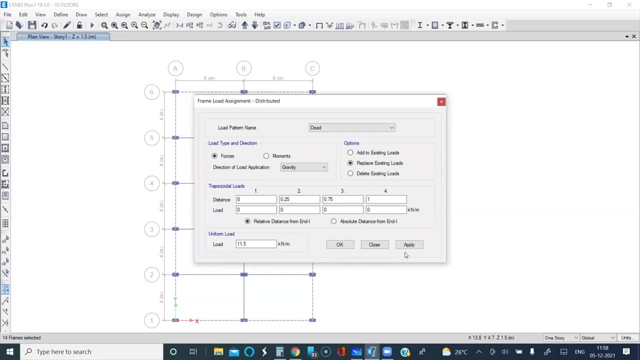 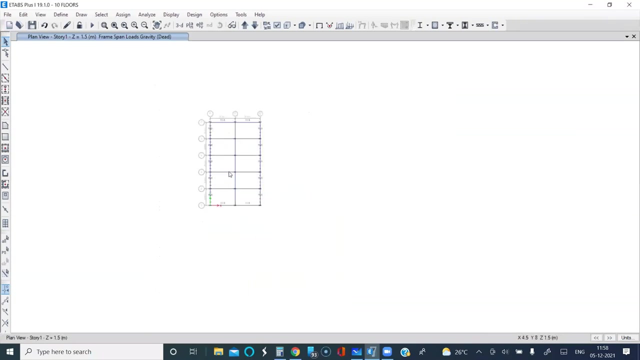 load. so assign frame loads, distributed dead 11.5. replace or add doesn't matter, so 11.5 is applied. yeah, so like this: wherever you have walls you have to apply that. i'm not doing it in all floors, it will take time, so let's do it only here. the other dead load: the slab weight, beam weight, everything. 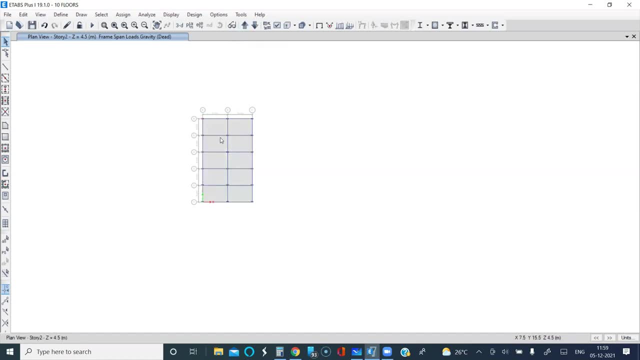 has automatically come. like: this: you have to apply in all the beams where you have wall load, fine. if you have any other loads, like a statue kept here or a big point load of an equipment, all this you need to apply. but then currently i'm not considering all that water tank staircase. all this are needed to be applied but with the time 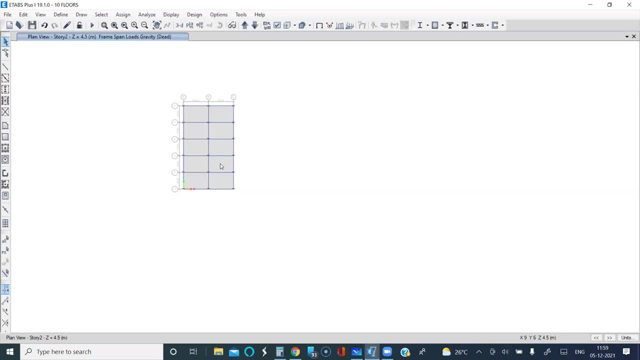 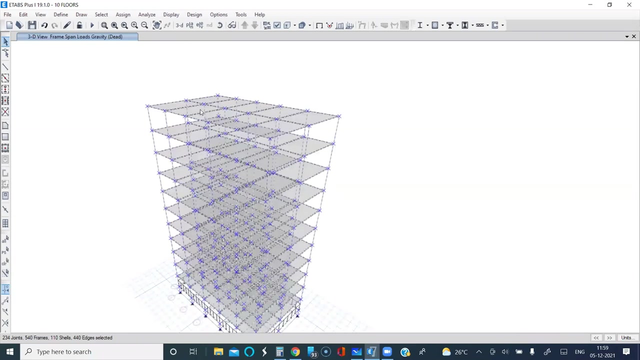 limitation. i'm ignoring that, okay, so now that's done. now live load, live load. i'm going to select everything. in fact, the live load in the terrace will be different, but i'm assuming that the terrace of this building is going to be used for assembly purpose, so i'm going to take every level load as. 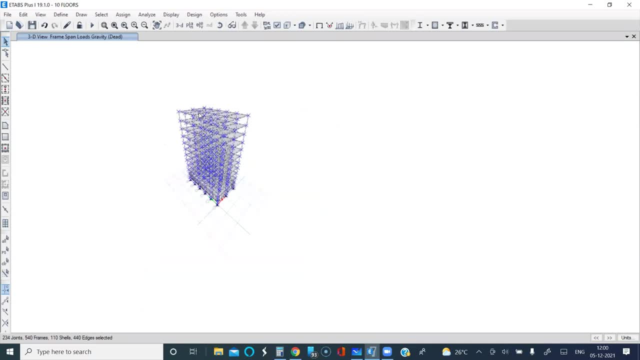 a office building. and three is the live load. how do you get that is 875, part two. so i'm going to say assign shell, shell loads, uniform live and three kilo newton per meter square this comes from is 875, part two. if it's an office building it may be 2.5 to 3 in the terrace you can reduce. 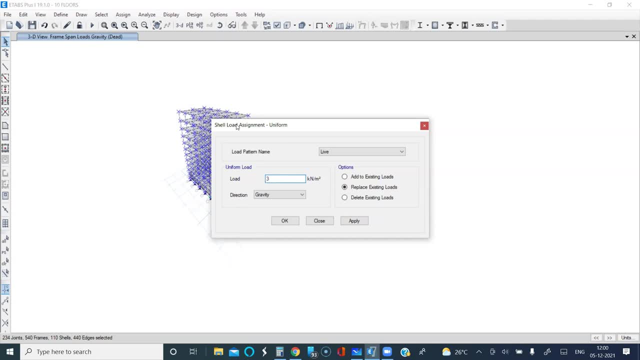 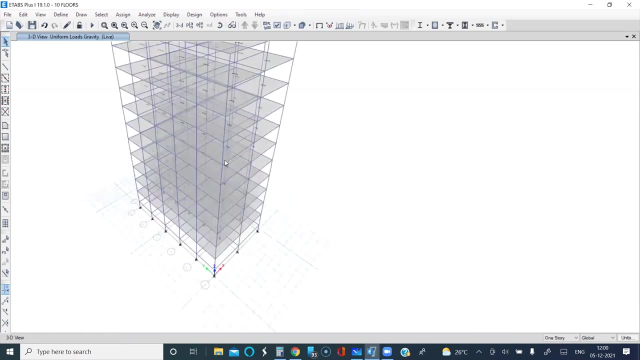 it, but then i am assuming that it is going to be used as an office building, so i'm going to take it as a assembly area for the functions and or a cafeteria or something like that. yeah, so i'm going to take three everywhere. so that's done. so we have applied dead load. we have applied live load. 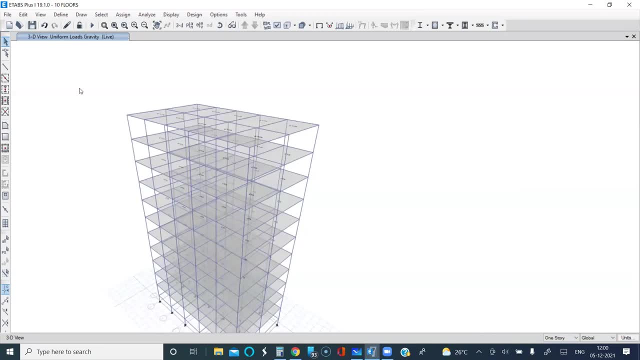 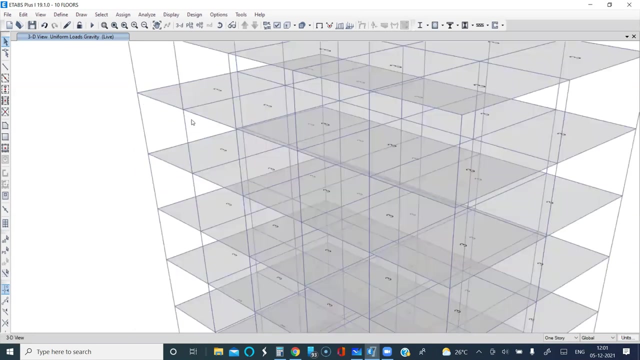 yeah, dead load. most of it will come automatic. you have to take the additional wall weight and other things which you have not modeled. separate live load you have to apply. okay. so now in all levels we have applied the live load. i have applied wall load only in one. 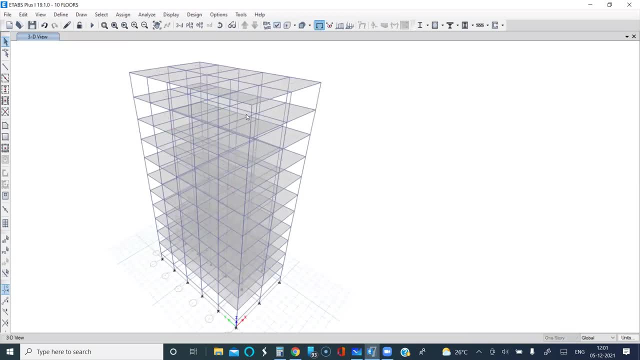 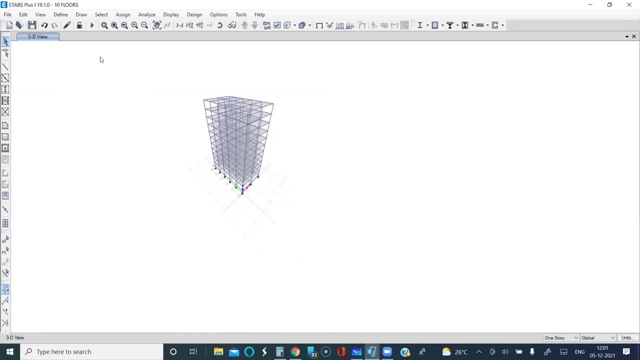 level, but you have to apply in all the levels. yeah, let us not waste time. that's the method that you have to apply now. we have to apply wind load and seismic load. now wind load: i cannot explain you every points in the code, so i'm going to quickly do it. yeah, 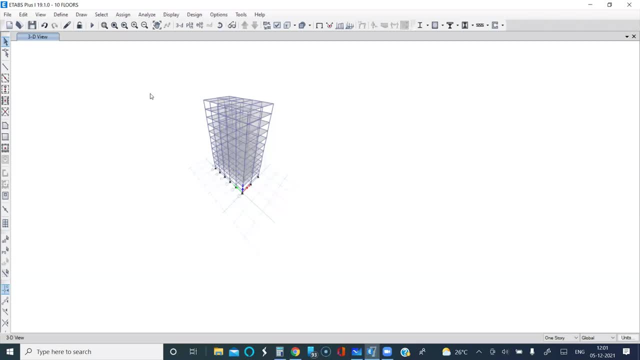 so for wind load to get applied, you need to assign a diaphragm for your slabs. now, what is a diaphragm? diaphragm in e-tabs has two requirements. one is to ensure that your rigidity of the slab, or the stiffness of your slab, or the diaphragm action of your slab, is. 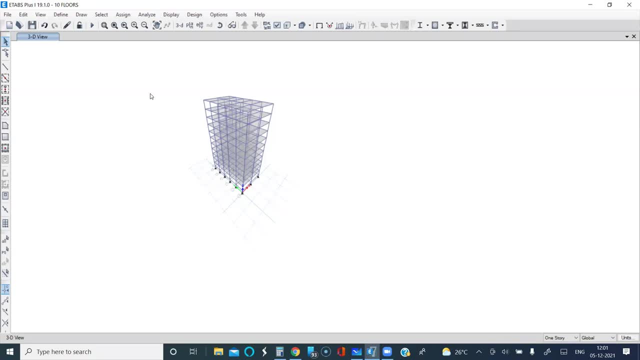 brought into your structure. yeah, that's one reason. second reason is that any wind load can be applied only if diaphragm is modeled. yeah, so define. there is something called diaphragm here. d1 modify. now there are two options: rigid and semi-rigid. i would go with rigid in this case. 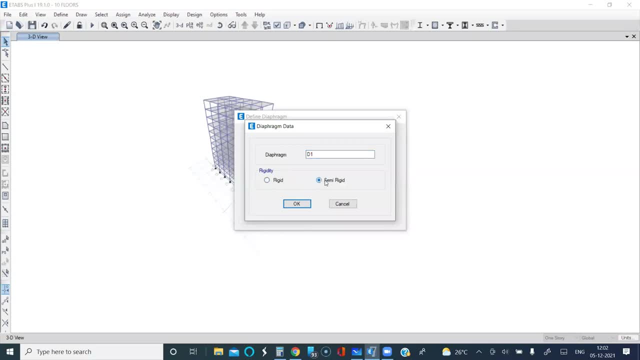 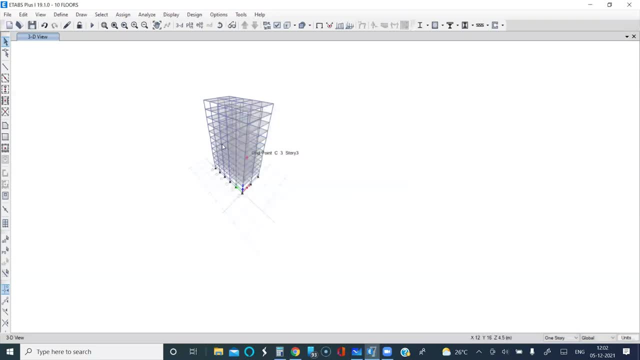 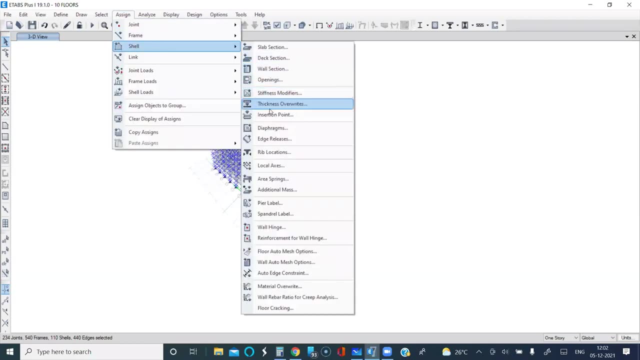 going to take rigid and then say, okay, now i'm selecting all the diaphragm or the slabs and then say assign shell and then there will be an option here: diaphragm so d1. so i have applied a rigid diaphragm and that's what is seen here. 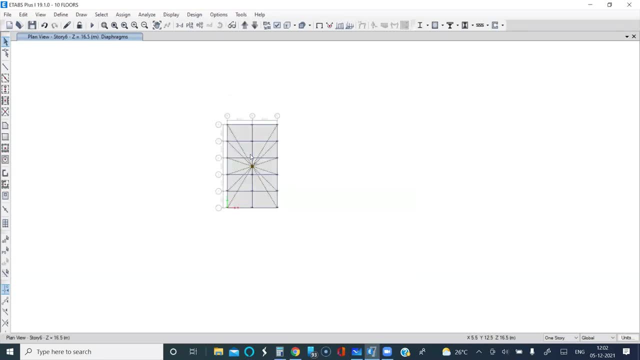 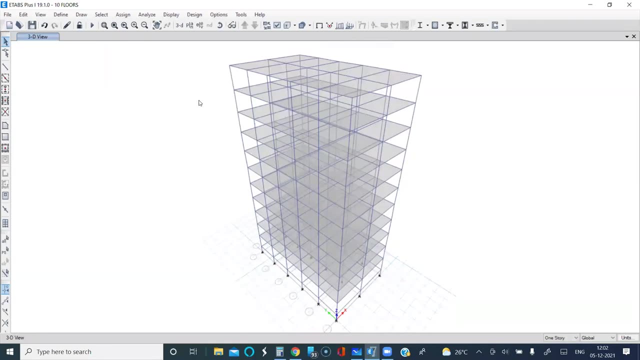 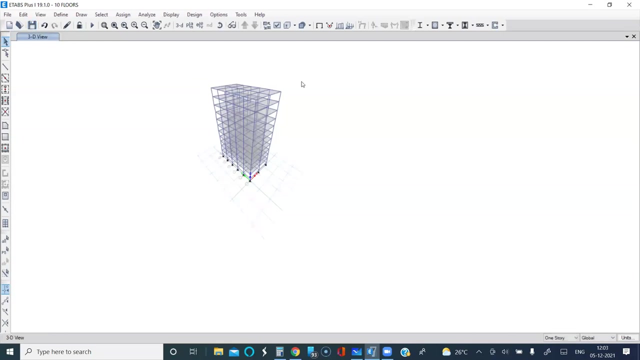 as a rigid diaphragm. yeah, so this is bringing in the rigidity of the slab in that plane and for wind load modeling that is a mandatory thing as well, so i'll save this. so we have done the diaphragm. now go to define. go to load patterns. again. in the load pattern you have to define your. 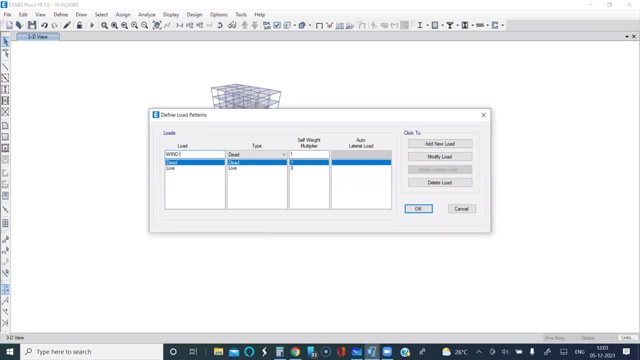 wind load. so i'm going to say wind x. i will say wind. here you can take the code as per which you want. the wind load so i'm going to take is 875, 2015. yeah, and then say new load. i'm going to say modify exposure from extent of diaphragm. 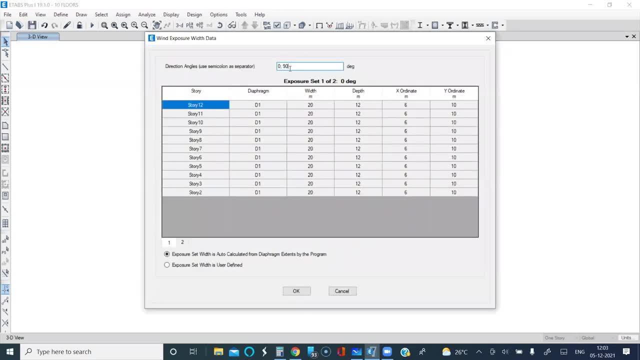 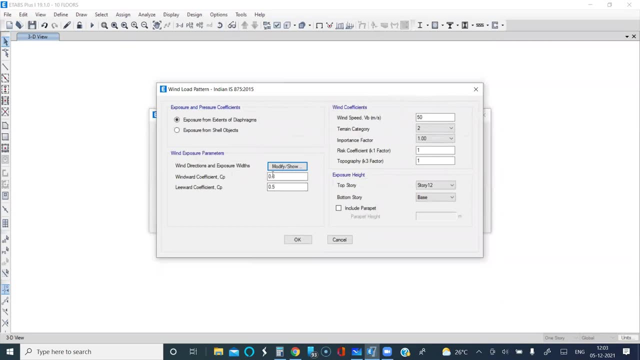 modify: show in x direction. zero degree. zero degree means x direction. this you need to go as per the code. i cannot again completely show you this because there is limitation to explain the code. so you have to go to code and go to table three or four and get this data cpe. 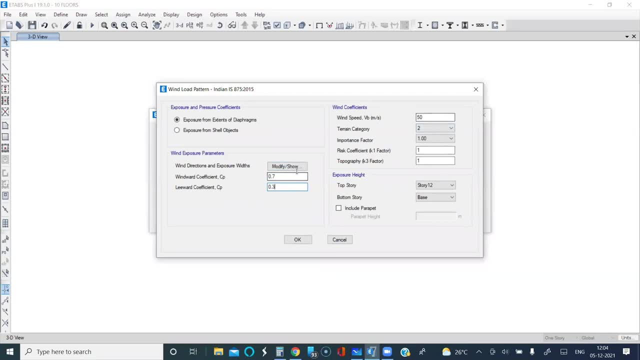 yeah, i'm blindly typing this. it could be different. it depends on the size of your building. yeah, so i'm going to go with 33 wind speed, assuming that the project is in bangalore. all these are parameters that are directly readable from code. okay, so these parameters. i'm not explaining you how to calculate the wind load here. 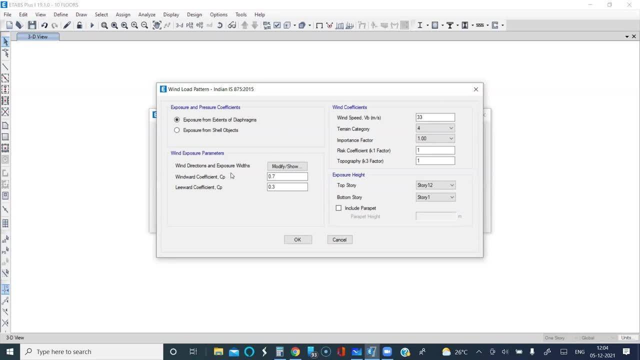 what you have to do is your load is cpe multiplied by. who can tell me external pressure coefficient? so that's what we defined here. this comes from table. this is your basic wind speed. this is the terrain calculation of the wind speed. this is the terrain calculation of the wind speed. this is the 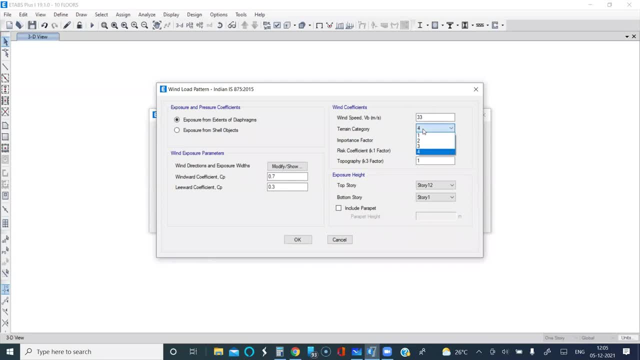 category means if your building is in a village, if your building is in a city. it all depends on the wind speeds. so all these are accounted. these are directly readable in is 875, part 3. yeah, now, the important thing that you need to understand is your wind should be applied from plinth to 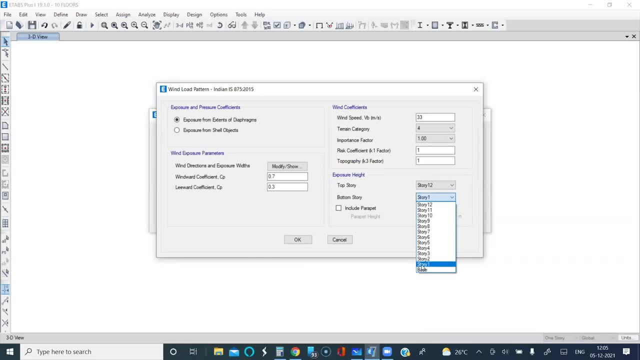 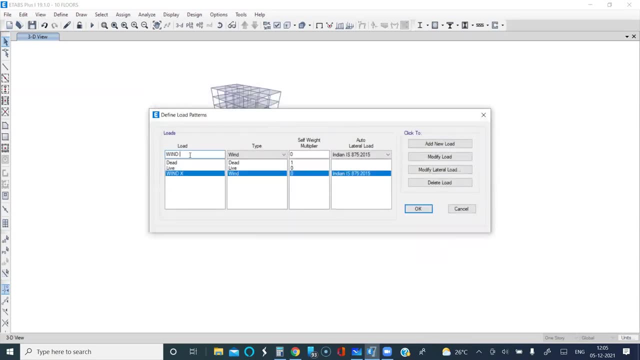 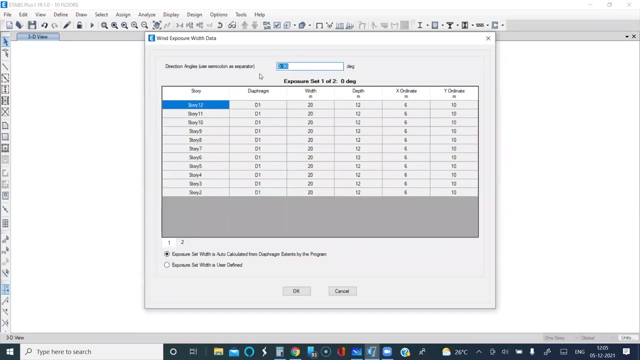 last level. yeah, so you can choose not base but story one. so i'm going to say, okay, now. next is wind in the other direction. add new load modify here. i'm going to change this to 90. now you can apply 0 and 90 or x and y. 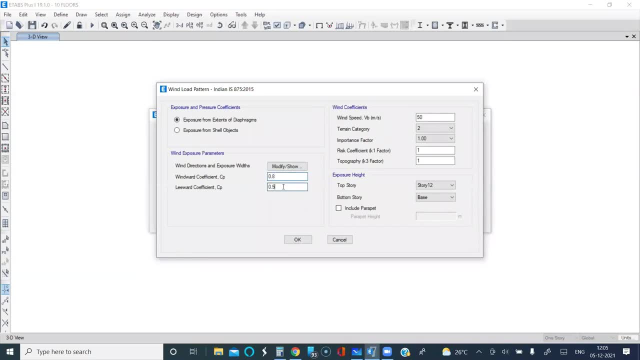 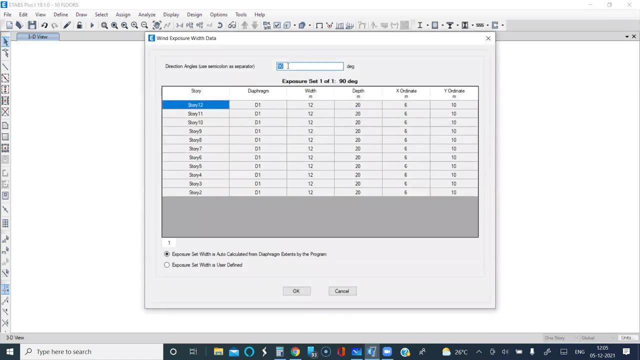 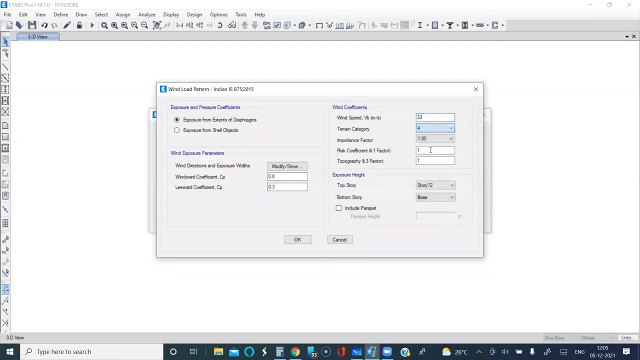 simultaneously. also. i'm not doing it for some other reason, so the cpe may be different in both directions. so that's the reason i have split this into two directions. if you really want, you can apply it in one direction also, but i'm not doing it, fine, so 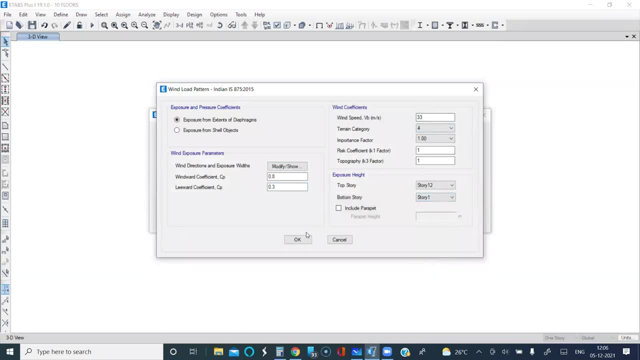 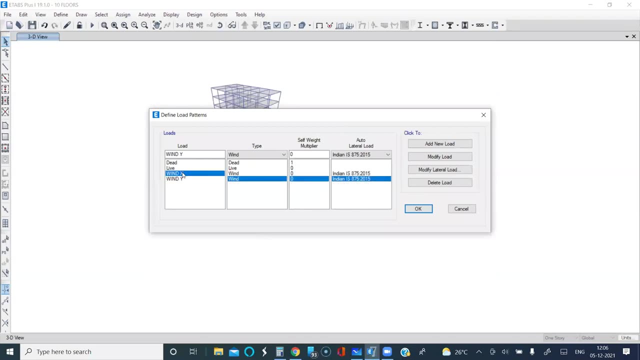 this is your wind load in the other direction. now those who know something about wind load please think why i am applying only in x and y direction. wind can come in any direction, so why are we applying wind load and earthquake load in x and y direction only? why don't we apply in other? 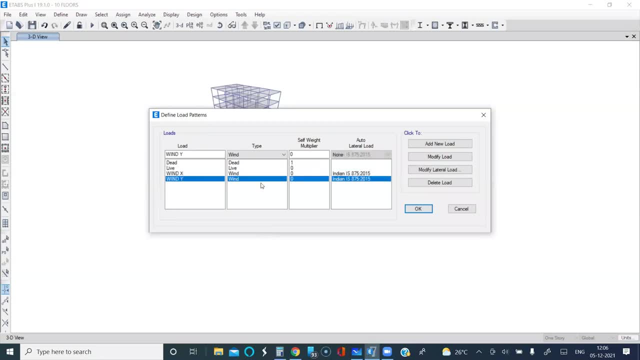 direction. it's a food for thought. think about it and then tell me later. yeah, we don't have time again to discuss that. so these are the minor, minor or important points, not minor, major points. but people don't think, students don't think about this. why are we applying only in x? 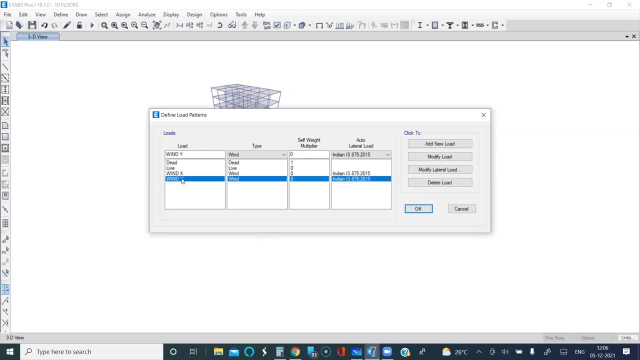 direction and y direction, when wind can come in any direction, same way seismic also can come in any direction, but we are applying in etabs or stad or anywhere, only in two direction. why, if anybody has an answer, they can type: okay, now, next is seismic. so i'm going to say eq or i will show you from. 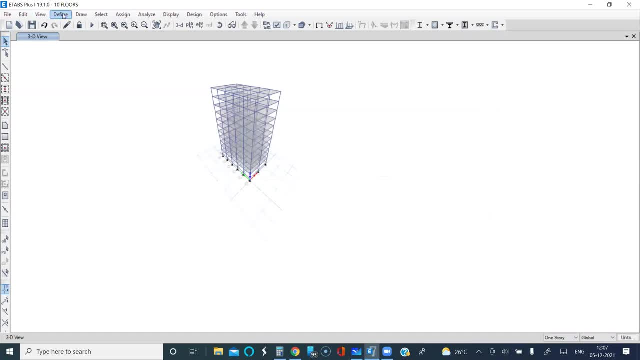 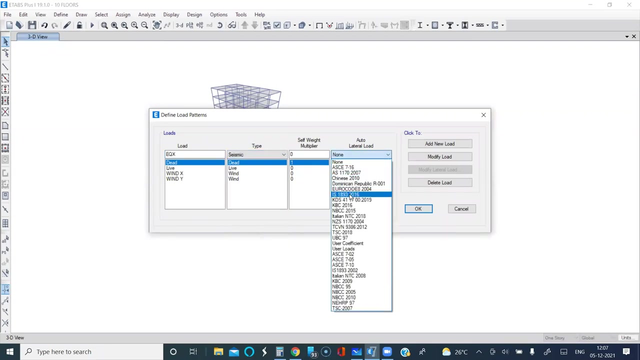 beginning. that is, you go to define load patterns. yeah, so load patterns windex. we have done so. i'm going to give eq x here. i'm going to take seismic again. here you have to take the code is 1893 again. add new load, then modify lateral load. 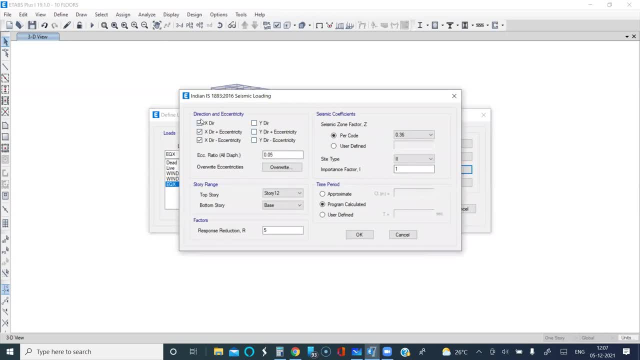 so i'm going to put x direction first. now, here you have x direction plus eccentricity, minus eccentricity. i'm ignoring this right now. again, this is an advanced thing. we will see that later. yeah, that is what is this? x direction plus eccentricity, minus eccentricity. i'm currently 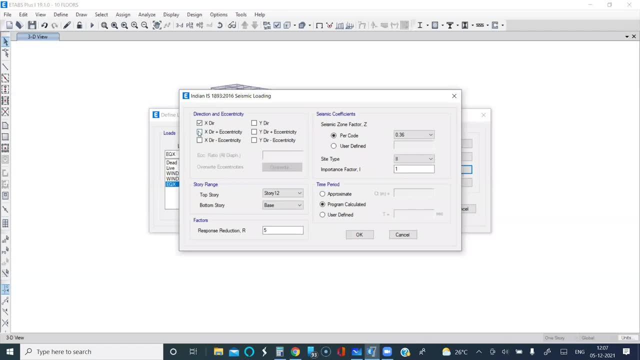 ignoring that, but this is something which you need to consider. but at this point in time i'm making it simple. so x direction from base to twelfth floor. that's where the seismic acts. now these are again. code specific 1893 2016. you have to see here: r means response reduction factor. this is 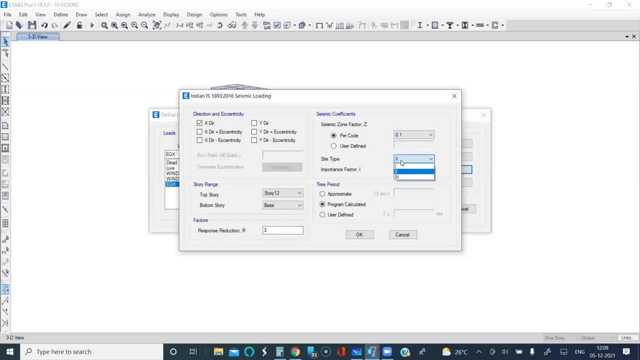 your zone factor. this is your type of soil, this is your importance factor. yeah, time period you have to calculate. Now I will quickly explain this because many of you may be confused about this, Because building resists itself. We will see that in the end, after the webinar, we will be discussing about that. 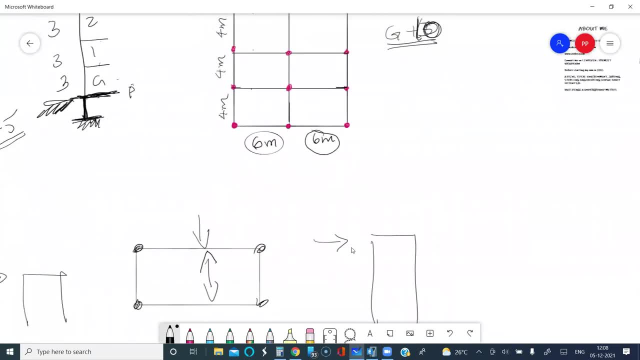 So be there. Now very quickly, I will explain you what is earthquake. Many think that earthquake is a wave coming and hitting your building. It's not like that. So if you have a building like this, say your ground is moving, that is earthquake. 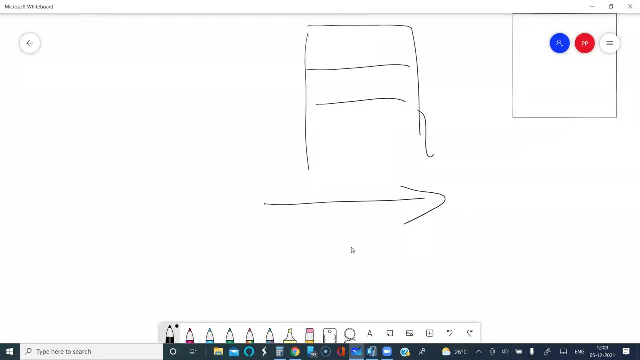 Ground moves or the plate moves, very minor movement. It's like you are standing in a bus. You are standing in a bus and the bus is taking off. What happens if you are not? if you are holding also somewhere, if you are holding also, all your joints will start paining if the bus moves suddenly. 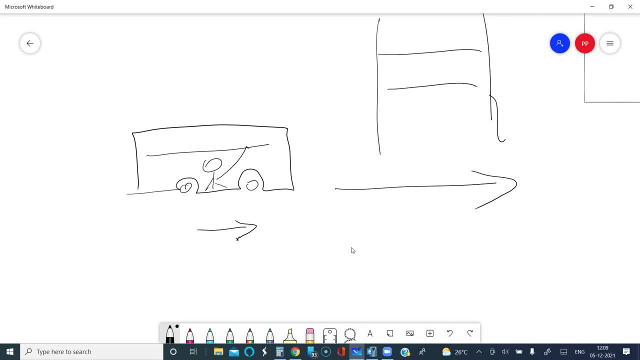 Why? Because all the force, All the force is acting at the joints where you have. What is that? It's inertia. That is, all of us are in the buses moving. You are being pulled into the center of the earth, So there is something stopping you from moving. 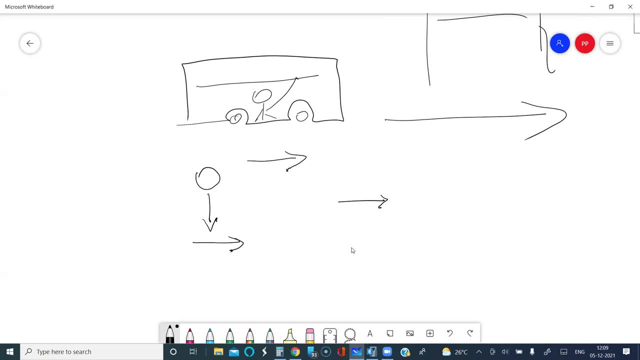 What is stopping you from moving The gravity? The gravity is to the center of the earth. The bus is moving horizontally. When you are being pulled vertically, you are resisting that horizontal movement. That is inertia, the reluctance to move. Or 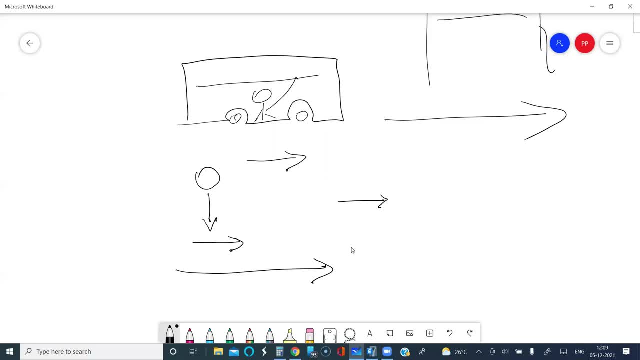 the wish to stay there because of the gravity. Yeah, So that is what inertia is. Because of that inertia, your joints get a lot of pain if the bus is moving very fast Or when the bus breaks suddenly. That's what earthquake is all about. 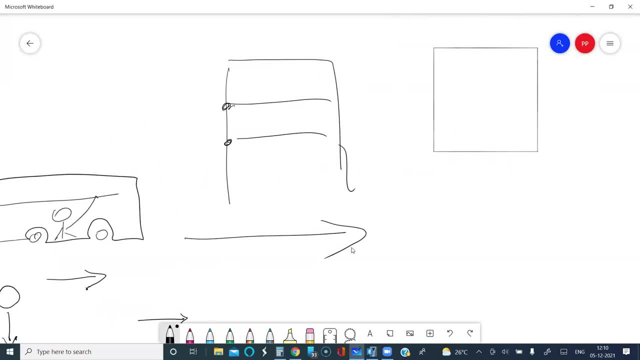 There is a sudden movement. Yeah, So all your column beam junction will get that thrust. What is that thrust? Your own weight. In the case of a building, what is your own weight? What is its own weight? It's building's weight. 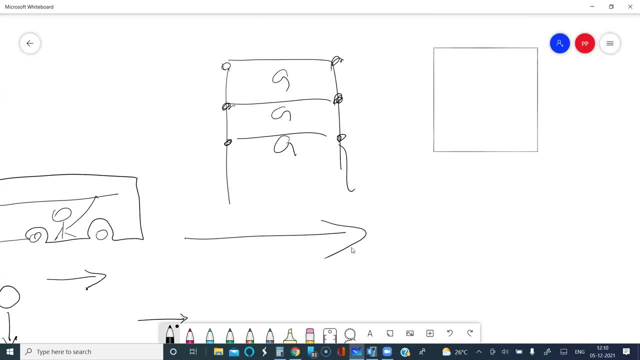 Yeah. So the gravity weight of your building adds up as an inertial mass. So your own or building's own weight is becoming a lateral thrust at these points. That's what's happening. That's what earthquake is, Nothing else, It's not a wave coming and hitting your building. 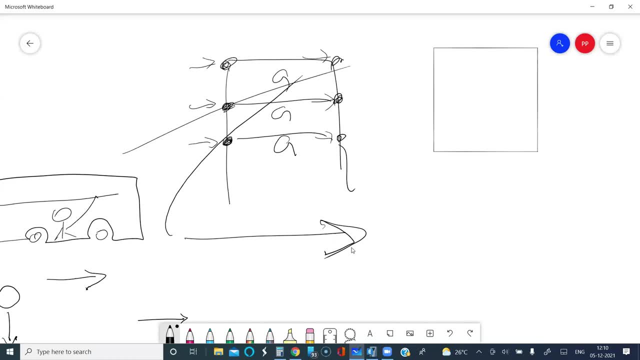 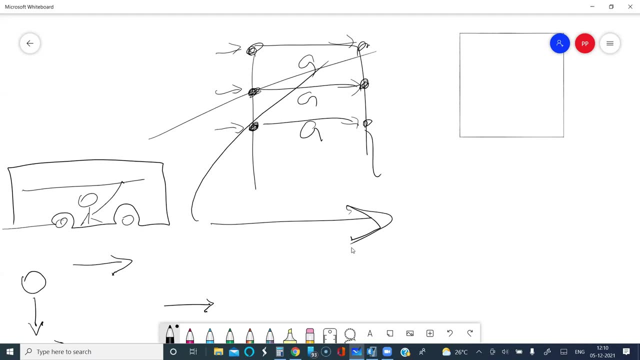 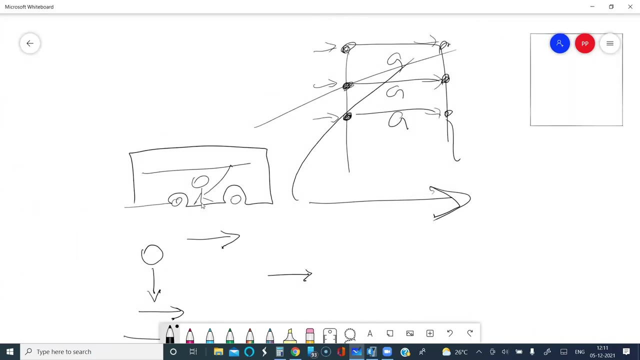 No, it's not that, Because of the ground movement, there is an inertia and that inertia lumps, or that inertia generates thrust. Thrust at the column beam junction, And that's what you are interested to apply. Yeah, So there are a lot of limitations because you don't know what is the speed of the ground. 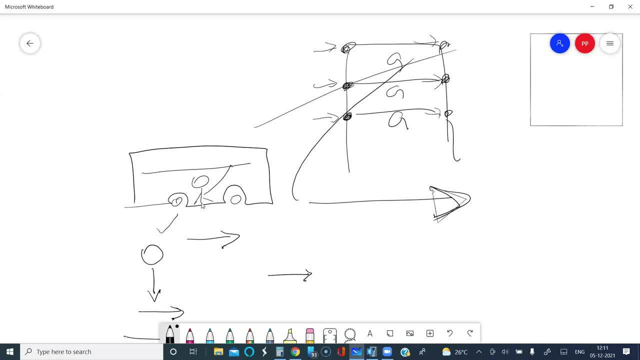 or the acceleration of the ground. You know the bus acceleration, but you don't know the earthquake acceleration. So what do you do? So for that, based on various research, based on history, based on seismological studies, engineers and scientists, 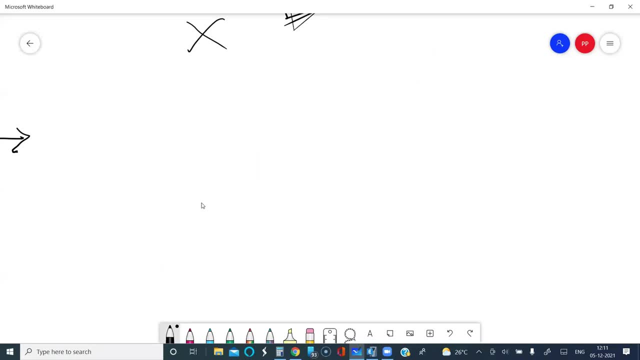 Have come up with a formula. What is that? Who can tell me the formula for the earthquake force? This is in 1893.. V be equal to H multiplied by W. What is this? W? Building's weight? Vertically acting, you convert that into horizontal inertia. 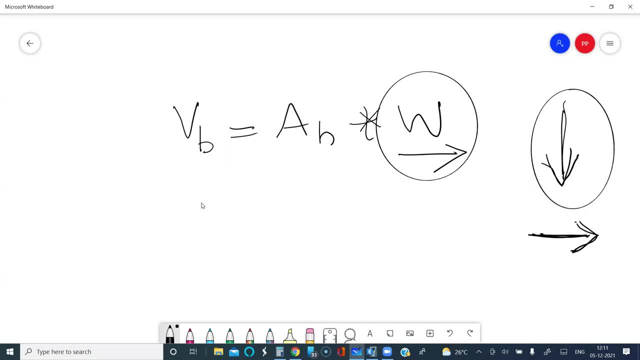 Same vertical, You add, You add, You add as, or add with gravity, as horizontal. That is this W. You call it seismic mass. What is acceleration? That's the acceleration of the ground. How much it is, I don't know. 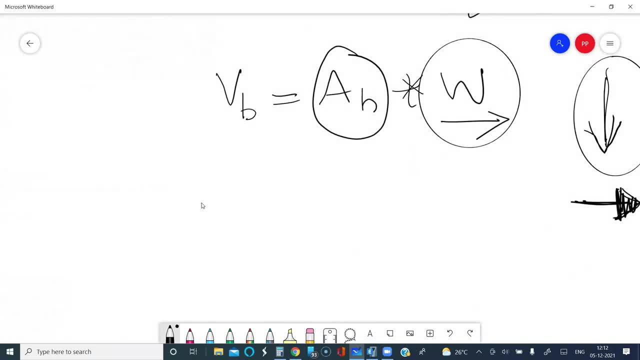 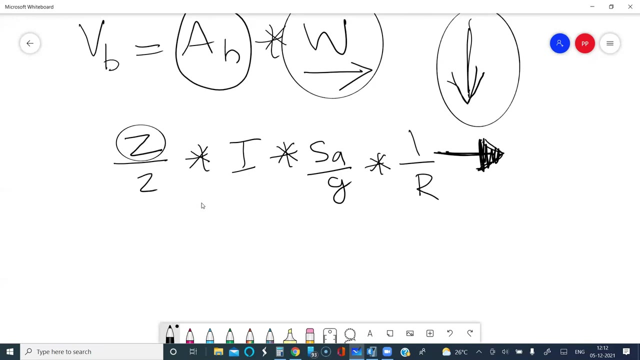 You don't know, Nobody knows. So the code gives you a formula. What is that Zone factor? by 2, multiplied by I, multiplied by SA, by G, multiplied by 1, by R? This is a formula. Z is zone factor. If you are in Bangalore, it is 0.1.. 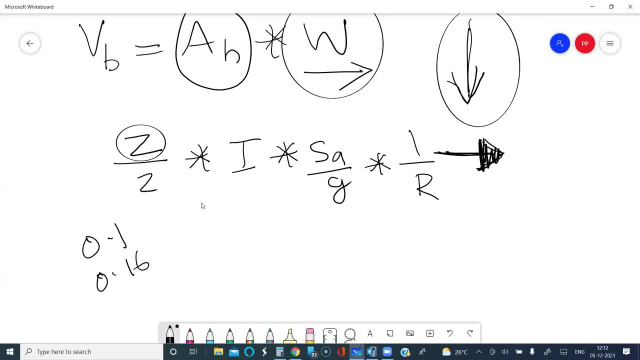 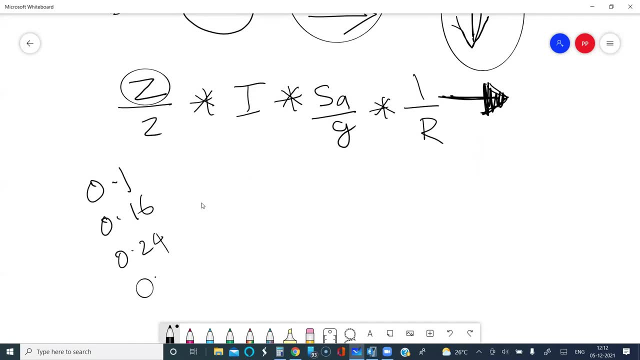 If you are in zone 3, it is 0.16.. If you are in zone 3, it is, I think, 0.24.. And in zone- this is zone 2,, 3,, 4, and 6,, 0.36, I guess. 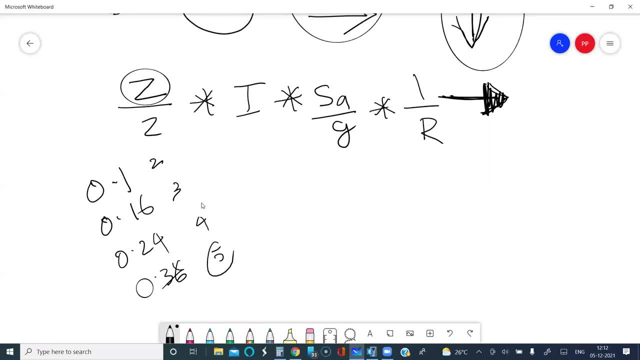 So that's in zone 5.. If you refer 1893, you will get this. So let us go with zone 2.. now, that is 0.1. what is i importance factor? you have three factors: 1, 1.2, 1.5 for normal buildings. 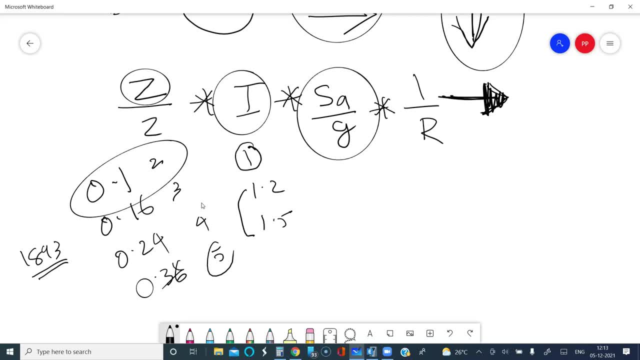 it is 1. you can refer code sa by g. again, it is a factor based on your time period and your soil type. yeah, based on soil type and your time period of the building, sa by g differs r if you are doing ductile detailing or not. yesterday i had done a blog. 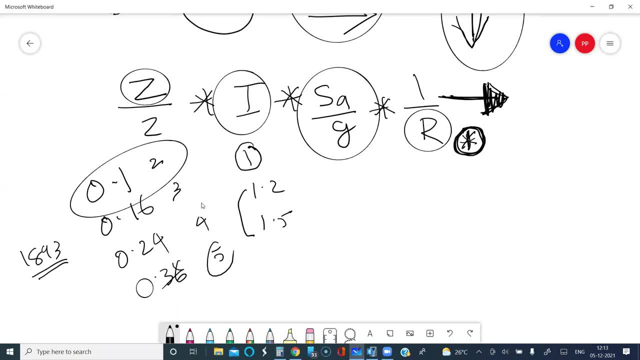 on this. it's very important to understand what ductility is. so r equal to three or five? it's very, very important topic. unfortunately, i need one hour for that. yeah, so three if you are doing non-ductile detailing, five if you are doing ductile detailing. yeah, so that is what the code. 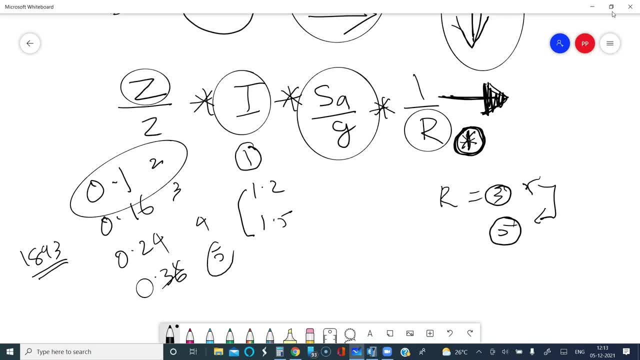 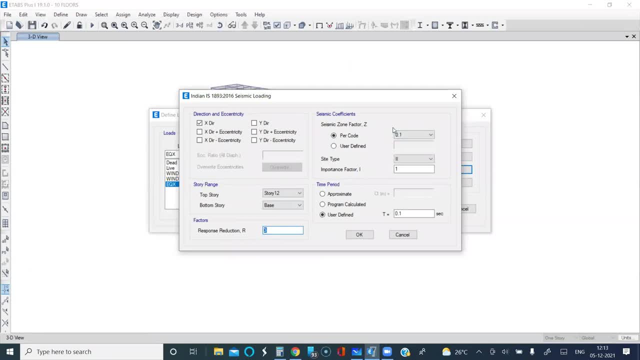 tells you why, what, when. that's a different thing. so currently we are going to use three r zone factor. i am considering the building to be in bangalore, so 0.1 soil type. this is needed for calculating sa by g importance factor. i am taking it as a normal building one. now time. 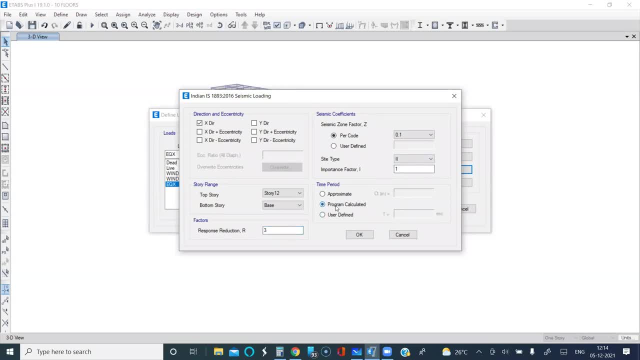 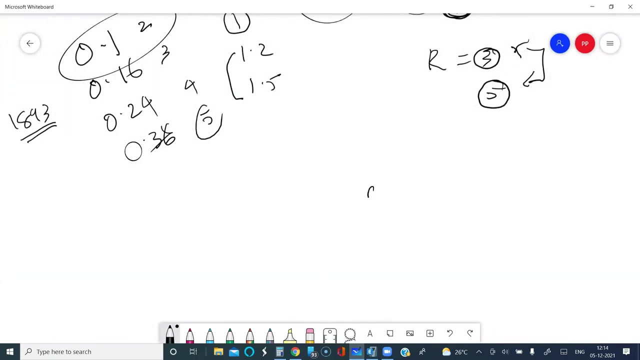 period. many engineers use program calculated, thinking that etabs will calculate. no, don't give that user defined. yeah, you have to give it user defined now. this is again based on your code. the formula for this is the formula: yeah, so this is the height of your building, d is the direction. say for: 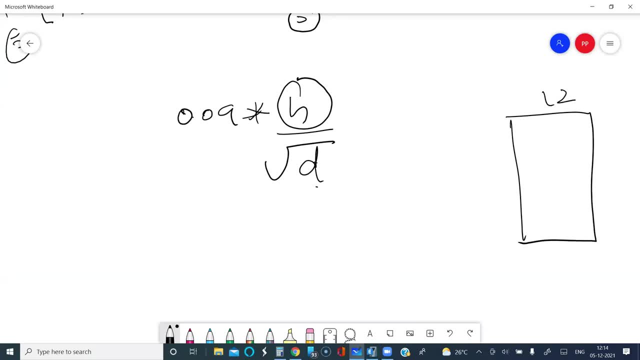 example, if this is your building, you have 12 meter. i think. here you have 16 meter, right? i don't remember whatever, it is 16 or 20, we have. yeah, so in this direction, your t time period is 0.09 multiplied by height of the building, which is 30 or 31.5, whatever, 10 floors. 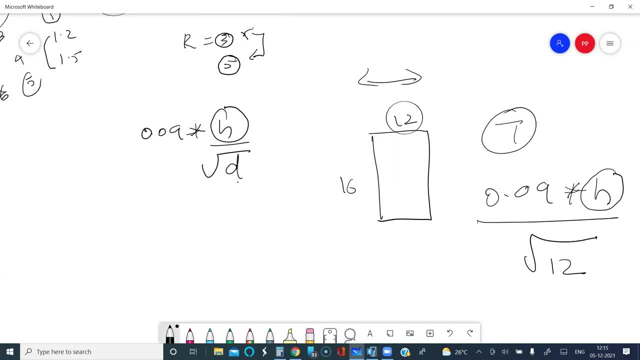 divided by root of 12, that is, in x direction. in this direction, same 0.09 h by root of 10.. distance: yeah, so in both direction you have two different values. this is when you have walls in your building. if you don't have walls, there is a different formula that if you don't. 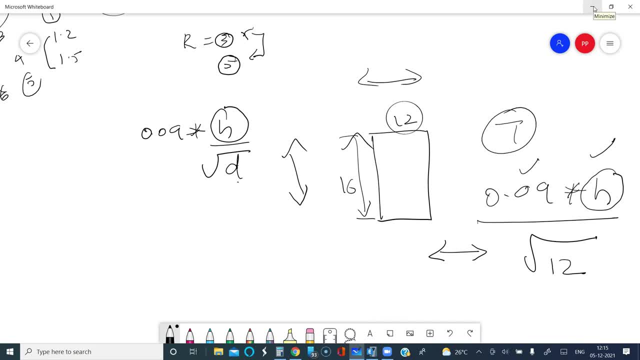 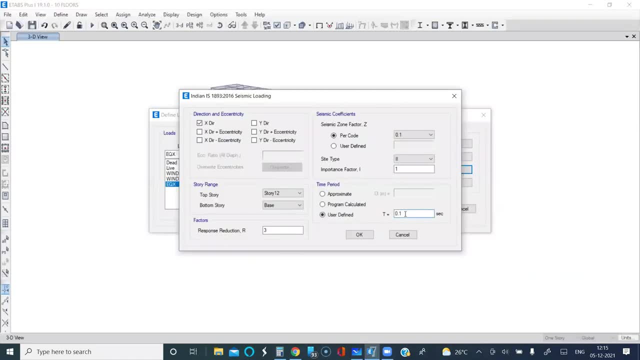 if you are not aware, please get into 1893 and understand about that. yeah, but it's all about calculating that. it's very simple, so i'm not calculating it here. i'm just taking it as 0.25. i don't blindly take 0.25. you have to calculate it. i don't have time, so that's the reason i'm 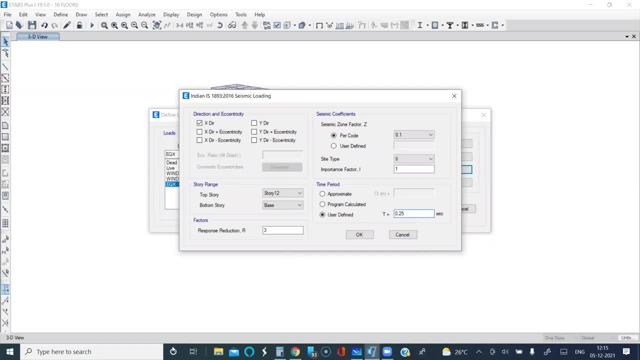 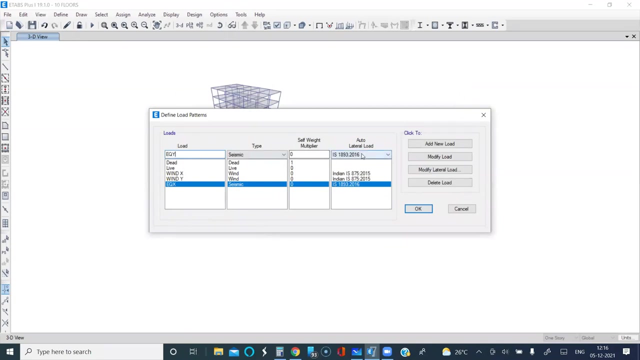 giving a value here. if you have calculated, please give me the value. i will write that okay. so as simple as that. but you need to understand how this is done now. eqy seismic 1893. add new load. modify lateral load. here i'm going to make it y direction in the 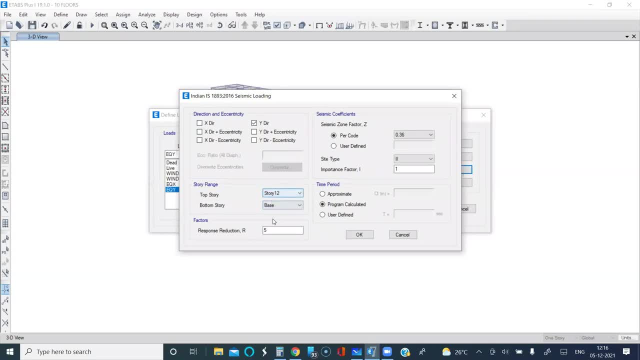 other direction. again based to 12 r, value 3, but y r is 3. that's very important. 0.1 importance factor one user defined. again, you have to calculate this. i don't have time to calculate it. i'm giving it a blind value: 0.09 h by root. d is the value if you have infill panels. 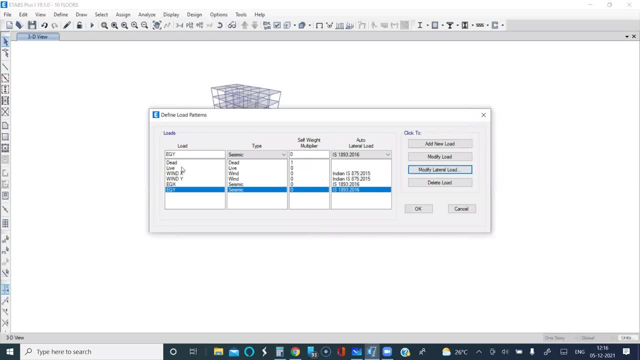 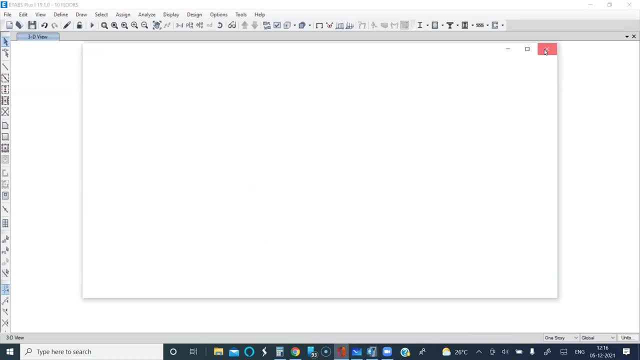 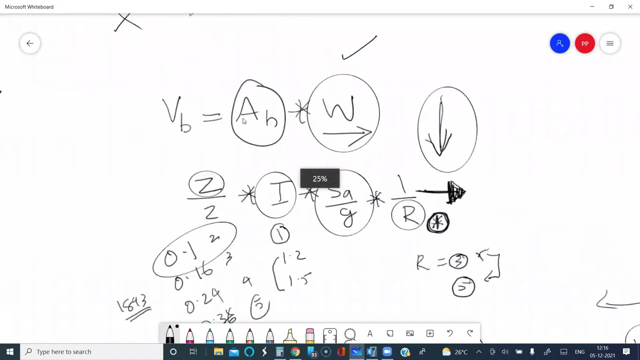 yeah, so i'm going to give this. So you have done dead life, wind and earthquake. Now I told you Vb equal to h multiplied by w. Acceleration z- we have given 0.1, i- we have given 1,. 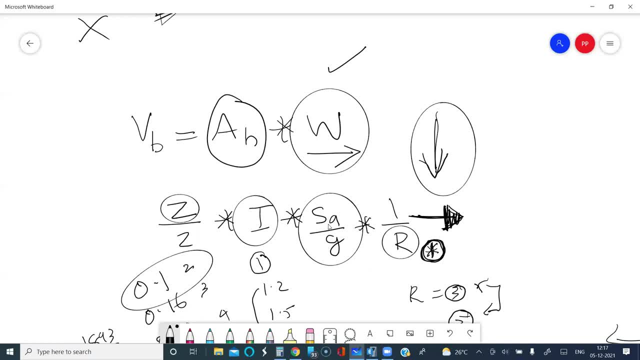 r, we have given 3.. Sayg: it's related to soil type. We have given soil type, So ETABS will calculate. And it's also related to time period- Time period also we have given. So Sa by g, ETABS will internally calculate. What about w? I told you w is nothing but. 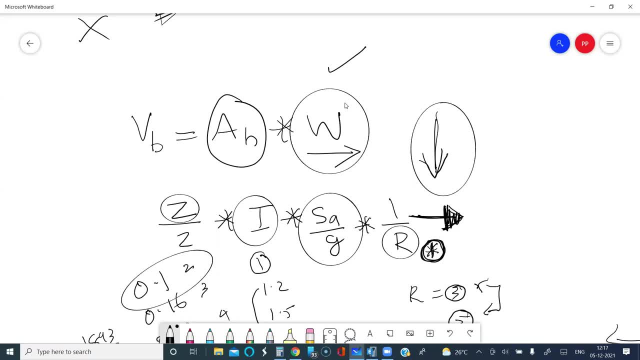 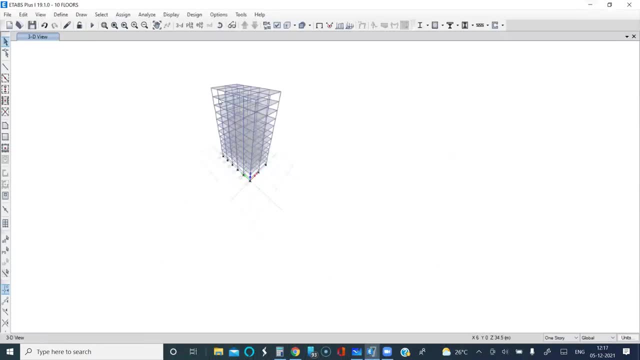 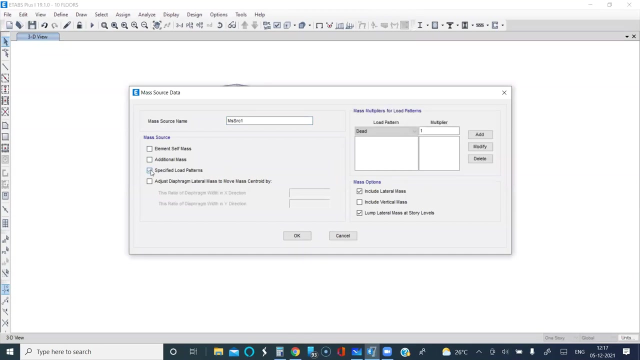 the building zone weight applied as lateral. because of inertia, the vertical load is getting added up as lateral load, So that you need to define- and that's what you have in define- something called mass source. So click on mass source Modify. I would recommend you to go with specified load patterns. We have dead load pattern and we 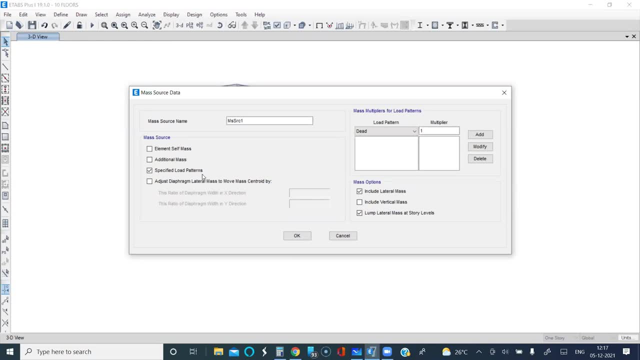 have live load pattern: wind and earthquake, all these patterns we have done now. So here, what is the inertial mass which is subjected to inertia? Dead load. So dead load into 1. Full dead load I have taken as live load. So dead load into 1. Full dead load I have taken as live load. So 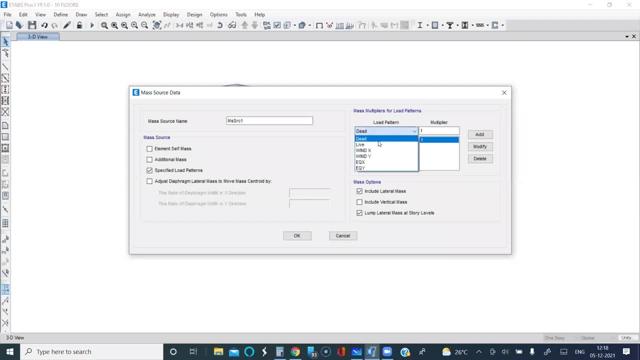 that's the meaning of this Live load As per code. you don't have to take full live load as lateral inertial mass. The reason is that most of the times when code says that the live load is 3, it is very much high. Actual load in the building will be much lesser If I say that the hotel 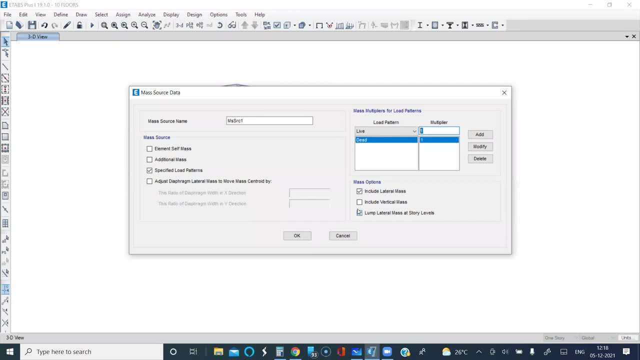 building or office building is 3 kilo Newton per meter, 3 kilo Newton per meter square. actually that will be much less. That 3 will come only if the room is full of people. So code gives you an 11's code tells you that you can take less, 0.25 or 0.5.. So I am taking. 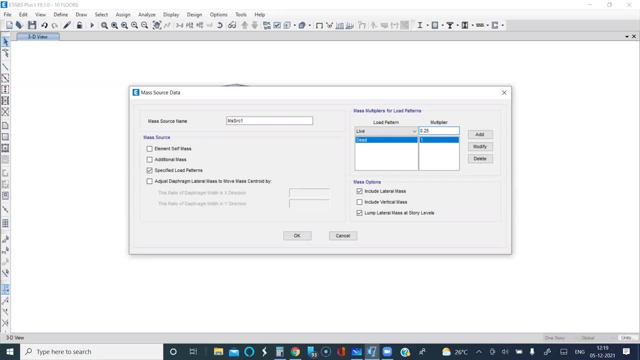 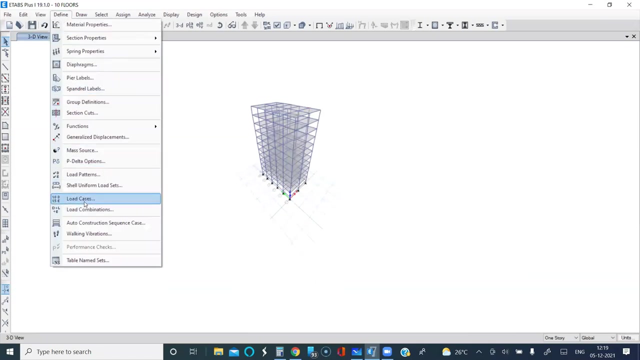 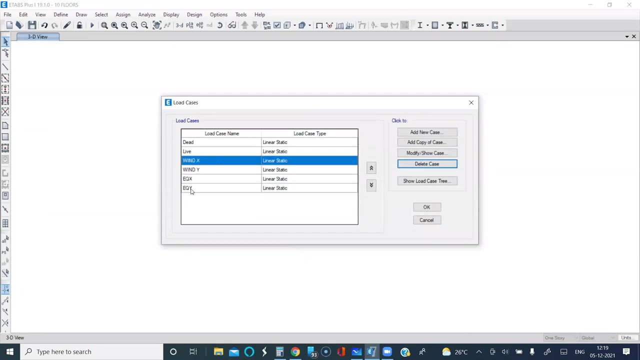 0.25.. Again, 1893, you can go and check. Only 0.25 is needed. Load lateral mass: lump lateral mass at story levels. So I am going to say, okay, So you have done with your loading, Define load case. So you have dead live wind, earthquake and earthquake. 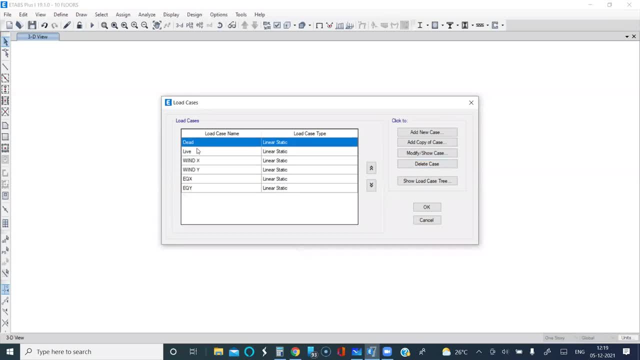 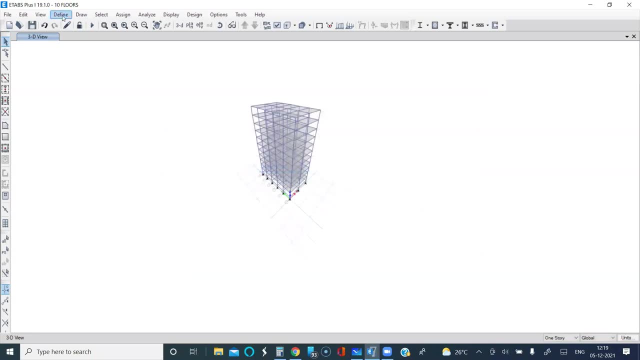 So load pattern: load case. You need to once ensure that all load pattern has come into your case. Done, Define load combinations. You can create auto combinations. So add default design combo, Concrete frame design. Convert to user combinations. Click on okay. So you get 26 load. 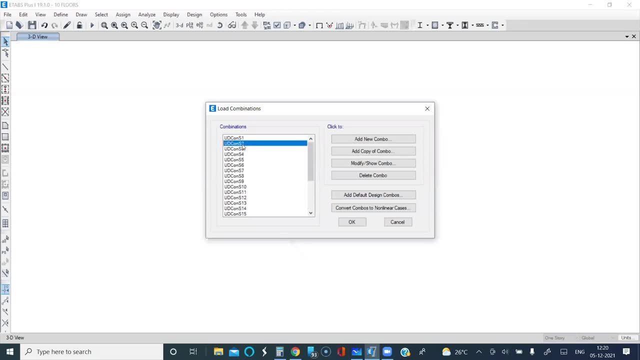 combinations automatically, But you need to know what are these combinations. Please go to IS455. And understand the load combinations. You will have all the combinations as per that in this Done See. Now you are done with your modeling and your load application. Now I have not explained a lot of things. I am aware that some of you might. 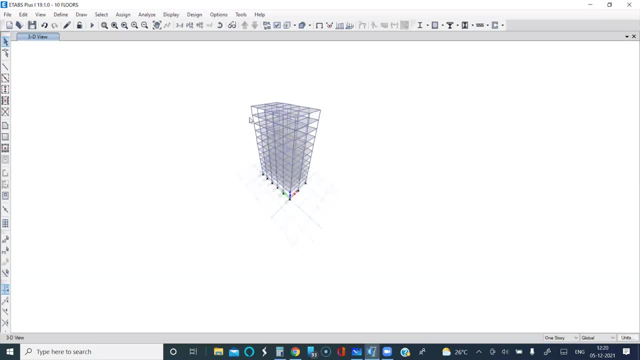 be interested to know more about seismic and all that, But time is limited. Please be with me. Understand At least the modeling part in this. Later you can ask me: Yeah, So now we have done the modeling, You can quickly check for an error. Anything is there or not, So I am going to check if there is. 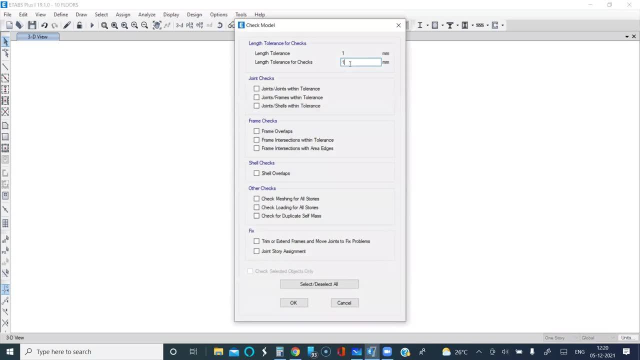 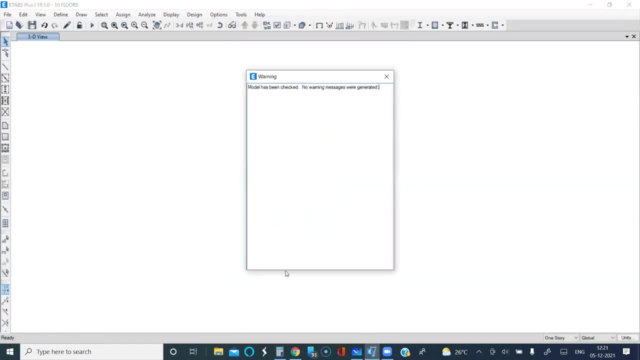 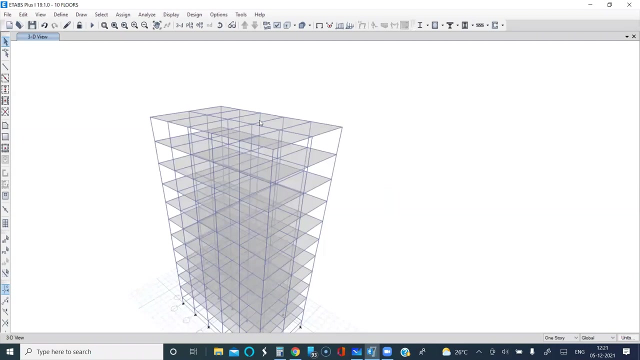 any error Check model. You can keep something like 10 millimeter as a tolerance and then check: Now model has been checked. No warning. Yeah, Sometimes ETAPs will not pick each and every kind of mistakes that you do, Only some kind of geometric. 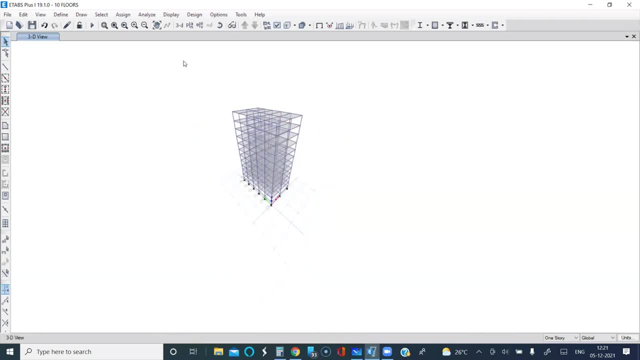 errors it's going to pick, Yeah, But then it's very important to do that check and ensure that there is no problem. Fine, So I am going to quickly analyze this. Run analysis Now. see this kind of simpler buildings. you don't take more than 10-20 minutes in ETAPs to be modeled. 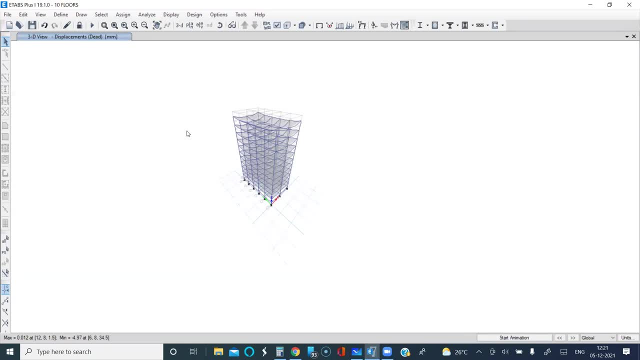 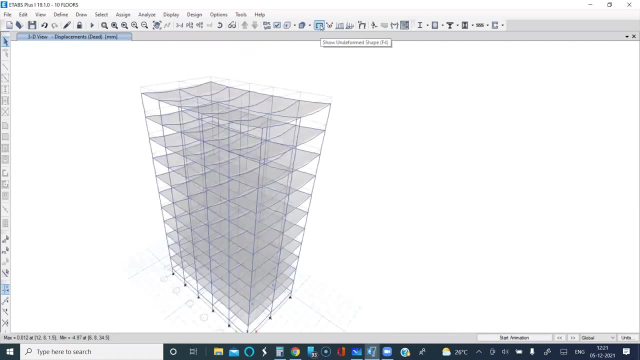 Whereas if you were using any other software, you will be taking a lot of time to model and analyze. It's much simpler and faster, Even if you have shear volts and things like that. Yeah, So your analysis is done right now. Now how do you interpret your results? I will quickly go to one. 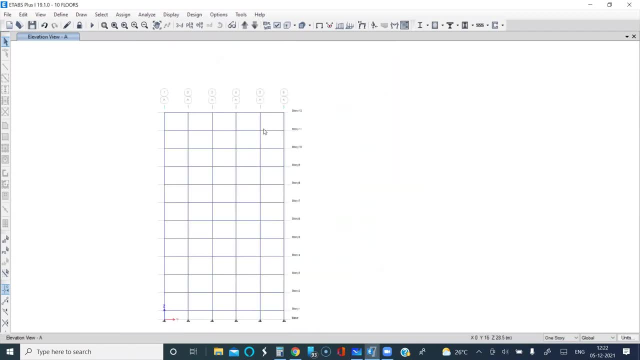 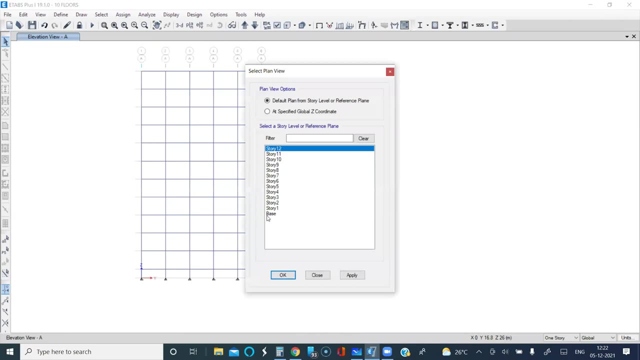 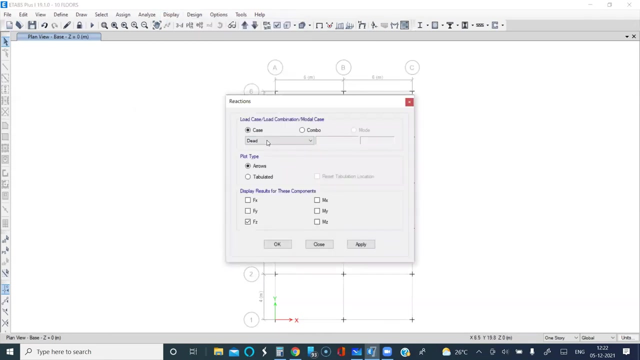 of the elevations. Yeah, And I will show you various result interpretation very quickly, Or I will first go to the plan and show you the reactions. Yeah, You just go to display, or you can go to this button You can take your reactions. 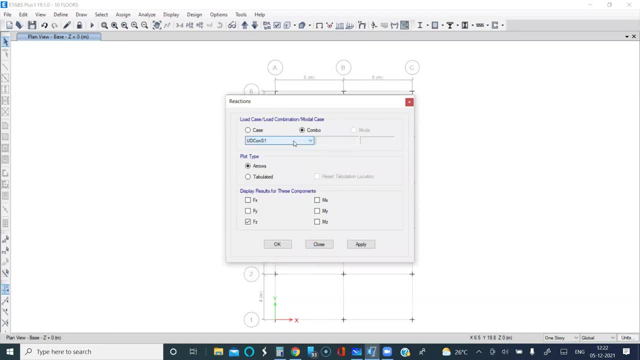 whichever combination you want, Generally, your foundation will be designed for unfactored combinations, So you need to create unfactored combinations also By default. what we have done is factored combinations, Yeah, But you have to create Unfactored combinations also, which I have not shown you. 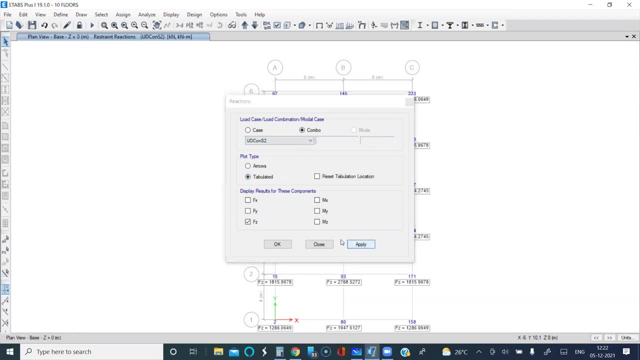 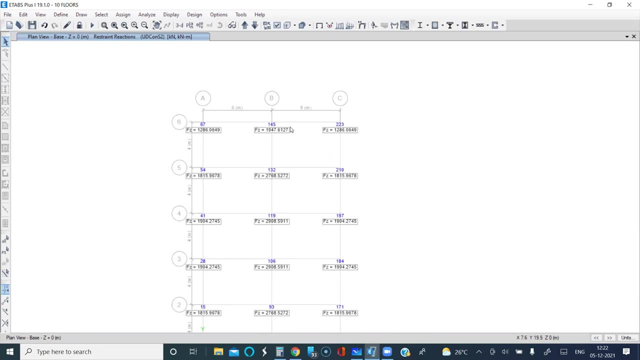 Fine, So if you go here and then make it tabulated, you can see all the reactions. These are factored reactions. It has to be unfactored. Yeah, Simply click this button. Choose your combination. You can display your. 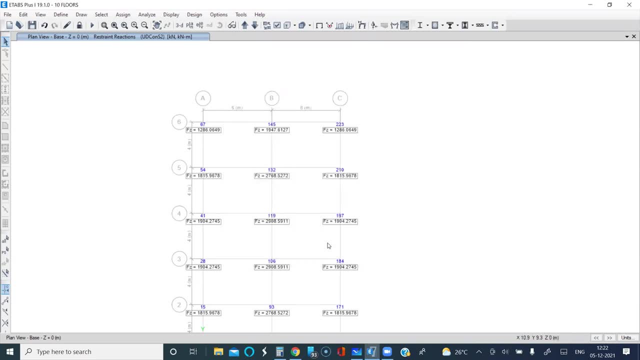 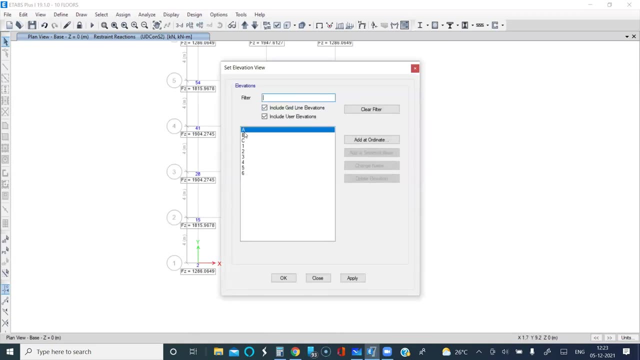 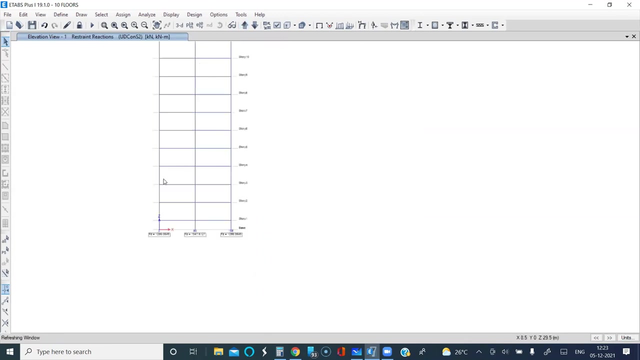 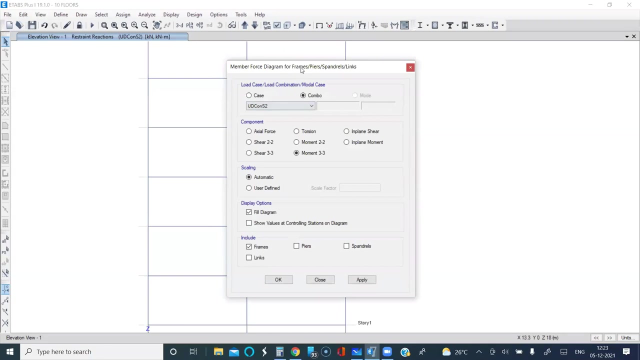 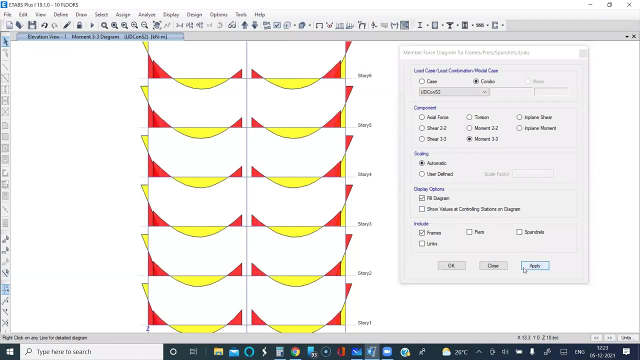 reactions. Now you can size your foundation based on unfactored reactions. Now let me show you how you can do this. So you need to get your rays much more different, All right. So if you go to eBay page, 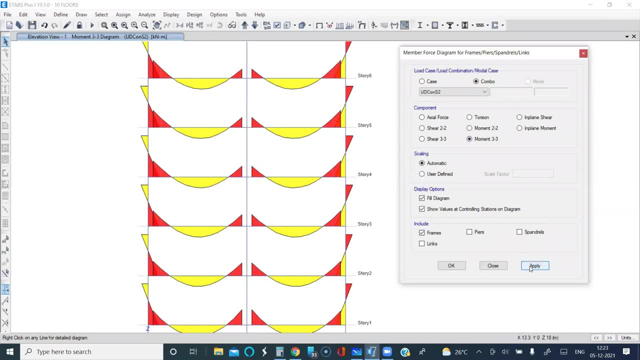 I have made it. Yeah, totally cannot zaar. You can save it doc. audio. Really, Yeah, Woo, Yeah, Yeah, pratic all the video. So let's show. we try this one mounting your movies by selecting f1.. If you go to my videos, 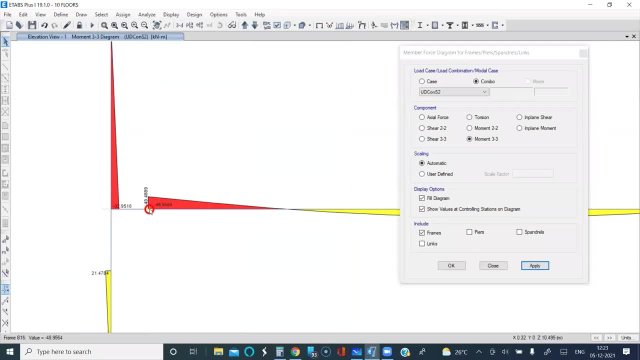 the beauty of ETAPS is see, it is reducing to the face of the column. STAT won't do this. Now, inside the column, say, if your column is very large- 600, yeah, you need not design the beam inside the column, because inside the column your beam is very stiff. It is not a beam, It's. 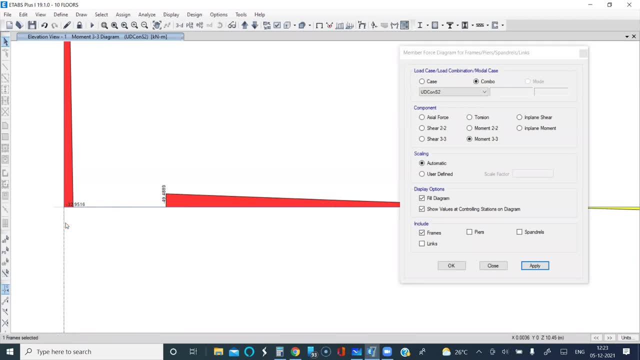 not going to bend. It's a part of the column. In model it is just a stick, But in reality it is a big piece. So your beam inside a column is not going to bend. Yeah, So because of that, ETAPS is automatically reducing it to the face of the column. 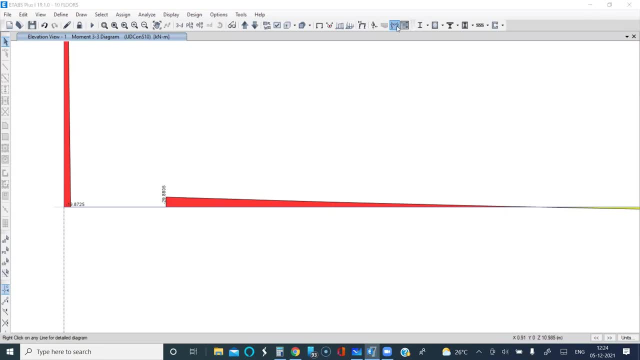 Yeah, So that's a beautiful feature. ETAPS does that, STAT doesn't do that. You can scroll and see various different bending moment. You can also create envelopes. Envelope means every combination together, which I have not shown here anyways. Now, another beauty is that if you click here and right-click, 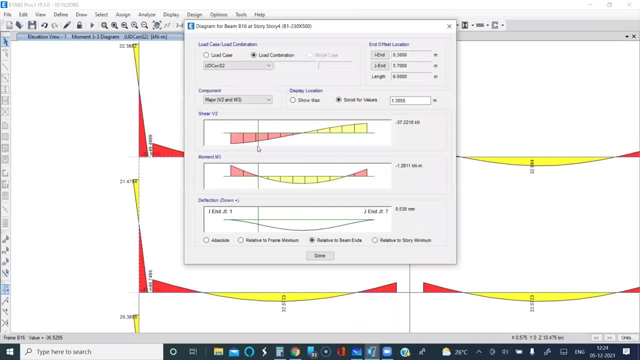 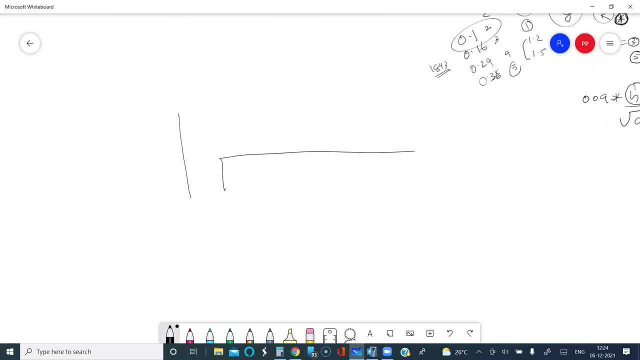 you can scroll and see the point of contra-flexure. Now, if you are detailing beams, you would have seen that the top reinforcement of your beams. you would have seen that the top reinforcement of your beams. if you have a beam like this, 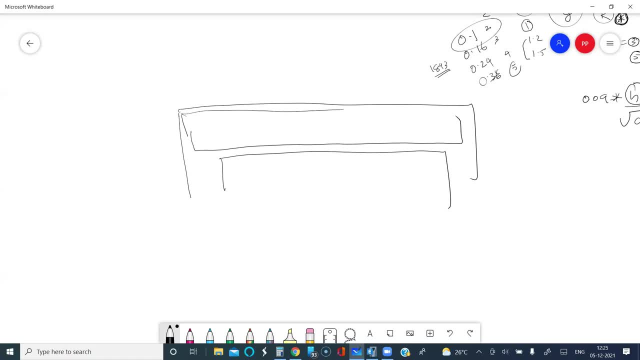 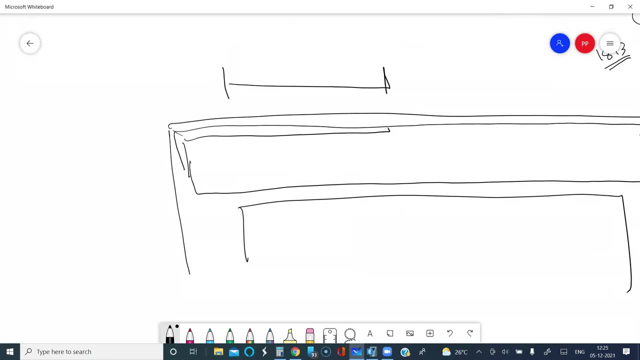 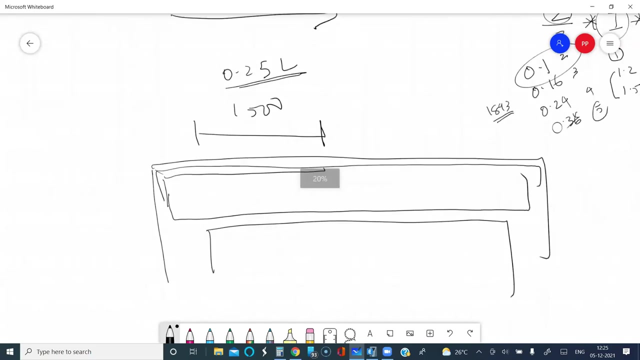 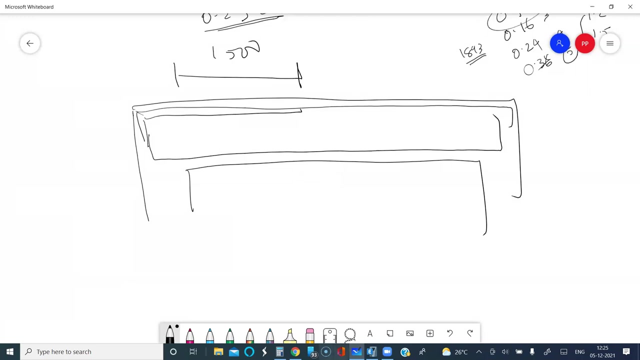 many times you would have seen this detail. Yeah, And this distance would be marked. Generally, this is 0.25 L, which comes from SP34, the second layer. Yeah, But in all the cases it need not be true, So ETAPS, lets you. 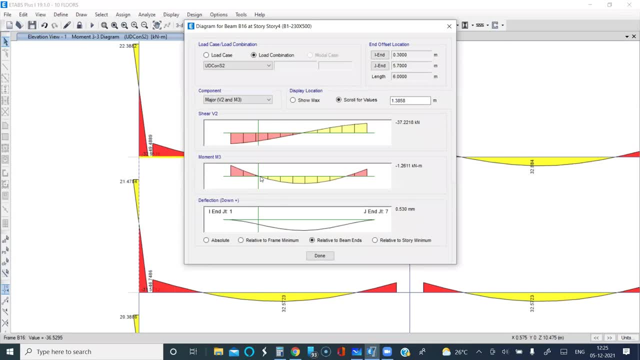 exactly find the point of contra-flexure. So you can see that the top reinforcement of your beams you can find out, especially when you have very huge point loads. If you have read SP34,- how many of you have read that I don't know, But if you have read SP34, it tells you that. 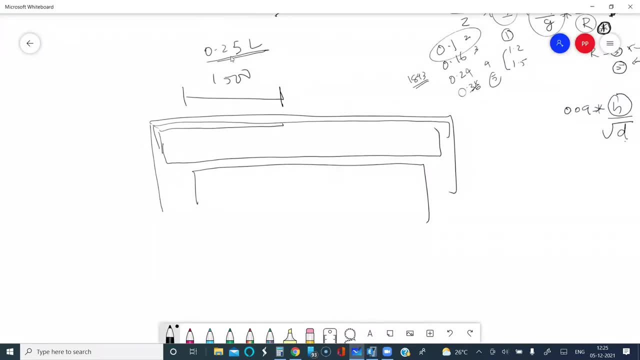 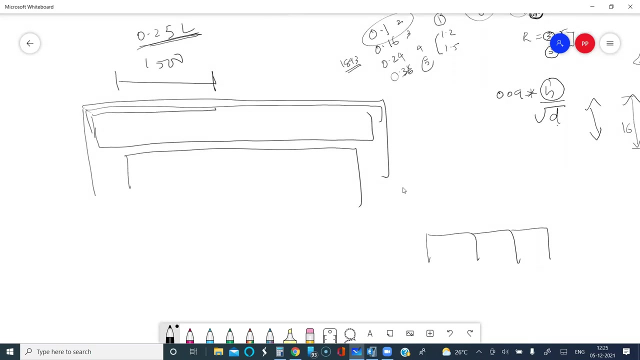 this rule- thumb rule, where you are curtailing 0.25 times L- is valid only if the load is uniform and if the spans are uniform, and if it is multi-span, which means you can use it only if there are three spans minimum. If it is a one span, you cannot use this rule. 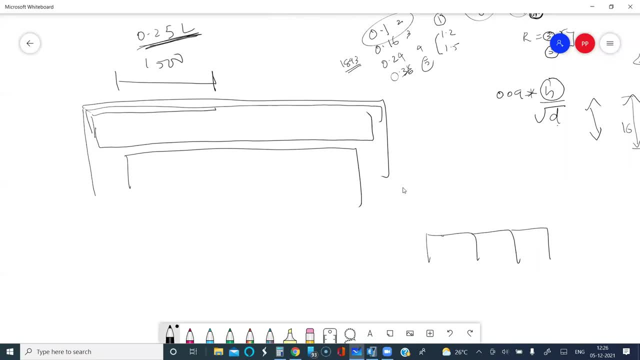 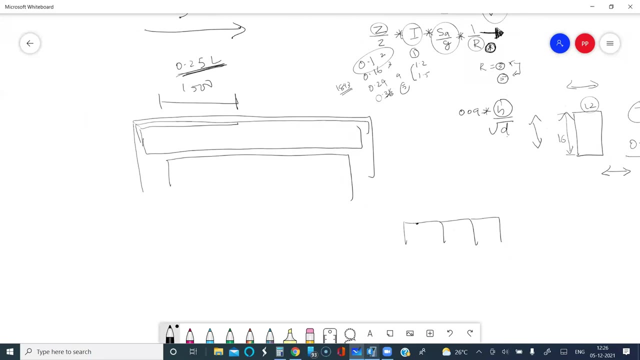 Secondly, if you have a point load that is, a secondary beam entering into this beam, then you can't use this rule. If it is a doubly reinforced section, you cannot use. Yeah, So when you have so much of limitations, when you have a heavily loaded beam, it is required. 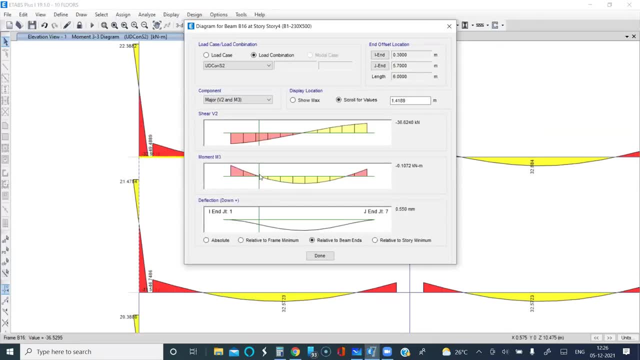 that you use this and understand that point of contra-flexure is within that 0.25 L. If it is far more, then you have to Extend your top bars more than 0.25 L. It's not always 0.25 L. You need to know that. 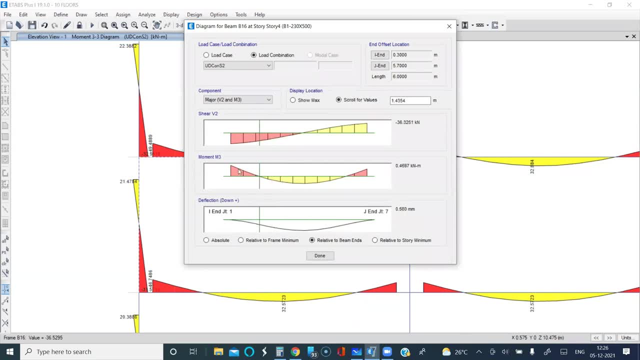 Yeah, So you can use the scroller and decide where- up to where you need the top reinforcement, up to where you need the bottom reinforcement- all that very easily. Now you don't have to do this for all the beams. By experience you will be in a position to decide which beam needs the stick. 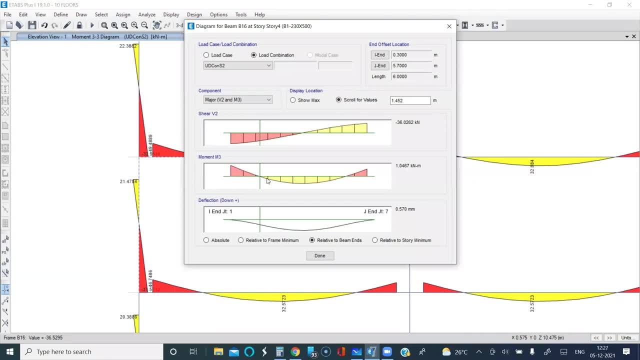 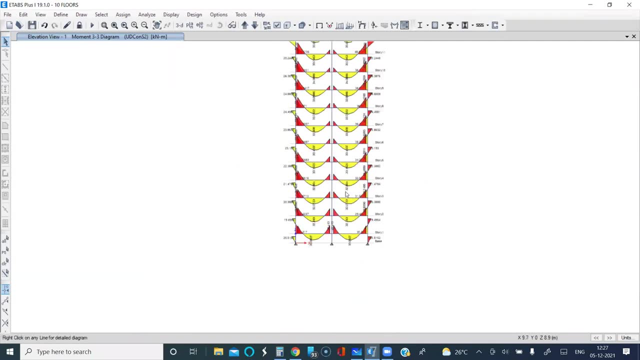 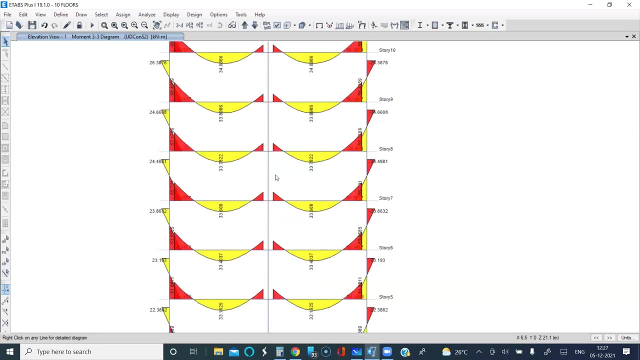 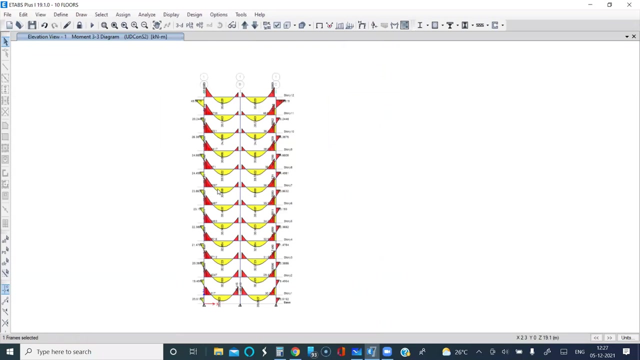 Okay, So that way you need to use this tool. So that's how you have to use this. There are many more things that you have to understand, including load combination. So many things are there which I'm unable to explain in a short span, but then I'm giving you some clues. 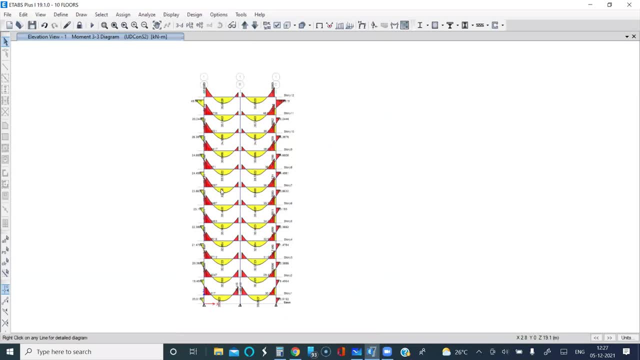 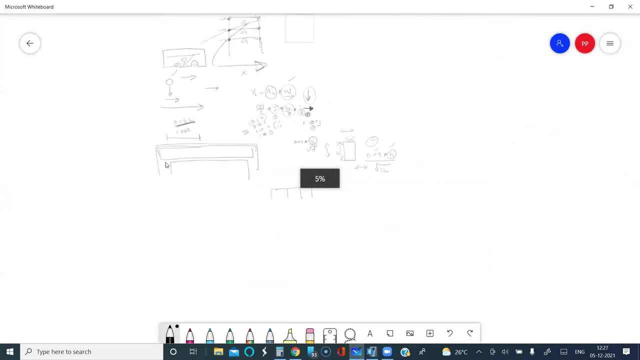 What I will do is I will give you time, in the end, to ask me questions, so that many things can you know, be discussed. Okay, Now design. Design is also a quick step, but I will take you to something else and then come back to design after explaining you something. So 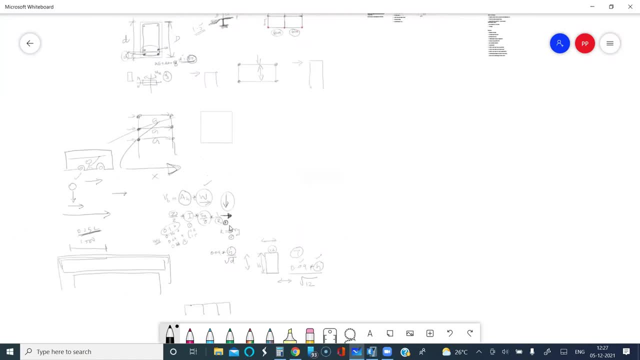 now a quick question to make you think: 0.9 DL plus 1.5 live load plus 1.5 DL plus 1.5.. Or 1.2. Live load plus 1.2 EQ. Do you know that such a combination exists? Is there such? 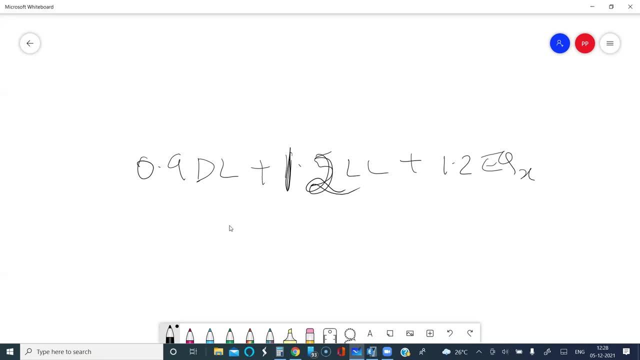 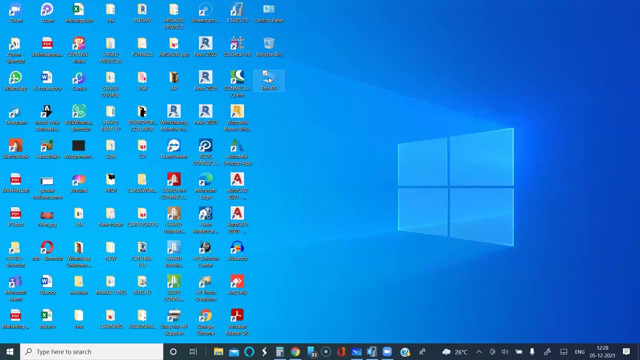 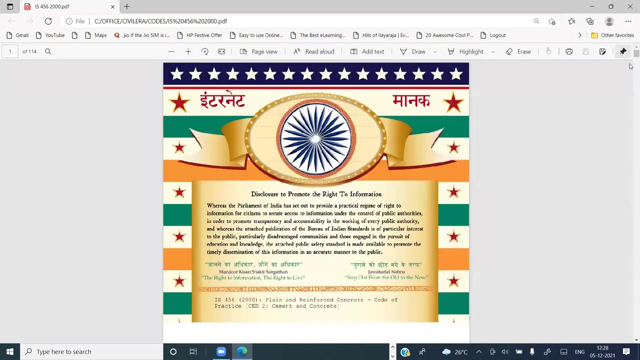 a combination, Yes or no? How many of you know the different load combinations? How many of you know that? load combinations? Okay, I will quickly take you to the load combinations. That is, in IS 456, page number 67, or something like that. Okay, So that's. 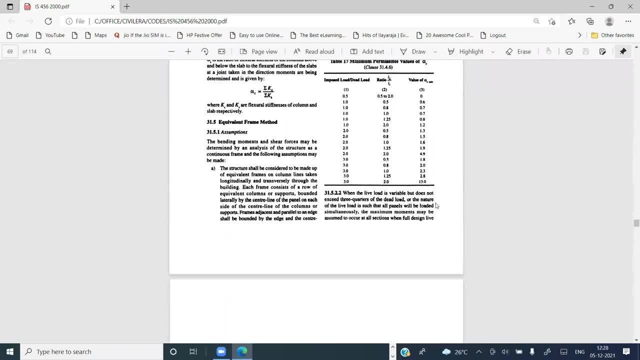 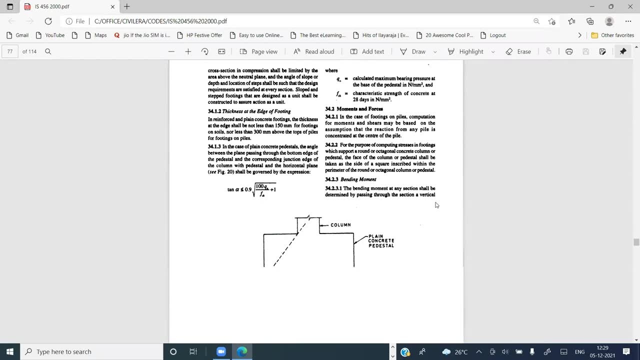 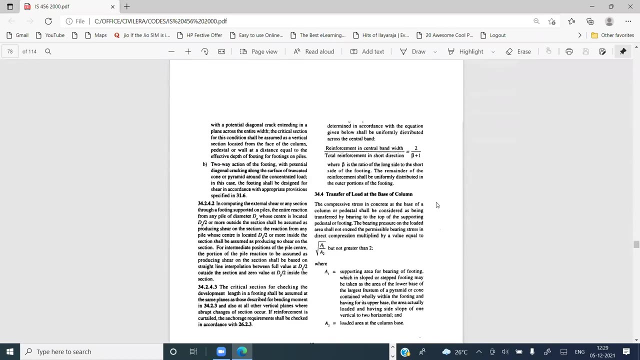 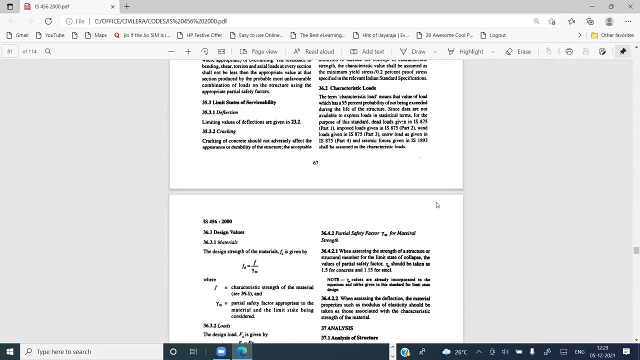 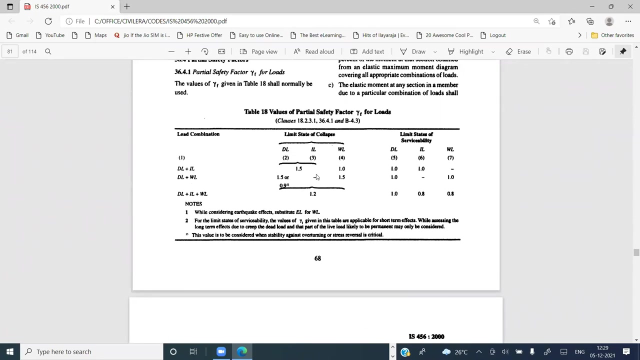 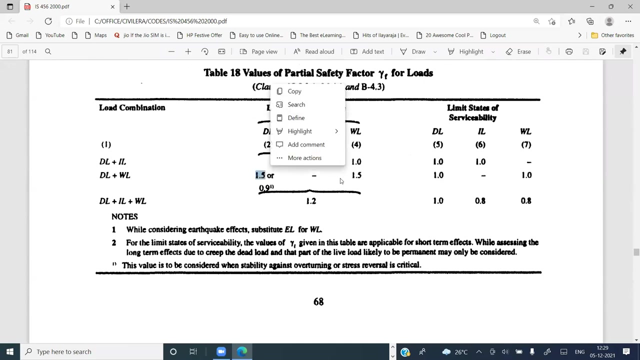 something, Or 68.. Why do you need load combinations? All these are some questions that you may have, but then everything cannot be answered in a short time. Yeah, So here you have the load combinations. If you see, here my question is on this: Dead load plus live load, 1.5 DL plus 1.5 wind load. 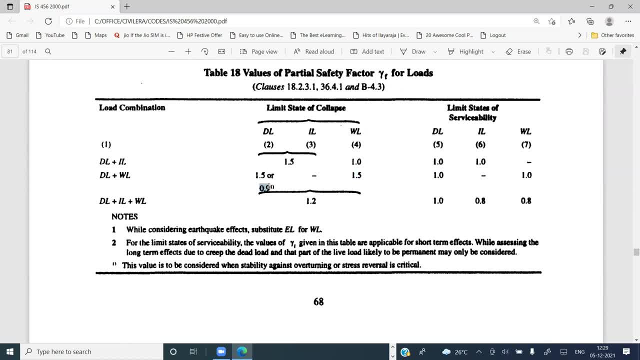 That's one combination. Another combination is 0.9 DL plus 1.5 wind load or earthquake, whatever, Yeah. So why do you need 0.9 when you already have 1.5, which is more than 0.9?? 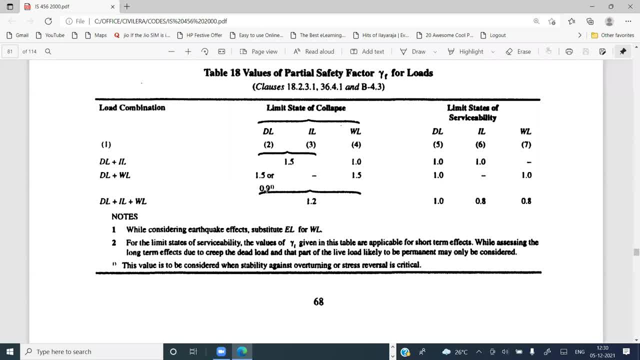 Why do you need 0.9 DL plus 1.5 wind load also? Yeah, So think about that. The answer is here in the notes. Yeah, But if you don't understand, you can get back to me. Yeah. 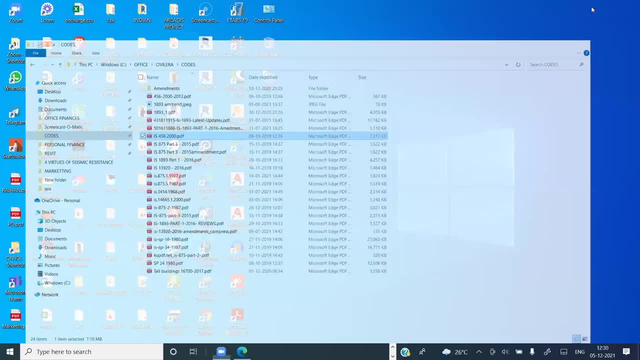 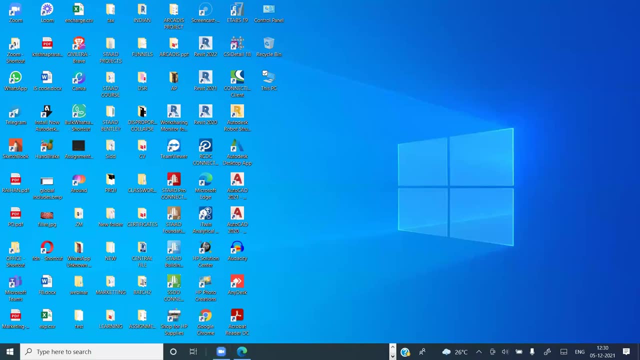 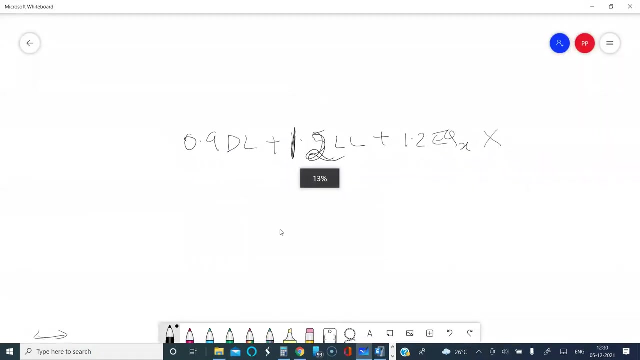 So there are many things like that which will help you to fine-tune your understanding and design. So please ensure you understand all this. Read all the notes in your notes. Remember code. Don't just focus on only modeling or only combination. Okay, I know. 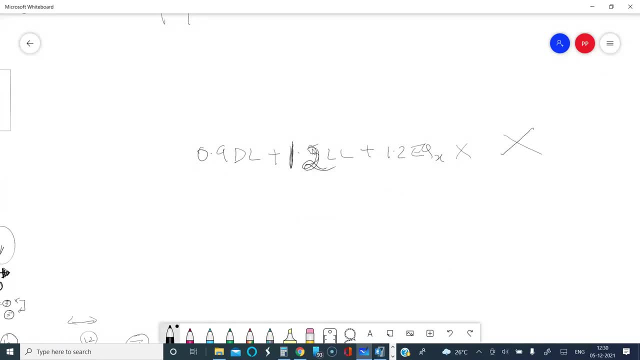 the combination, but why? Yeah, This combination doesn't exist. 0.9 DL plus 1.5 EQX exists, But why do you need it when you have this? That's my question. Let me know. if somebody has the answer, You can message me. One bonus for the right answer. 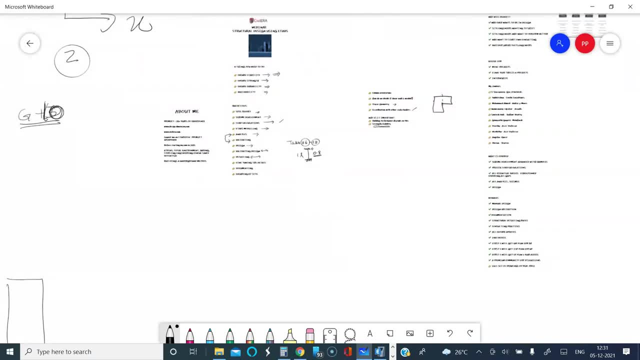 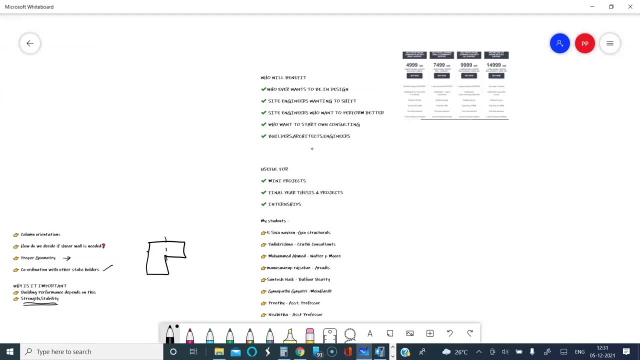 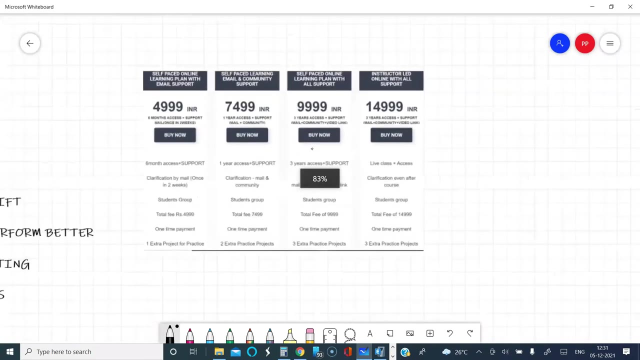 Okay, Now, let me quickly tell you something about one of the course that I'm offering. After that, I will come back to the design and take your questions as well. Okay, Now, if you are keen to learn the entire design in a consulting way, the way that I do, 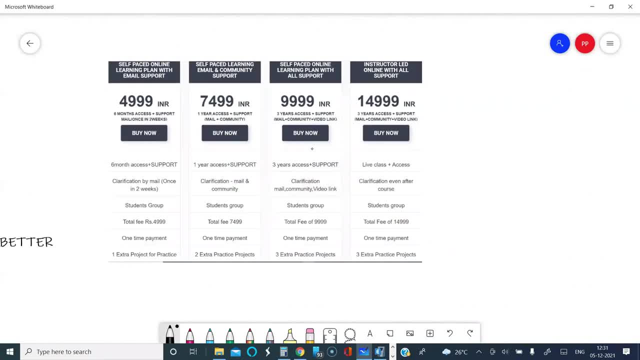 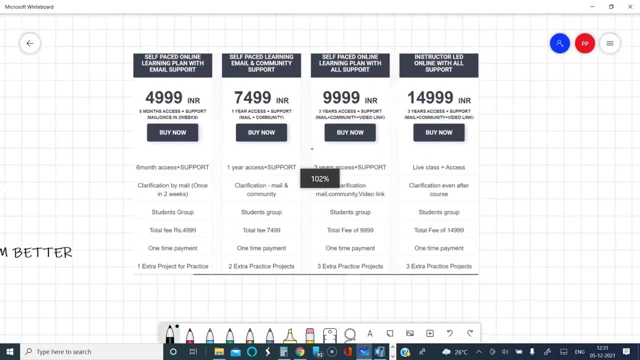 in my office. I do have a plan, a premium plan on training, which I'm offering you in this webinar for a reduced price. Okay, So stay. I'm going to explain you about the plans. This is a complete live plan, which 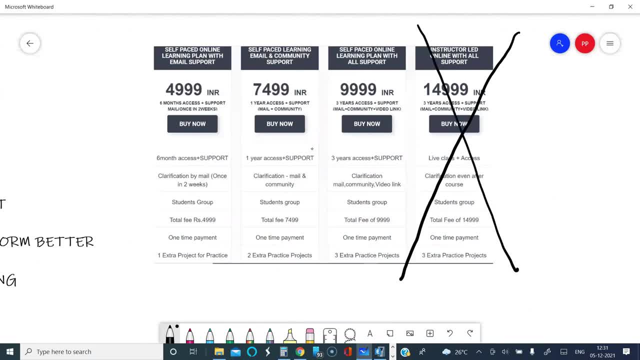 is not there right now because of the pandemic. We are not running the direct classes, but online live will be there, but that will start somewhere in February. the next batch: Now these three plans are available Now. in all the three plans you have the same content. 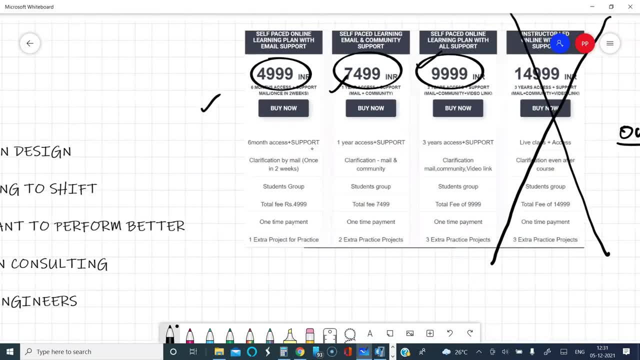 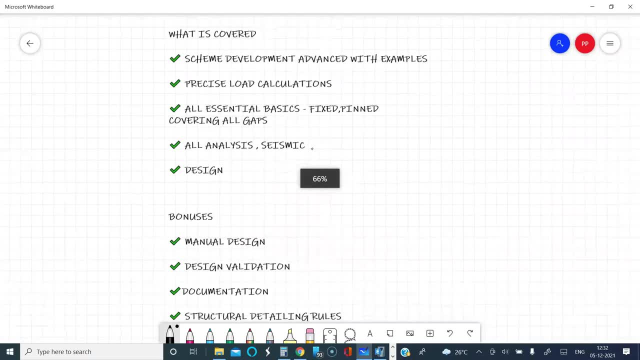 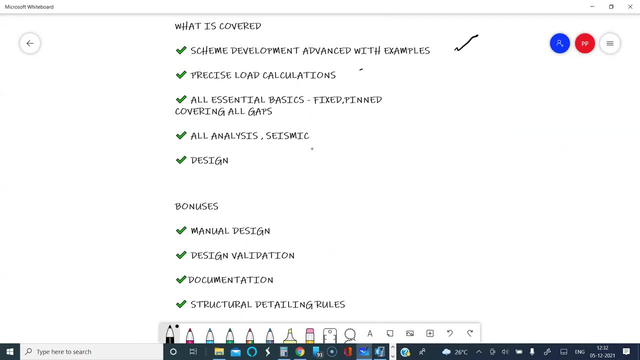 Yeah, And what will be that content? It will contain the entire scheme development. It will have all the advanced things, with examples. It will have precise load calculations. It will have all essential basics, like fixed pinned covering all the gaps, the load combinations that I'm talking about. 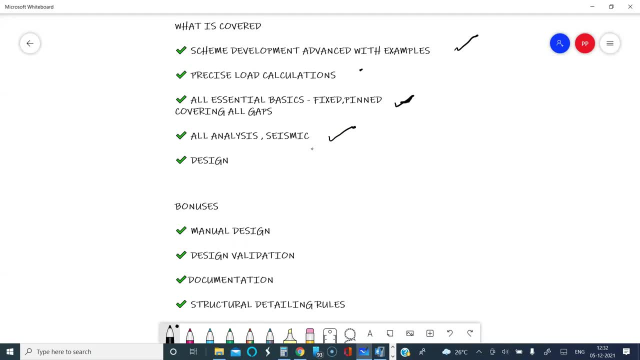 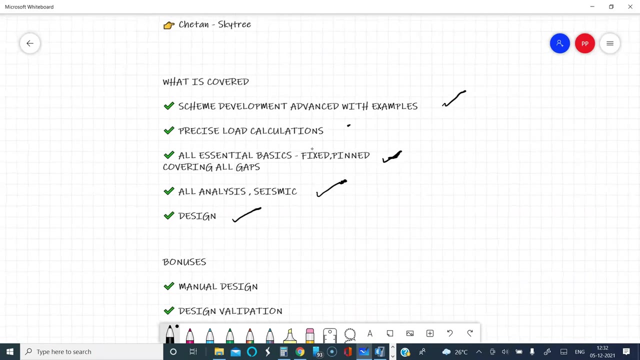 all the analysis, seismic analysis, all the points, diaphragm, action, what it means, stiffness, modifications, everything. It will cover all the design. It will cover all the manual design and it will be a complete thing, from scheming onwards to detailing The way that I do in my office will be covered in this. 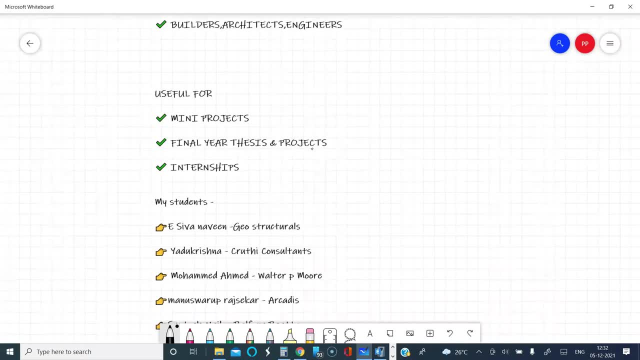 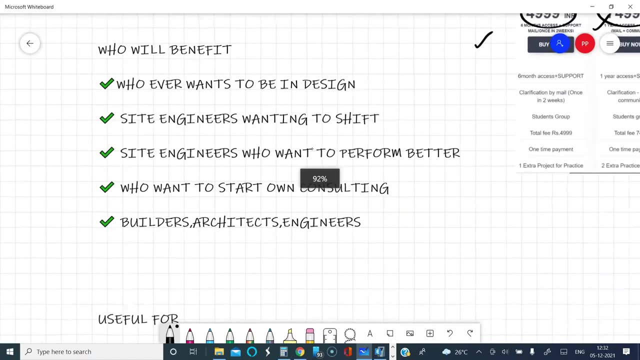 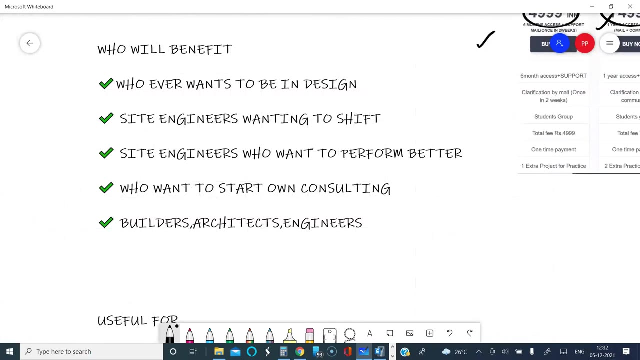 And who will be benefited? It will be benefited to all people who want to start design. Yeah, It could be site engineers. It could be design engineers with some experience. It could be site engineers who want to perform better. Yeah, Even site engineering needs understanding of structures. 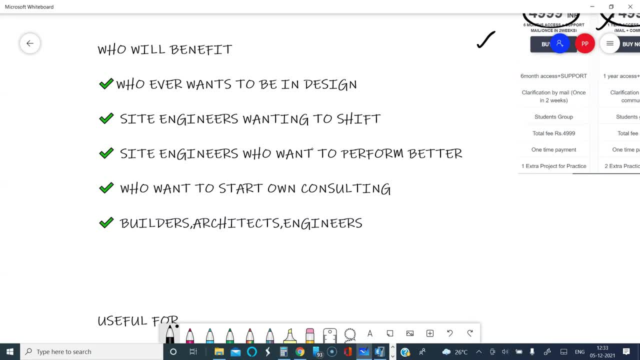 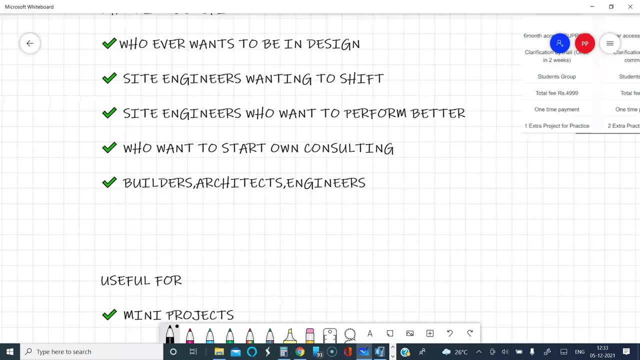 Yeah, Who wants to start consulting on your own? Who wants, say, who are builders and want to start designing in-house? It will be beneficial for all these categories. I'll be hand-helding and guiding you with this. It's not that you will get only the access. You will also have a community. 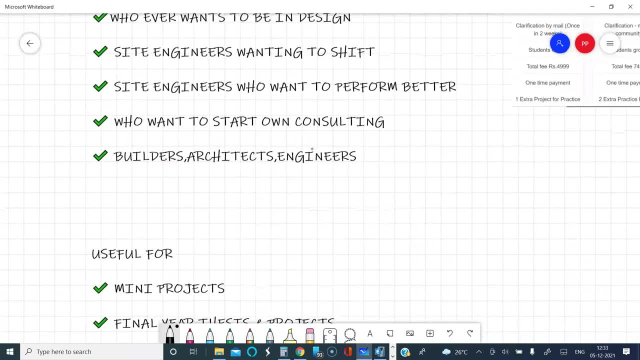 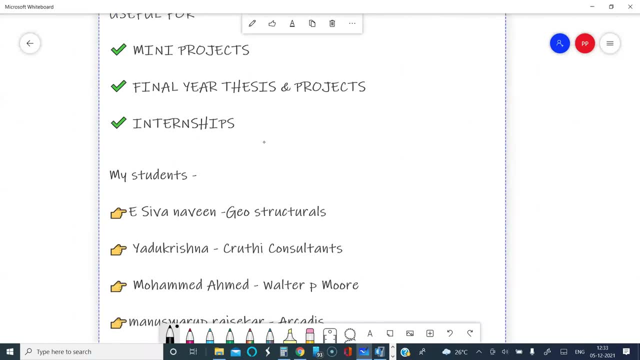 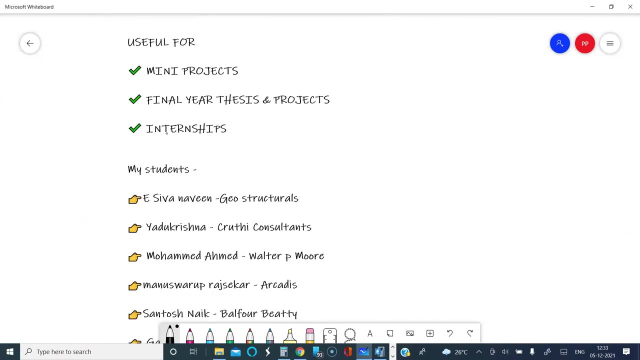 where you can engage with me. You will have a premium community, not like the WhatsApp group. It'll be a better one. It'll be also useful for many projects in your final year or your pre-final year things- internships. It will satisfy all these requirements of final year thesis and projects. 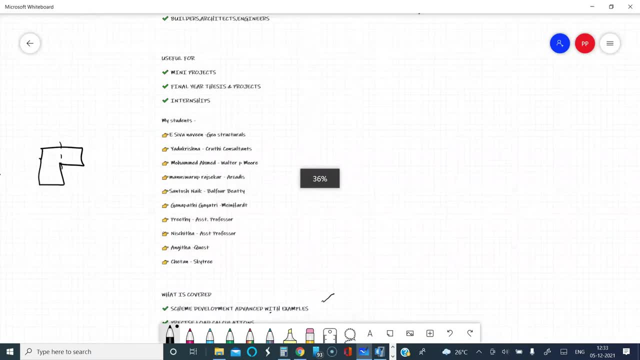 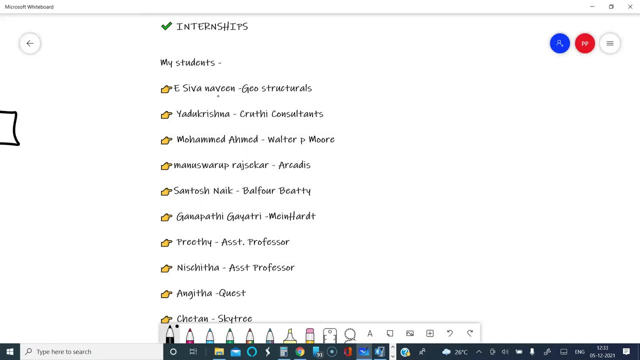 internships and all that. Okay, And I will also just introduce you to some of my students who are on LinkedIn. You can see their profile. If you want, you can speak to them as well to understand better, rather than me telling about this. So you can see, Shiva Navin is one of our. 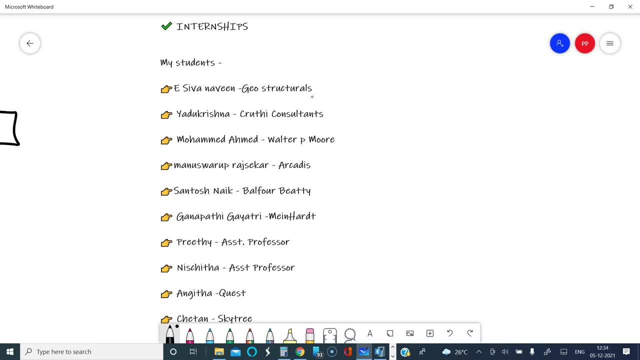 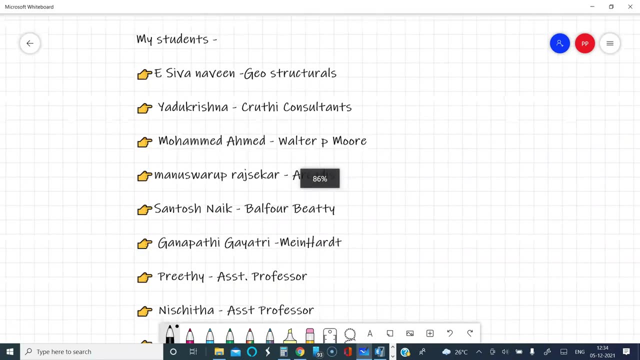 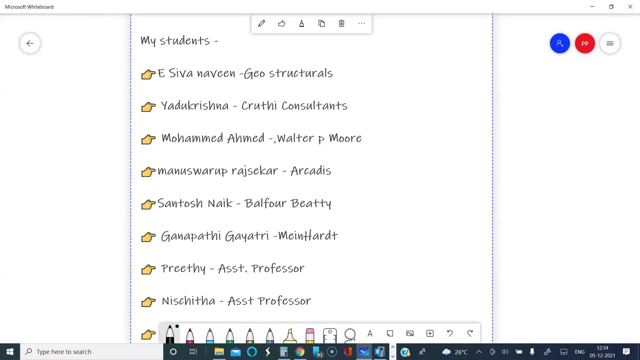 high-performing students who works as a team leader in geostructurals, And you have Yadu Krishna, who is working in Kruti Consultants in Bangalore, And Mohammed Ahmad is a very, very active guy. If you want any kind of guidance, he will be happy to help you. He works in Waterpey Murali and he's 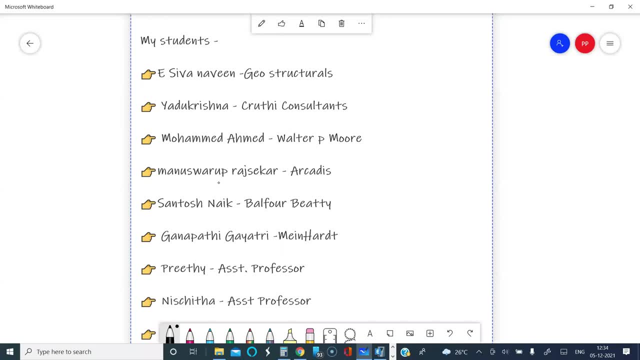 in Pune. He's very active in LinkedIn. Same case with Santosh Naik. He's also a team leader in Balfour Betty. Anybody here? I'll let you know, I'll let you know, I'll let you know, I'll let you. 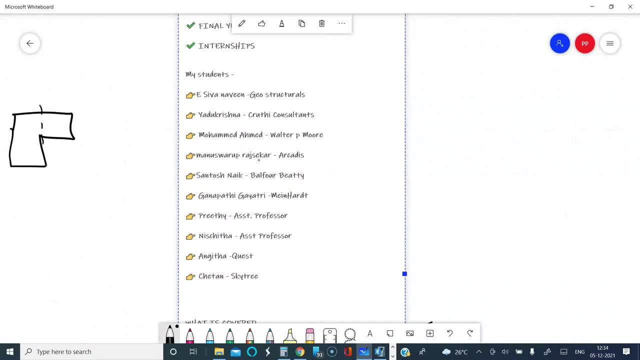 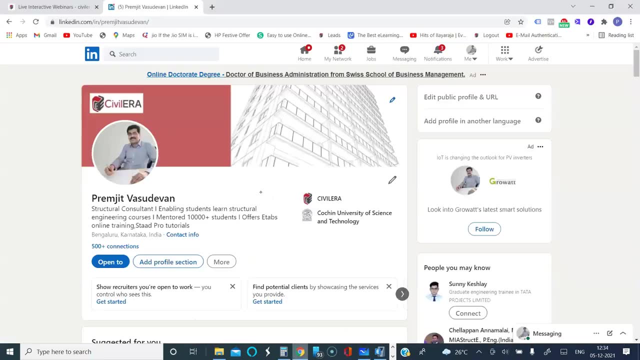 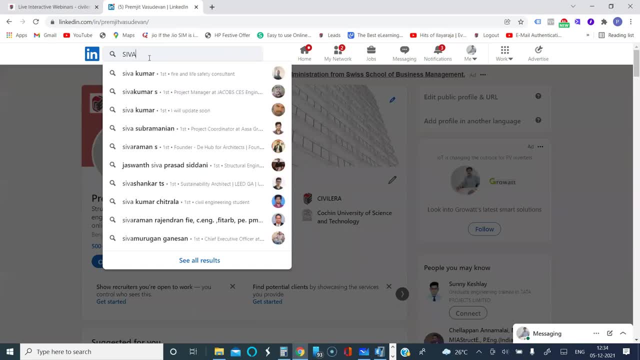 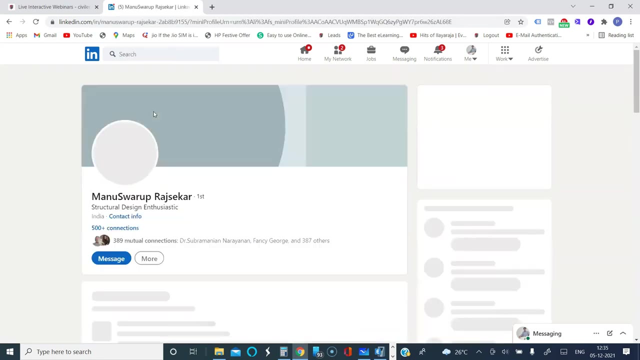 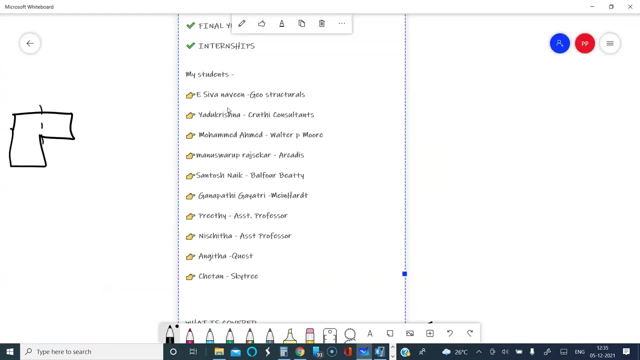 Not Google. You can check in your LinkedIn and they will be there. Most of them are there in the LinkedIn. So this is Manu. He works for Arcadis and he's a structural engineer there. Like that, you can find them and then discuss with them about their career advancement and their various 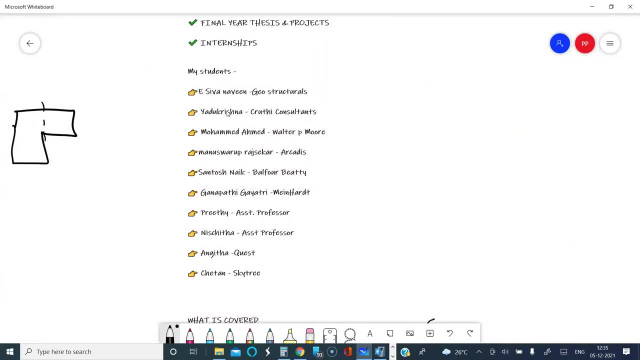 methods that they adopted to land a job. I can guide you as well, But then, hearing from the students directly, you can understand their way of approach for jobs and all that. So you can take a screenshot as well and then find them on LinkedIn. if you are keen to do that, Then you will also have some bonuses if you are. 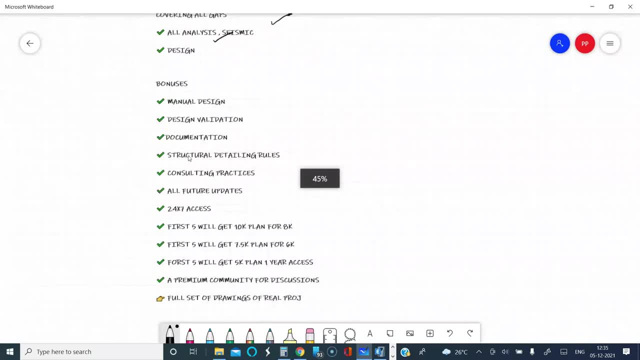 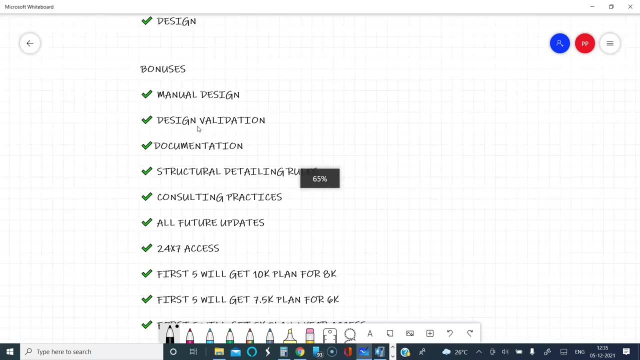 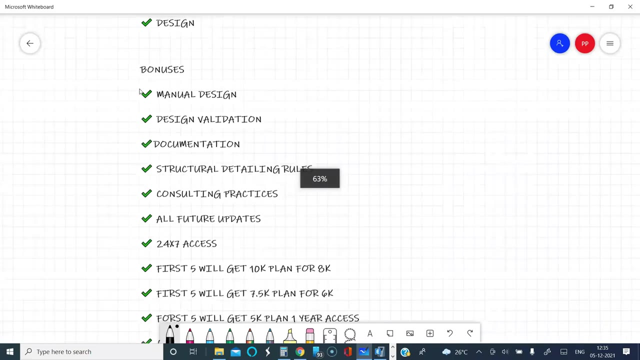 taking it right now, after this webinar, The main bonuses will be: manual design: I'll be handing over a set of drawings to you of a real project, and a model as well. You will be learning design validation: You will be design documentation: You will be learning. I'll be. 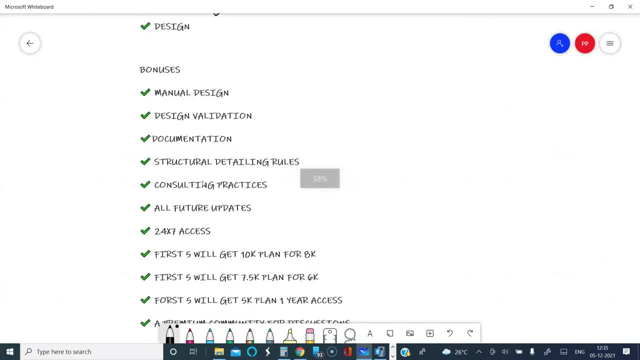 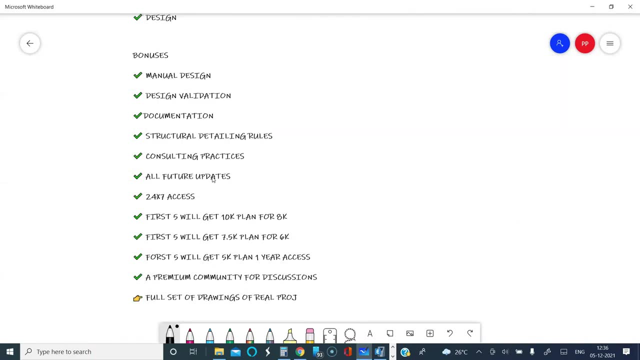 showing you. if you are waiting, I will show you how I document Then structural drawing and detailing rules. I'll be covering All the consulting practices I'll be covering. You will have all future updates for the course. You will have 24 bar 7 access as well for the entire content that. 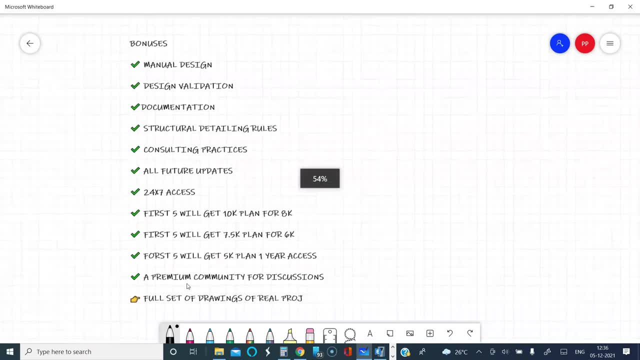 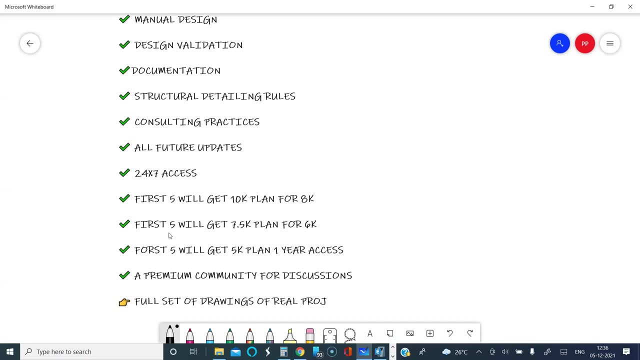 I'm going to share with you Now. the first five who are booking this 10,000 plan are going to get it for 8,000.. The first five who are booking also will get the 7,500 plan for 6,000.. And for the first five, 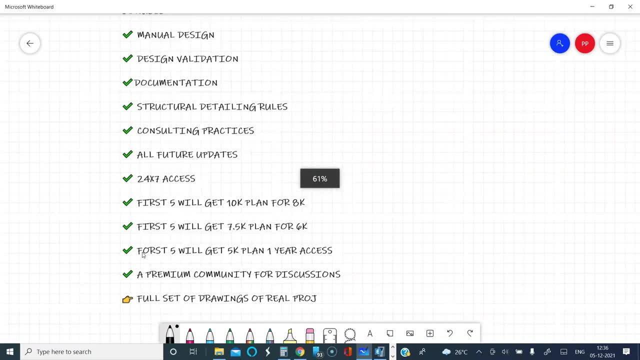 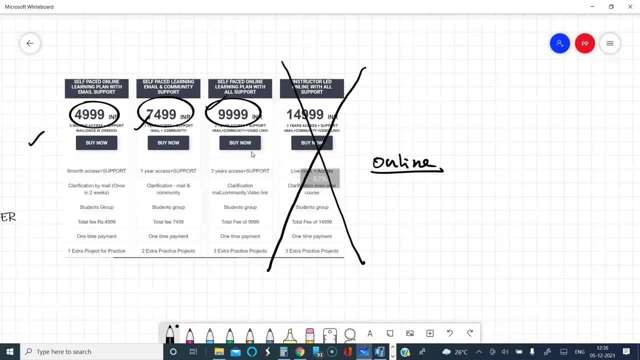 I'll give the 5,000 plan for one year access. So, coming back to the plans, In 10,000 plan you are going to get three years of access and my support. I'll be hand-helding you and encouraging you to learn. Your doubts are going to be clarified in a 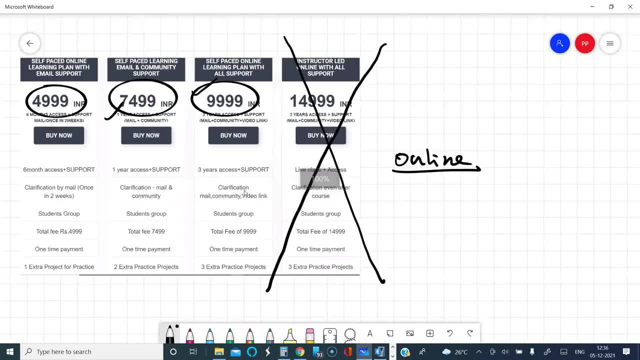 community. in a premium community, You will have clarification by mail, community and video link. Occasionally I'm happy to call you as well And you will get a student's group And you will get three projects for practice. So this 9,000 or 10,000 plan is what you are going to get for 8,000 if you are booking it. 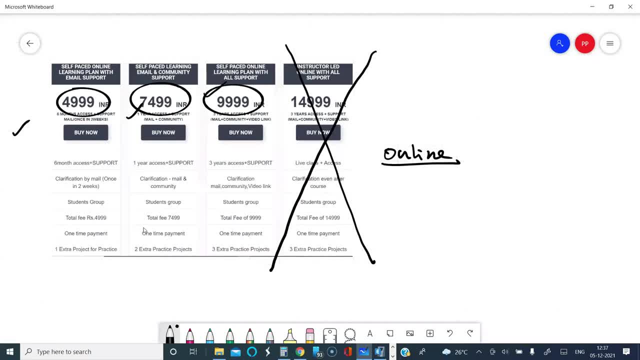 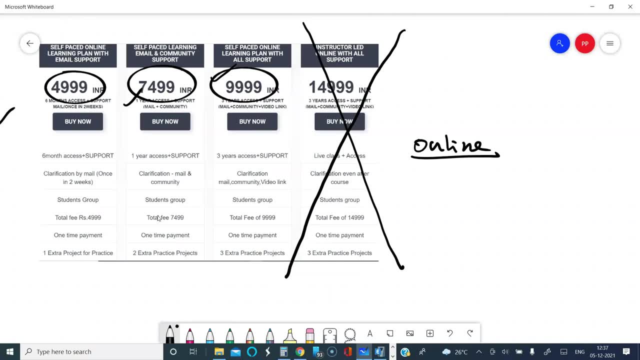 First five only I can give you And this plan for 6,000.. That is one year. access Clarification by mail and in community. You will get a student's group And there will be two extra projects for this. So you will have 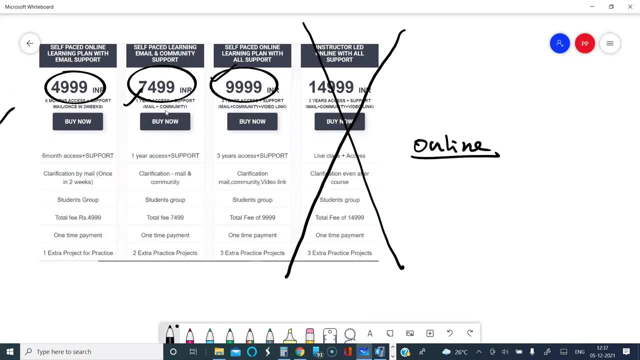 one-year access. Yeah, And the 5,000 plan will remain as it is. I will increase the access to one year, So you will have one-year access and you will have one extra project and you will have only email clarification in this particular plan. So you can choose. But then the advantage is that 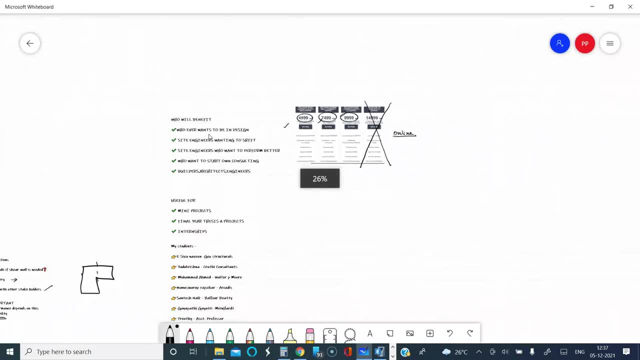 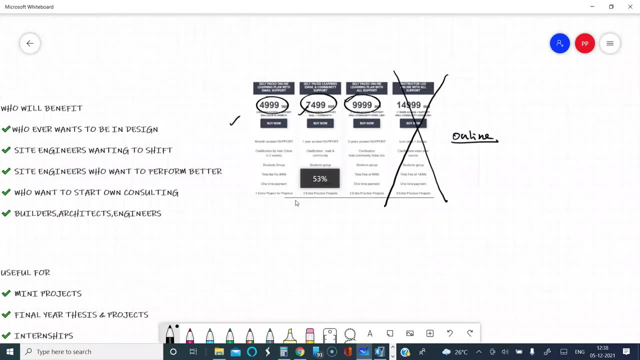 you get a lot of bonuses if you are booking it very soon, And you will get a lot of bonuses if you are booking it very soon. So you get a premium community where I'm going to engage with you for your clarifications That I will hand it out even to 5,000 plan. I have mentioned only email. 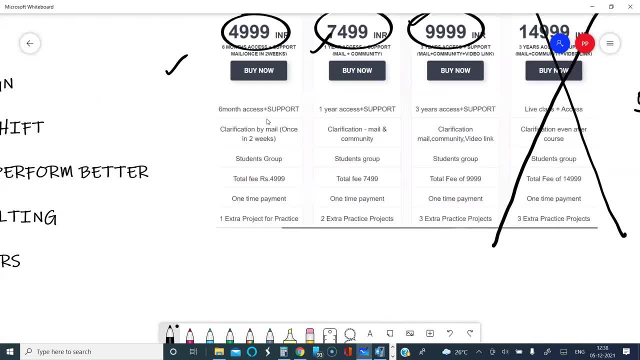 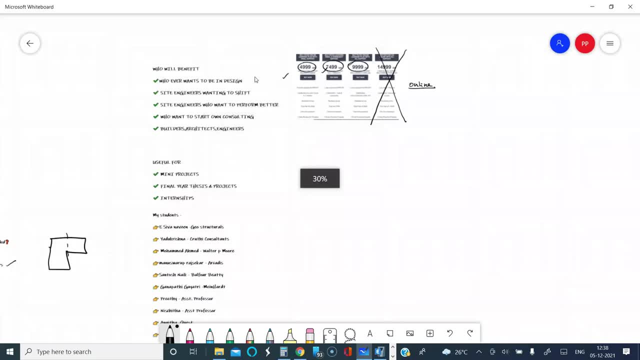 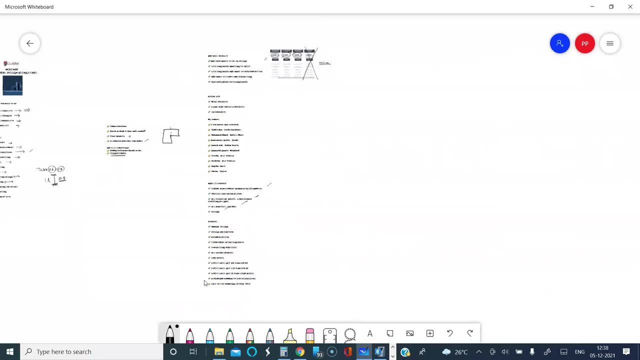 here, But then you will also get a premium community where you can engage and discuss with me- All that will be in your login for who are joining after this webinar. Okay, So those who are really interested, please message me after this webinar directly on my WhatsApp. You will get. 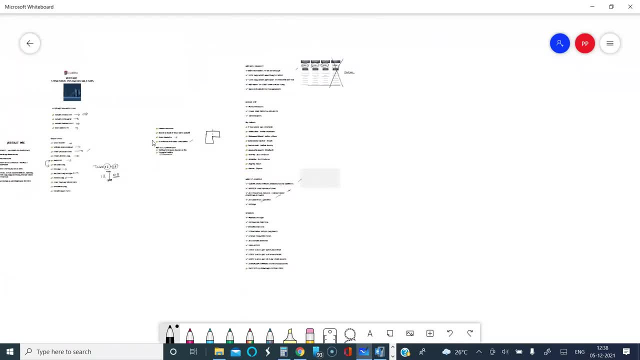 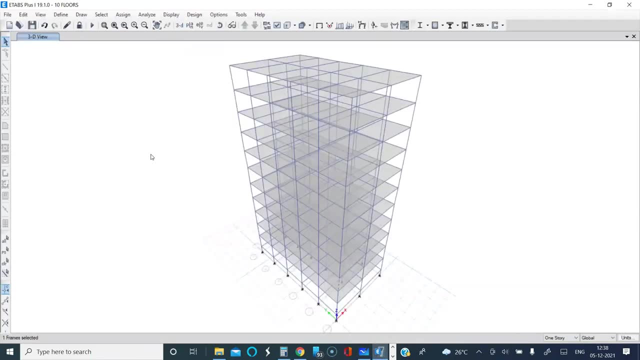 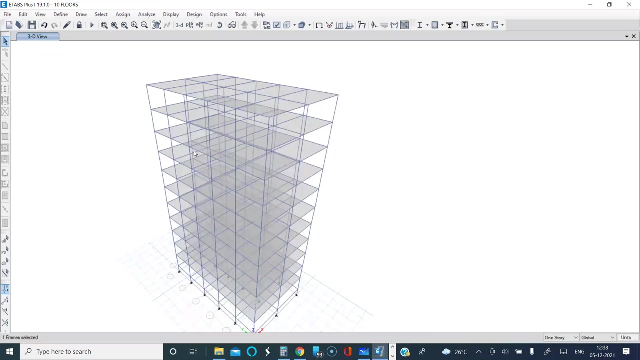 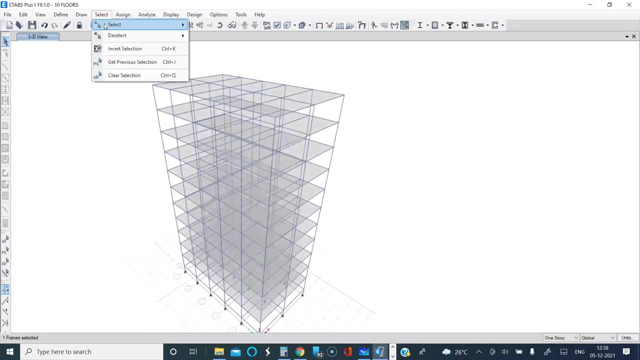 the bonuses, So you will get the benefits that I explained. Now, coming back to design, it's very easy to design in A-Tabs, It's not a big deal, But I encourage you to understand the design principles manually and ensure that you are able to validate what you are doing in A-Tabs. Yeah, So let us select. 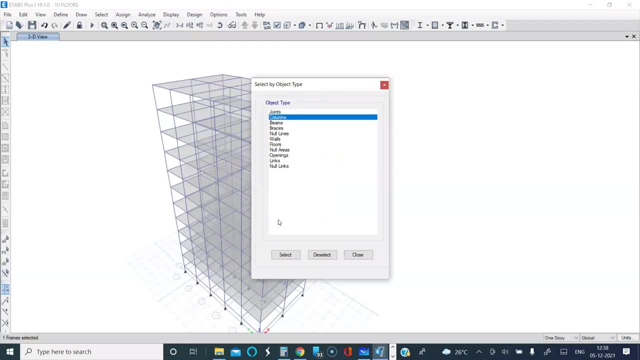 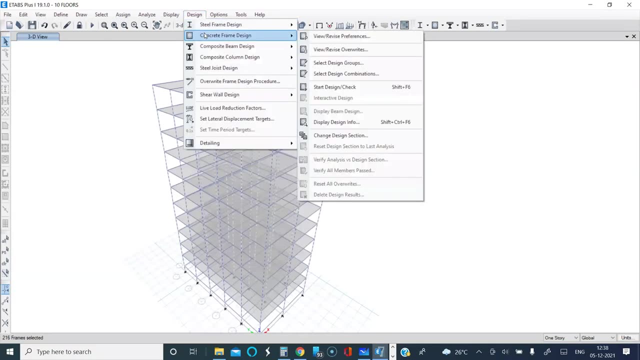 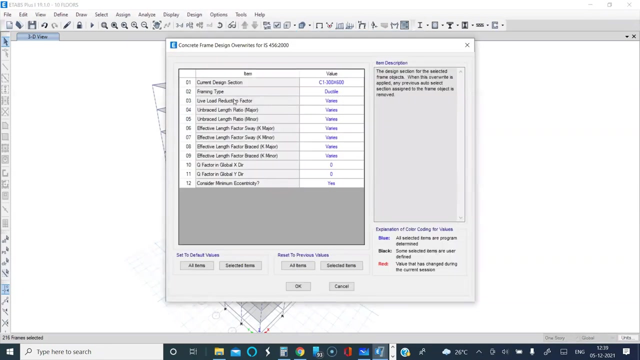 select object type columns. So I'm choosing the columns here for design- right now Only columns- And then go to design concrete frame design And come to overrides. Now, this is a very important part which many engineers, even experienced, do compromise or do something without their 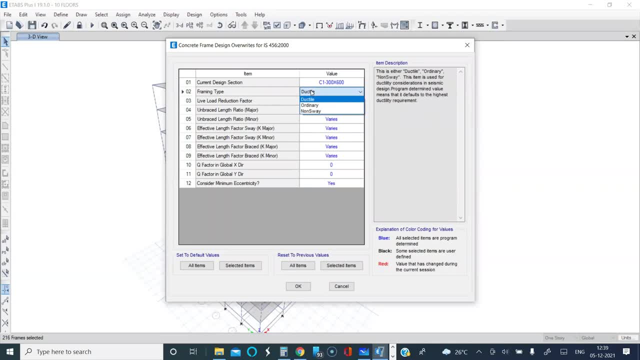 knowledge. Okay, So here there are three options: Ductile, ordinary and non-sway. So it's very easy to decide between ductile and ordinary. Very clear: If you click ductile, it will do ductile detailing, which is needed for zone 3 and above. 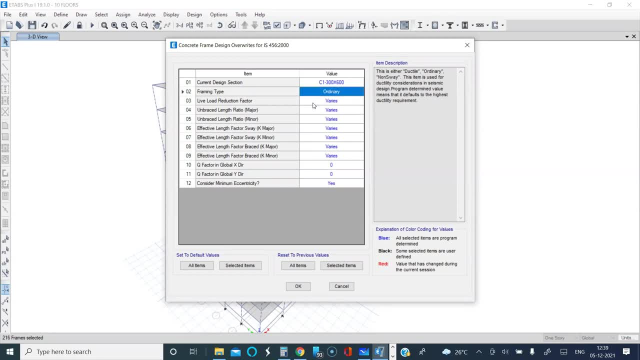 Which is a special detailing. When you do ordinary, it's an ordinary detailing. it will perform which is needed for zone 2 buildings. That's very clear. But many simply hop to non-sway, saying that the steel is drastically less when it is non-sway. But many people don't understand. 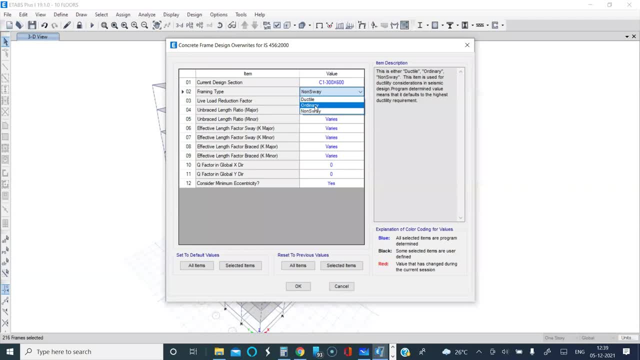 or appreciate what is non-sway and what is ordinary. Yeah, So it's very important. In my opinion, you should never use non-sway, It should be only ordinary. Now, the difference is, if you choose non-sway, ETABS don't calculate the sway index. Now, what do you? 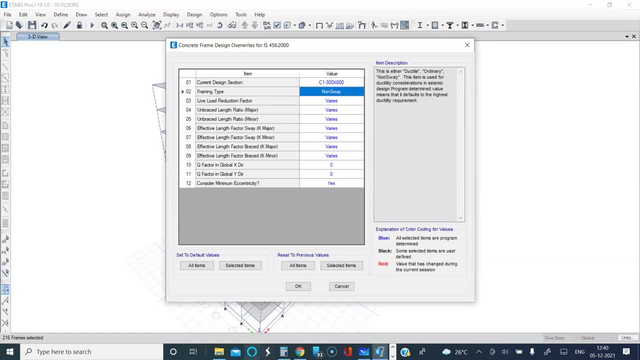 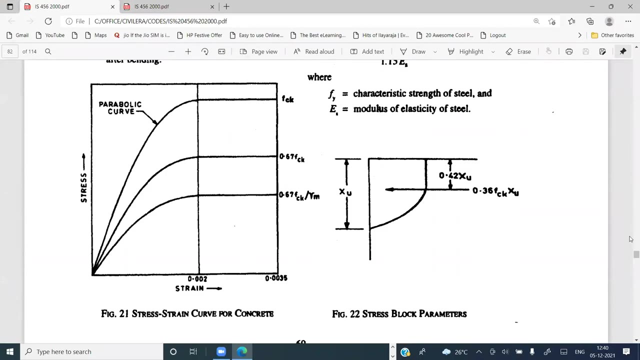 mean by that Your effective length, If you remember effective length, If you know about it. some of you, at least, are intermediate, So you may be knowing about the effective length factor for the column. Yeah, So I can quickly show you in the code If you go to table 26 or 28,. 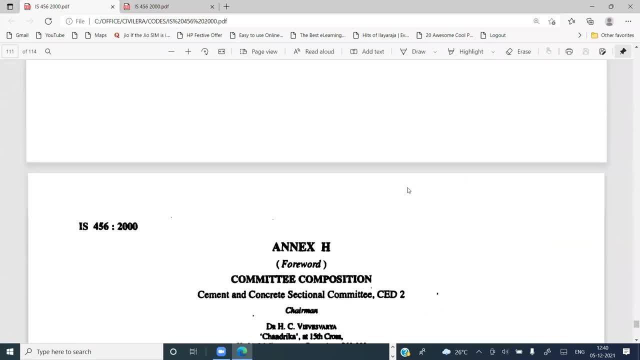 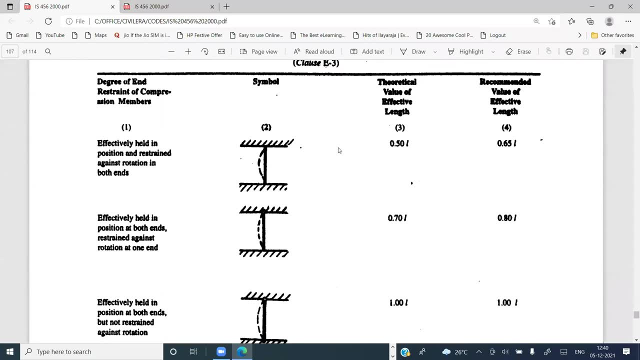 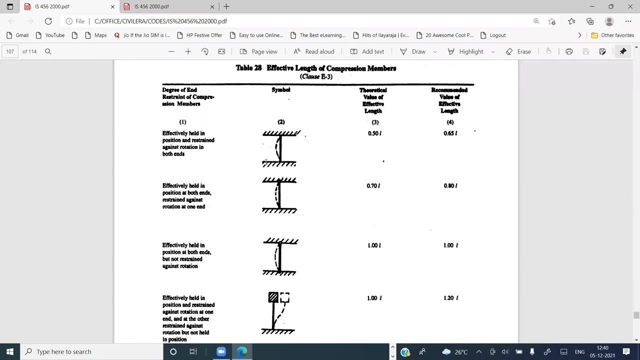 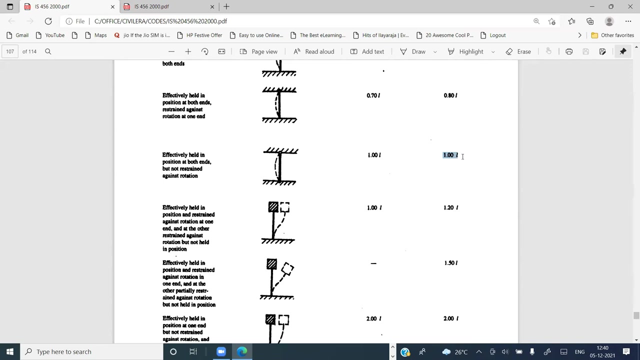 consultants, even experienced consultants, go with that table 26 for calculating effective length, This table Table 28.. Yeah, And most of the people go with this fixed condition or pin condition and then say my effective length is 1.. Effective length factor is 1.. And then in ETABS you start. 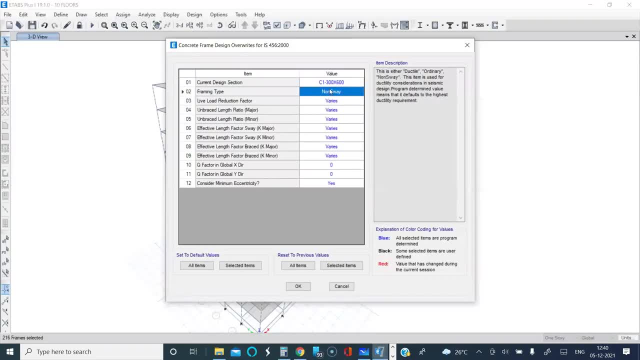 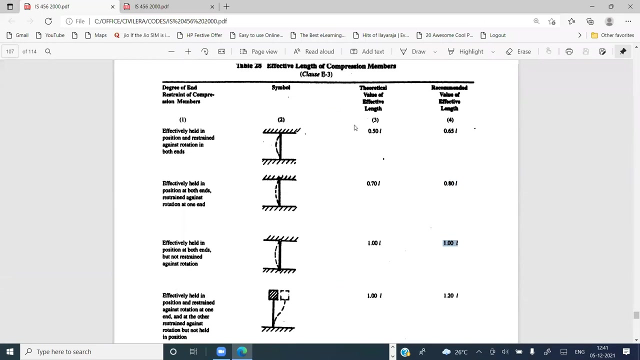 taking non-sway and then you start giving that value here as 0.8 and all that, which is not really right. You have to always choose this as at least ordinary if you are not doing ductile detailing. The reason is: Give me a minute, Where is my? Yeah? The reason is that this table 28 is useful. 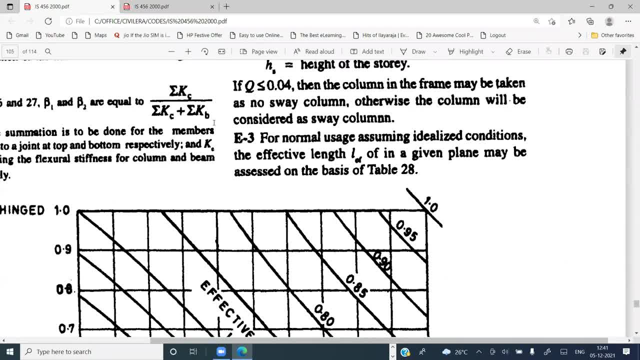 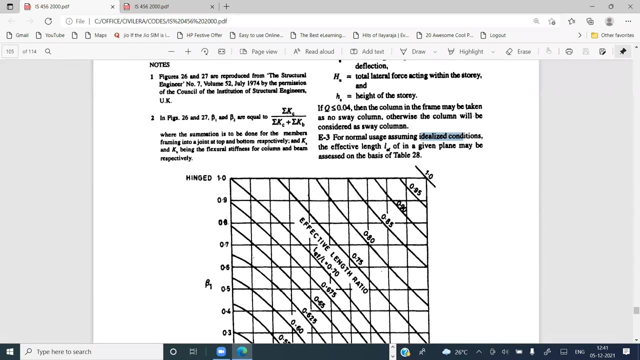 Only if this condition exists. E3. For normal usage. assuming idealized conditions, effective length in a given plane may be based on table 28,, which is for normal usage. What is normal usage? What is idealized condition? Code is not saying this. Yeah, So for larger buildings. 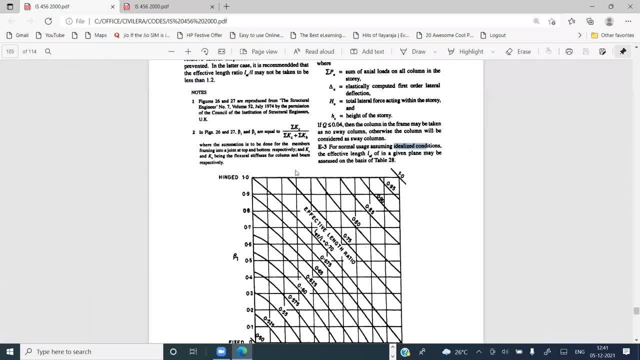 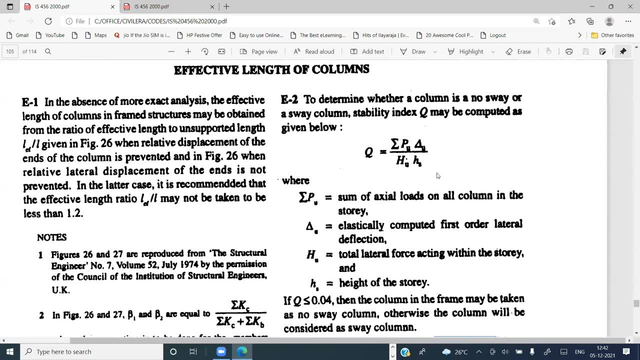 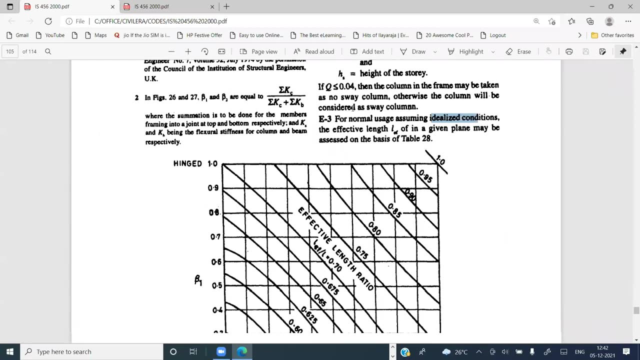 like a 10 floor building or even three floor building. you should use these graphs. You need to calculate sway index as per this. I cannot explain this again. You need to read and understand if you don't know. but then you have to adopt this calculation and your effective length. 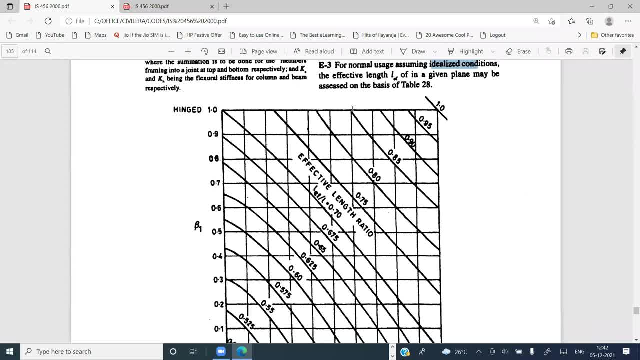 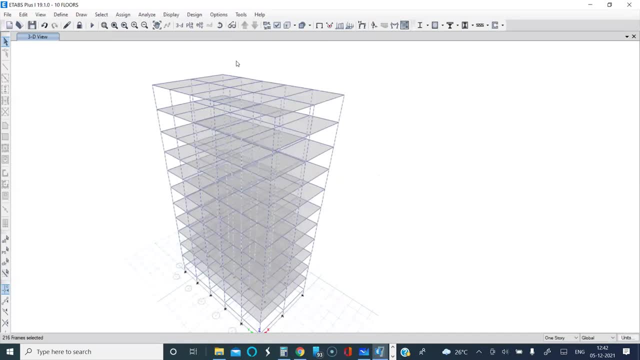 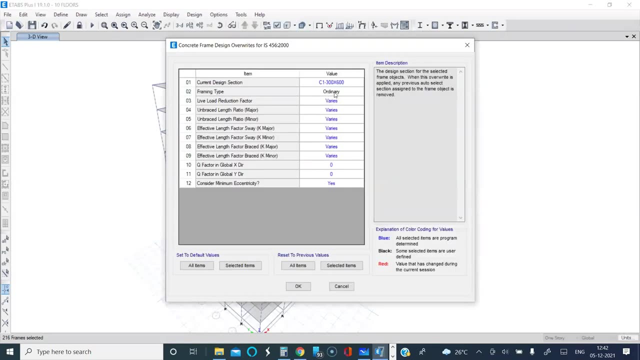 will be much more than the height of your building. That's all you need to know right now. You cannot use simply table 28.. What I mean to say is: in ETABS, you cannot blindly use your design parameter just like that. You need to know why you are using ordinary. 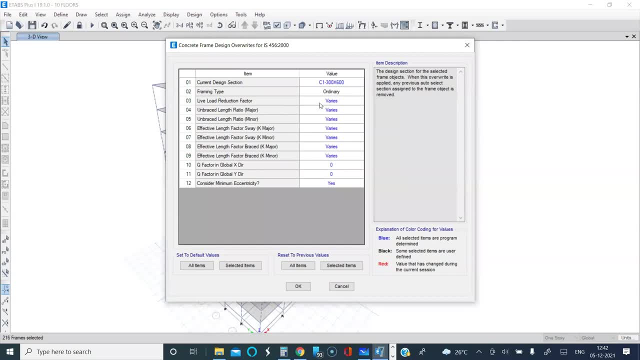 why you are using non-sway when you have to use the other thing, Same way, various things like live load reduction factor. you need to appreciate why we are going to give that. Yeah, Once you know that ETABS will do it correctly. Yeah, So knowing that understanding, 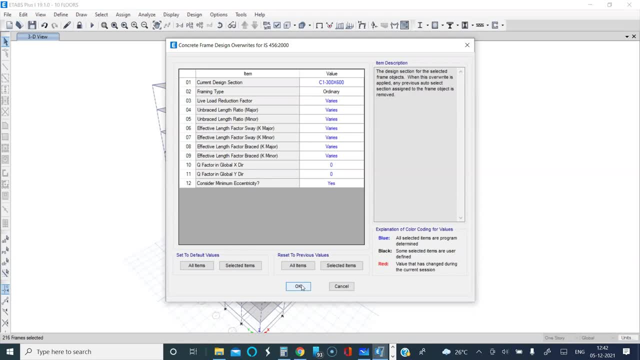 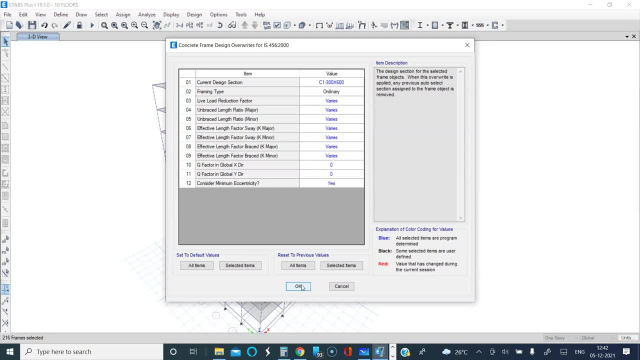 and things like that. Okay, So that decision cannot be taken, or I cannot convey that in one hour's time. So that's where experience matters And that's where I'm going to handheld you and make you aware of these things and then make you independent to take these decisions. 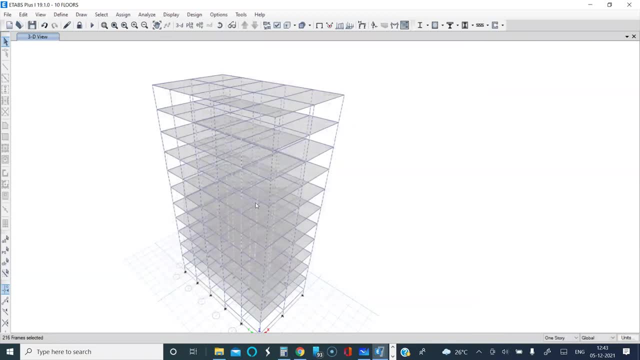 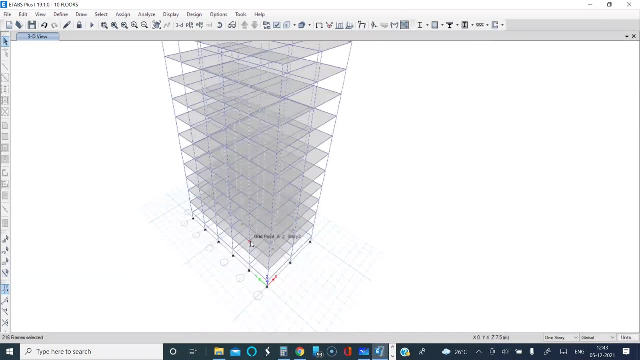 Yeah, It depends on a lot of parameters. In your textbook, if you see, you will see the column is in double curvature. In your textbook you will see the column is braced. But then how do you know if it is braced or unbraced? ETABS or STAT cannot decide it. 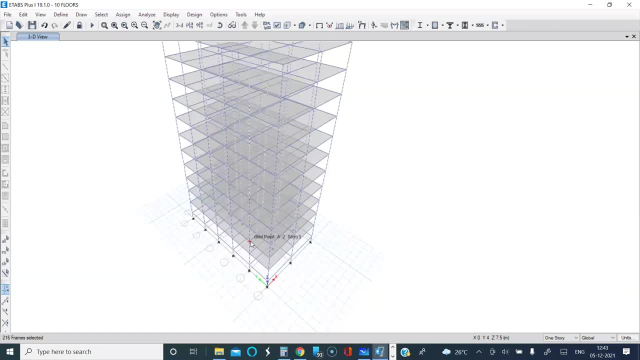 completely on its own. STAT cannot do it, even partially. ETABS can do it to an extent. Yeah, So you need to take that call if your column is braced or not, not column your floor. Yeah, So that decisions come only with experience, only with understanding of what it really means. 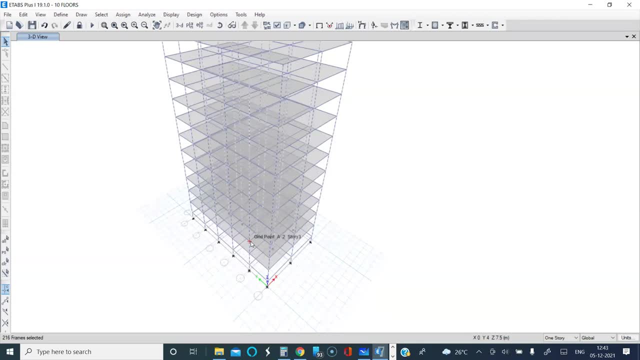 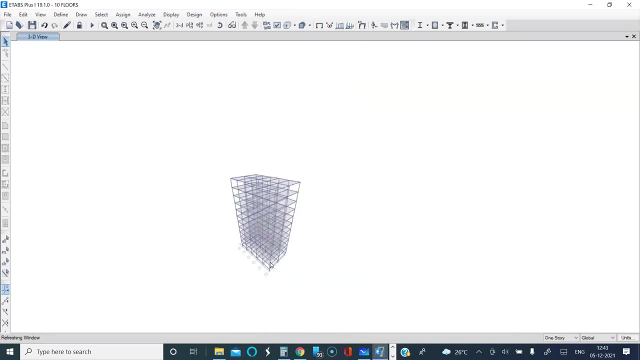 Textbook gives you. unfortunately, in BTEC or even in MTEC, your textbook is giving you that value Or that message that your column is braced or unbraced, or it's in double curvature, or whatever. Yeah, So that is what matters. Modeling and designing: you can do it just like that. 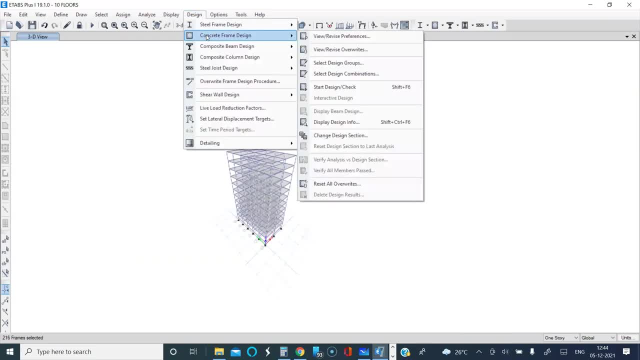 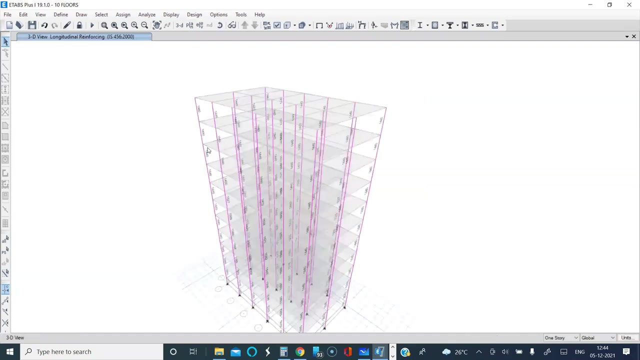 Okay, So here: design, concrete frame design. select your design combinations. design, concrete frame design. start design, check. That's all in ETABS. But then until and unless you know how that parameter, the parameters, are taken, you won't be able to arrive at that. So it's displaying your steel here. 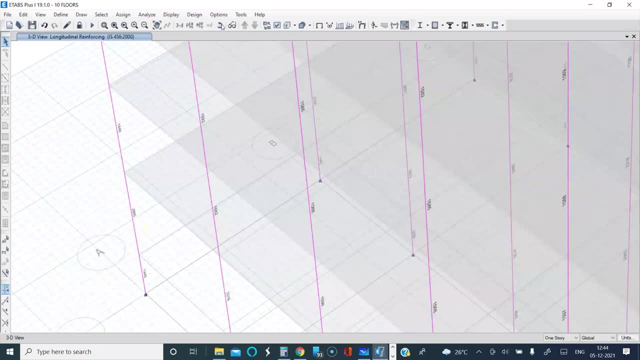 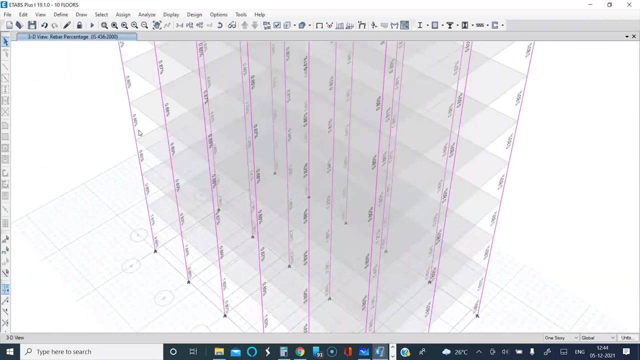 Now you can start refining it based on if it's more or not. So design: concrete frame design, display, design info. You can even say rebar percentage. So you can see the rebar percentage here: 1.61,, which is very less. So you can maybe slightly reduce the size of the column. 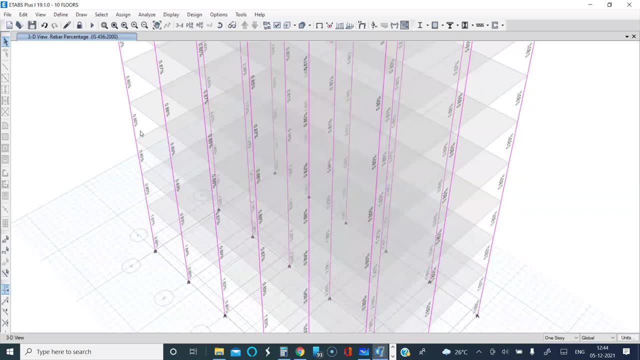 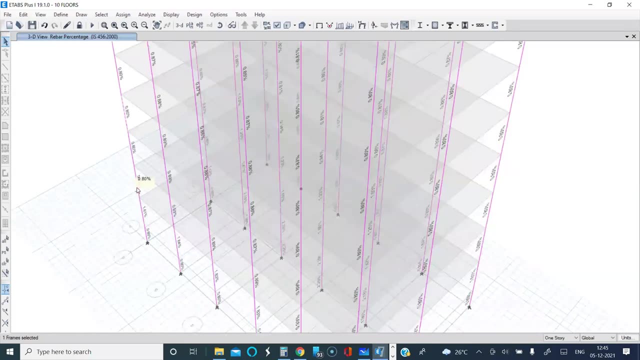 But we have not put a dead load in every- I mean the wall load in every floor, things like that. So, based on the final design, you can decide if you have the opportunity to reduce the column size, things like that. 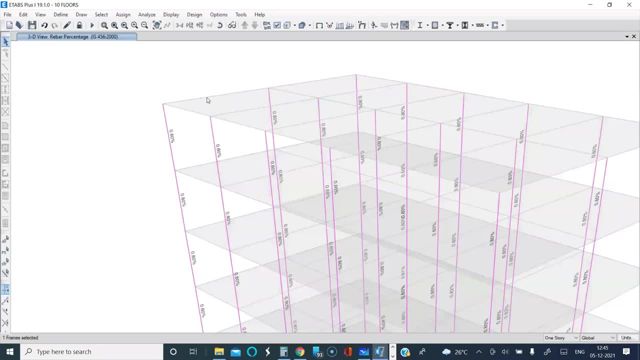 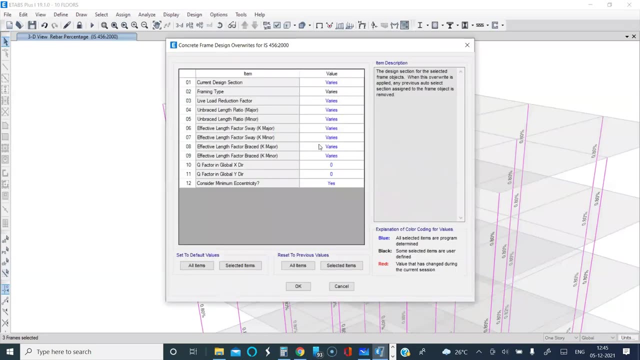 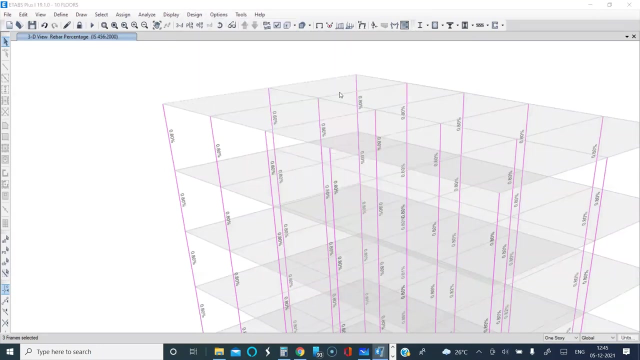 Yeah, Same way. design of beam is also very easy. You select the beam to be designed, go to design concrete frame design, give the parameters, as I said, and then say design- concrete frame design. start design Design. check So that will display the top and bottom reinforcement You need to convert. 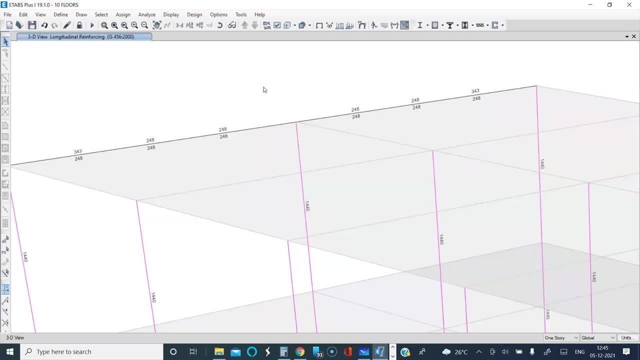 this into a drawing. Yeah, So you have the top steel at the left, support 343.. Top steel at the right, support 248.. Bottom steel: throughout: 248.. Here again, right end, top steel 343.. So you can infer this and then come back. 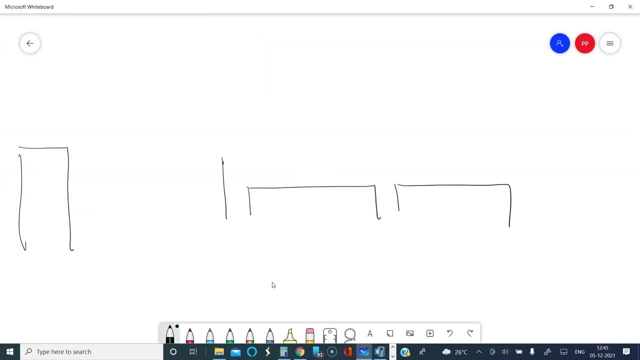 And convert that into a drawing. So you have 343, right, So you can take the message and then give 212, extra bar, extra bar. So this may be 212, this may be 212, because 343, something was required there, Yeah, So that way you can do that Same way. 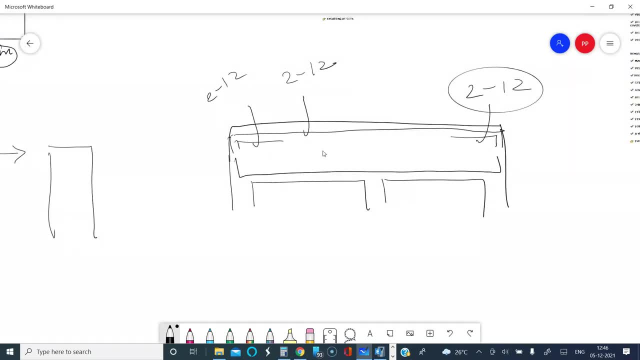 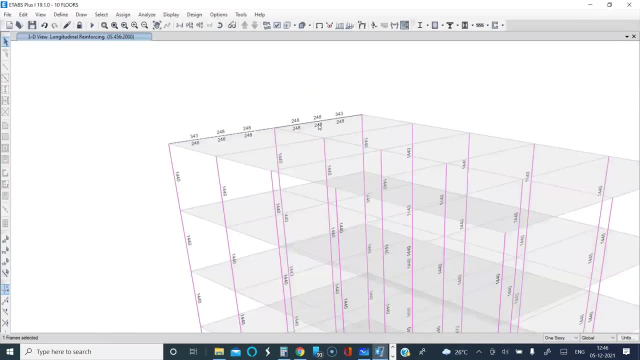 shear force everything. you can do it, but with time limitation I won't be able to explain each and everything. There are many videos in my YouTube which are freely available. You can learn from that. See those who don't think that these programs are. 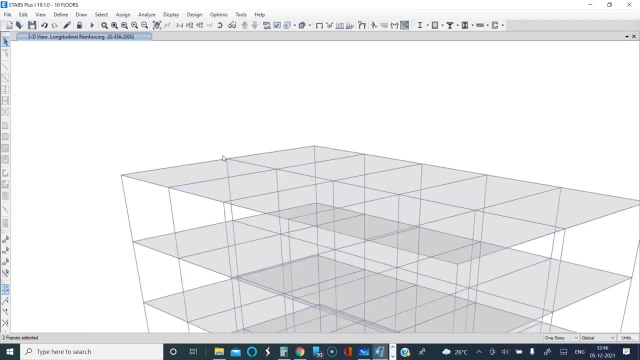 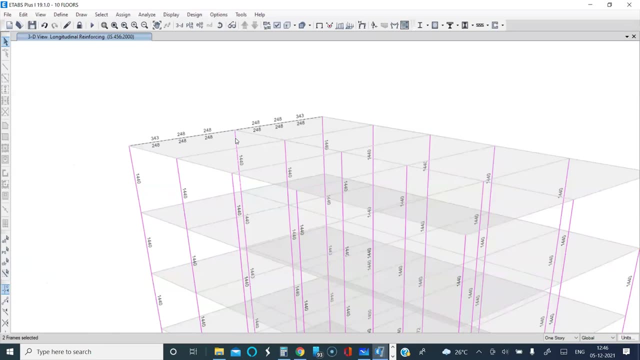 valid enough for you. you can stay in the group and then learn free, but that will be a more time consuming and a tedious process. If you want quick hand-helding and then learn faster and then be independent and learn each and every tip and tricks that I'm going to teach, then enroll for. 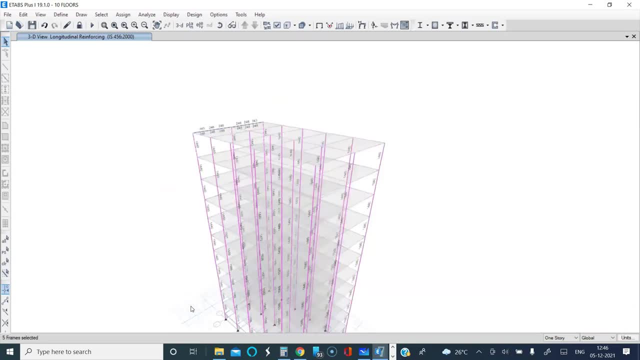 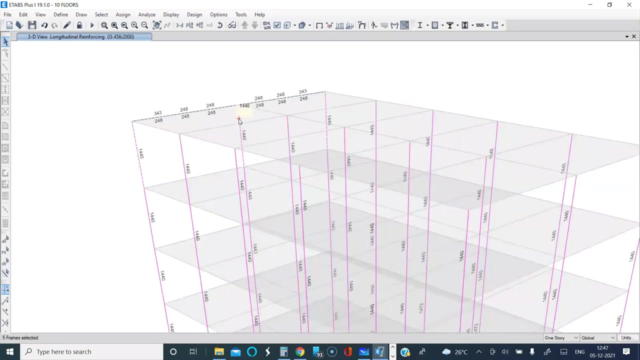 that. So that's it, Thank you. the courses. Now what I will do is I will open up this forum for questions or any discussions, because it's already nearing one o'clock. I'm sorry for rushing through the modeling, because I don't have any other way to finish the thing, Because in two hours you can see. 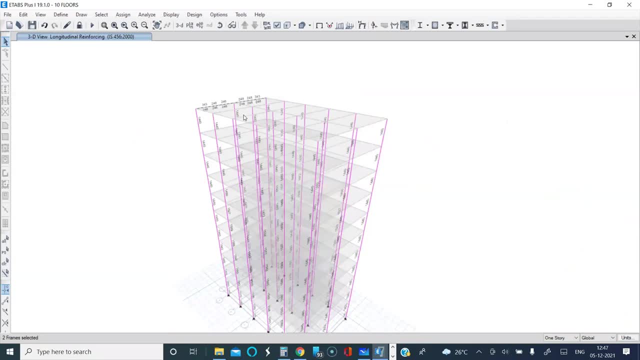 we could only cover this much. Explaining each and every point will take days, because it's not a simple thing. So I will open up this forum for discussion. you can ask me your questions. give me a minute and i have not read each and every chat. 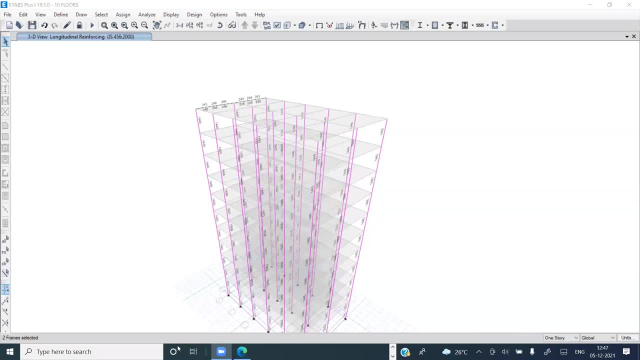 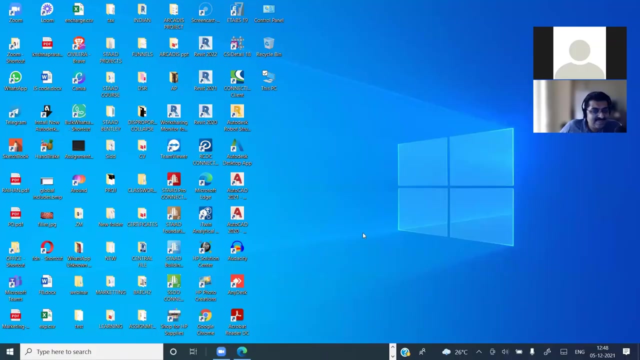 so if you have asked any question in the chat, uh, please ask me again, because i might have missed. there are so many messages here. give me a second. let me open up. yeah, so anybody has questions? you can, uh, ask your questions. siddish, you have raised the hands, amit. 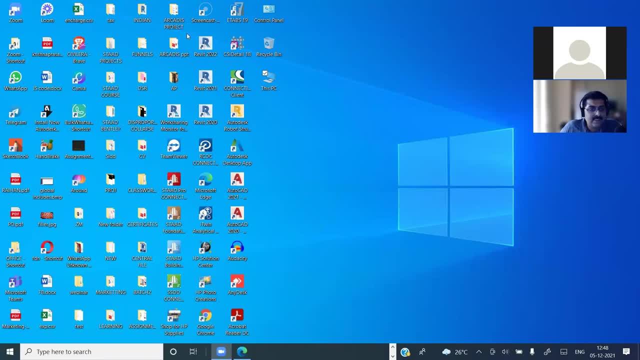 you can unmute and ask me now. your mics are open. hello sir. yeah, who is this sir? i'm hemant, sir from bangalore. yeah, go ahead, hemant, you can ask me your question. good afternoon sir. good afternoon sir. uh, could you suggest me whether for steel structures, either etaps is good or 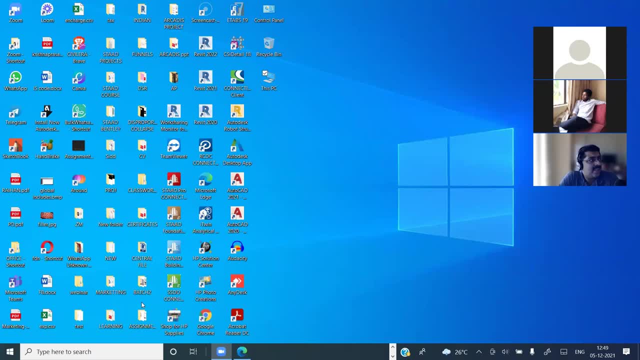 statpro is good, sir, for designing of steel. see, it's like uh asking virat kholi is better or rohit sharma is better for being the captain. yeah, captain is as good as the team. the same way software is as good as your technical understanding. 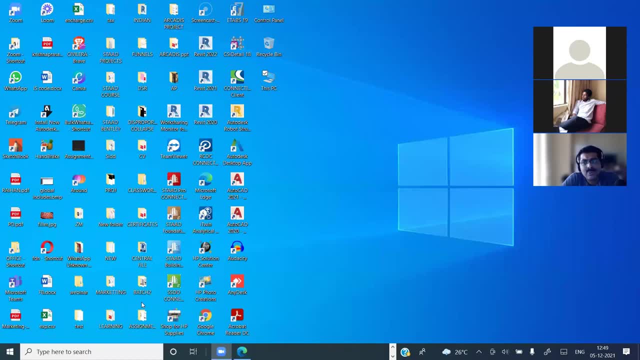 you can use stad. you can use etabs, both for steel or rc. both has options for designing, analyzing everything. options are there in stand as well as in uh eight apps. you can use either of this, but you need to be thorough in connection details and you should also be thorough in scheming and 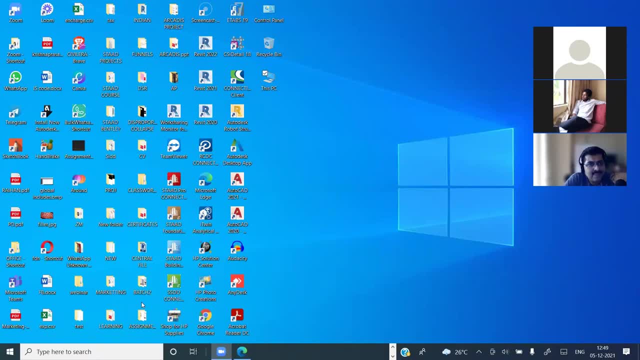 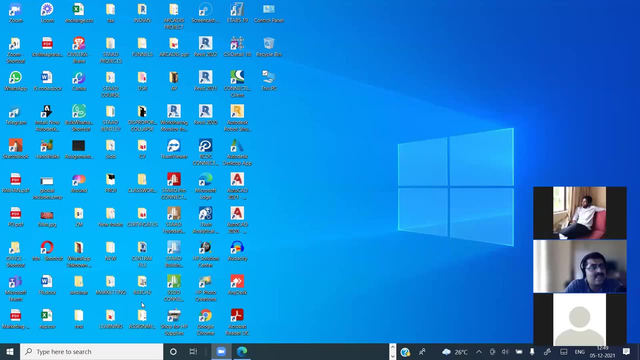 the various options that you have in scheming. yeah, how do you brace, how do you decide your wind load path? so all that becomes very critical. steel structures are more about connections, more about finding a way to brace, finding a way to load transfer. so if you have that expertise, 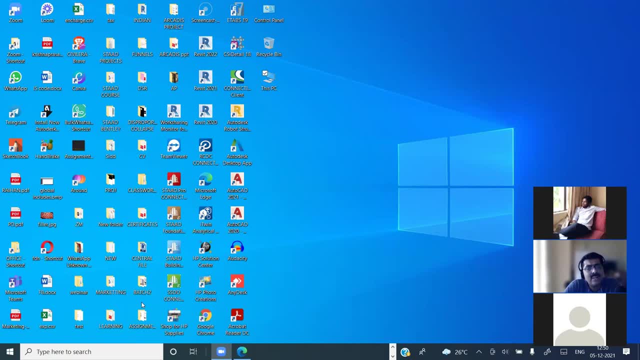 i don't see any reason that you cannot use stade. you cannot use etabs. both are equally good. stade, unfortunately, is very poor for rc, but it's really good for steel. etabs is good for both, sir. okay, thank you, sir. do the both give same value, sir, like quantity of steel? 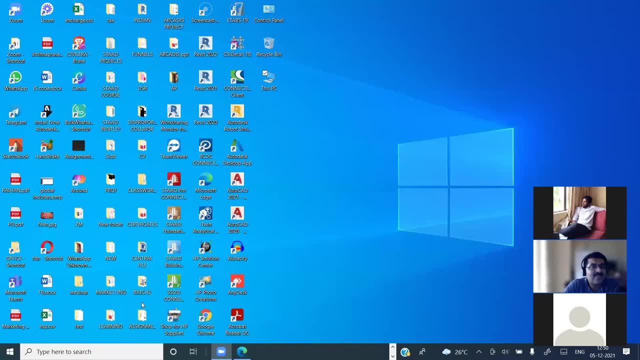 see that's again coming back to, uh, what i said about the effective length factor. yeah, so if you don't know how to use the effective length factor, you will think that stat is giving less steel and etabs is giving more steel. but if you know what etabs does and what stat does when you don't- 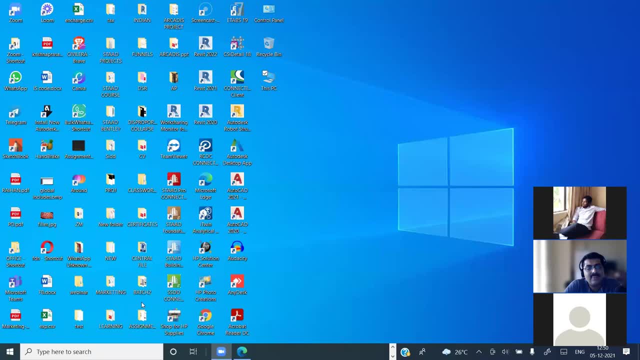 give that uh option when, when, when, you let it choose its own, then you will understand that the change is because of that. so, in fact, if you know how to use each software, understanding its limitations and its strengths, if you give the inputs in the way that you should, 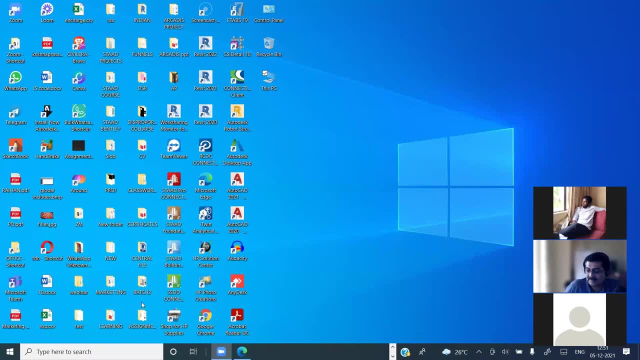 give in both of it. both will give you the same answer, because both are tools and both analyze in more or less the same manner. design commands are much, much simpler when it comes to, uh, steel or concrete design commands are very minor things. analysis is what the most gist of it is, and it employs similar methods and 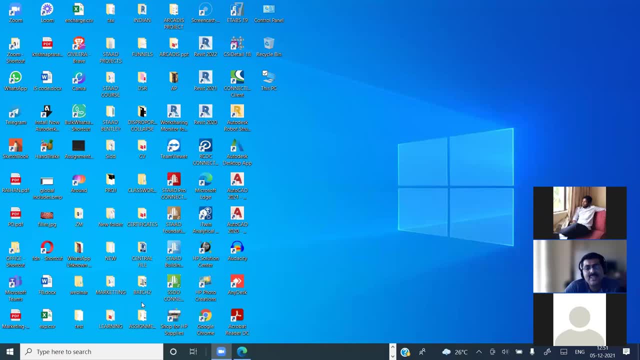 similar accuracy will be there when it comes to design. there will be slight differences. the reason is it treats things in different ways. for example, stat designs- uh, an rc beam at the center of the column. etabs design is the center of the column. etabs design is the center of the column. 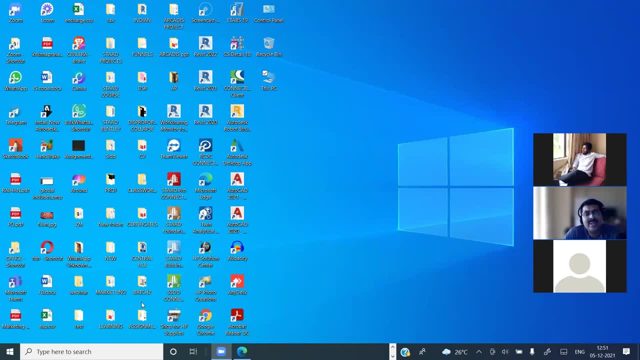 at the edge of the column. now you can make stat do it by doing certain things. but if you use the default option in stat, it will design at the center of the column and you will think that the steel is more. so you cannot blame the software. it's made for that or made in that way, so you 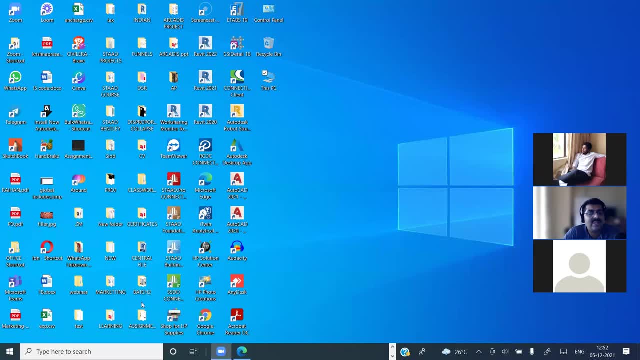 need to know how to use it, to tweak it to suit so that you get the right answer. yeah, so if your parameters are correct and if your interpretation is correct, both will give you the same value. hello, sir, my name is amit. i'm from lucknow. yes, sir. uh, super dead. 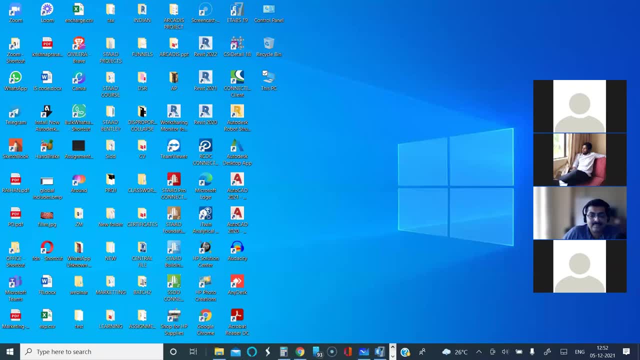 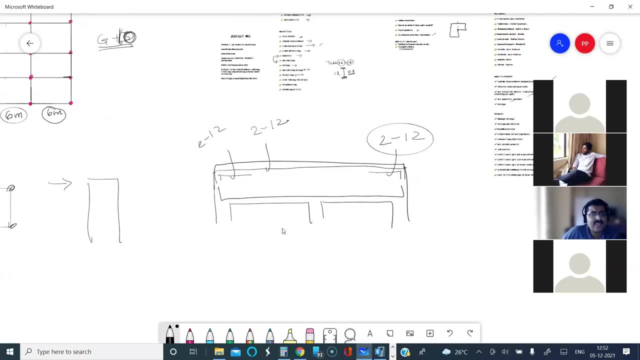 load. uh yeah, see, there are different uh uh loads. dead load itself you can classify into many because, see, whatever you are modeling, your core member loads, beam slab columns, all these are dead loads. now there are super dead load means you have things like finishes, you have things like, sometimes, equipments, yeah, even. 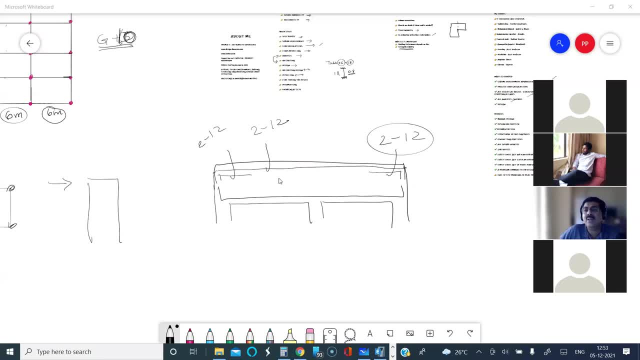 though, uh, most of the furniture are all part of live load. there are certain things like that. yeah, so these are all super dead load which we are not modeling, so that needs to be applied separate. hello sir, yeah, uh, my question is: uh, the soil report is required for g plus one building, or? for every building you need a soil report from which city you are. okay, see, the cost of one uh soil test pit for a residential building in bangalore is as less as five thousand to seven thousand rupees. yeah, so there is no harm in getting a soil report done. 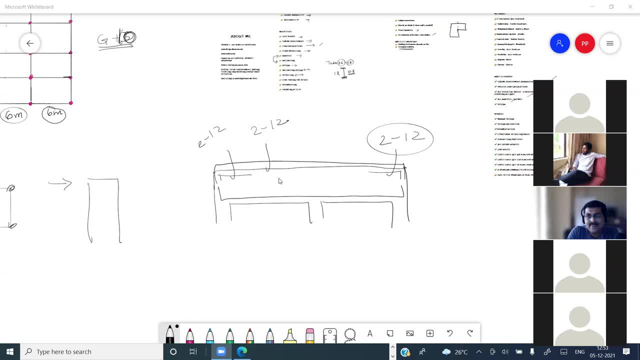 for one floor building as well, okay, otherwise local, uh yeah, otherwise you will go to. ms3 is designed so if you are okay with that, with that then you can get the actual soil bearing capacity and then sometimes see, if you don't get a soil capacity, what will you do? you will assume a soil. 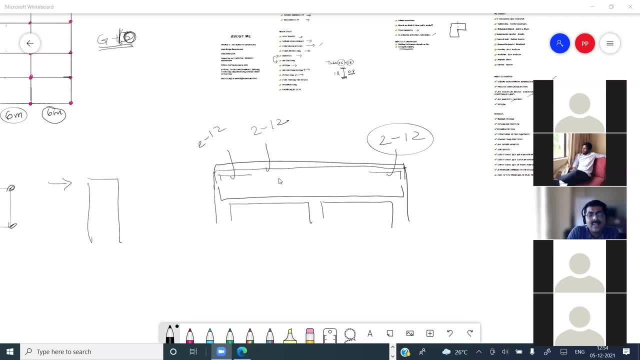 bearing capacity right now. yeah, if you assume it to be 200 and in reality if it is 300, you are. you are wasting your client's money. so tell the client that if you do it and if your value is 300, you will save much more than the soil investigation cost. at the same time, okay, you assume 200, and if 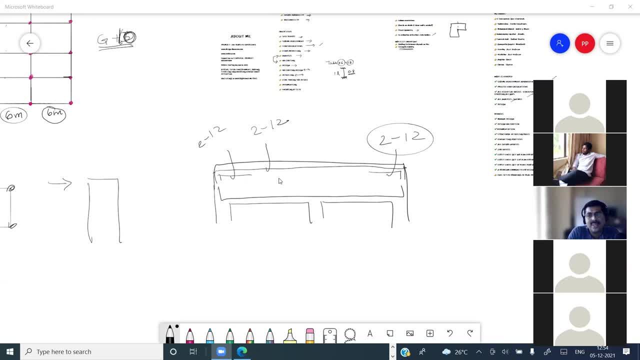 it is actually 100, then what happens? then? there are chances of settlement also. so you are risking. so educate them, yeah, about the risk and also the savings. if your sbc is more, you save, if the sbc is less, you are risking. so if you are able to convince them, seven thousand five hundred to ten, 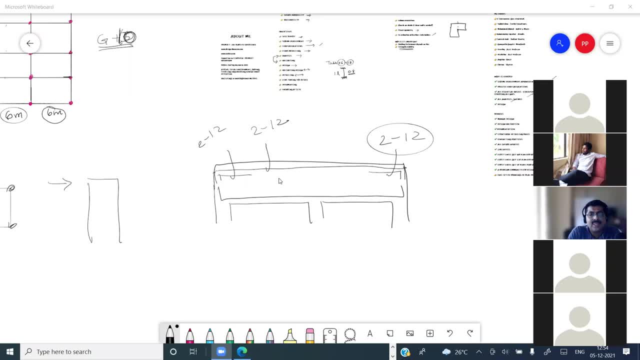 thousand rupees will not make a big difference. now in case, if your loads are very light and if you are waiting, yeah, go ahead. what we can gain footing in it is see, uh, footing slabs and all that uh, you cannot design because it's all shell based analysis in etabs or any software for that matter. yeah, so if you 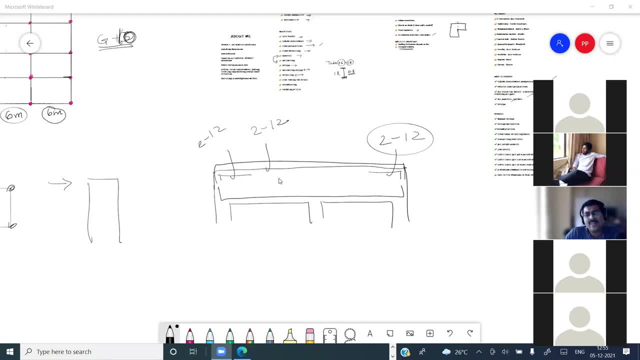 are wanting to do that. you can interpret the results when you model it as a shell and then designing something uh from the result is a two-step method. you just need to find the steel for your moments. you need to ensure your shear is within limits and your punching is within limits, so you don't need any software for a normal. 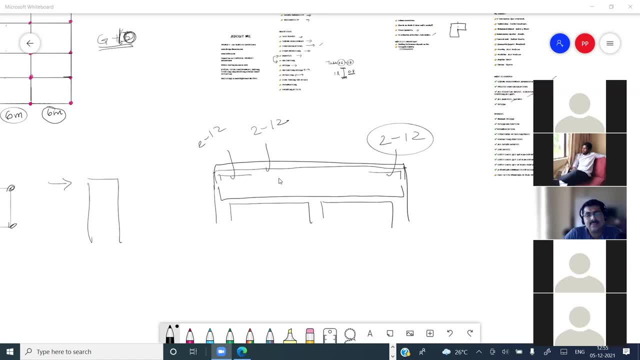 isolated footing design. okay, sir, hello sir, yeah, sir, hello, yeah, hello sir. how to decide if a slab needs a secondary beam with a lbc beam? okay, so you can do it with a concrete slab or with a shell, with a concrete slab. so you can do it with a concrete slab. so you can do it with a concrete slab. 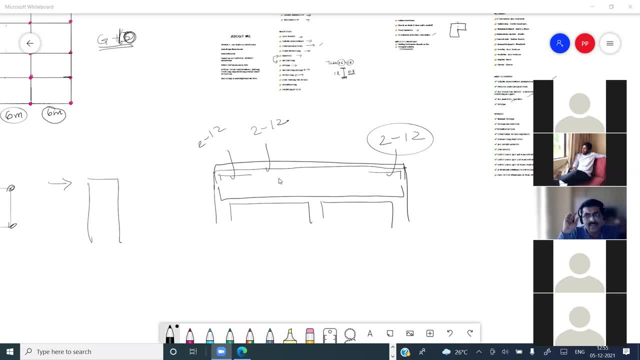 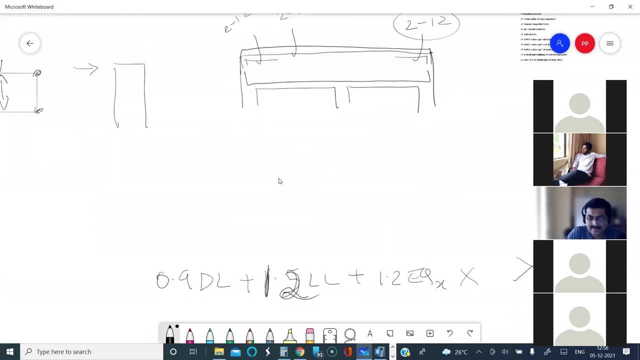 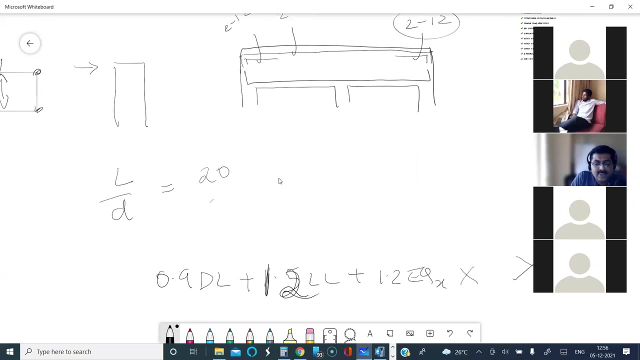 ratio factor. yeah. so, uh see, in slabs, in most of the cases deflection will govern. moments are unlikely to govern. in most of the cases, deflections are going to govern. okay. so if you refer codes based on l by d ratios, if you are having a simply supported, it's 20, correct. if it is continuous, it. 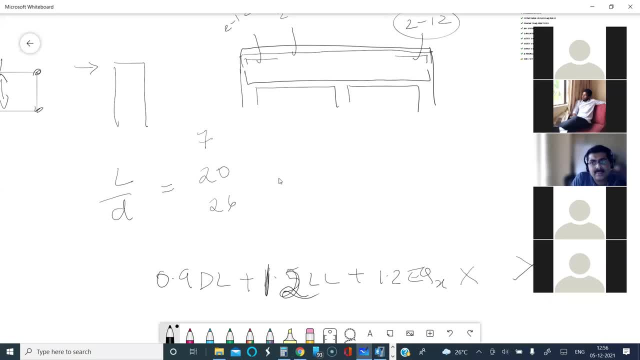 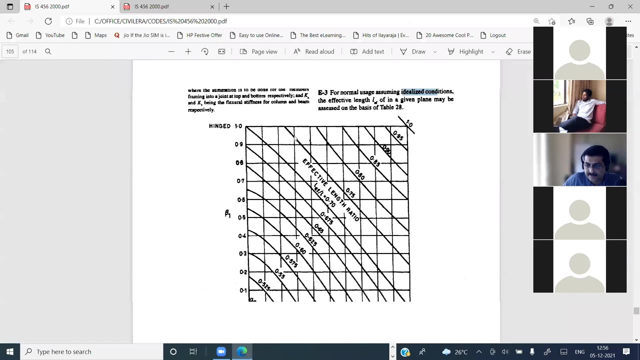 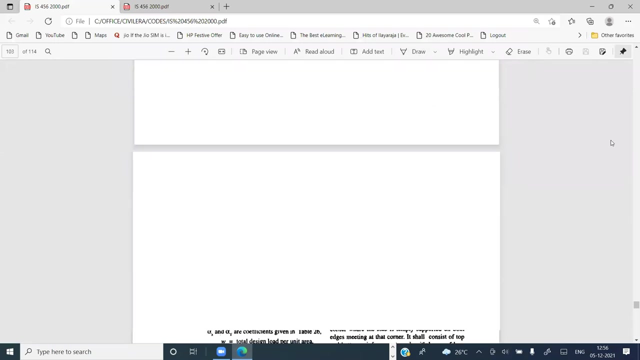 is 26, if it is cantilever it is 7. yeah, so you can adopt this. but then there are certain things. if you have time, i can just show you one second you give me. it's very important. good that you asked me. see, first thing is give me a minute. yes, the close is around 23. close number 23 or something. 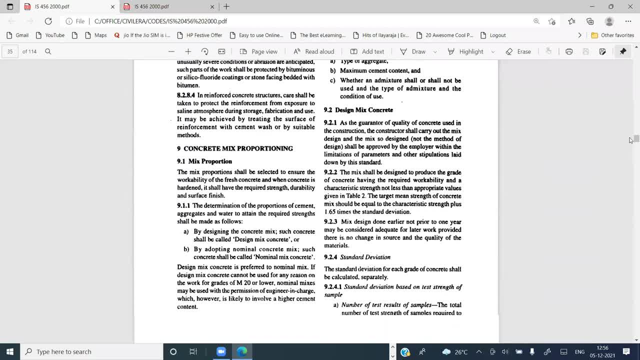 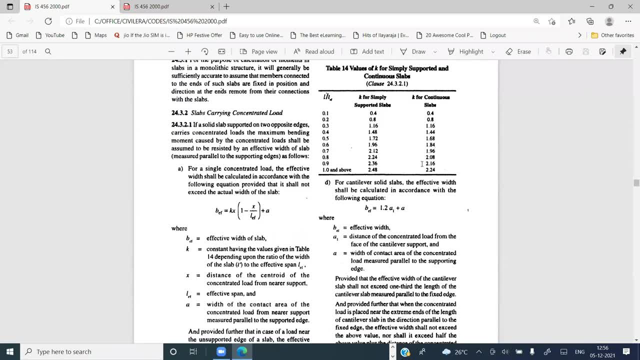 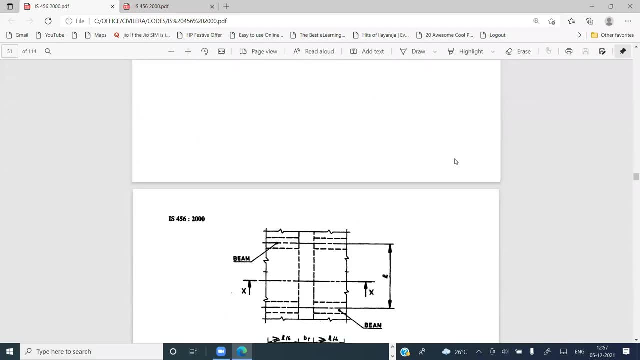 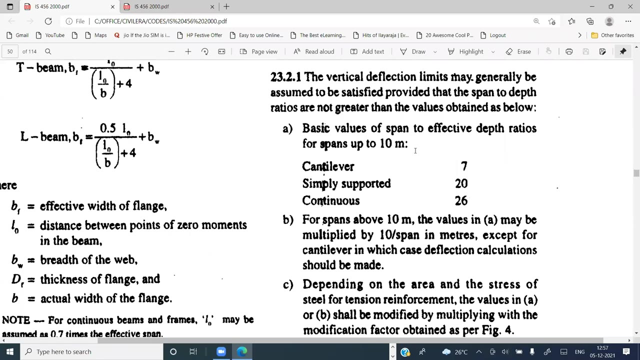 like that. let me come to that close in the code. yeah, so first thing that you need to understand is this: l by d ratio, given here 720 and 26. okay, now this you need to correct it with the steel. see, if you read here, depending on the area. 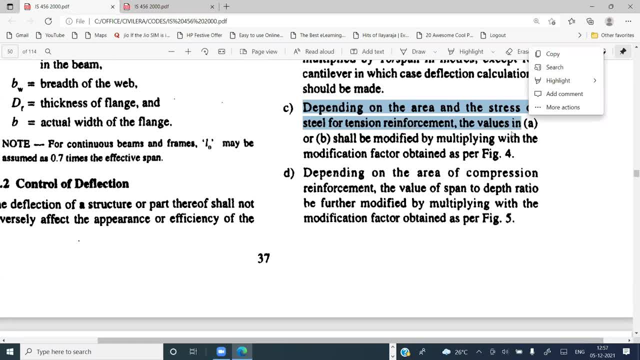 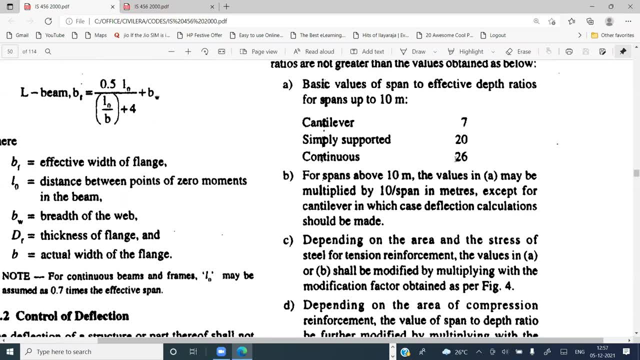 and the stress of steel, of tension bar. the values in a or b shall be modified by multiplying with the modification factor. so this say: assume that you have a continuous slab. yeah, so this is 26, but but this can be 32, this can be 40, this can be 50, depending upon your steel provided. so you have to 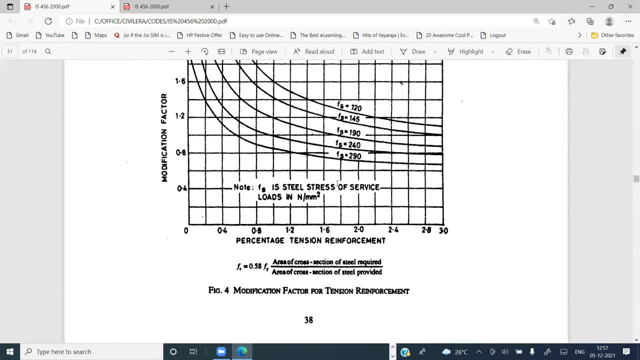 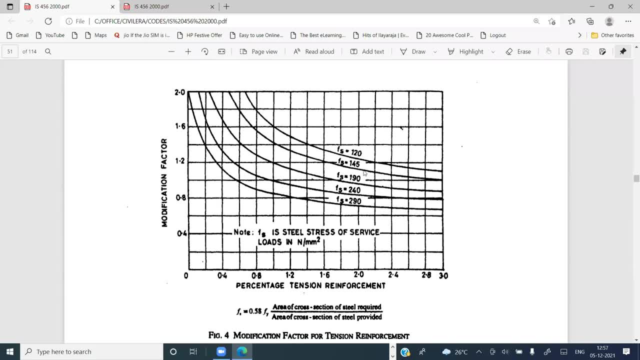 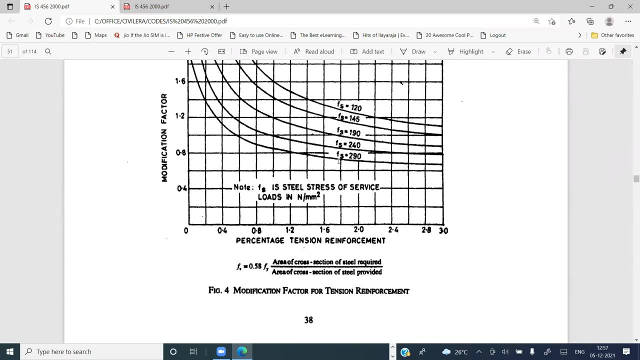 use this particular graph. okay and based on this modification factor, it depends on the percentage of steel that you have provided and the stress in your rebar. see if you are using fe 415 grade of steel or fe 500 grade of steel, it is not fully stressed. 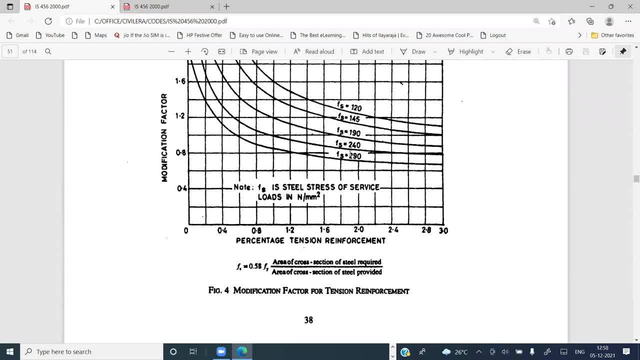 sometimes because you may need eight at, say, 220, yeah, but then you may round off it to eight at 200, which means your stress in the rebar is lesser, correct, say, you need eight at 300 but you rounded off it to eight at 200. so your steel that you have provided is much more than actual. 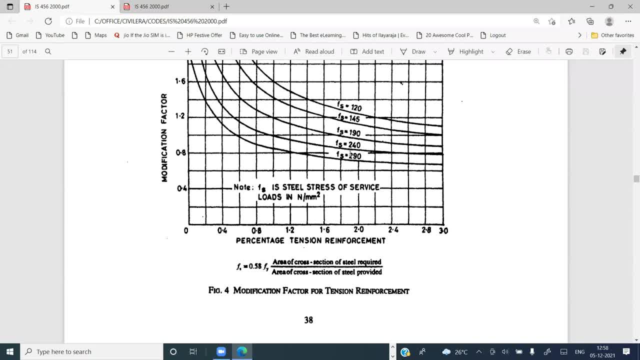 correct. you are getting me see eight at 300. you got by design, yes, sir, but you gave eight at 200 because maximum spacing- something, some rule. you decided that you will give eight at 200, which means you are given more steel than needed, which means that your stress is lesser. so when the 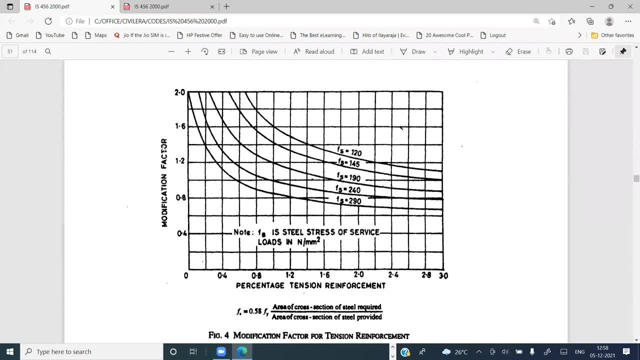 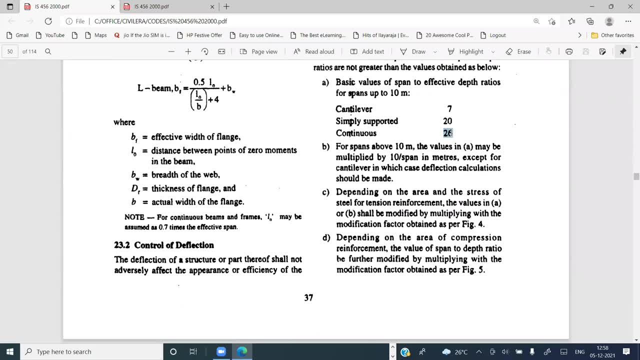 stress is lesser, you can take a modification factor. that's what this tells you. yeah, so you so that modification factor. you have to multiply and then this 26 may become 50, which means your thickness can be lesser. got it okay, blindly. take 26. you need to apply based on the steel. 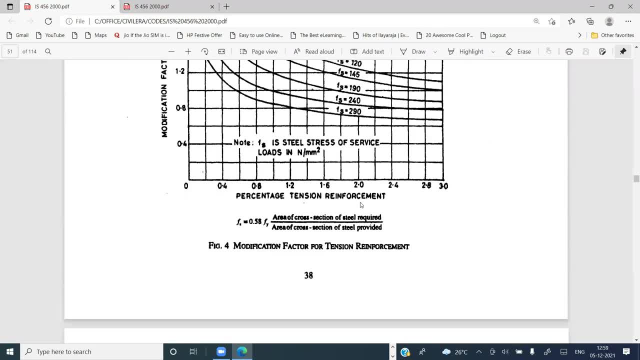 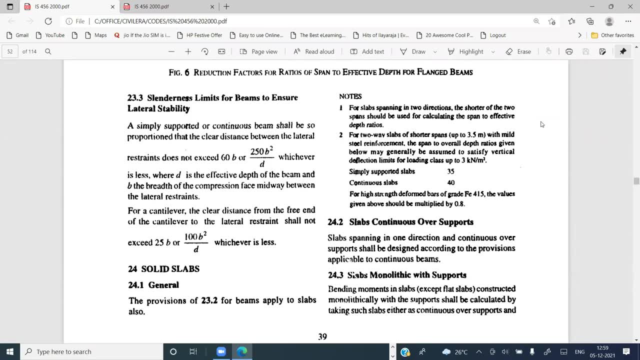 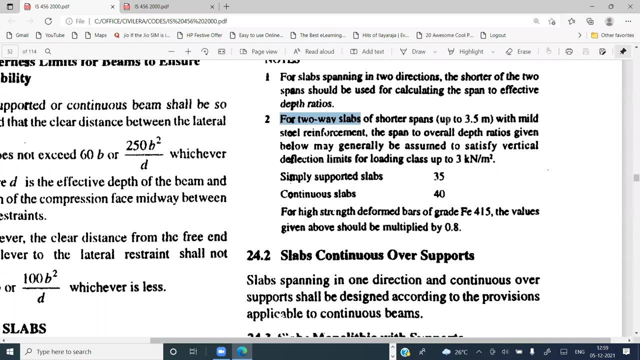 and the stress. second thing, if your slab is very less in span. okay, if your slab is very less in span, please read this note for two-way slabs, only for two-way, not for one way, okay. and for shorter spans up to three and a half meter. yeah, your uh value is 40, not 26, okay, but 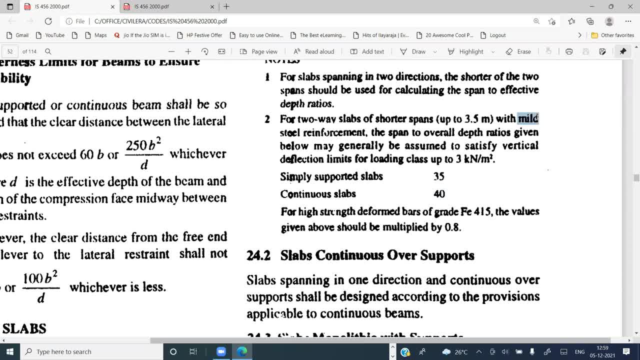 40 for mild steel. you have to read very carefully. we don't use mild steel, okay, so it says that if you are using hysd, you have to multiply it with 0.8. so if your slab is a small slab and if the live load is less than three, listen carefully. 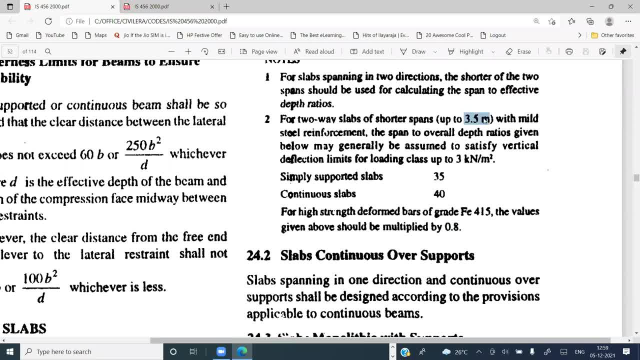 if your span is up to 3.5 meter and if your live load is less than three load class. loading class means live load. if it is less than or equal to 3, then l by d ratio can be 40 multiplied by 0.8, that is 30.8. 40 multiplied by 0.8: 32. so this 26 is for larger slabs for smaller. 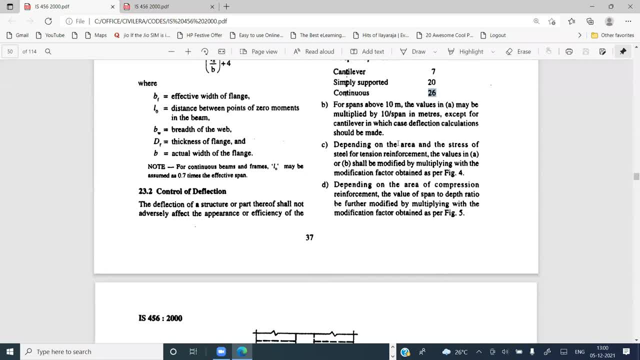 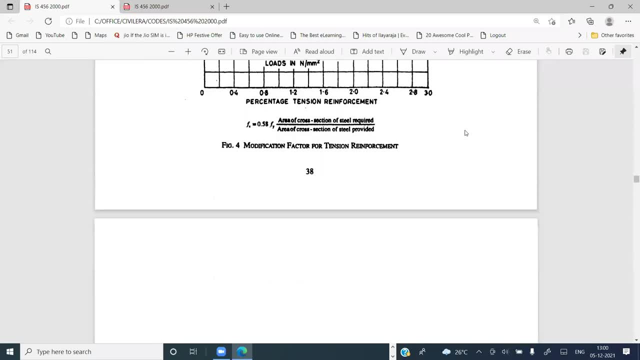 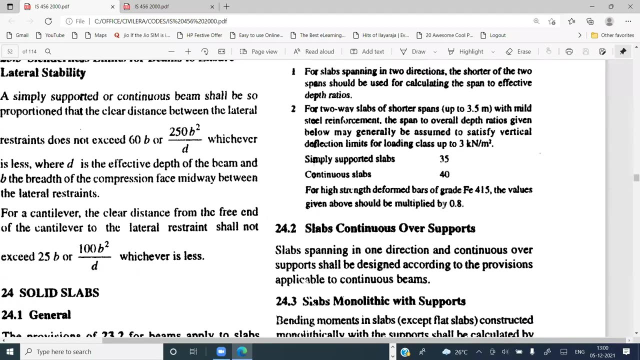 slab, it can be 32. yeah, sir, excuse me, what is what is for fe 5.8 then? what is that? what is for what? what's through? which factor should be multiplied for fe 500? just union code for every one. you can, you can, you can use the same you can use. 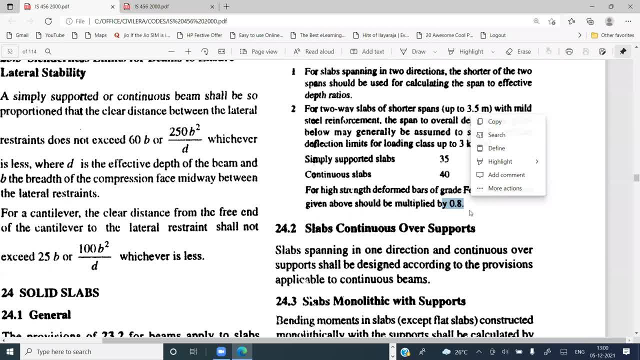 the same, but in case, uh, 500, sir, 5.5, you can use the same thing you can use. yeah, same thing you can use, and in most of the cases the same thing can be used. yeah, same thing you can use, and in most of the cases, 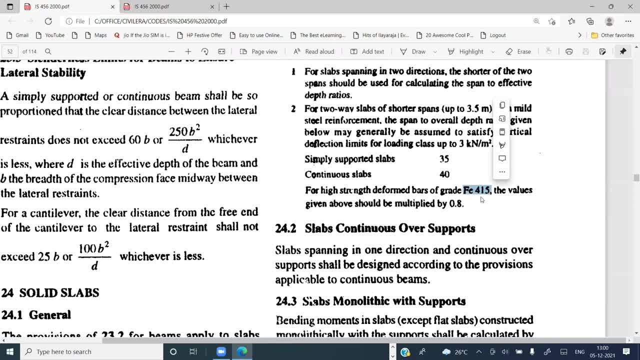 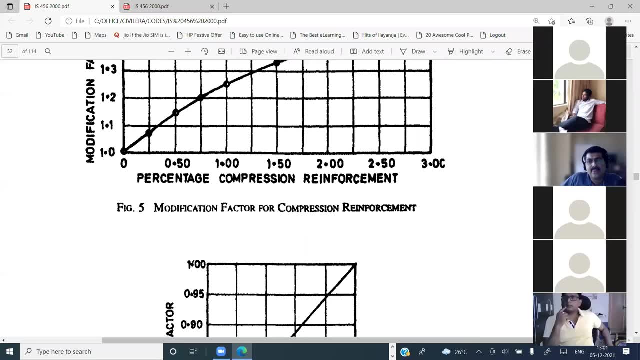 in slabs, smaller slabs, grade of steel is not going to be much different, in the sense it is not going to make a big difference in a design. Any other question, Sir: what is torsion constant at moment about 2 and 3 inches. 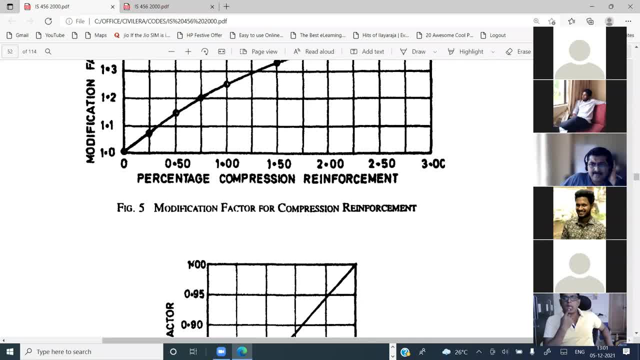 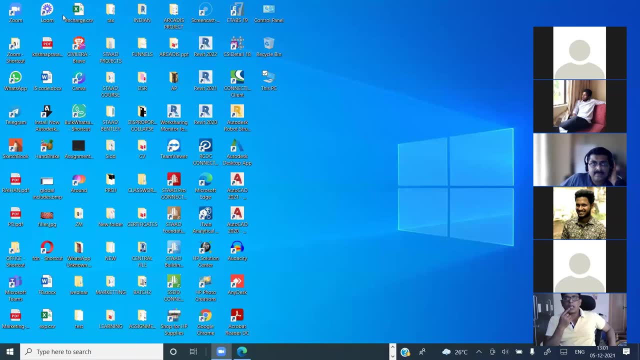 I didn't get you. What is torsion constant? at moment about 2 and 3 inches, while we are defining material properties, While defining material properties Three times. When we are defining material properties, then there is a column where you have to put the values of 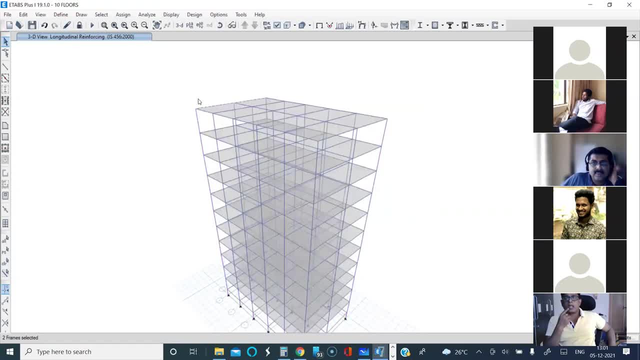 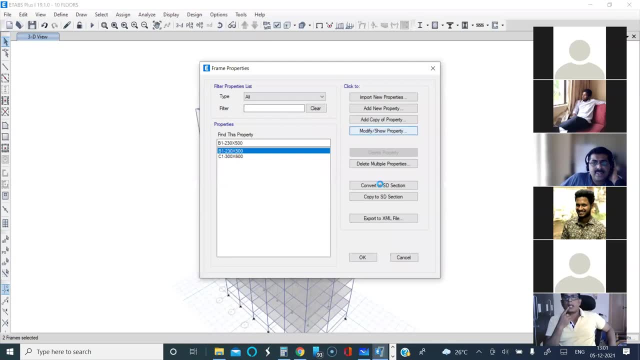 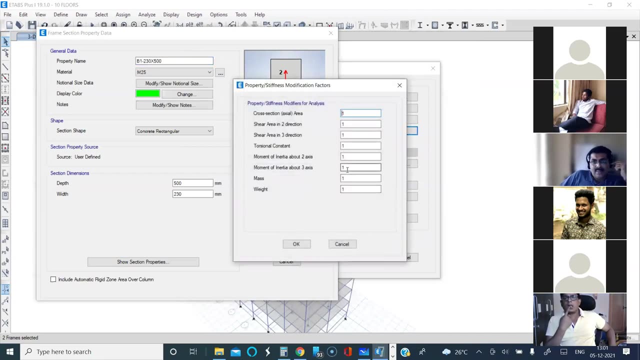 moment of inertia about 2 and 3 inches and torsion constant. Yeah, yeah, See any material you are talking about this, right? Yes, sir, This value, Okay, See when you analyze, when you are using Canis method or moment. 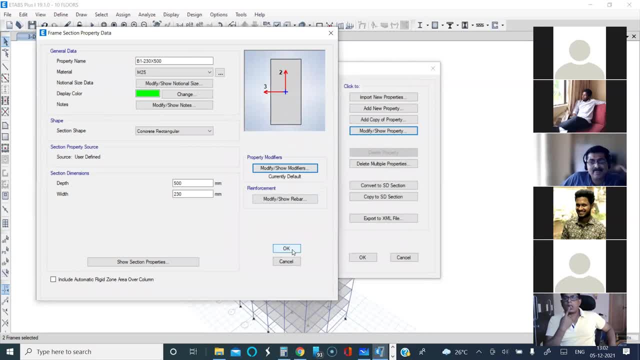 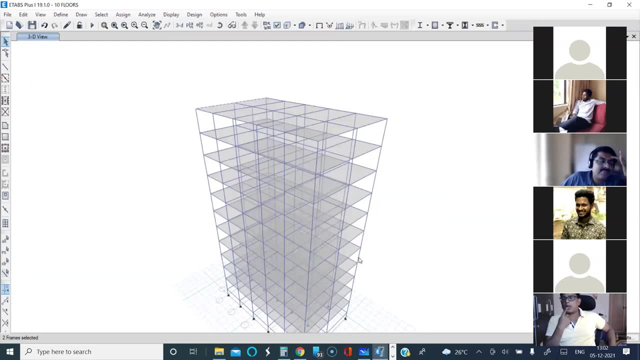 distribution method. have you done moment distribution method and do you remember? Yes, sir, Okay, So when you do it, your stiffness is calculated based on inertia, BDQ by 12, right? Yes, sir, Now did you account for. 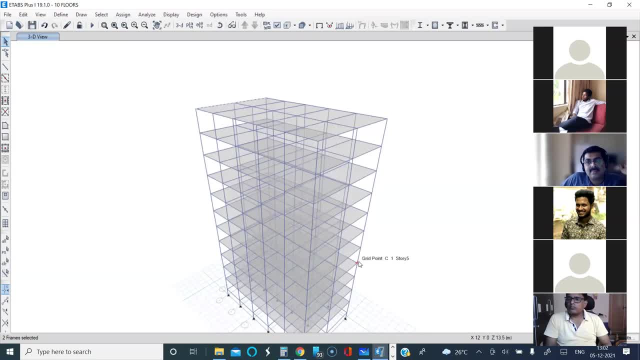 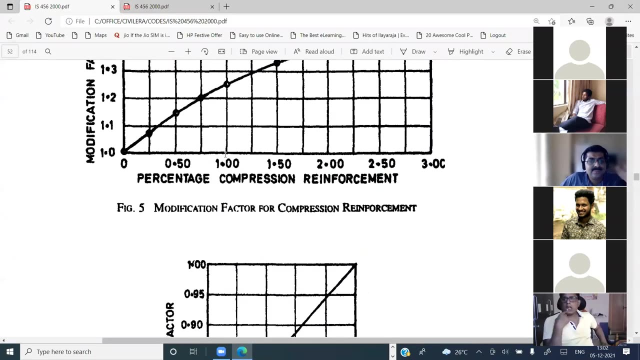 your steel's presence. When you calculated inertia, did you account for the presence of rebars in it? No, Why you didn't do that? Because code tells you if you, everything is in code. In fact, if you read code, if you read, 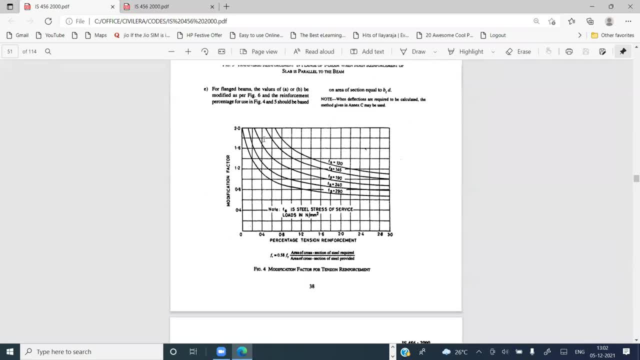 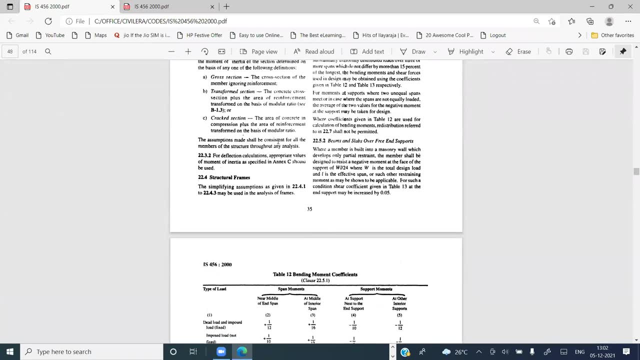 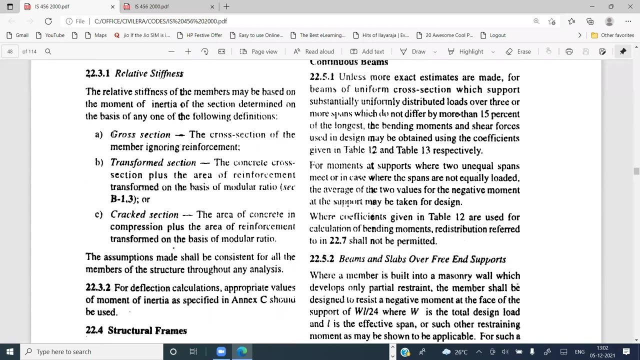 code. I think close number or this is in IS456.. Equivalent equivalent: See if you read 22.. Quantity is very. code is allowing you to use gross sectional property or transform section or crack section, Any of it you can use, The only. 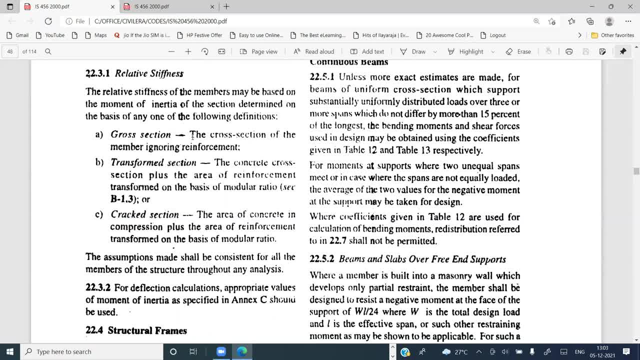 condition the code tells you is: you need to have consistent consideration. That is one beam Gross section and another beam cracked section. One beam cross section- gross section, one beam transform section. You cannot adopt. You have to have consistent practice. So gross section. that's what we were doing. 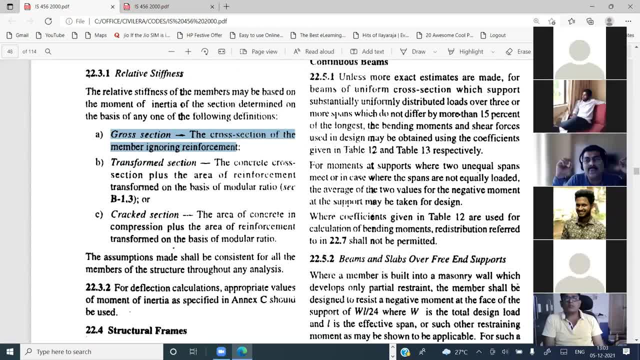 Yeah, But then in reality, what happens is any member, you like it or not, will crack, Yes or no Microcracks. Now, when cracking occurs, what happens? Your stiffness is different. Yeah, your deflections will be higher. 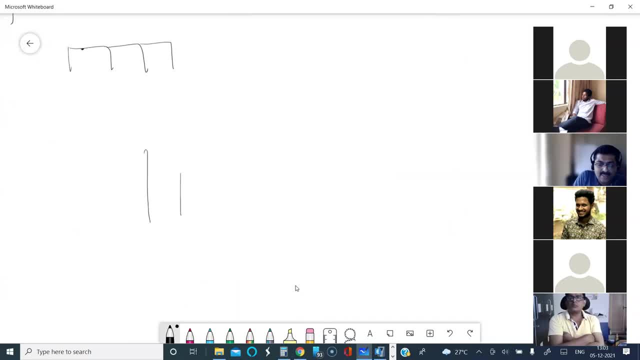 Lateral deflections I'm talking about. See, I designed a beam, I gave a steel, Something like this, But in reality this I gave, say, 212, and say I gave 216 extra, But in reality the stiffness is not this much because it cracked. 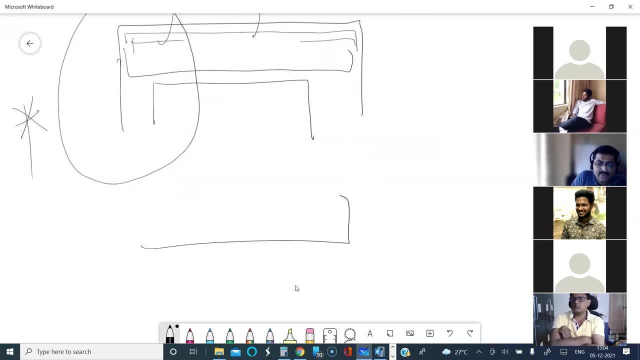 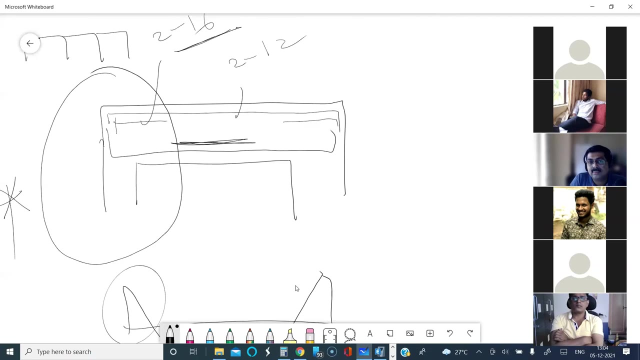 Yeah. So what happened? It will redistribute. The span moment will become more, The support moment will become less. So you don't need say 216 there, but you need more here. Yes, sir, Yeah. But now how do you know how much it cracked? 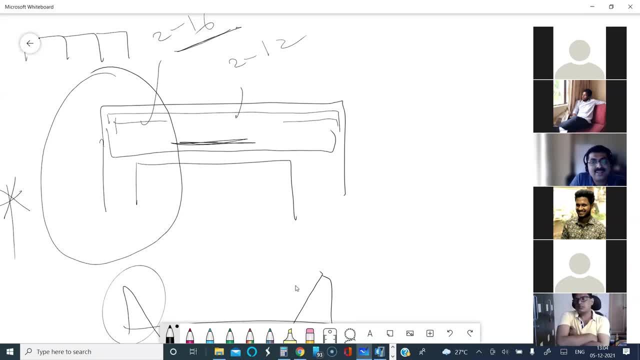 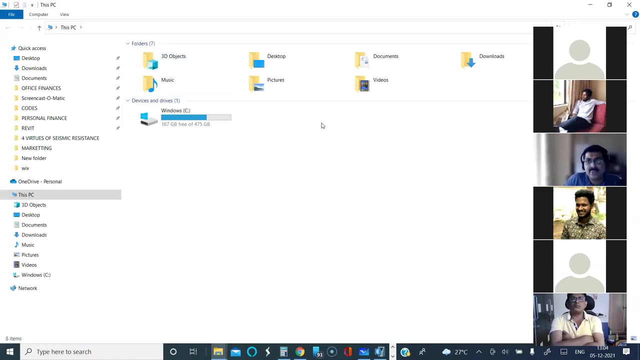 How do you know what is each beam, How much it will crack? You have no idea about this. So I guess 1893 tells you. if you go to 1893, it's a global practice- Even even if you go and check American codes, it's there. 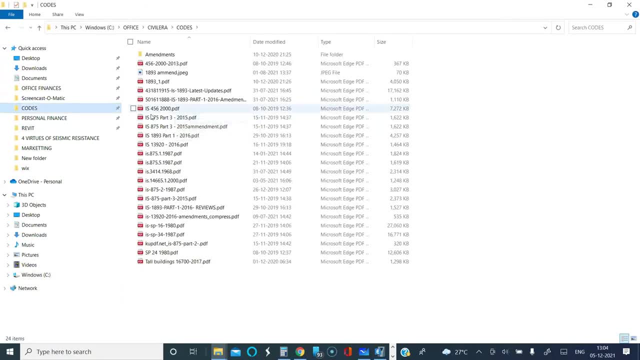 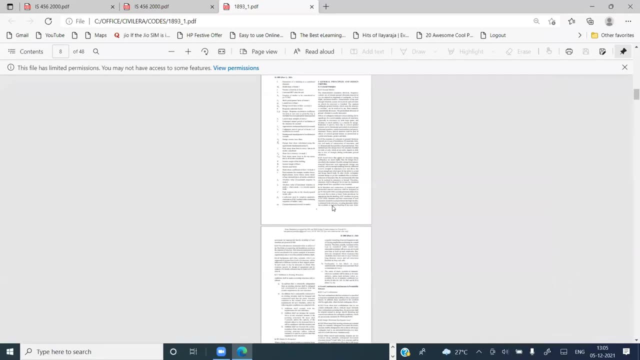 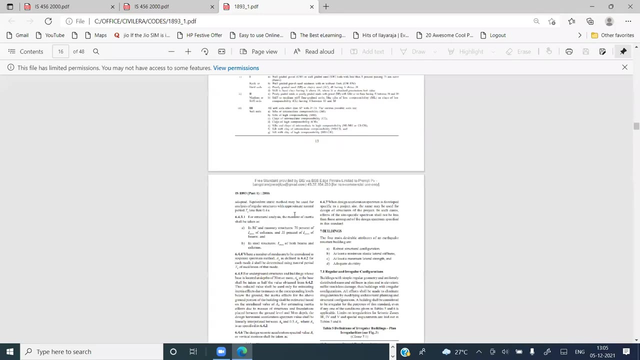 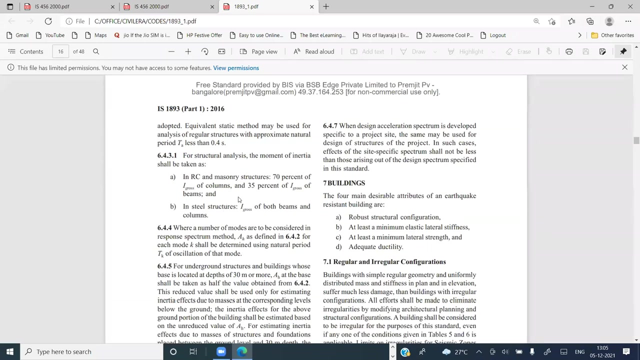 If you check 1893, I don't remember the close number, Let me just check it out- Yeah, 6431.. It tells you for structural analysis, This is a new code in 2016.. It was enforced in 2017.. 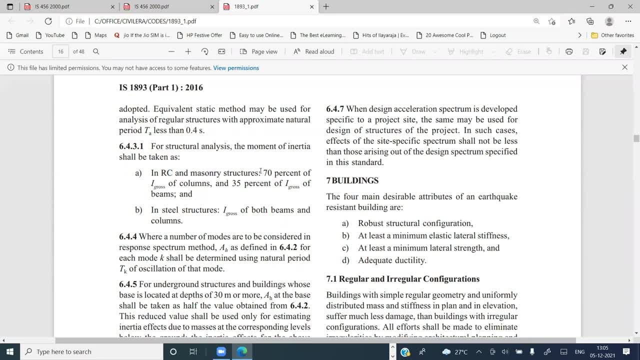 So it tells you that in RC and masonry structures, 70 percentage of igros of columns and 35 percentage of igros of beams needs to be taken. Yeah, So this should be your analysis value. Your I value should be this much. but generally many consultants do adopt this only for high rise buildings. 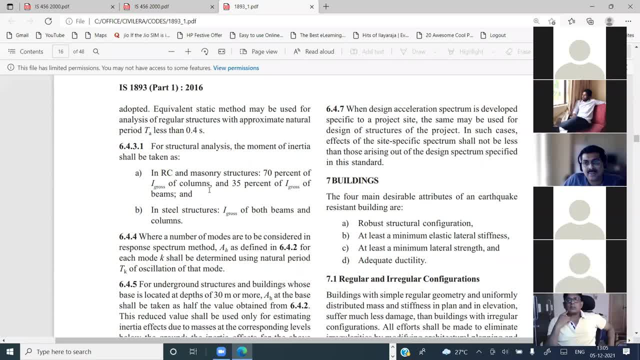 But as per code, you have to adopt this. So if you don't use this 0.7, 0.35 in that location, you are doing it as gross property. Got it? Thank you? So that option is to modify it as per this clause. 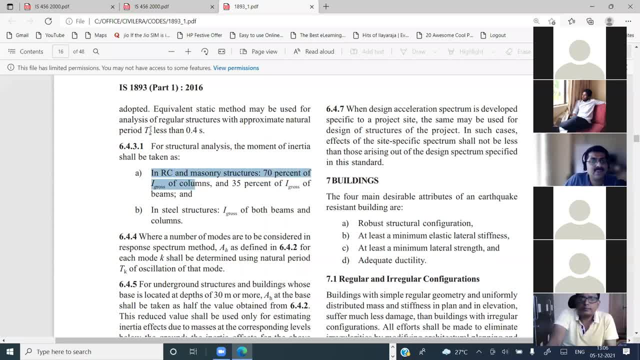 Any other question? Yeah, go ahead. I wanted to know how much time will it take to cover the topics included in E-Types course. That's a related question, Just like the stiffness. It depends on you. Yeah, Yeah, Yeah. 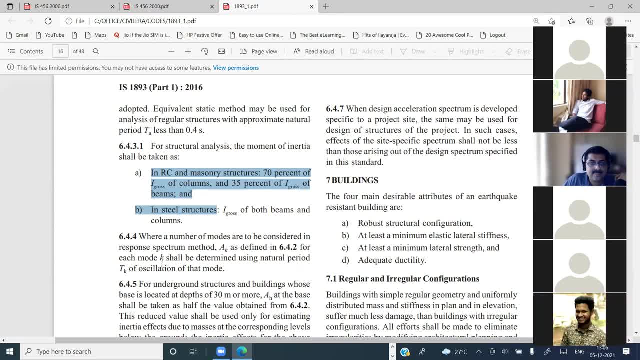 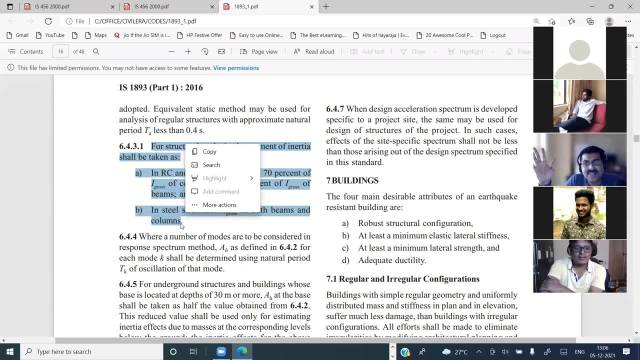 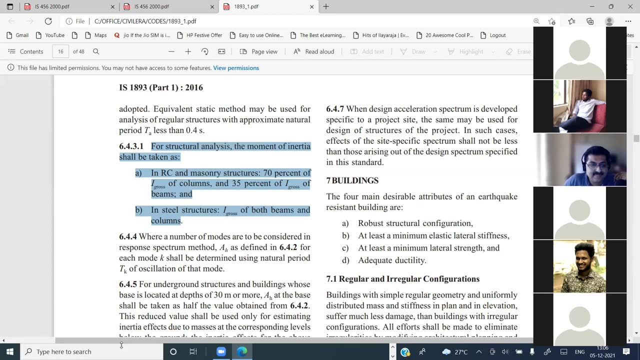 So it depends on how much time you're going to spend and about all things you are planning to learn. I would say you will take six months for good, learn No. So that's it, And I'm looking for you. Yeah, Not of this thing. 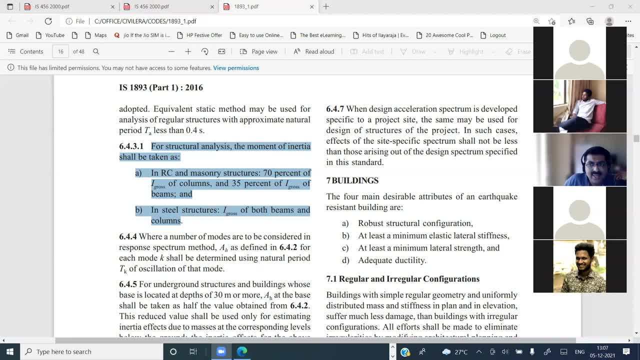 No, Yeah, mute, you can unmute once more and, yeah, go ahead. actually, I have recently graduated, yeah, and I am trying to search a job in design field, yeah, so could you help me out by suggesting something that I have time to learn: software, yeah, so 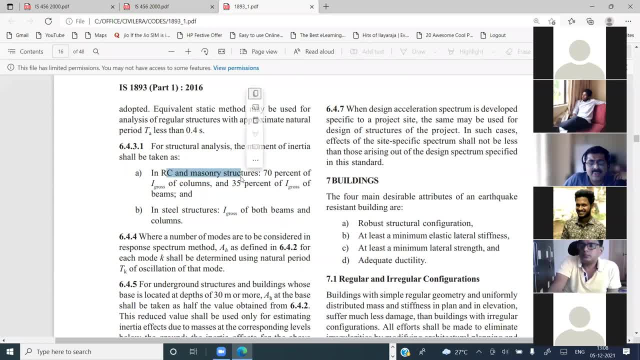 what you could do is, if you are enrolling for the program, you message me. if you are not, then you can be in the group and then you can continue to discuss your questions. so, as and when I have time. actually, I am planning to take a plan. 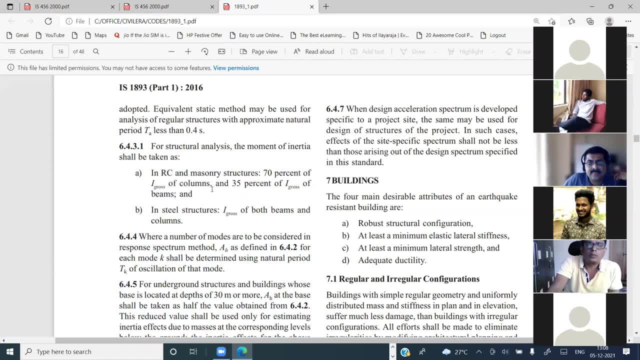 so that I have a rough idea of how much time will it take to complete the. so see, I will guide you with tips on how to attend interviews and how you need to plan your career, and things like that. so for that, some minimal understanding and some minimal. 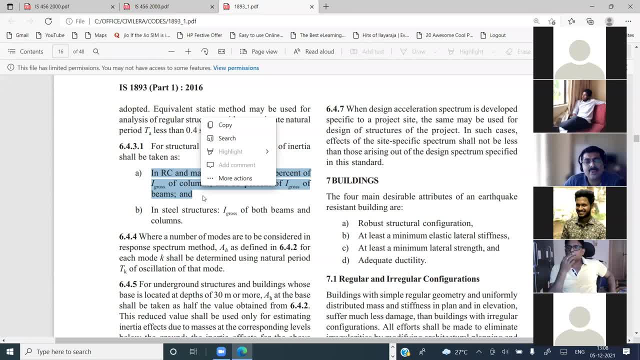 learning is needed at least one or two projects. you will have to do so. account minimum three to six months for a good learning. you cannot do it in one week, two week, three week. now again, it depends on your current level, which I don't know. so if you 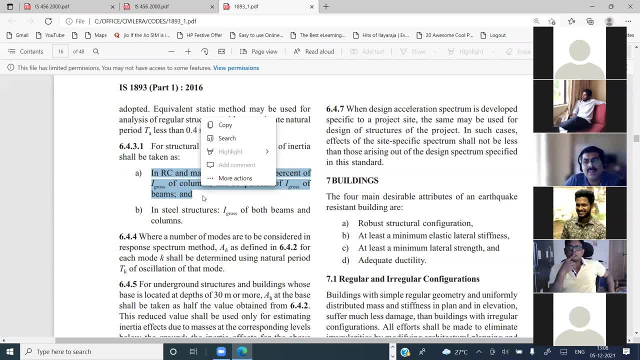 are currently in a good technical ability, then it will be faster for you. otherwise it will take around that much time minimum. you have to basically do projects to experience this. see, it's like learning four-year series by reading. yeah, you will understand. you will think that you will. 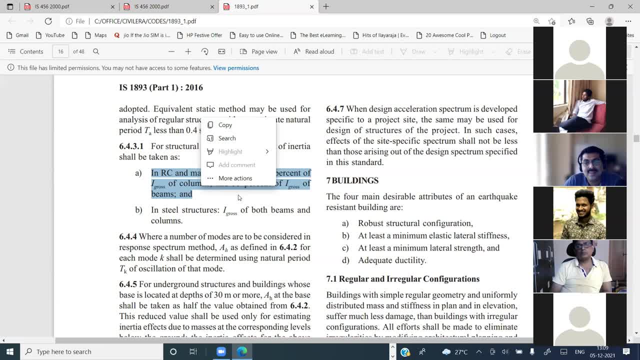 understand that. but then when you go to the exam it will not come there. so the same way here. you have to put many things together. it's not just doing a model. doing a model will not take more than half an hour. I have shown, you, demonstrated that. 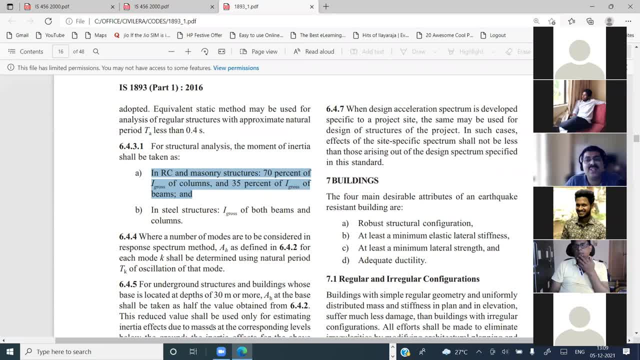 yeah, so you have to put a lot of things together, which comes when you do projects, so that can happen only over a period of time. so account some good amount of time. yeah, three to six months. you, if you are current, and you should have a great what you. 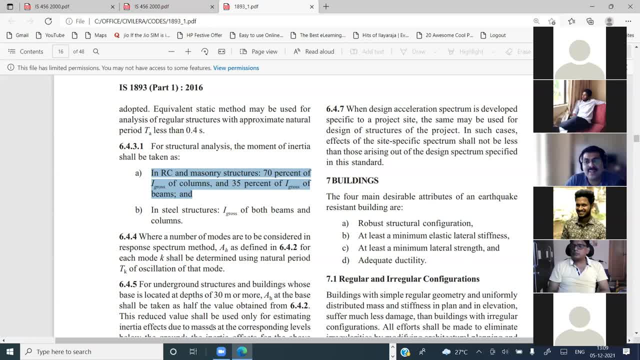 call logical skill in appreciating certain things. so if you understand most of the things I explained here, then you are good to go. yeah, if you didn't understand many things which I explained here, that means you need more time. it's not that you can't actually. 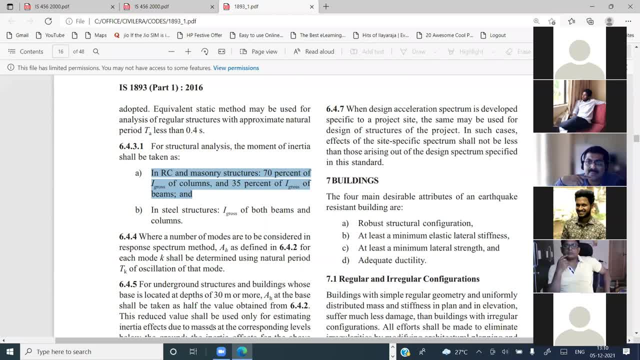 have some basic knowledge about t-types and some things, and I have completed my structures. I am taking structures and that I don't. I mean, I am taking structures, yes, that's good, but then that's not the criteria. yeah, but I think you appreciate things better than 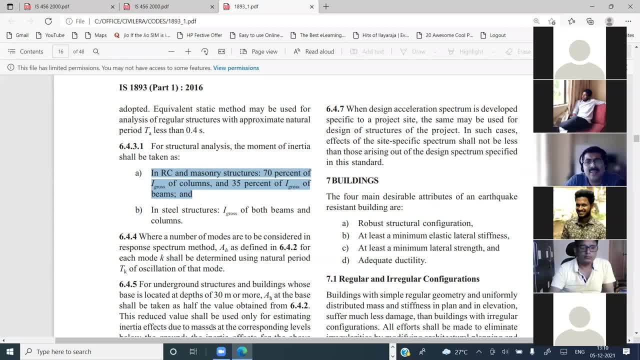 many. so, yes, you will need something like three months to do one project and maybe in that you can be ready. sure, sure, thank you. yeah, any other question? hello sir. my name is Amir sir pushna. the e-tab is: is it a link provide to let the 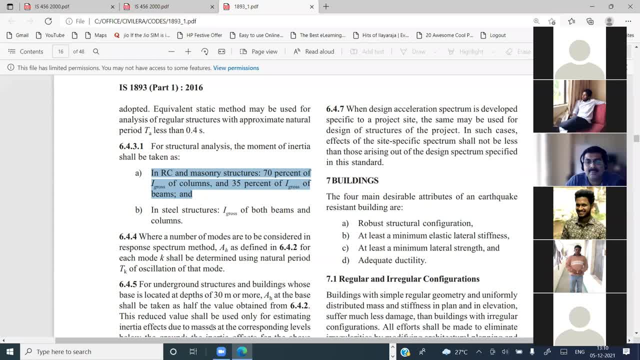 pb building ke liye so site to execute, karni me drawing provide karte. waha se detailing mil jati hai. sir, no detailing, koi software apko usi tarah ka final detailing to nahi dega apko dosra software sab. 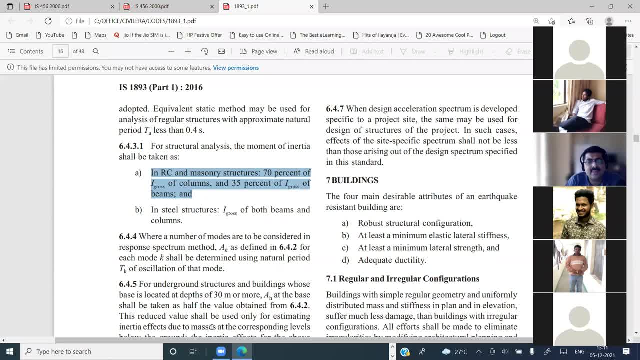 leke, detail karke drawing, final drawing karna padega. e-tabs is good for pb ke liye bhi, drawing kuch bhi nahi deta hai. it can maximum give you centerline drawings jo member sizes ka intent convey karne ke liye. 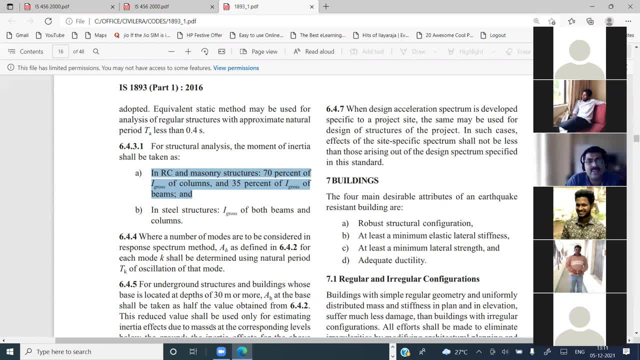 jo chahiye. wohi hota hai. it can't give you fabrication drawing. uske liye apko revit ya tecla ya autocad use karna padega. ok, ok, thank you sir. hello, hello sir, yeah, hello, yes sir, sir, which other 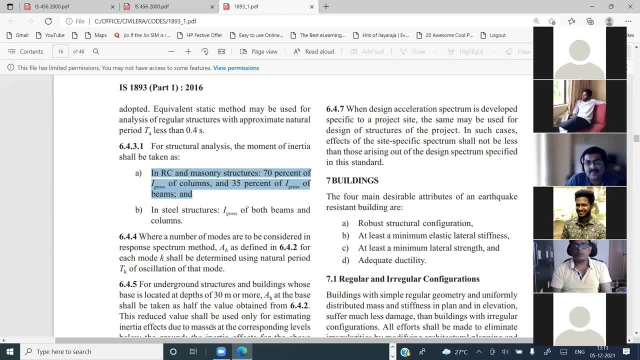 course are required for this design, apart from your shoulders? no, yes, see, for RC building structures. the course is focusing on RC mid-rise buildings and for that analysis and design you won't need any other software than ETAPS for level buildings. the best and the only thing. 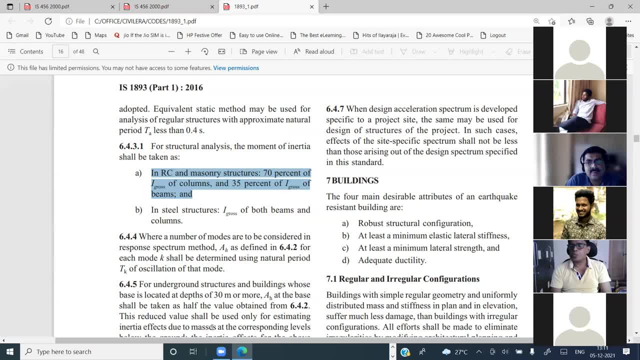 that you need is ETAPS for your analysis and design, for detailing and for your workflows. if you learn revit, that would be good, because all the modern companies are switching from autocad to revit. yeah, so now from autocad to revit when they shift. 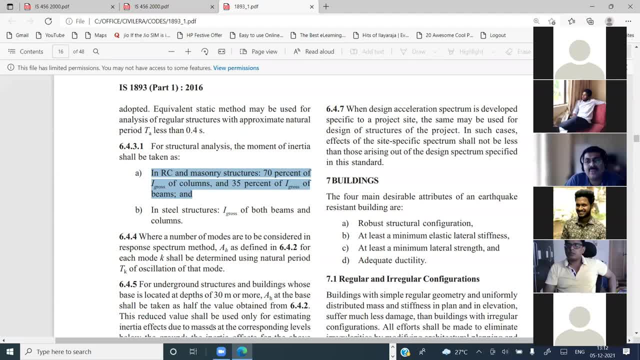 there is a huge difference in the way that we are going to work on that workflow. it's not just drawing production, there are a few things there. so if you are wanting to work in larger MNC kind of companies, then it's good to learn revit. 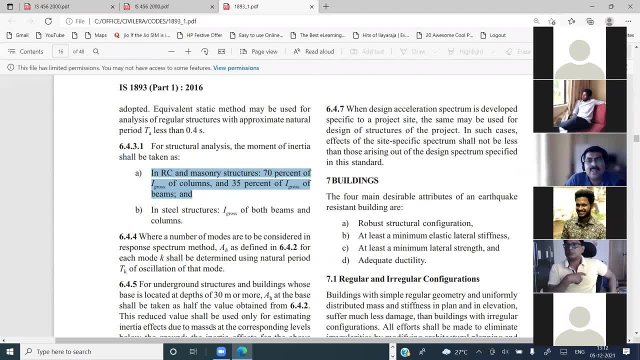 as well. but, as I start, if you ask me and the ETAPs, okay, and what about the course, sir? what are the course we have to refer? that's what I'm saying. we do have lot of courses- STAD and all that- but then, if your 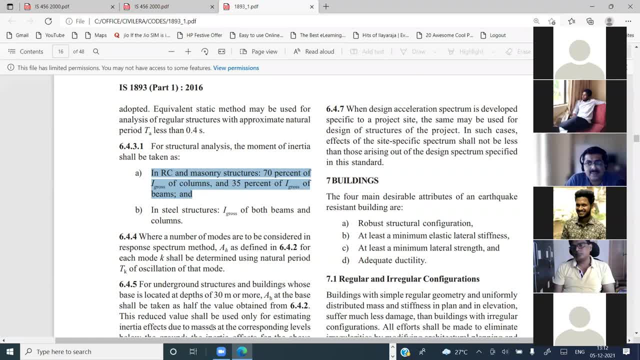 intention is to be in building sector, my suggestion would be to take ETAPs. don't waste your money on STAD. if you want, I have also, but then I don't recommend you doing that. and what about this IS course, sir? what are the IS course? 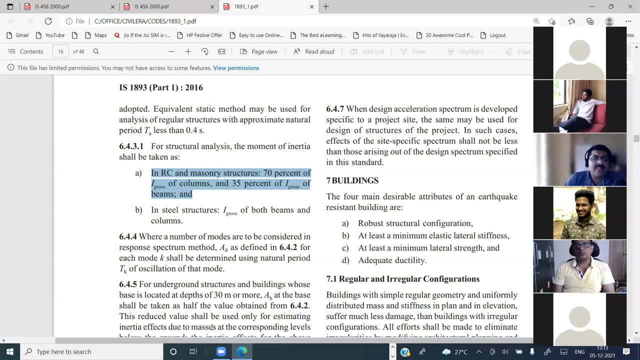 we have to refer. which are these? see, there are many, but the basic minimum thing that you will have to refer is IS 456 for generic country related stuff, 1893 for seismic, IS 875, part 3, for wind. 13920 for ductile detailing. 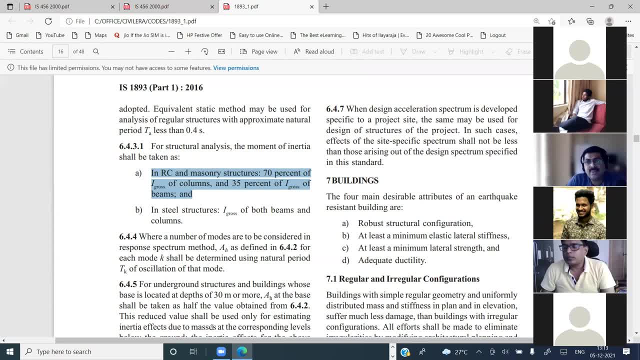 that's the basic course that you need to refer. IS 875, part 1, and 1, part 2. these are there, but then that's not really needed. SP 16: we do use. that's a handbook for your easy calculations. yes, instead of using the 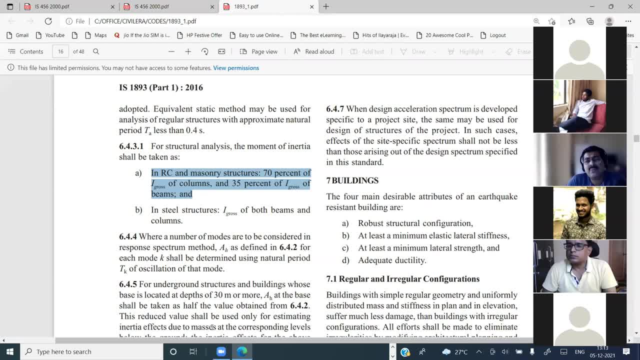 IS 456 formulas, but it's an extension of IS 456. sir, one thing I want, one thing I want to know, sir: after you produce the right design, appropriate design, the best design, do you validate through this all these SP 15 and all those empirical formulas? 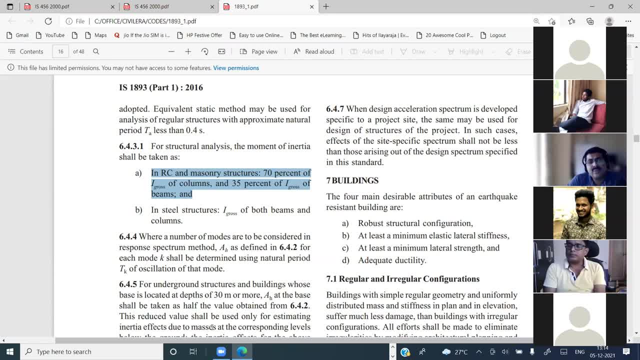 manual, not everything, see. first thing that you need to validate is your analysis behavior. yeah, so once you have good experience on how it works and how it is, you will be able to understand if there are any kind of errors in that. yeah, so your analysis validation is. 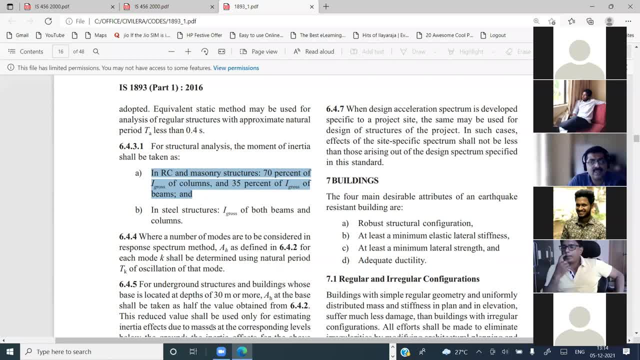 very important. you need to ensure your area method calculation and ensure that your reactions are matching. and once you validate your analysis, then design validation. see, I will ask you another question. see, you are, say you are using a boat, say you are traveling in a boat. okay, you. 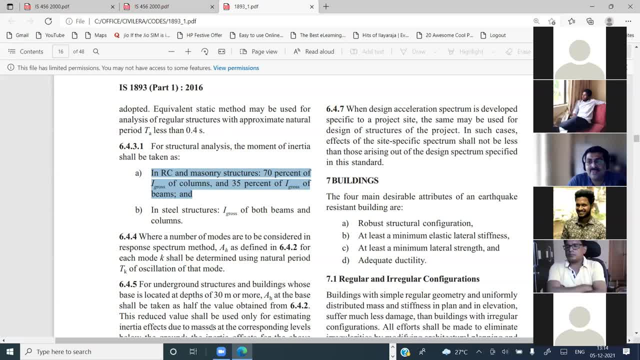 trusted the boat guy till you went into the middle of the river. yeah, that is. you trusted ETAP till it analyzed. now why are you not trusting it when you are designing? because designing is a very simple step compared to analysis. so that's why I am telling. 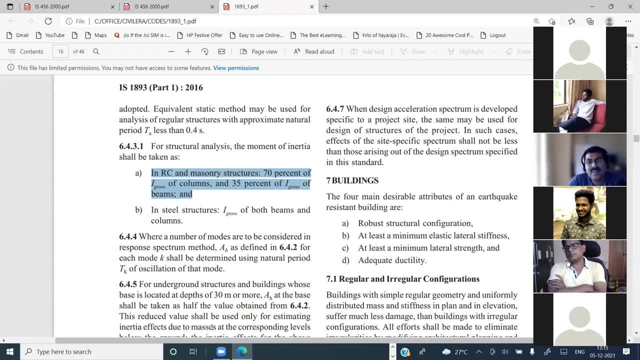 you the importance of giving the parameters correctly. yeah, yes, of course you can validate it by manual designs. that's also covered in the course as a beginner. yes, you have to do that. yeah, you can easily do it. you can use SP16 handbooks and do your. 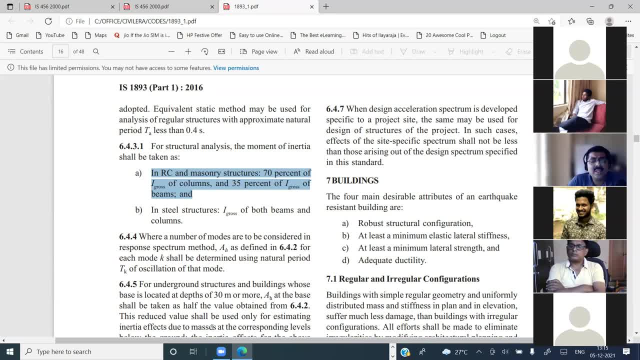 validation, it's not a problem. but then there are certain things which you may not be able to validate. yeah, if you release the torsion, you will not be able to validate the analysis part of it, how it is getting redistributed. things like that you cannot validate manually. 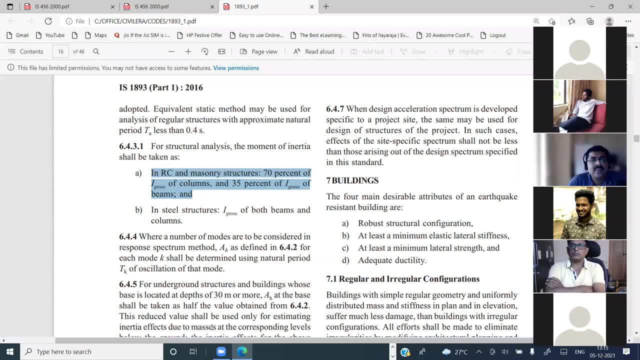 even if you adopt any method, like canis method or moment distribution method- these are plane frame analysis- it will not account for the 3D effect, say, if the load distribution- because there are seismic loads as well, so that cannot be done- validated manually 100%. 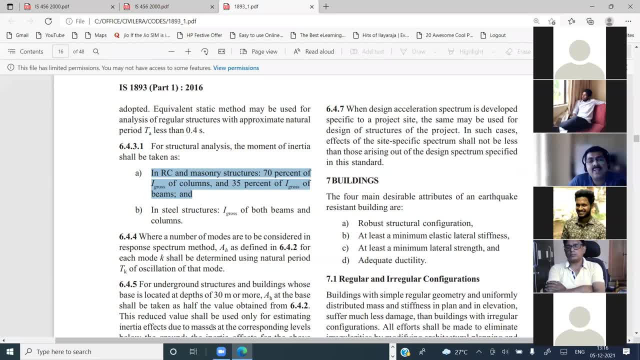 but you get the clues, you get the behavior, you get an idea based on the behavior that you expect. if you don't see, you can validate it. in that way, you cannot exactly match values in analysis, so can we design foundation 3D? I already answered this. 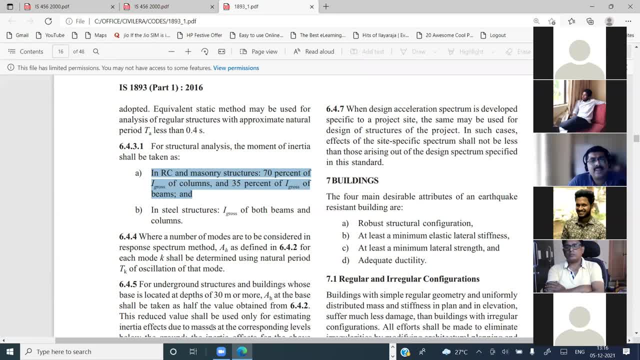 see foundation don't need a design in the sense. see, many designs are thumb. rule is how many of you appreciate it? I don't know. if you look at slab design, if you go by IS456 method, that design is in fact a rule of thumb- triangular, trapezoidal. 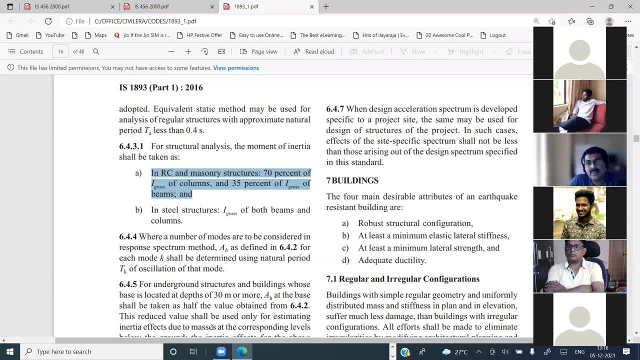 load distribution is. thumb rule is shell behavior is different. so if you get a shell value, that is, if you get a moment value from a shell analysis, then how much time will you need to find out the steel? if you are using SP16, it is MU by. 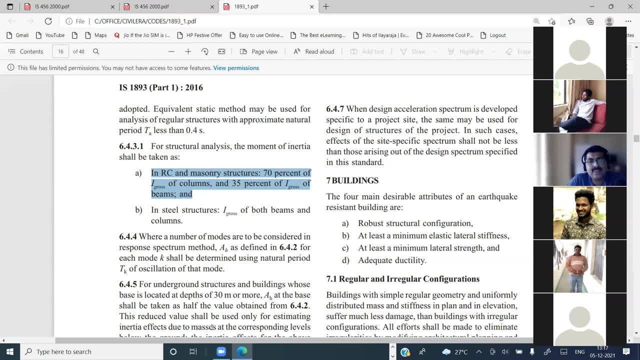 BT square, you get the PT. so what are you talking about? there is no much design involved in an isolated footing design. you can quickly, very quickly, in five minutes you can arrive at the result. but if you are using raft- I mean if you are designing raft or- 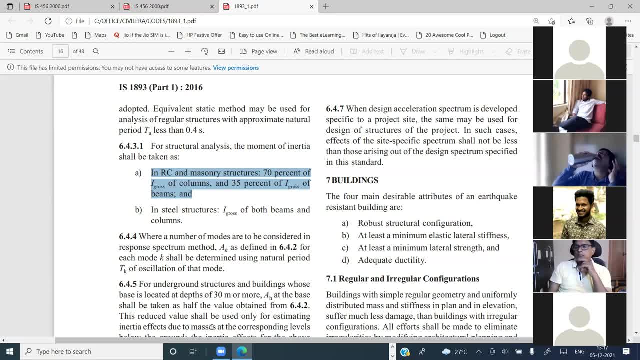 if you are designing a piled raft, then you can model this as a plate or a shell in ETAPS or SAFE or STAT or whichever software you want, and then get the results, get the moments and shear and design it very quickly. there is a strip based method. 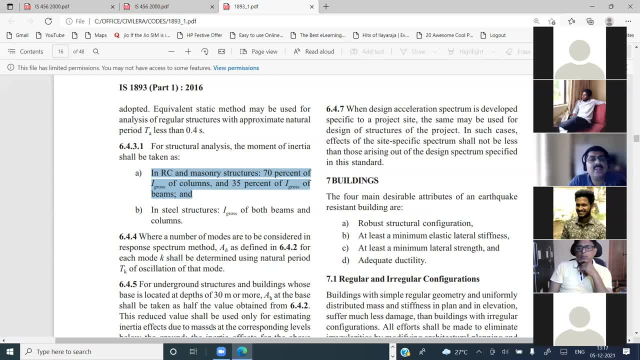 of design in SAFE and ETAPS which you can adopt, but I don't see it necessary, especially if, at this point in time, master the superstructure, in that you will understand what shells are. then, once you start understanding how to interpret shell results, you will find different. 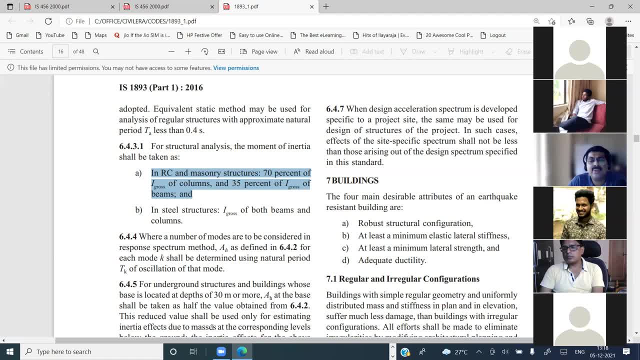 methods for analyzing a slab like that or a foundation like that. it is much simpler than you think means if we are master of ETAPS so we can design or we can calculate the loading or resisting bending by the foundation. yes, you can, but you need to know. 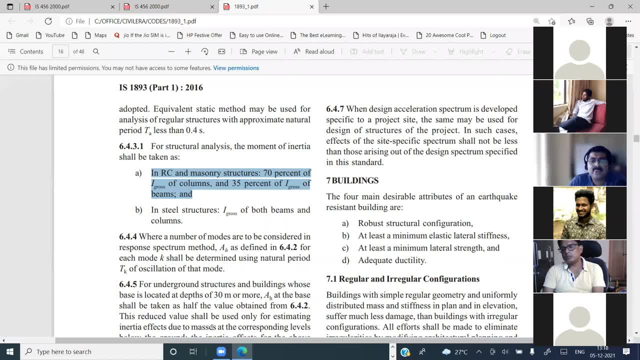 how to use it. but for foundations we have a separate course on covering all the aspects of pile foundations, raft, isolated footings, combined footings, everything that's a different course altogether, but the same tool you can use, but you need to know how to use it, what. 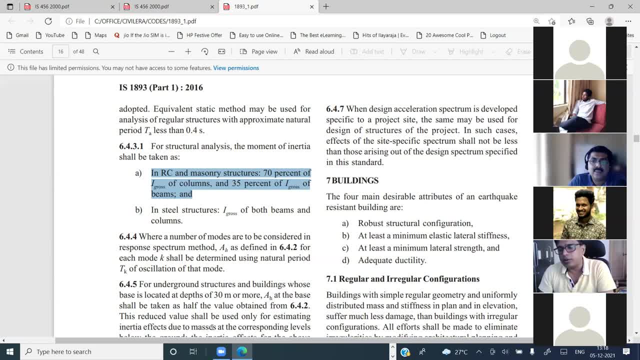 is that? what is that course, particularly that you have mentioned right now? that's a foundation design course. foundation design course, it's all about in it's in etabs also. yeah, yeah, see, some of it you can do in etabs, whatever you can do it in. 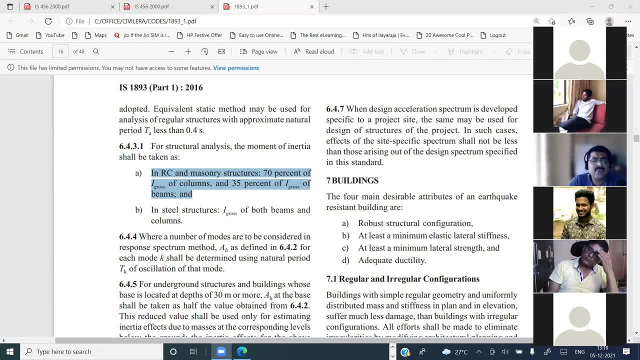 other software you can do in etabs also, but there are certain things you will have to do manually. what is that property modifier you all? it may use the thing. structural property modifier, sir. property modifier: constant, constant germ use: see explain. to explain I need two hours, see. 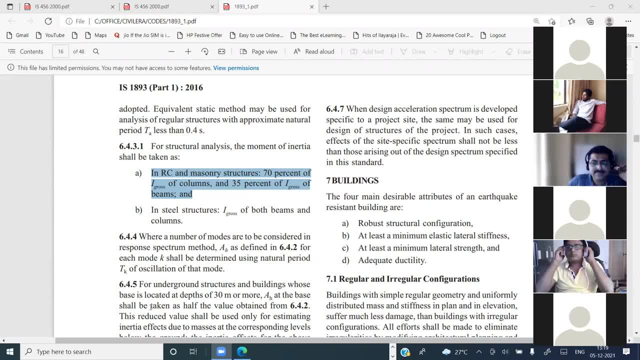 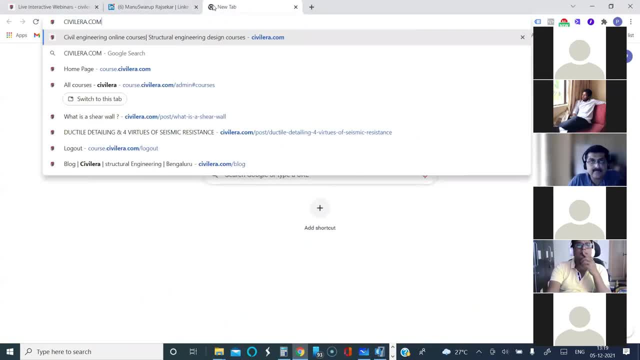 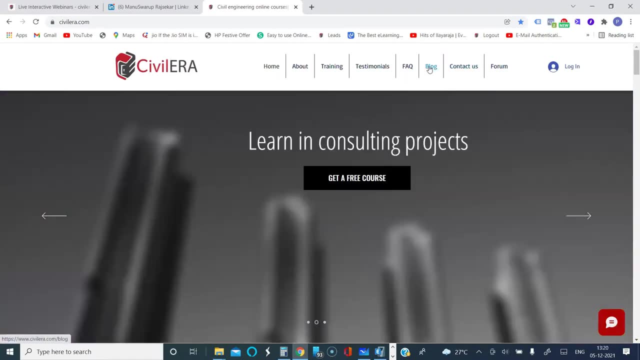 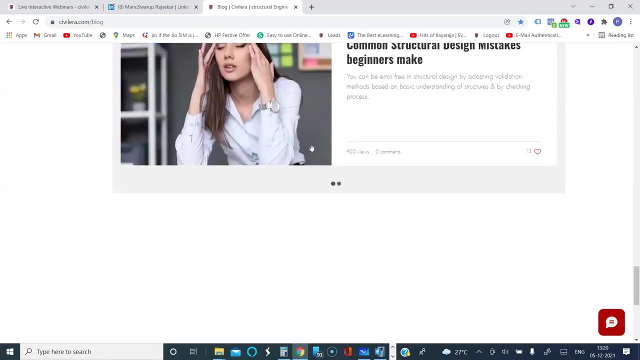 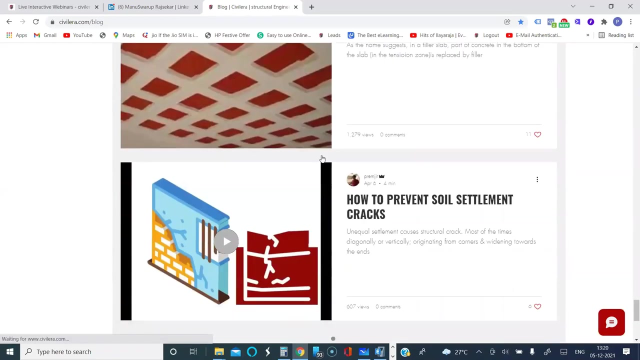 I have a blog on this. if you go to civileracom I will show you you. and if you go to blog and if you come to the very first or the very last, the first blog that I wrote, which will be at the end, is on torsion. 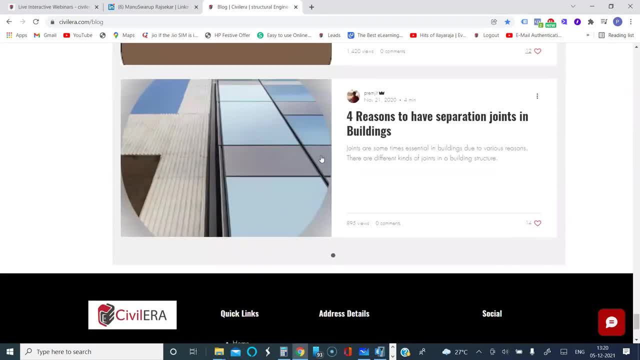 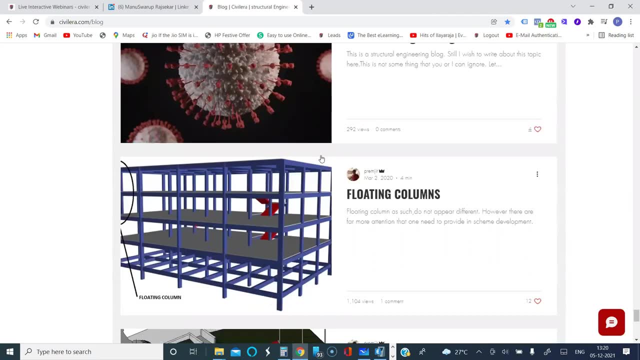 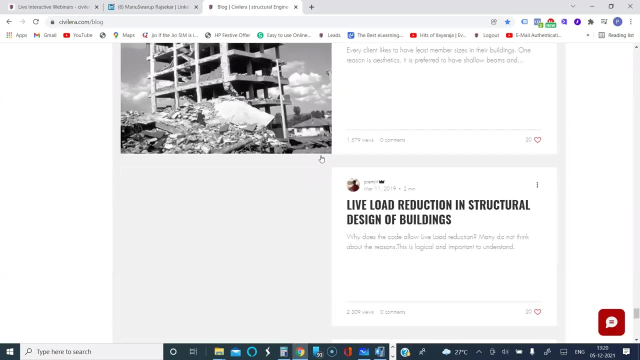 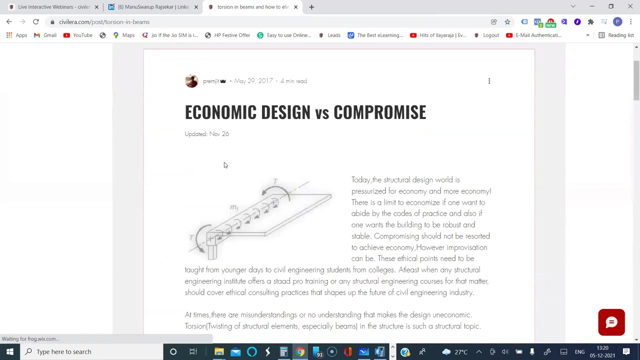 you read that, it gives you complete understanding of what torsion is and why we are releasing. see, basically there are two kinds of torsion: compatibility torsion and equilibrium torsion. yeah, so now equilibrium torsion needs attention. compatibility torsion you can leave it out. yeah. 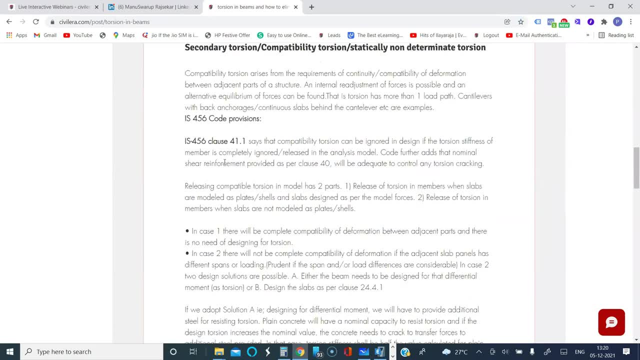 so here it tells you everything that you need. basically, in a simple language, the code is asking you to design torsion by a formula. if you know, yeah, so that formula is a term rule. now, if you release, same thing happens. yeah, so release of torsion and using 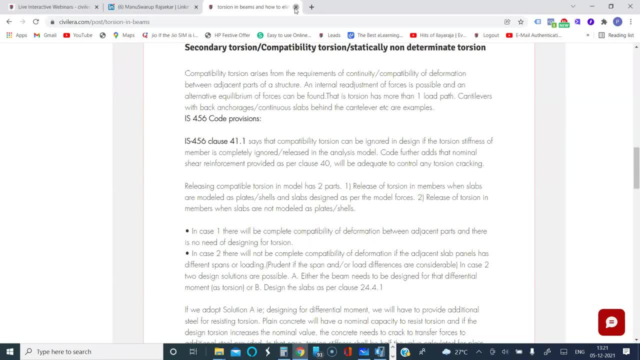 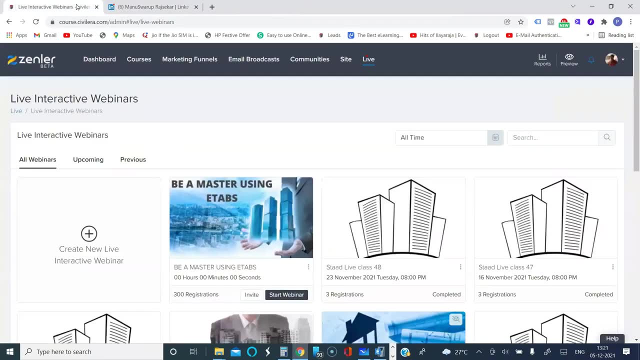 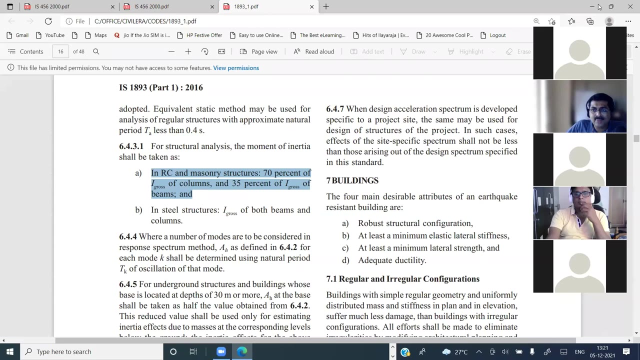 that formula is same, but only thing is, when it is a equilibrium torsion you cannot release like that. yeah, why you read that? you will get to know. okay, sir, thank you, yeah, no problem, so yeah, so yeah, any more question? it's almost time we have to wind. 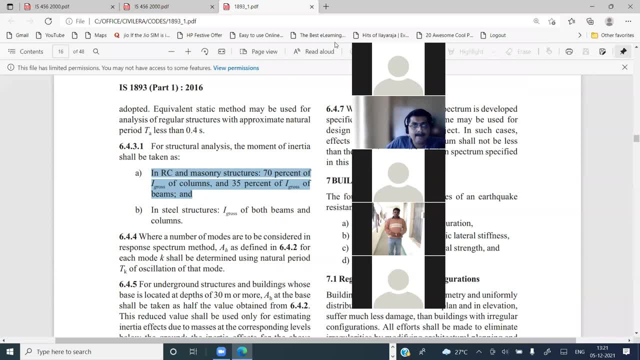 off. another question: yeah, yeah, go ahead. so you didn't tell me how to detail from etabs to autocad. i quickly showed you how to interpret the result and sketch the beam detail. so if we will have a separate session sometime or i will share you the, 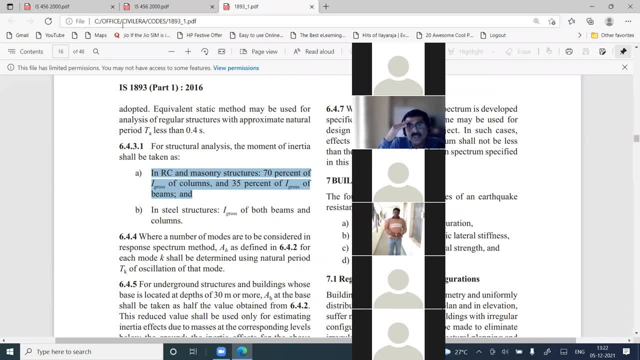 video. something will be there in your, in my youtube. you can go on my youtube channel. there are one or two videos on beam detailing, one or two videos on column detailing also. so i suggest you go there and check it out, because in a one hour or two hours 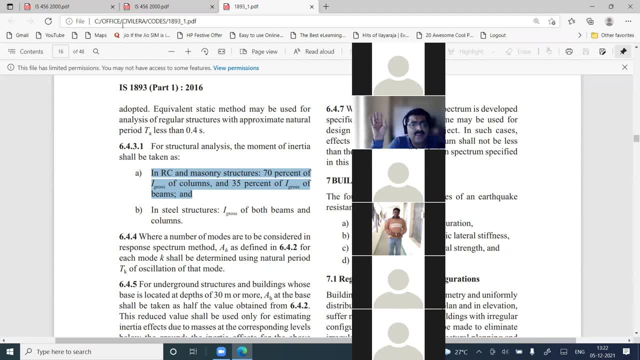 webinar. i cannot completely show it. yeah, etabs cannot detail everything. you will have to detail manually, either using autocad or using revit. etabs can give you, at the best, some design intent drawing, but it's not great to issue to site. yeah, so i generally. 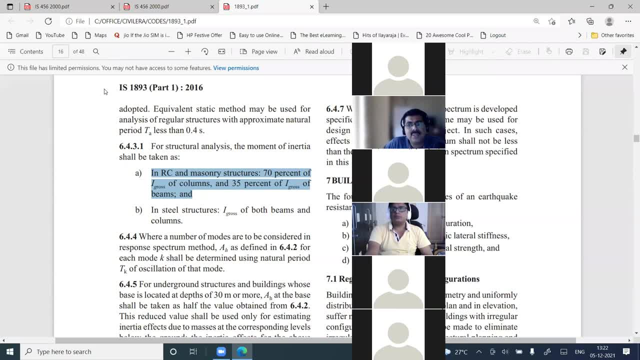 detail in revit, so you have to use a separate tool. you can interpret and make a sketch. any other question? yes, sir, yeah, go ahead. mhm, see, there are so many things to explain. if you ask this: 0.8 percent is the minimum still needed? yeah, so if you are still using more than, 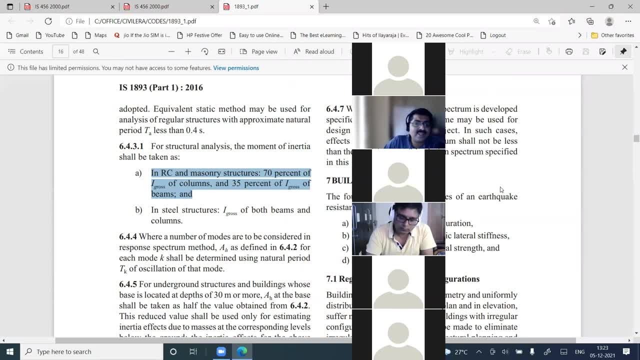 0.8 percent is the minimum still needed. yeah, so if your skill is more than if it is more than needed, i mean more than 0.8 percent, of course- you have to give that now 0.8 percentage of what many think, that 0.8 percentage of provided area. it's not like that. 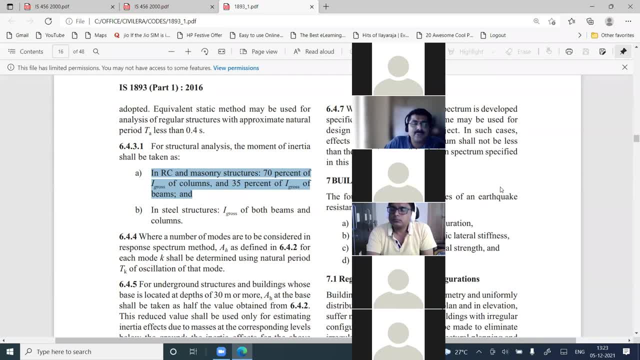 0.8 percentage of required area to read uh to to resist the compression. that's what the code tells you. yeah, so if your value in etabs is 0.8, that definitely and clearly means that your size is more than needed. got it so you can refine it and reduce uh one second. 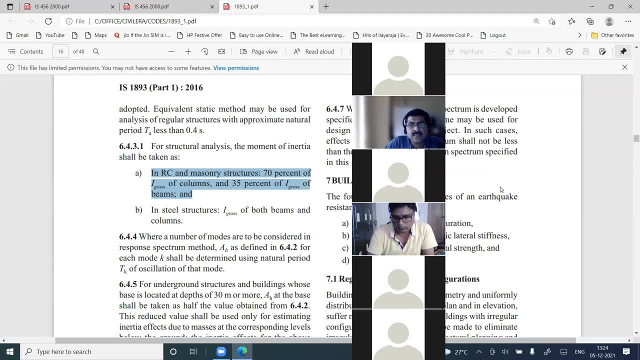 so, uh, you need to uh reduce the column size. you have the opportunity to reduce the column size. so we look the column size. if it is seen as 0.8 percent, you, yes, thank you. any other question? so one thing i want to ask, sir: yeah, apart from learning, apart from learning etf, sir, 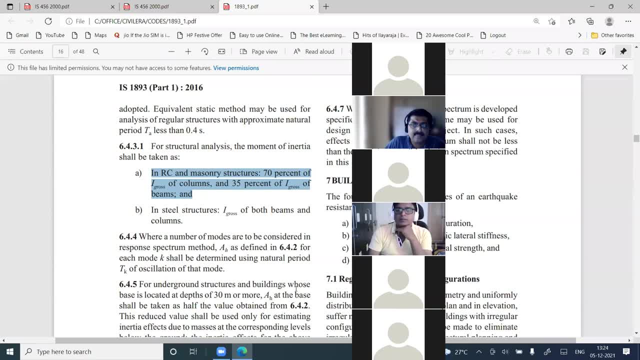 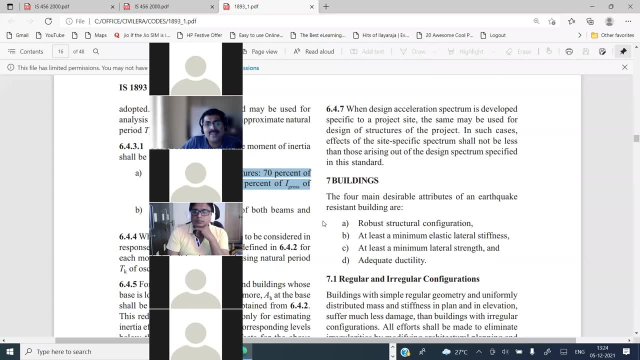 what should be done adjustably to master analysis and design. but, sir see, you have to have that understanding, so you need to go and, uh, if you want to be a master in analysis, you have to revisit your uh. test principles text: yeah, practice books, yes, and master that. 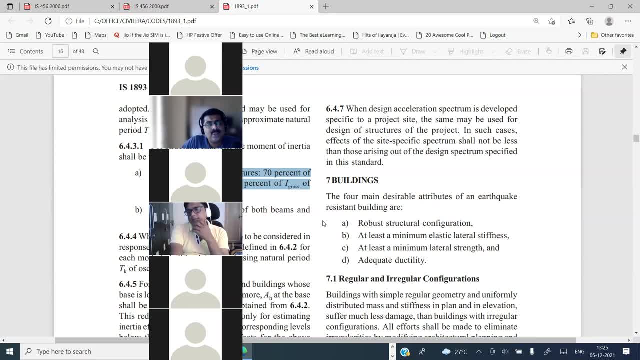 uh, but again, as i said, there are a few things that you cannot uh do in hand calculations because, see the presence of she of all, the 3d analysis cannot be done manually. but the plane frame basics, yes, you need to revisit your uh first principles, but logically you can understand from the course: yeah, but again, the: если you are to Lamwait, you will need theMr Fox's and Mr Kang's. of course. we are complete problems. so if nobody else sits after you, you can give a written review as an expectation of this performance, but no one really cares about it. 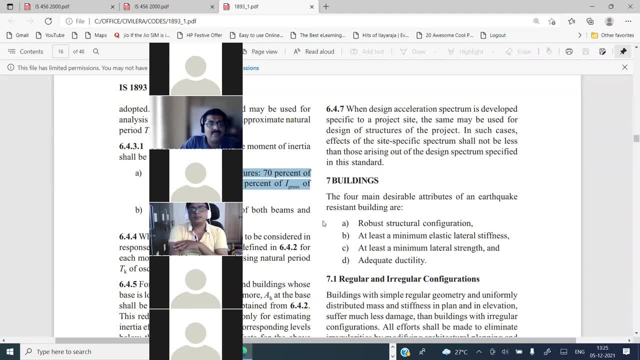 because- but we see possibility for this example- that this is the book there is certainly given on paper. BTU asks: you course you will be knowing what is meant by reorientation, orientation of column when it changes what happens. all that will be covered in a very systematic and in a logical. 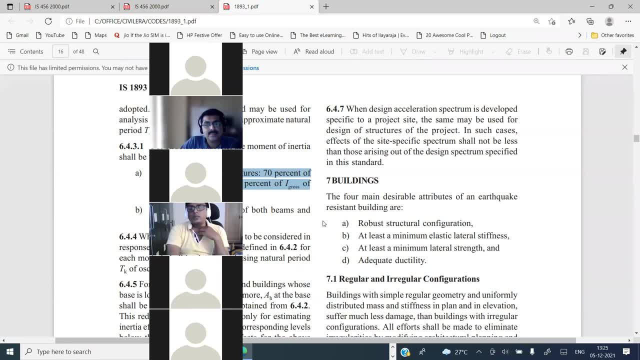 manner. See the type, the way which you explained, sir. it is quite nice, sir. Actually, I have never seen such a person actually having a good technical depth in your knowledge, sir, Thank you very much. It's basically again coming from when I was a student, when I was. 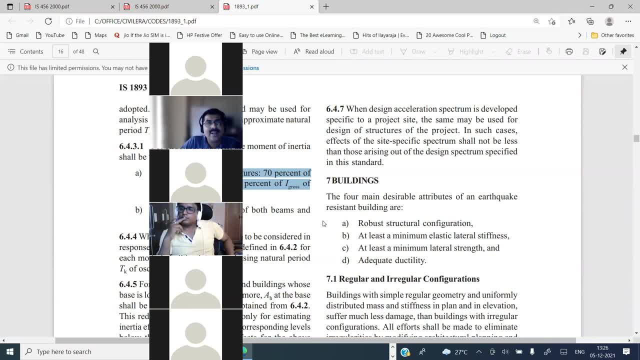 young and when I was struggling to find answers, I had the same kind of question. So I decided that I will start with my doubts, which I had when I was a beginner, And then I have, over a period of time, trained a lot of students. So whatever they ask, I note down- I don't. 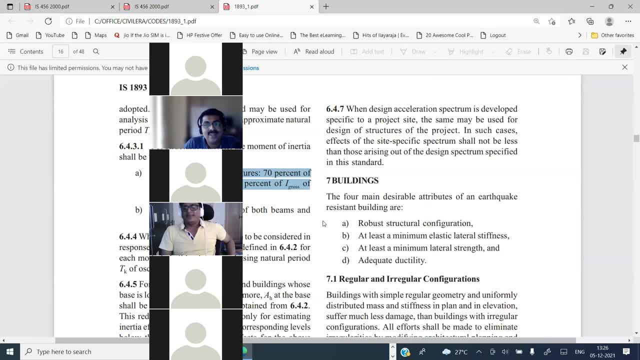 leave even a small doubt as an unnecessary doubt And I have developed a certain style of questioning and a sense of uncertainty And I have developed, develop the course from the doubts of students. So it started from my doubt. even my wife is a civil structural engineer, So she had doubts when she started And she was a teacher. 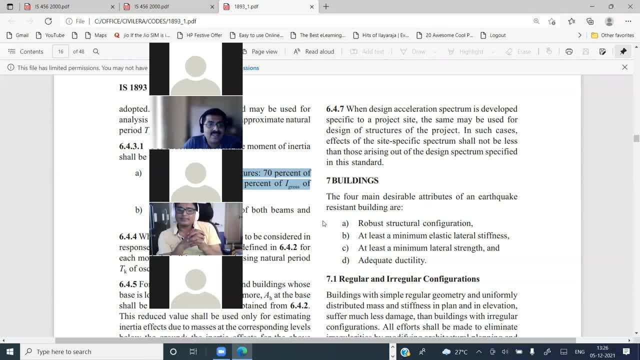 So she has considerable experience in teaching students. So all this we gathered over a period of time And we decided that we are not going to leave even a minute out so that everything is clear to students. In your ETABS course, do you give this type of parallel explaining, just like you are right? 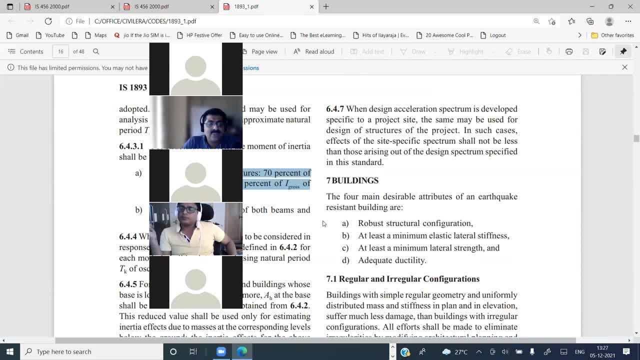 now, Yes, yes, And you also have the opportunity to ask me see. Yes, Yes, And you also have the opportunity to ask me: see, I share you a blog, So if you don't understand anything in that blog, you have a premium. 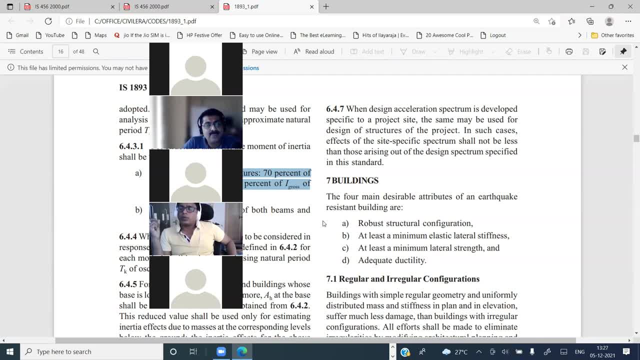 community where you can ask me that question. Even in the free group you can ask. But only thing is: I will prioritize other things And when I have time I will answer here. But in the premium community that is my priority. So I will be answering you more. 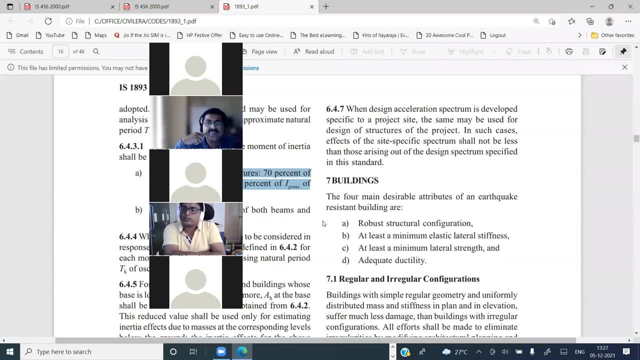 I'm a member of that community, sir. What's a similar group? structural engineers? No, for the enrolled students, you will have one more which is much more premium. Yeah, Yeah, no problem, Sumit, any question? 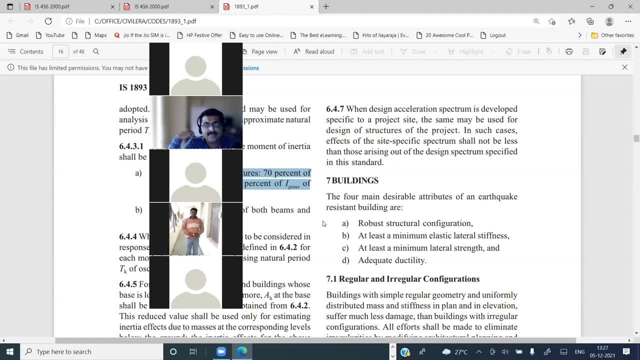 Yeah. so that again is a long process We cannot completely discuss in this. What I can roughly say is that, as I said, consistent approach is fine. If you either pin or fix, go with that throughout the project. Now, generally, if you have hard strata, as somebody had pointed out, if you have hard 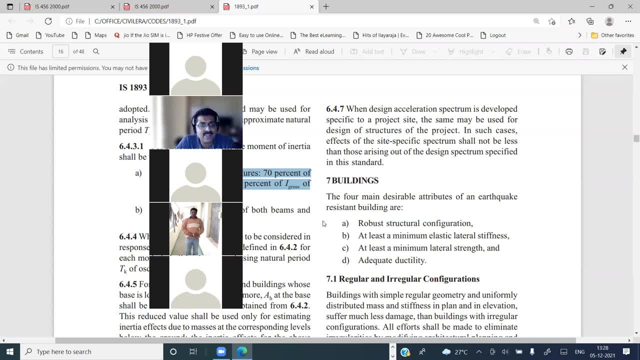 strata, you can fix it because you will have more of fixity conditions And if you have compressible soil, go for a pin condition And when you have raft and pile raft and all that you can fix, When you have isolated footing you can pin it. I would love to explain. 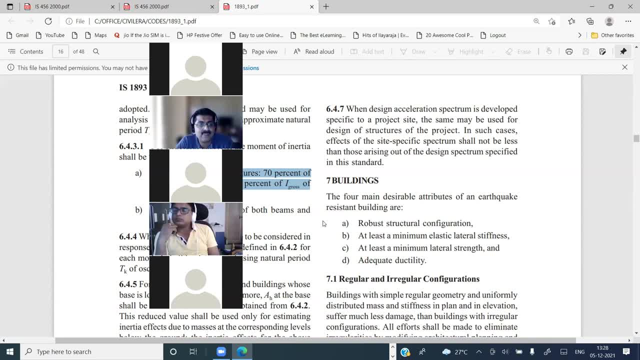 it, because it's not limited to what I said Now. there are more things to be explained and discussed about that, But unfortunately we don't have enough time to do that, So we don't have time for that. But there is a number of things. What I would suggest is you take a model, one structure. 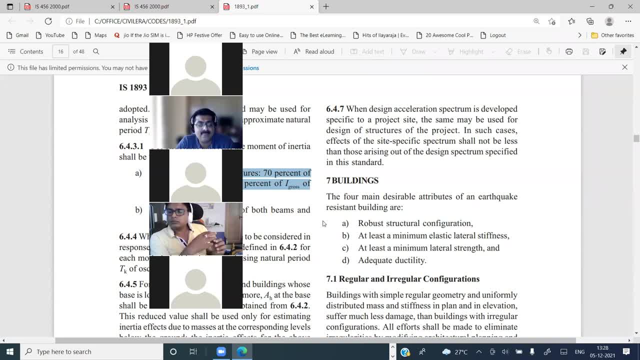 you pin it one structure, you fix it. or take a simple frame: one frame, one, you pin it, one, you fix it and appreciate the differences. Now what I'm trying to say is, yes, you can go and design both. the design will be different, But in most cases both will behave both. 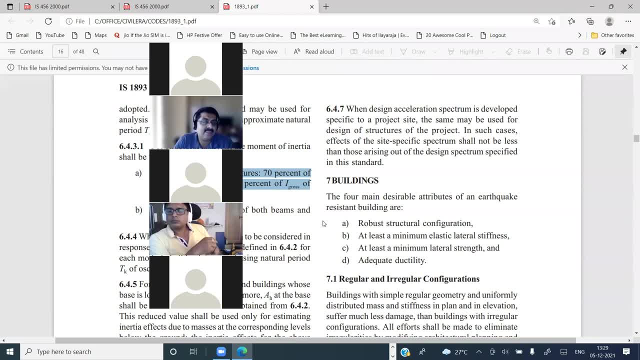 will give you no problematic result at site. you don't have to bother much. there are situations where you have to bother, but then if you pin it, whatever you get, you detail it like that, you fix it. you just take the result, detail it like that it will be different. say, for example, if you pin, your foundation size will be 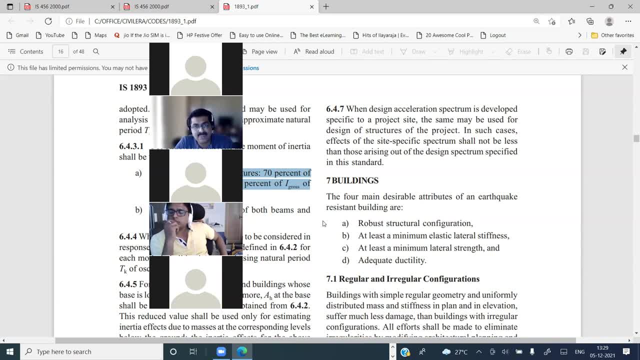 lesser, because your moments are not, but your column size may be higher and when you fix it, your foundation size may be lesser, sorry, more- and your column size may be less. yeah, yes, why is it so? because, in the reality is, it's neither pin nor fixed. it's in between that, yeah, both will work. 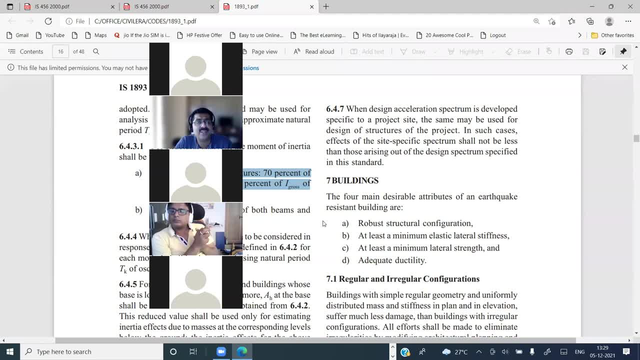 but you have to have consistent considerations after issuing foundation drawing with a pinned condition. if you change- oh column is coming larger, so let me fix it now- then you will have problem because you already issued your foundation and reconstructed a smaller size footing. now you are saying: column is coming larger, so i'll fix you. cannot do it. you cannot change it in between the 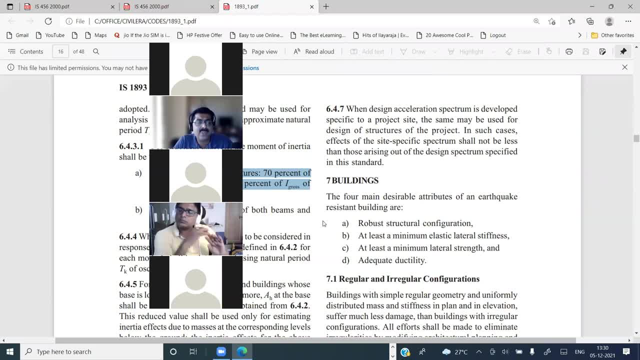 project. yeah, but a rough rule is that when your soil is compressible, you go with pin. when the soil is hard, you go with fixed. or when you have a raft which is very much heavy and uh, which can replicate a fixed condition, you go with fixed. the course is covering it for this judgment. uh, i am not sure about literature. 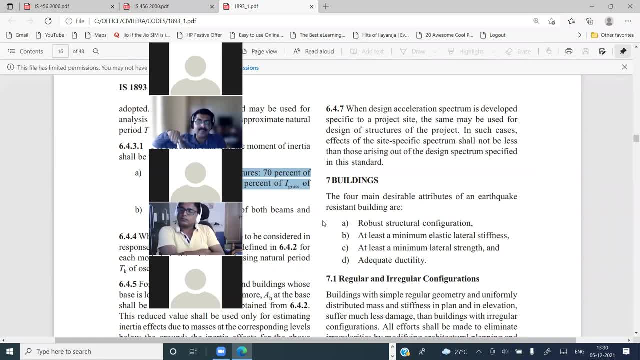 but based on my experience, i have covered a much more uh elaborate explanation in the course. no, sir, i am not asking what about that. in the bubbles uh balls handbook you can check. there may be some information available. i'm not remembering. but then i mean, in reality you will have to bring in the soil structure interaction. so that's what you have. 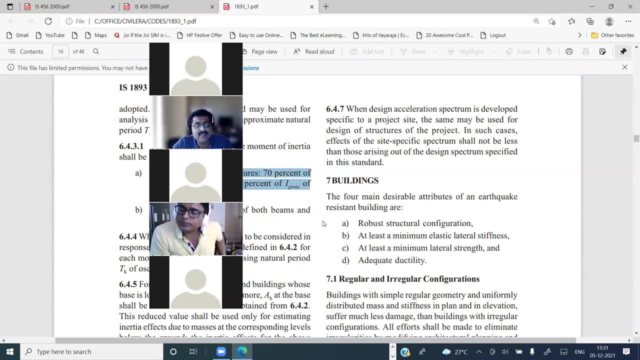 to do. if it's a large structure, you can model a raft and bring in the subgrade reaction into play, and you can analyze it in that way as well. so if you look at uh large structures like burj towers, burj khalifa and all that, uh probably they would have had an 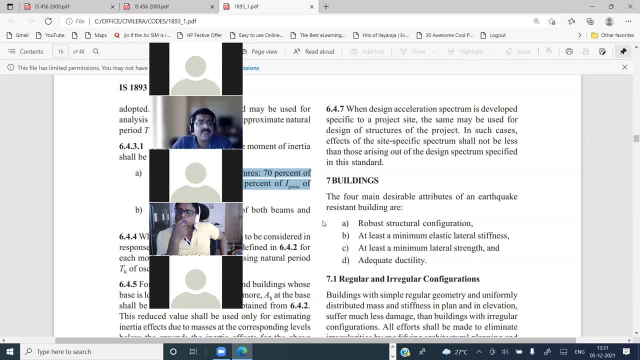 integrated model, where foundation and the superstructure is modeled simultaneously in the same model. but if you start doing that for each and every small building, your analysis- uh- is becoming complicated and the accuracy that you are getting is not that much desired. you don't need that kind of accuracy for a one-floor building. yeah, so you can do that, but if you 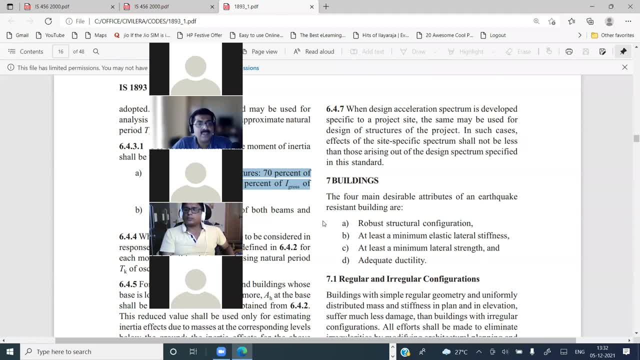 your structure has a lot of redistribution ability, so you don't need that kind of accuracy for a one floor building. that's why we are okay to fix a pin, but when you need more and more accuracy, even 1 mm deflection becomes critical. in such situations, you model everything integrated. 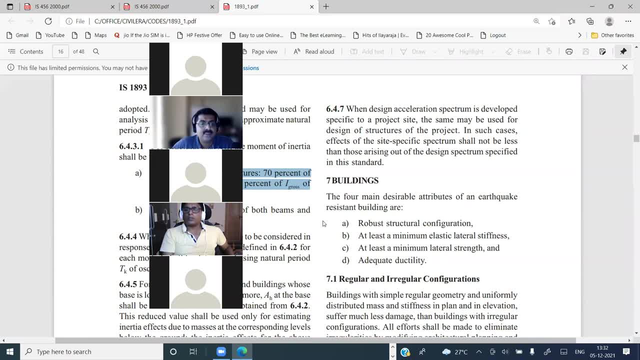 and then capture the soil structure interaction. yeah, so in such cases you can model your raft in the same building itself, in the same superstructure building itself, and then provide the soil parameters in it and get the correct, more accurate result. you can use save. you can use c tabs you can use there are better software when you want to do. 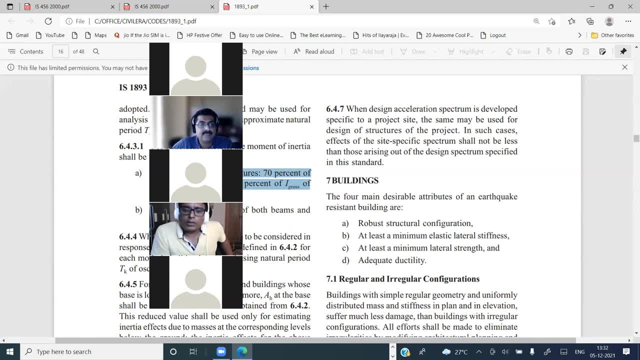 that, sir. one thing, uh. i think one question has still become unusual. one of the participants had made a query about the judgment of providing a secondary beam in a slab actually, so that i already told there are three reasons for having a beam. one is most important aspect: if you dis uh, you decide for uh having a. 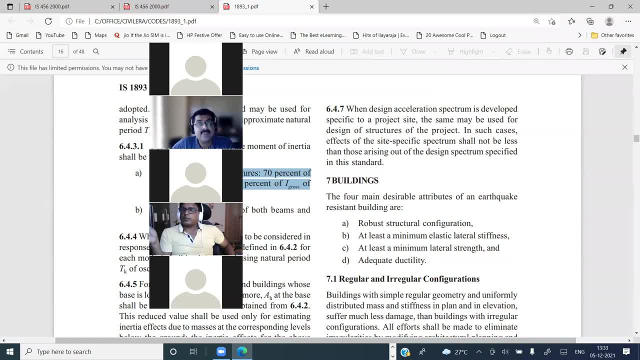 beam or not, apart from architectural and- uh, functional is that? uh, if you, if your thickness is very large, yeah, so if your slab thickness, i gave you l by d rules, two locations where you need to refer. so if your thickness is coming, something like 300 for a residential building, 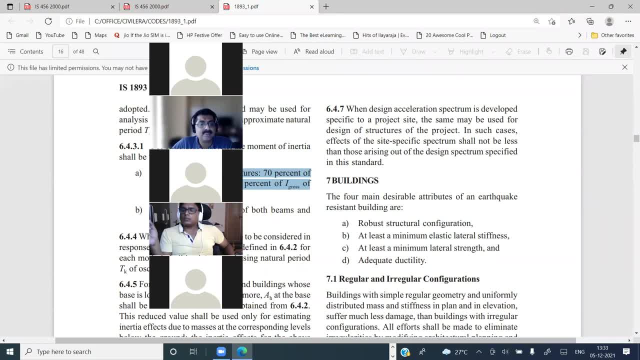 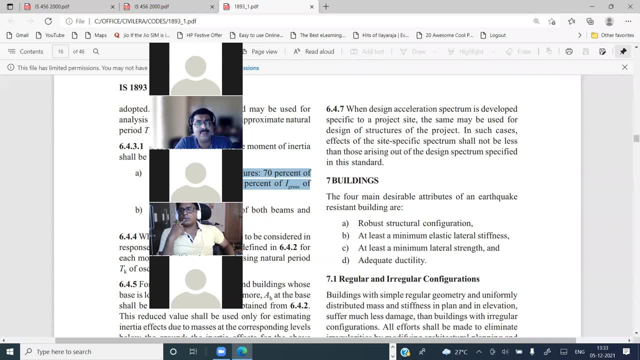 go with 300 thickness. second reason for having a beam is your uh wall coming on top of the slab. try to avoid that and give a beam there. third situation is you have to tie the columns in either direction. so these three are the requirements. so, based on that, you have a sensible plan arrangement. 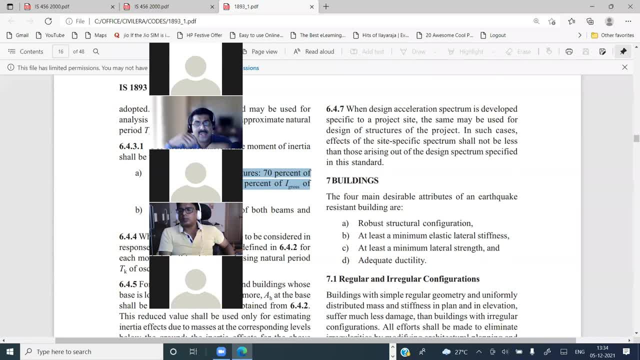 meeting all these three together. so what i will do in the course is i will give you examples which has these kind of complications and you can scheme and ask me questions about that. fine, so i think we have to wind off now. any one one more question i will take and then we will wind up for the day.